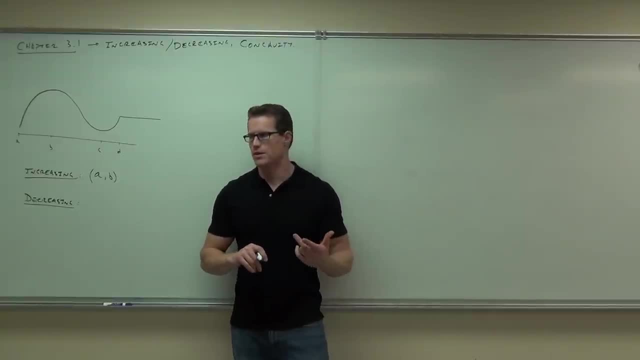 something special happens At B. it's no longer increasing. We'll talk about that later. How about another interval? Do you have another interval where we're increasing C to D? C to D works good, because from here to here we're growing up. 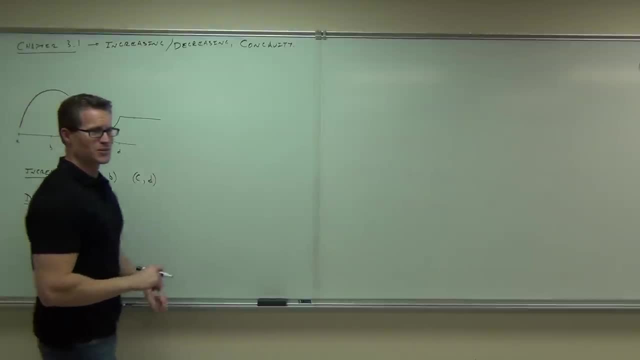 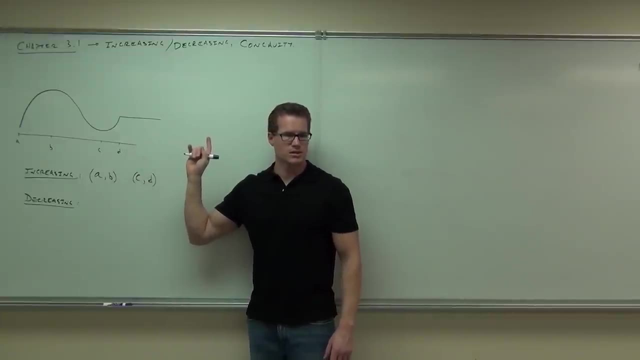 Growing up. This function's getting so old, so fast. How about from D onward? What's happening there? Is it increasing? No, Is it decreasing? Constant, Okay, constant, very good. Any areas intervals that are decreasing B to C. 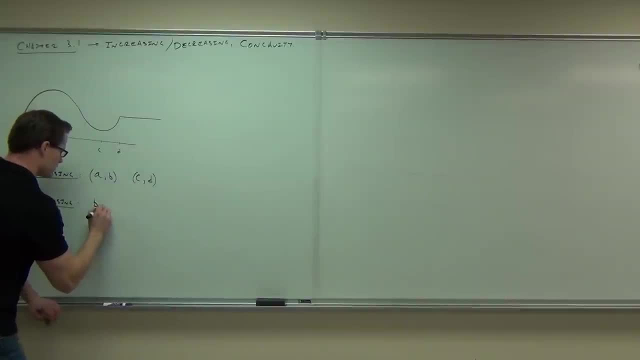 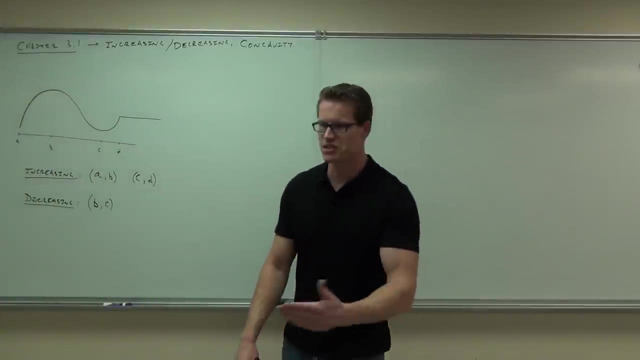 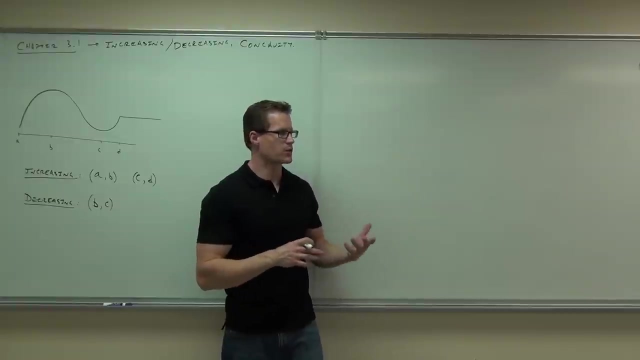 For sure. B to C, D onward's- pretty boring, D onward's- just a constant. The slope is zero. It's gonna stay zero forever. What I do want to talk about are the slopes of the increasing and the decreasing intervals. What's happening to that function on those intervals? 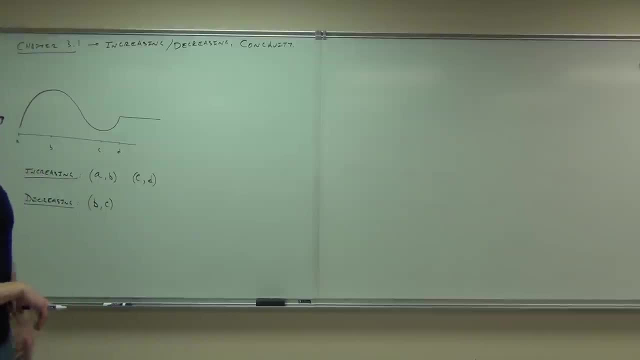 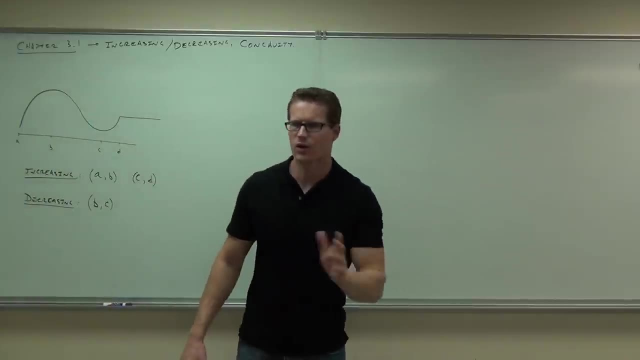 Let's look at A to B. What would you say, would the slope be for this point? And I don't mean like, oh, this is about three over one or five over one, I don't care about that. What I really care about is whether 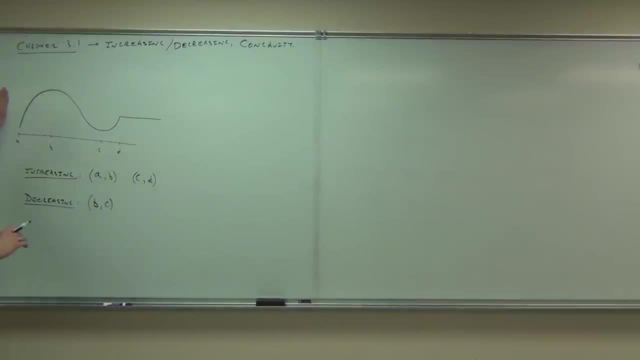 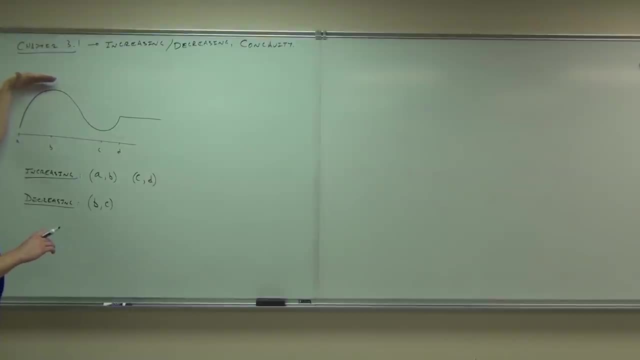 How about here? Positive, positive, positive. Hey, how about at B Zero? That's why B's not included, right? So from A all the way to B, would you say that we have a positive slope? Do you understand that when I have a positive slope? 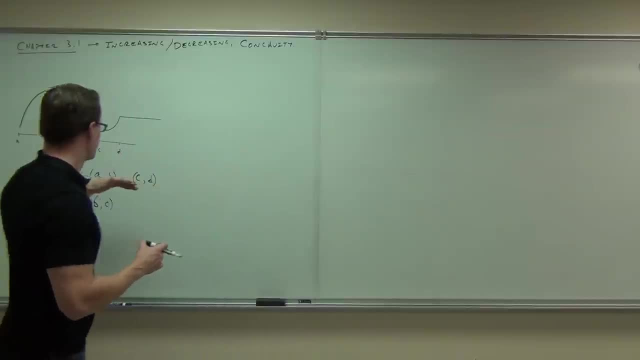 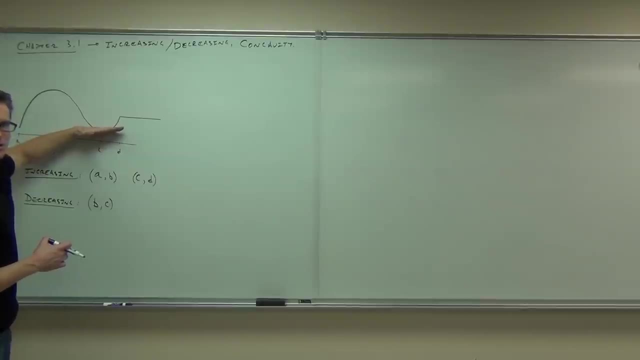 that means that my function is actually climbing. Do you see that? Look again from C to D. Let's look at C, At C, at C zero, But just past C is that positive, still Positive, positive, positive. 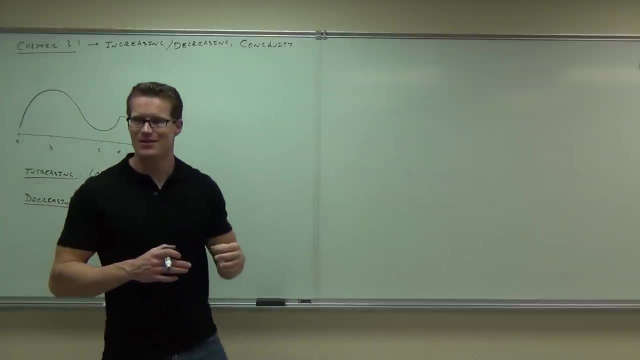 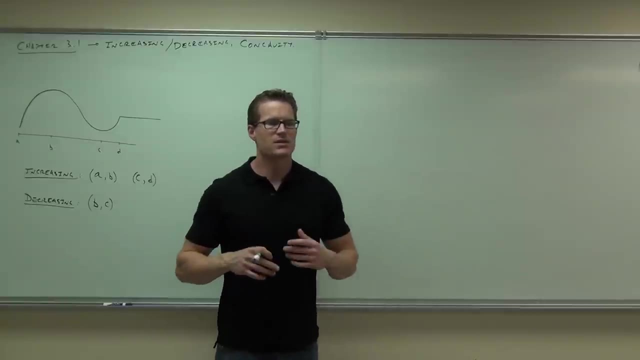 It's still positive all the way up until the point D. You follow me on this. When we say we're increasing what that means for us as far as a derivative and the relationships that we're building in this class, that means that your slope is positive. 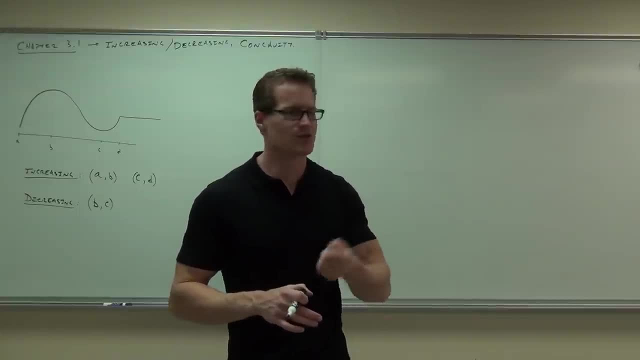 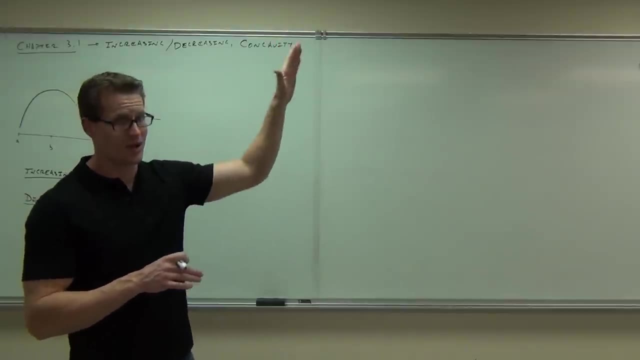 So increasing will happen if your slope is positive. There's no way you can draw a positive slope and not be going upwards. Are you with me on that? If you draw a positive slope, you're going upwards, true, Even if it's just at that moment. 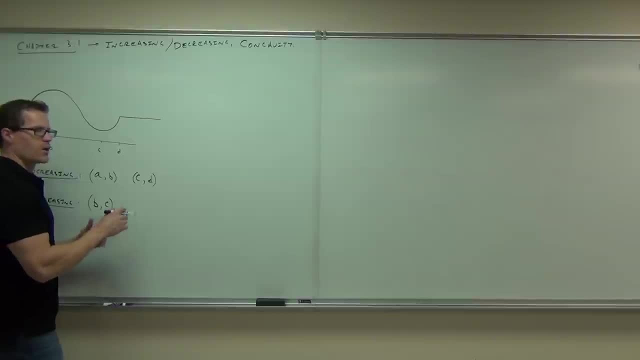 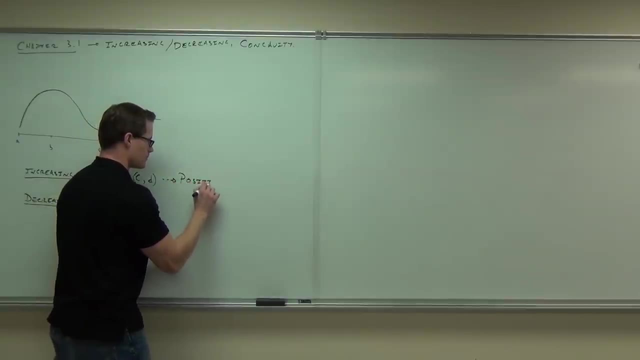 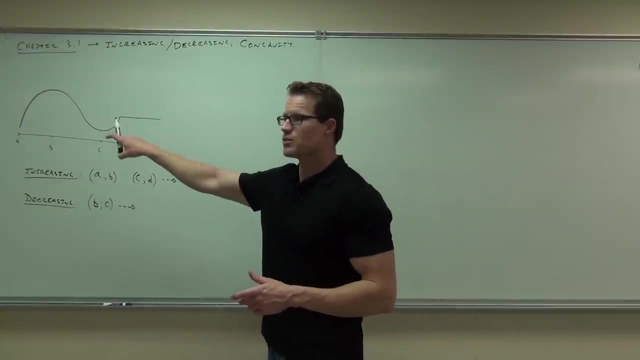 you're going upwards for that moment. So increasing intervals will have a positive slope. That should imply something. It should imply that a decreasing interval will have a negative slope. Let's look at our decreasing interval. There's only one of them. Is a slope negative for our entire decreasing interval? 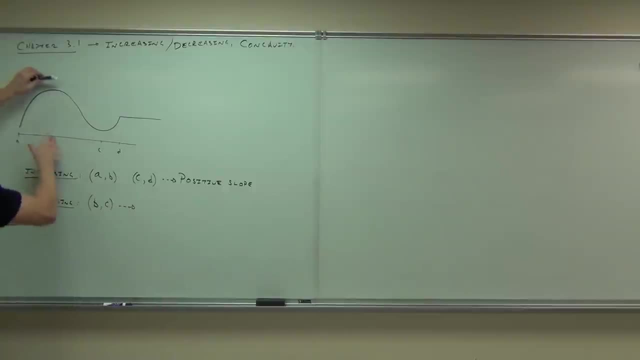 Let's check it out. Use your hand or your pencil if you want to. Here's our decreasing interval. Here it's at zero, right at B, But as we go past that is that negative, Negative. Even when you get down to here, it is still negative. 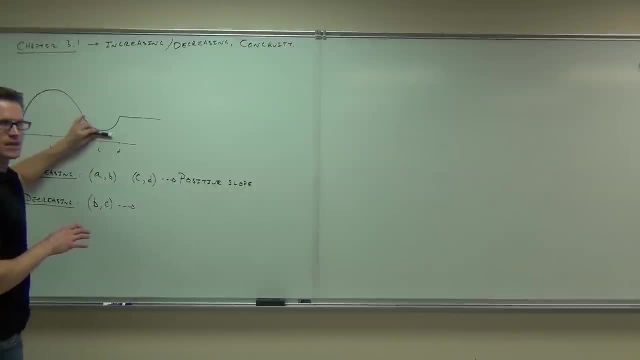 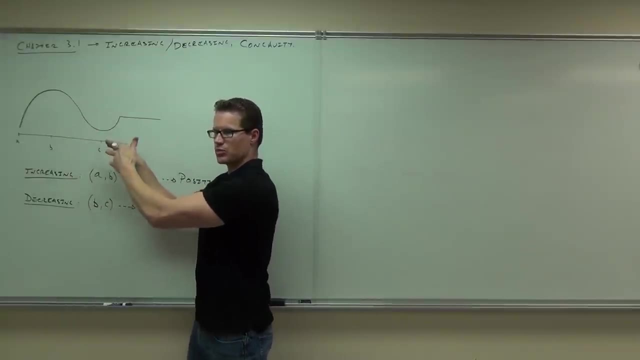 but then it's becoming still negative, but less negative until we get down to that point. At this point, look what happens. What's gonna happen when we change from decreasing to increasing. What happens to our slope As we change from decreasing to increasing? 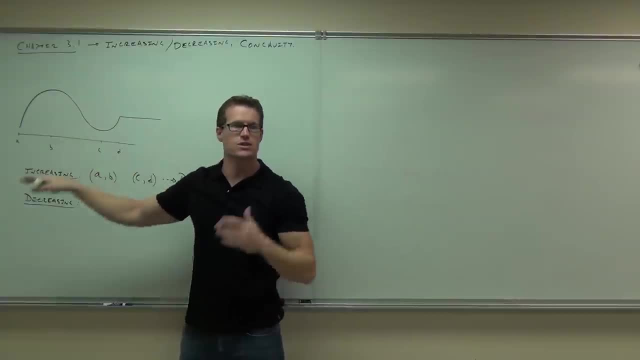 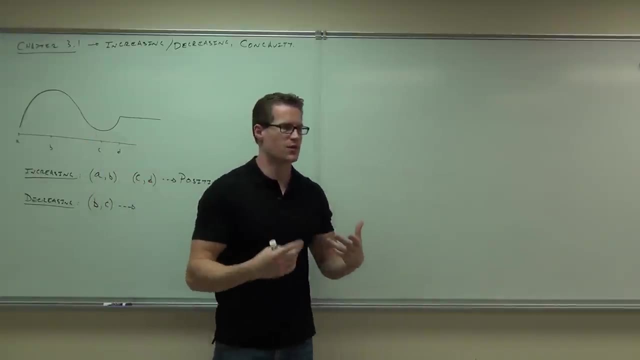 our slope goes from Negative to zero, Negative to zero to positive. Does that make sense to you? From increasing to decreasing, we go from positive to negative, And we're gonna incorporate all this stuff into our graphing of functions in just a little while. 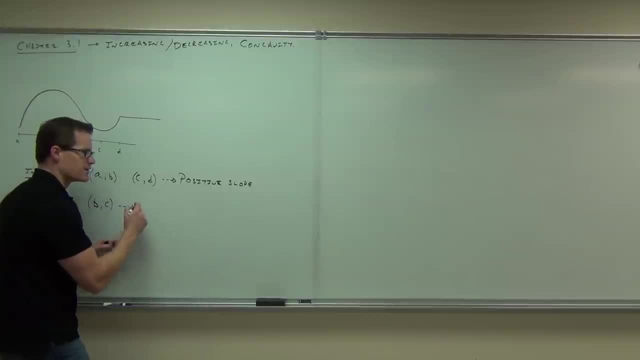 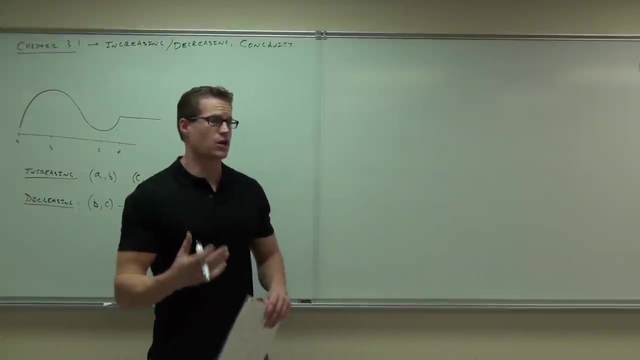 So right here, we need to know that a decreasing interval will have a slope which is negative, Definitely negative slope. I'm going to write out what I just talked about, So this is nothing else than what I've just described. This implies a couple things. 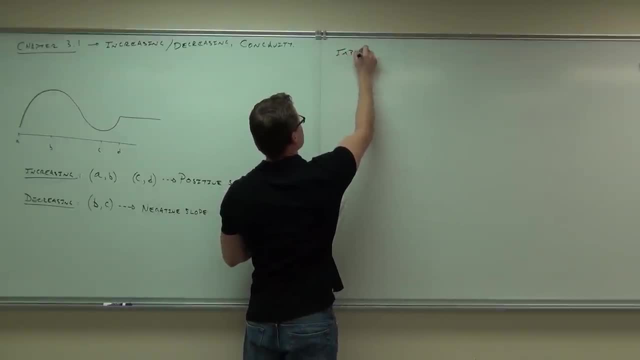 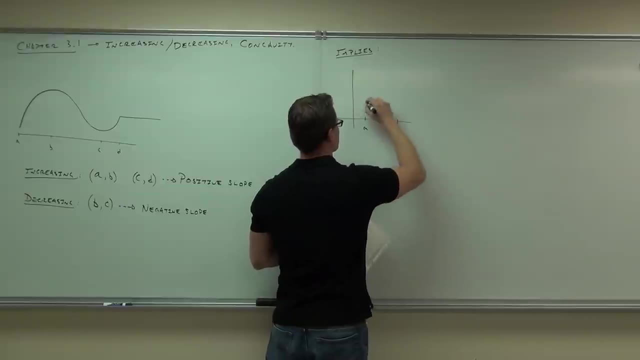 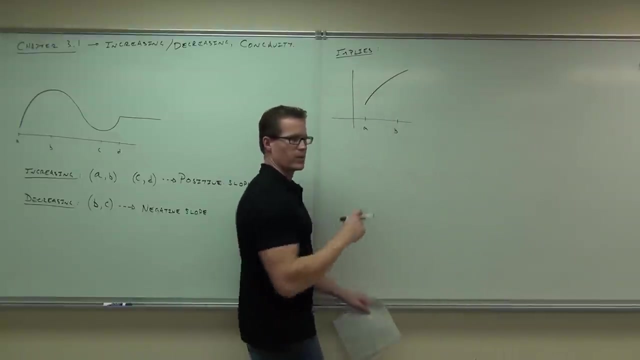 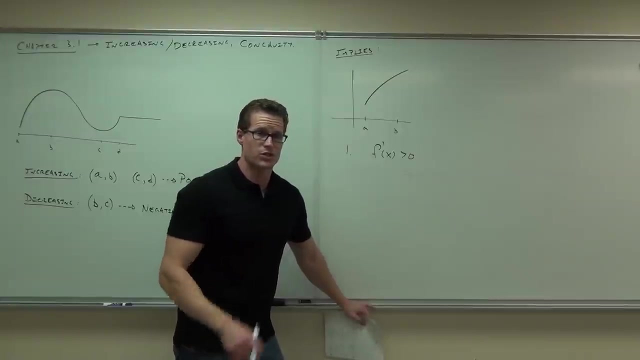 It implies? It implies that if our wait, we'll slope again. How do we find slope in calculus? What gives us a slope Derivative If our derivative is greater than zero? If our derivative is greater than zero, that means our slope is positive. 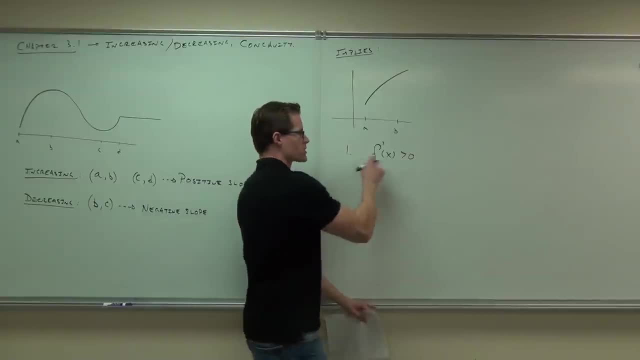 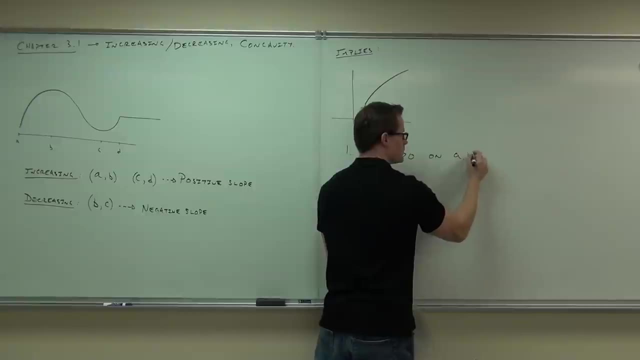 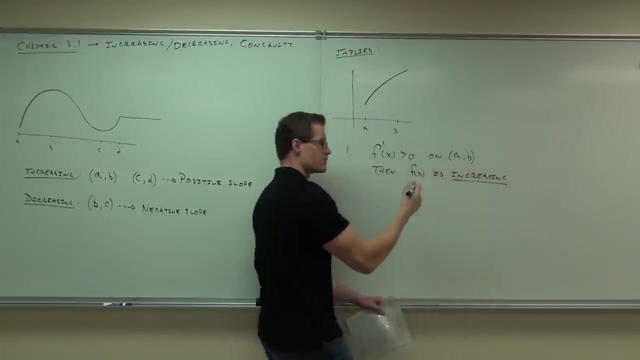 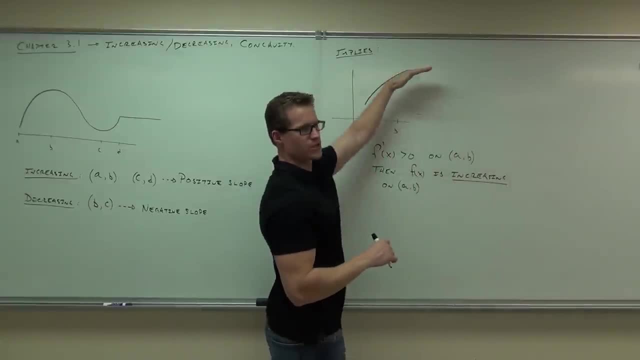 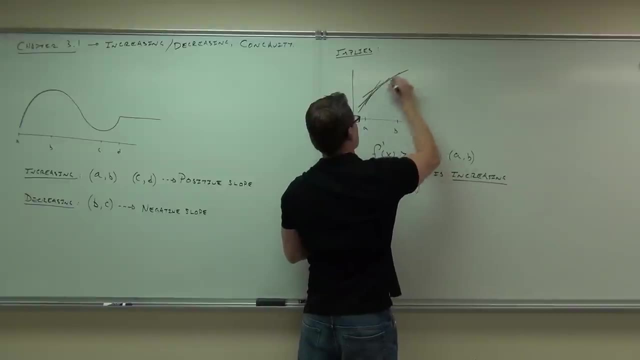 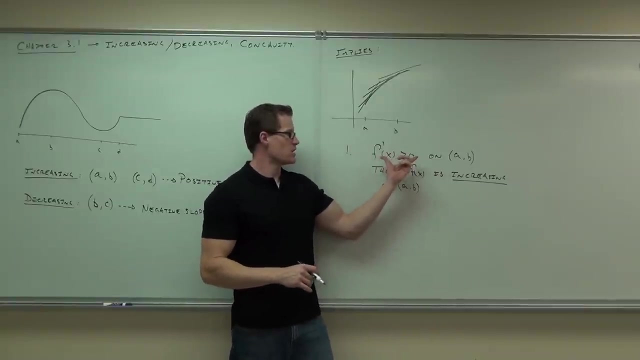 On that interval. You can see from our examples This is definitely increasing, right? Our slope is positive at every single point, From a to b. Positive Every one of those slopes, at every single point is gonna be positive. That's all this says. 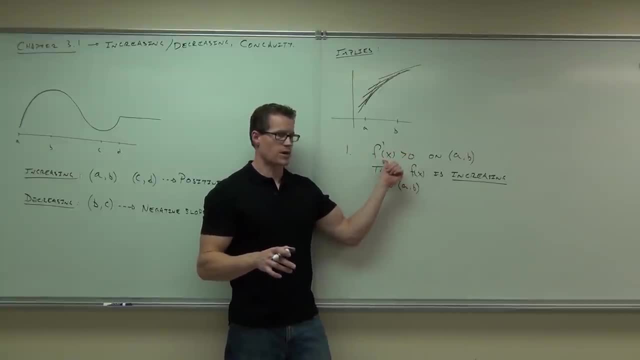 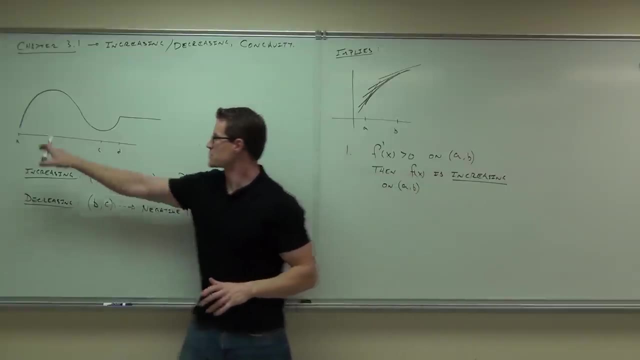 This says in English Here. it is in English for you: If the slope, this slope, right. If the slope's positive, you're increasing. That's all it says. You guys understand that idea. If the slope's positive, you're increasing. 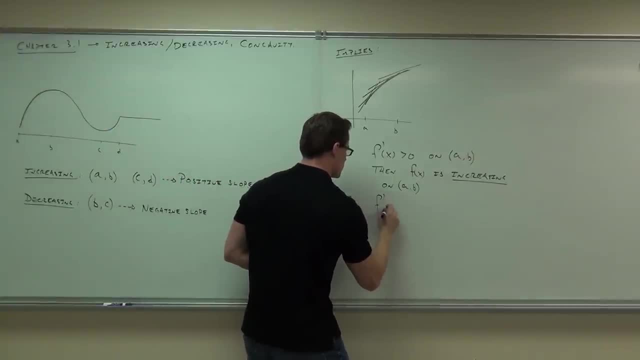 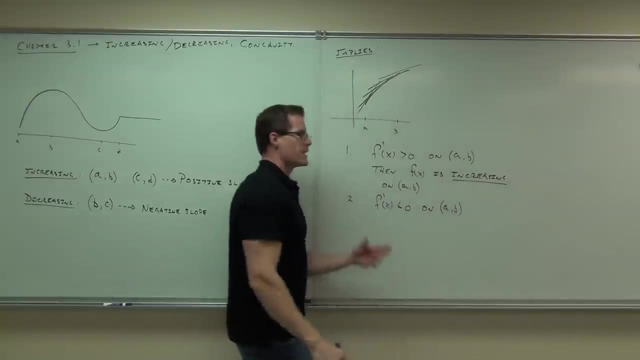 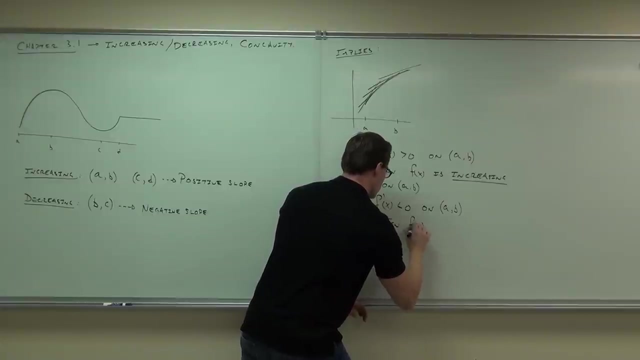 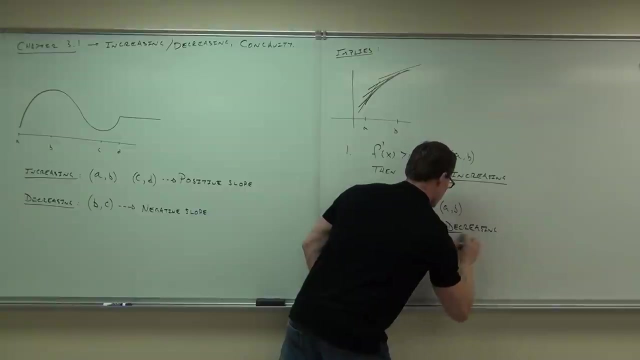 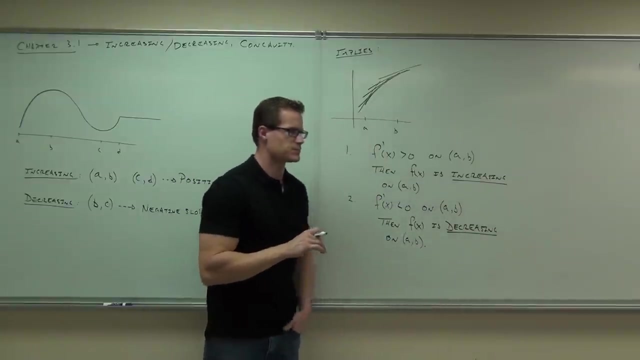 If the slope is negative, then f of x is decreasing on the interval. You still okay so far. In English again, what this says is: if your slope, remember first we have a slope. if your slope's negative, you're decreasing. 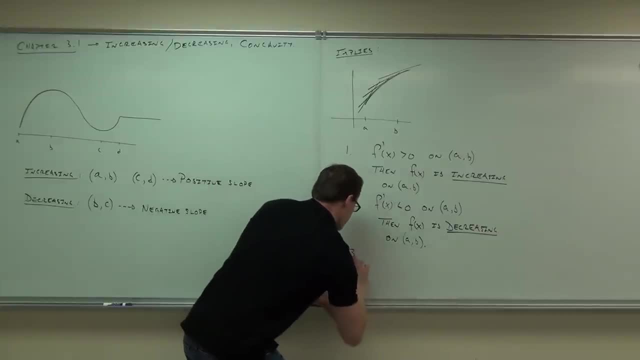 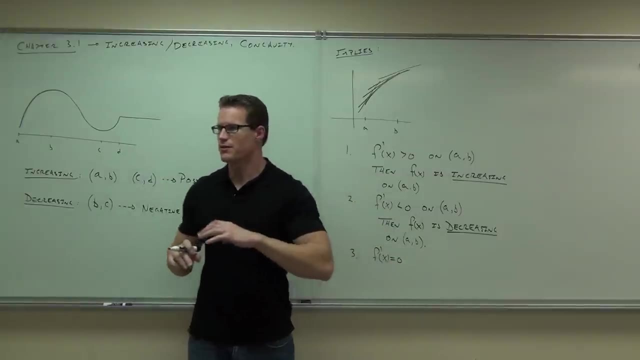 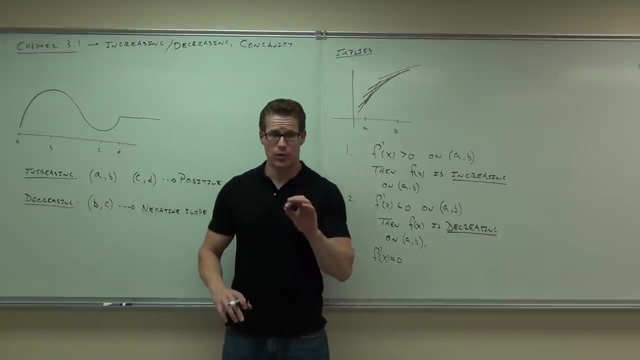 That's all it says. The last case is: if f prime of x, if your derivative equals zero, so your slope is zero. what that says is that, well, if your slope's zero, you're constant at that point or on the interval. 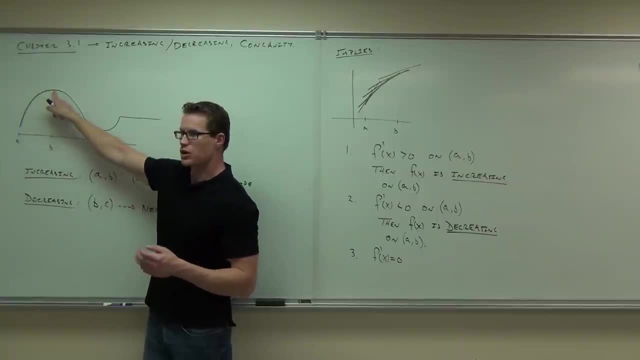 So, for instance, right here at b, our slope is zero. right, That means we have a, we're not increasing, we're not decreasing, we're constant. right there, That means a horizontal line. true, Constant means slope being constant. 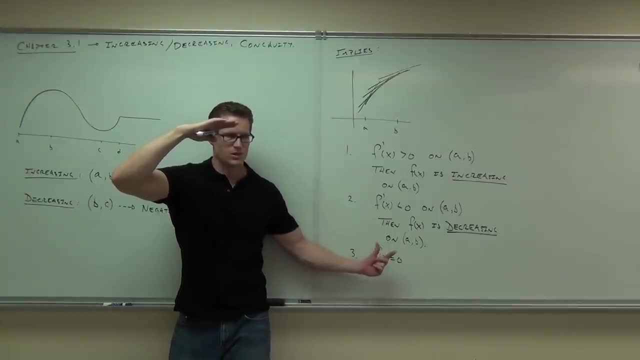 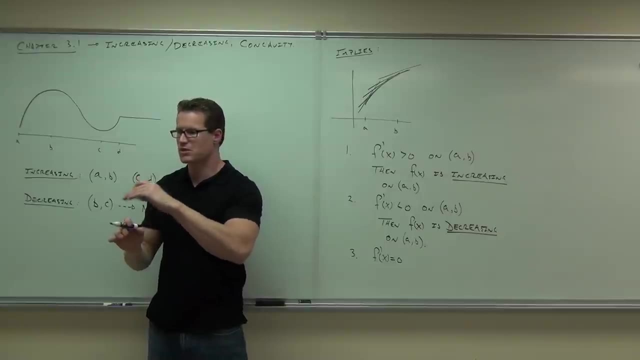 means a horizontal line. So if we have our f prime of x equals zero, we're talking about a constant line right there. That means for us a change typically. typically, that's a change from increasing to decreasing or from decreasing to increasing. 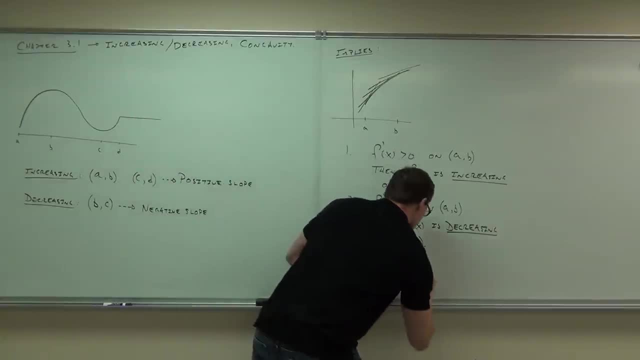 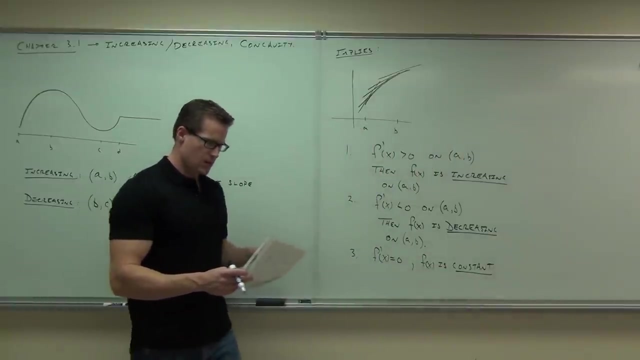 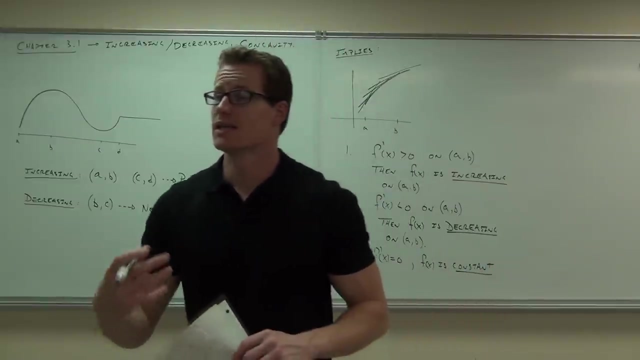 or that we're constant. that's what we're talking about. What's very cool is that we don't really have a graph to do this With just a function. if we know how to find the derivative, you can give me the intervals of increasing and decreasing. 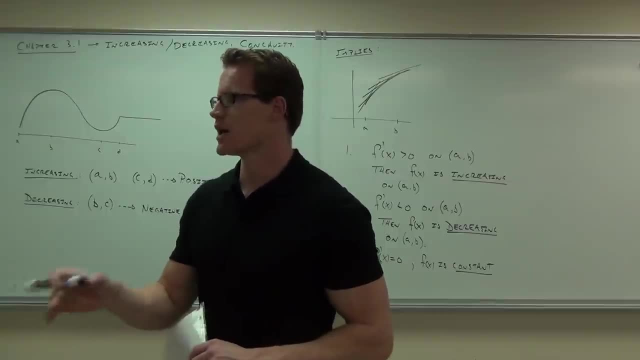 We're just gonna be having a set equals zero and do what's called the sine analysis. I'll teach you how to do that as we go on in the next sections. The last thing we need to talk about in increasing, decreasing and concavity is 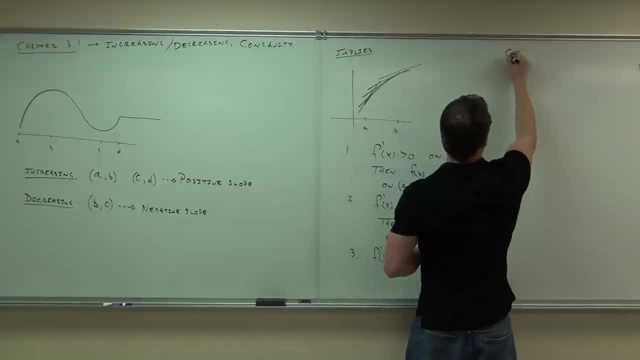 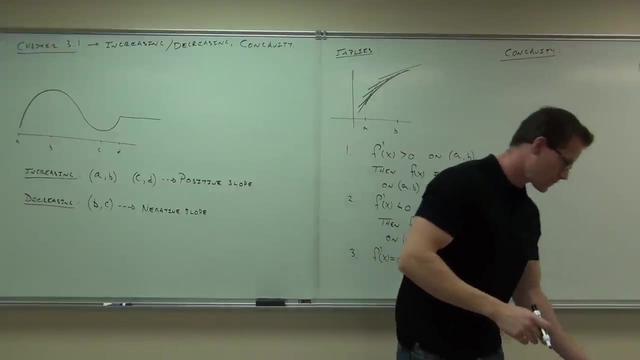 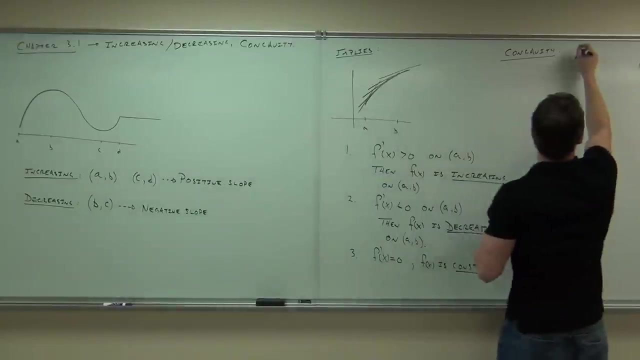 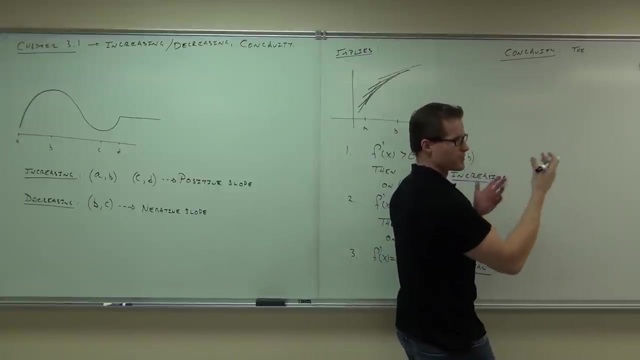 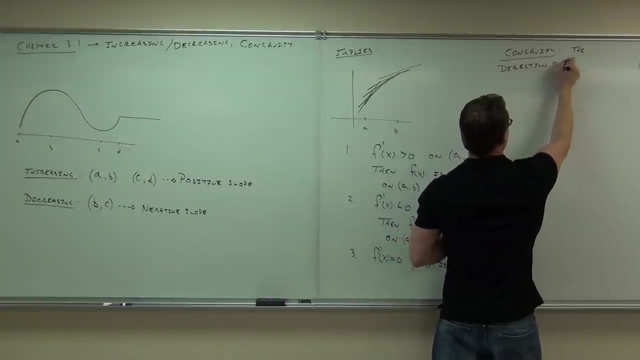 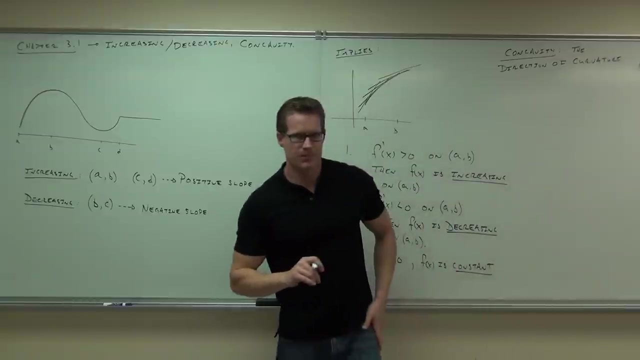 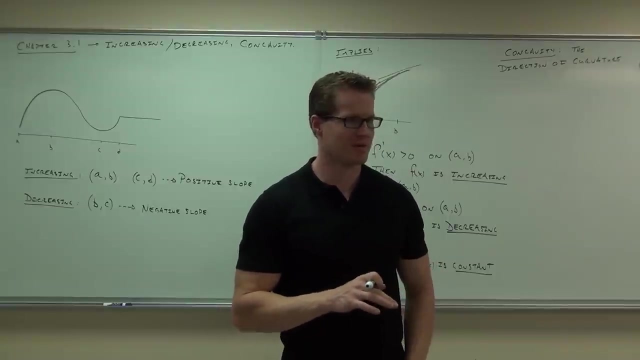 well, of course, concavity. Concavity is the direction of the curvature of your line, Or the description of the curvature. It might be a- I'll say- direction, Or basically it's how the slope is changing. Now I'm gonna try to match this up for you right now. 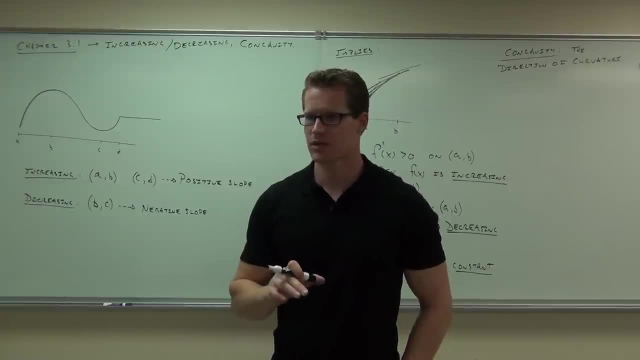 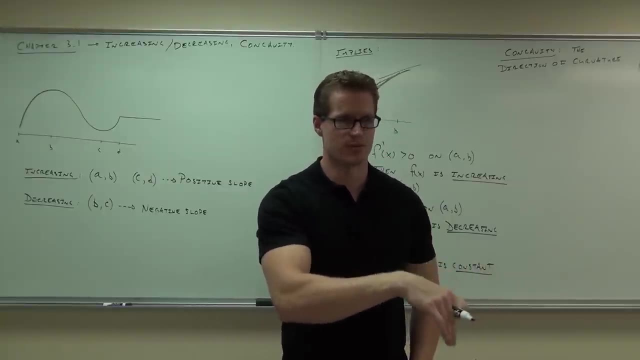 You know this first derivative means the slope. correct How the slope is changing. that's a rate of change of the slope should be a. what type of derivative? Second derivative: First derivative gives you slope. Second derivative gives you how the slope is changing. 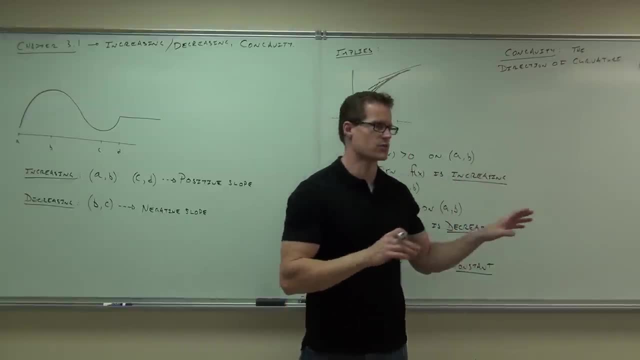 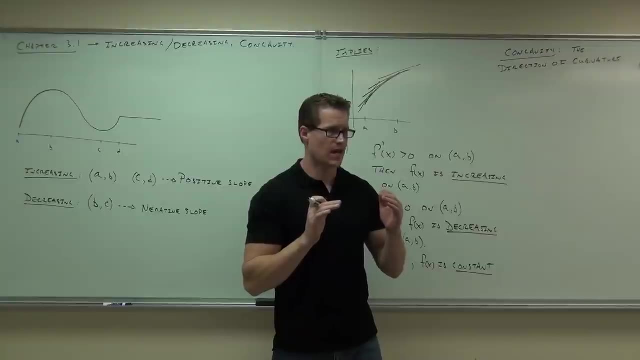 a rate of change of the slope. And so when we're talking about concavity, you're gonna find out in just a second. concavity has to do with the second derivative. First derivative gives you increasing and decreasing Concavity gives you the way that you are curved. 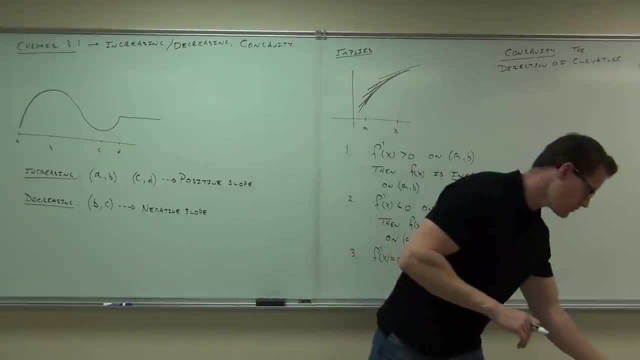 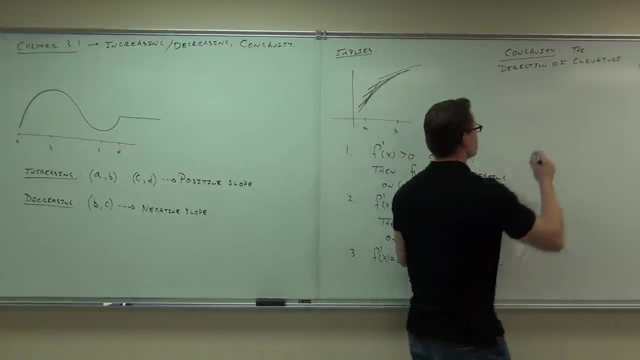 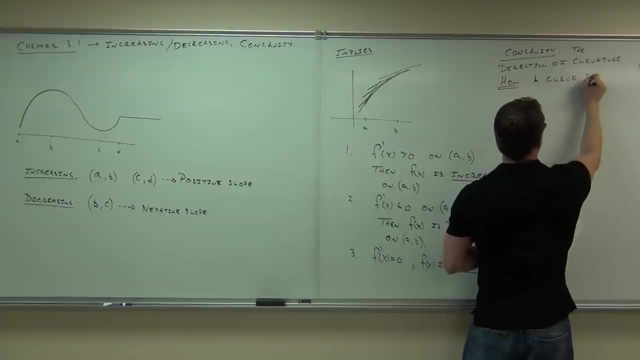 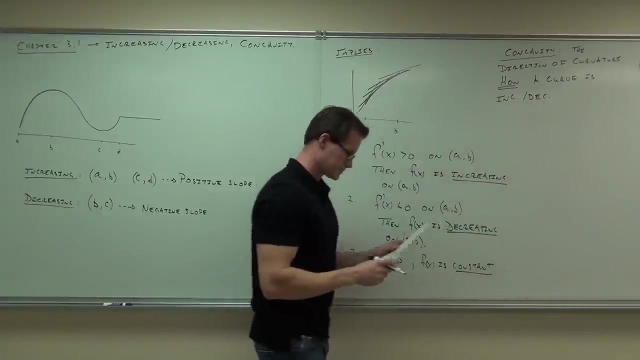 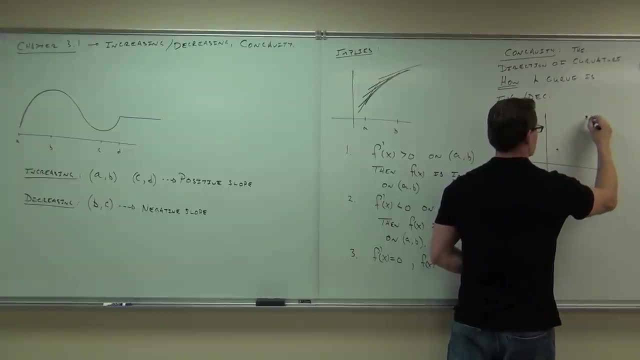 the direction of curvature. That's the second derivative. So basically it's how a curve is increasing and decreasing. Let me give you an example about why this might kind of be important for you. Would you agree that, to get from this point to this point? 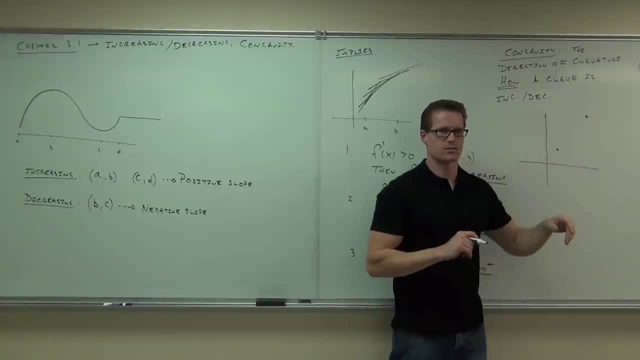 and be continuous, that you are gonna be increasing on this, And let's just pretend that we're not gonna go up and down. Let's go from here to here and not go back down again. So we'll definitely, overall, be increasing. 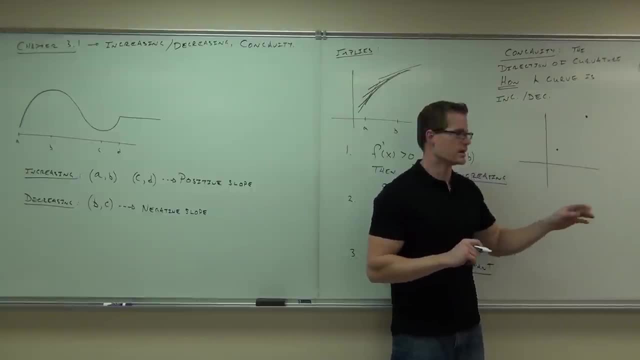 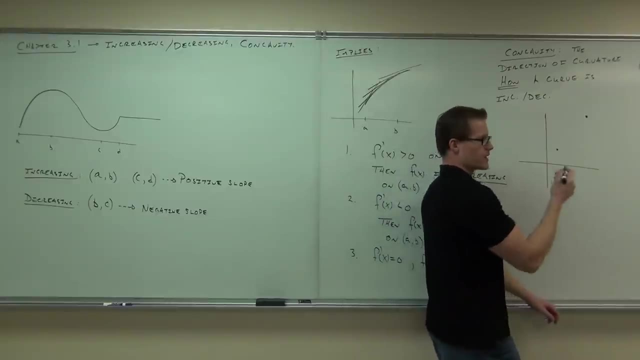 from here to here. right, Is there more than one way to get from here to here? Well, and still be increasing? Sure, You can probably think of it. I mean, I'm gonna be kind of simplistic about this. You could be straight, right. 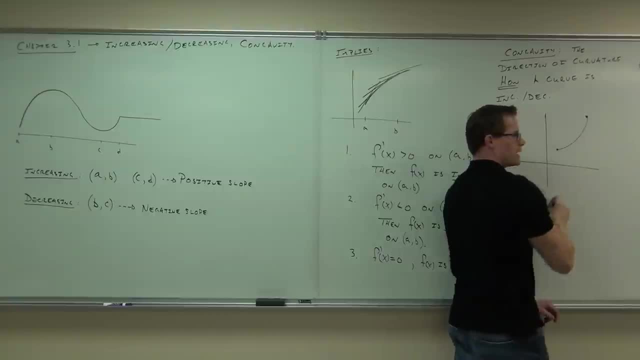 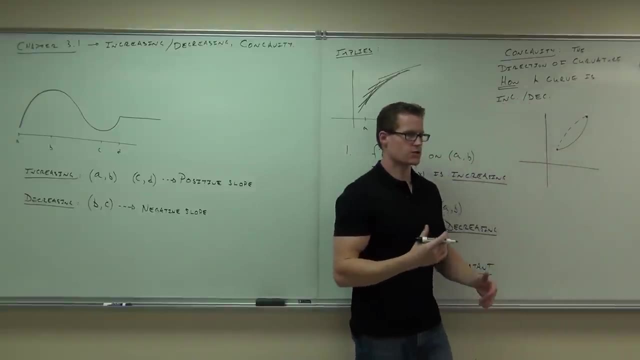 But that's not fun. You could do that, couldn't you? But you could also do that. Those have different curvatures. Here's one type of curvature. Here's another type of curvature. Here's one that's increasing at an increasing rate. 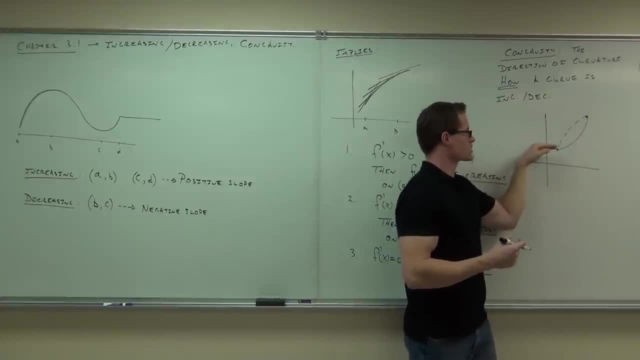 Here's another type of curvature. It's an increasing rate. Do you see what I'm talking about? It's starting to go up and it's going up faster, faster and faster. Here's one that's increasing at a decreasing rate. 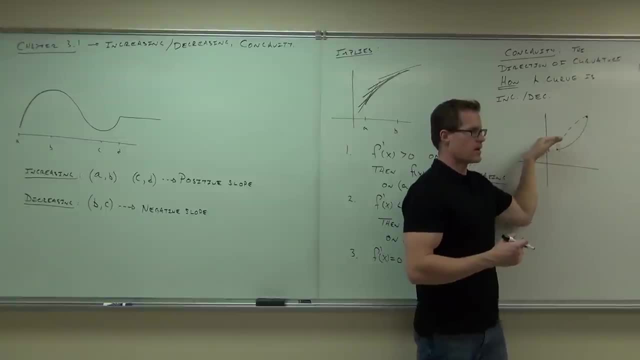 It's going up, but it's going up slower, slower, slower. and it finally gets there right, increasing at an increasing rate. The slope. look at the slope of this. Here's my slope right. My slope is positive for every point. 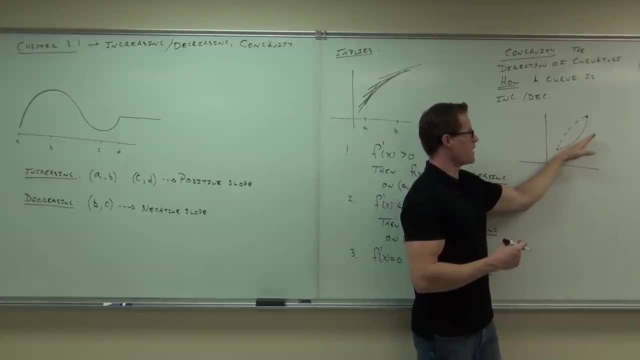 Do you understand? But my slope is positive here, but it's even higher and higher and higher and higher. My slope is actually increasing. Do you see what I'm saying? The slope is increasing Here- listen is increasing, but the slope is actually decreasing. The slope is going downward. What that does: 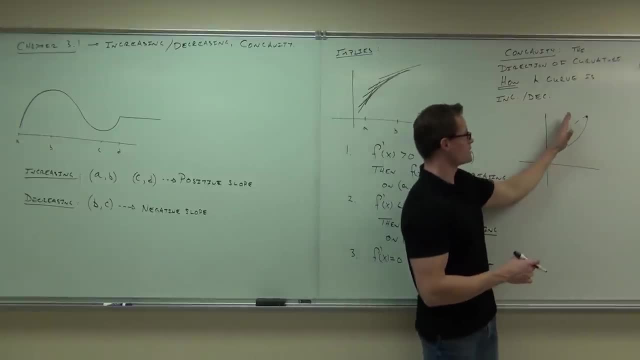 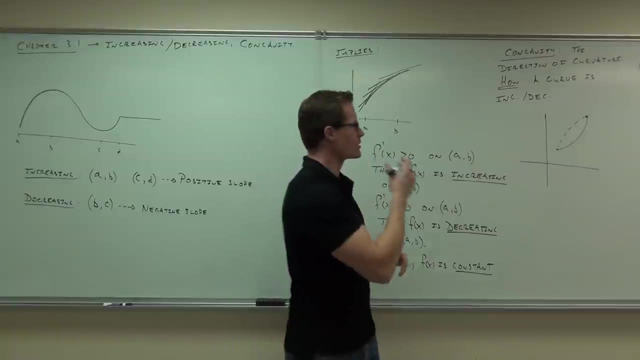 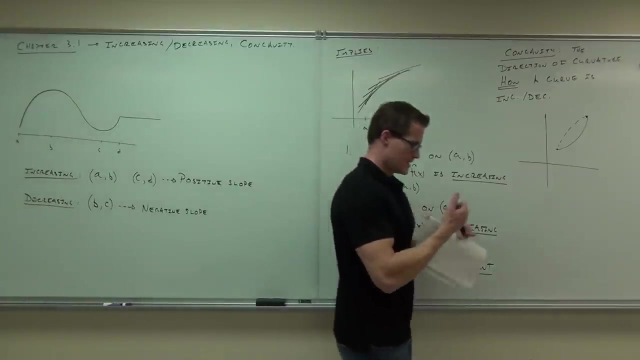 is gives us the curvature notice really positive, but the end not so much positive. What it does is gives us how our curve is shaped. That's basically it. So concavity is the curvature of our graph, And right now I really just need you to get to be familiar. 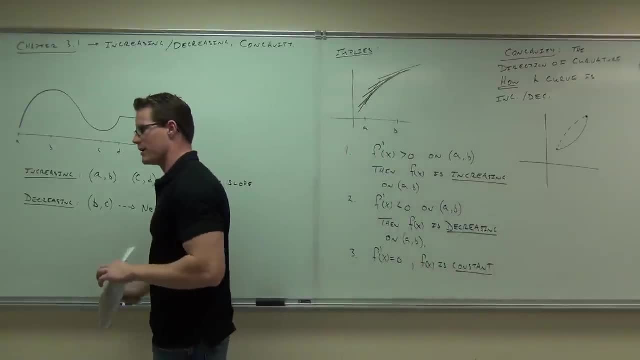 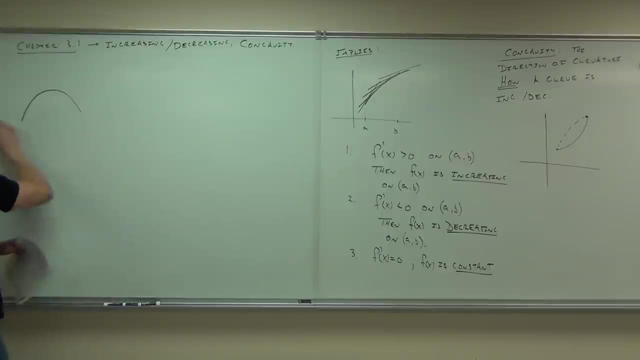 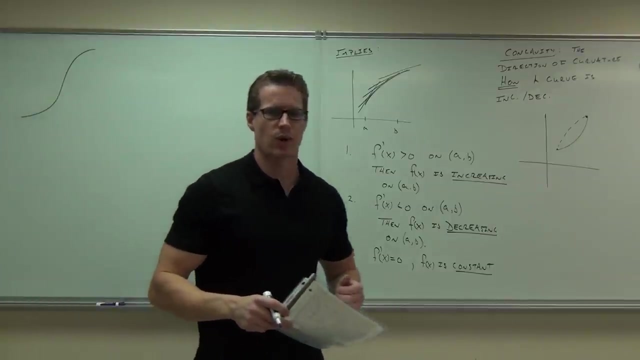 with concavity, what's concave up and what's concave down. So we'll talk about that for a little bit, Then hopefully get on to how to find these out. form just functions. This function is increasing everywhere, true or false? 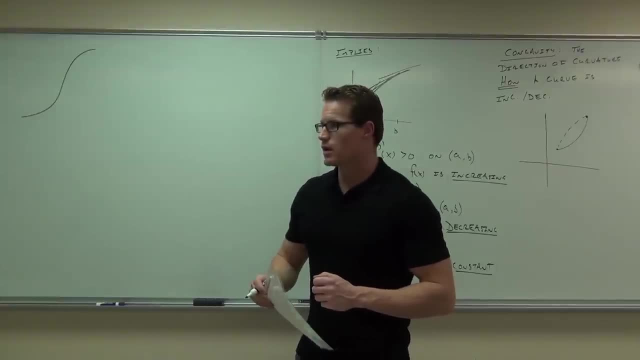 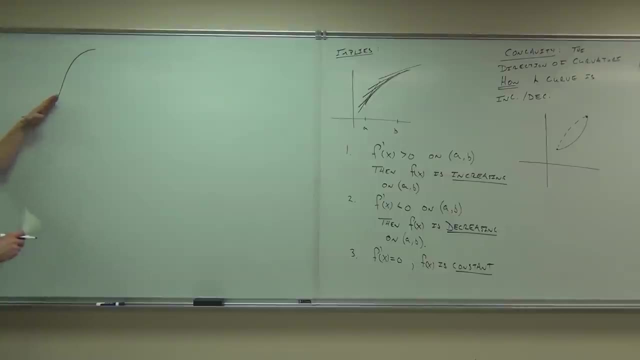 Clear, Definitely true. it's always going up. Is it going up at the same rate? No, In fact, you'll notice this. Yes, This is going up at an increasing rate. Oh wait, and then something happens, doesn't it? 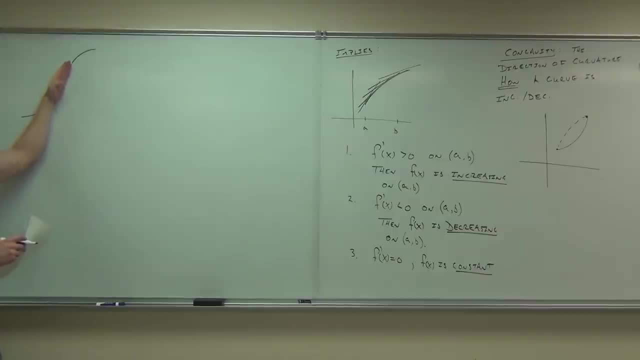 And then we're level. It looks like we're even for a while, And then we start increasing, but at a decreasing rate until we get to the top. See what I'm talking about. This is our two different types of concavity we have. 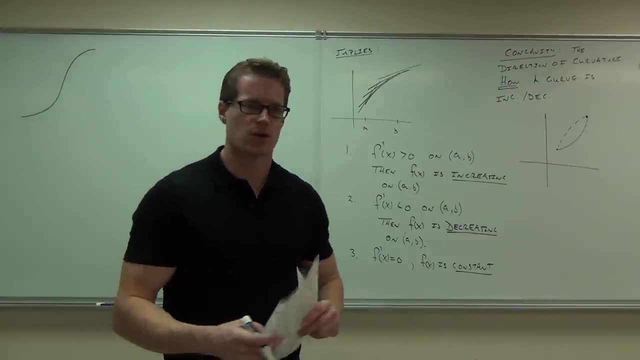 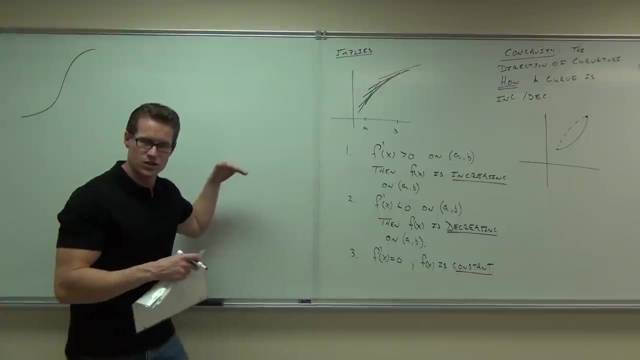 One region of this is going to be called concave up. If the curve is increasing at an increasing rate, that's this way. this is going to be concave up. Your slope is positive, Your slope is increasing. Actually, all we need is really: the slope is increasing. 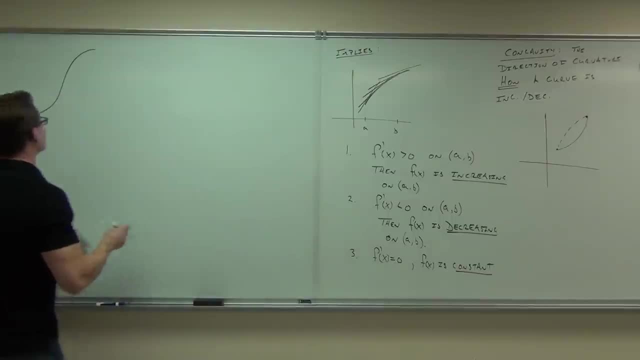 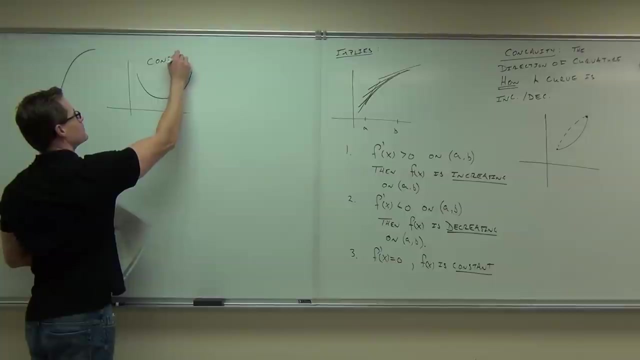 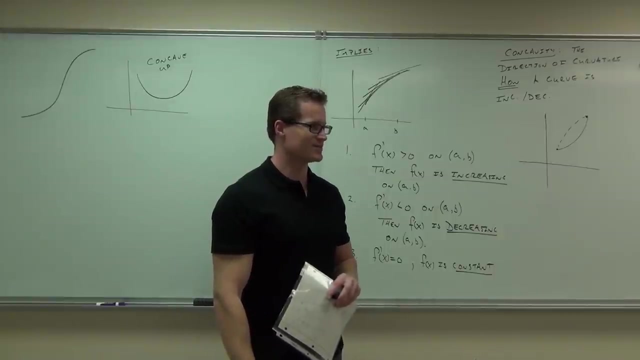 The slope is increasing. It's going to give you a concave up, Concave up, Concave up. You okay with that? Yeah, as in concave. Well, what I'm saying is: concave up doesn't have to be increasing. 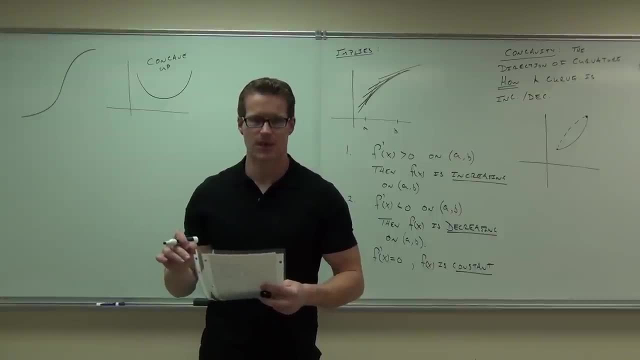 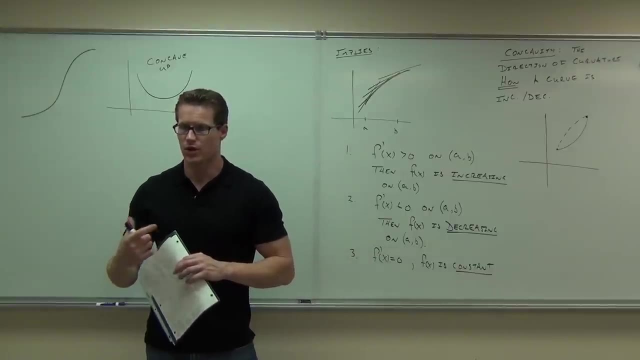 or decreasing as far as the function is concerned, but the slope must be increasing. I know this is going to be kind of weird for you to wrap your head around, but this is a completely concave up shape right here. Would it hold water? 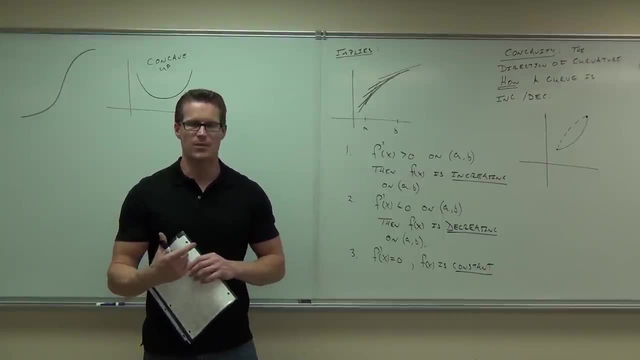 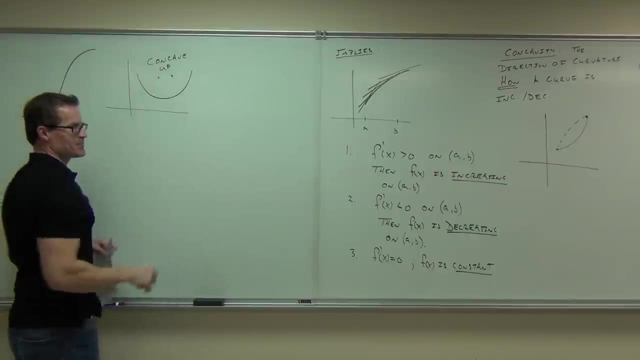 Yeah, Concave up will hold water. Also, how do you feel when you're happy, when you're up, when you're feeling up? I think you smile, You're feeling concave up, happy. Concave up is going to hold water. 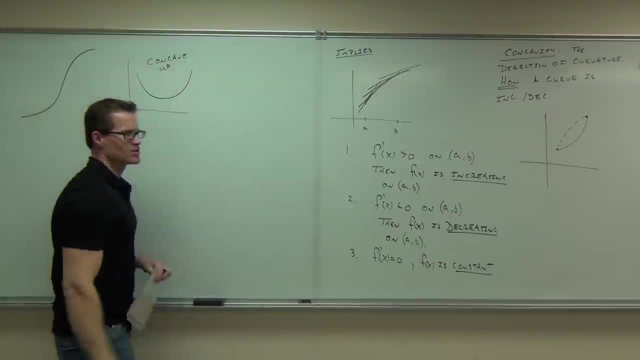 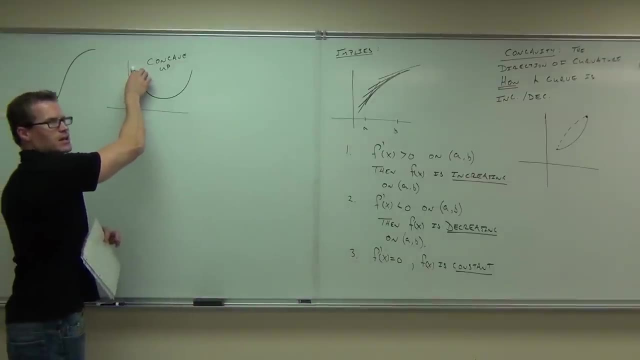 It's going to be upper facing. Now, if you're confused as to Mr Leonard, why did you say that the slope is increasing? The slope is increasing here. Watch What's the slope here. Very negative. What's the slope here? 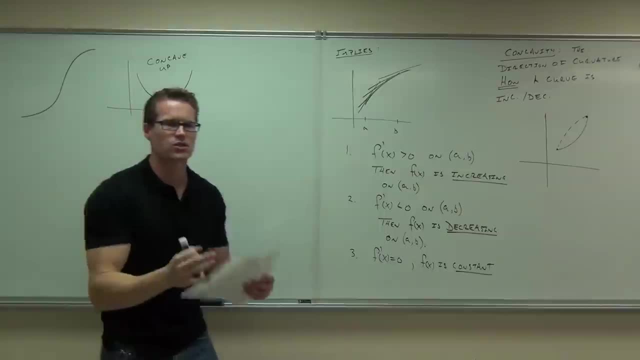 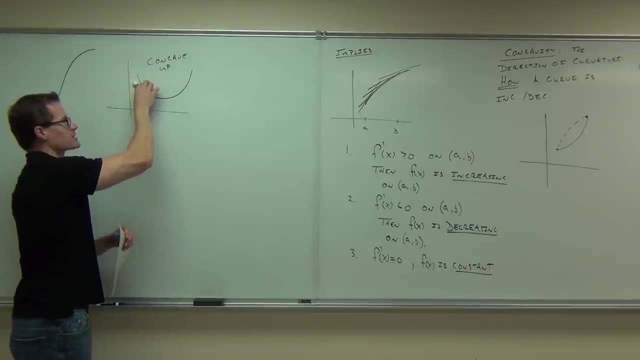 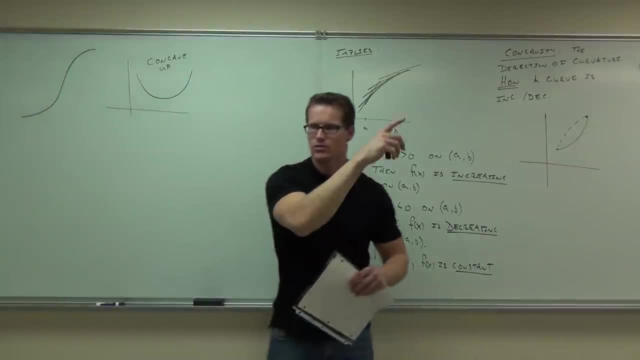 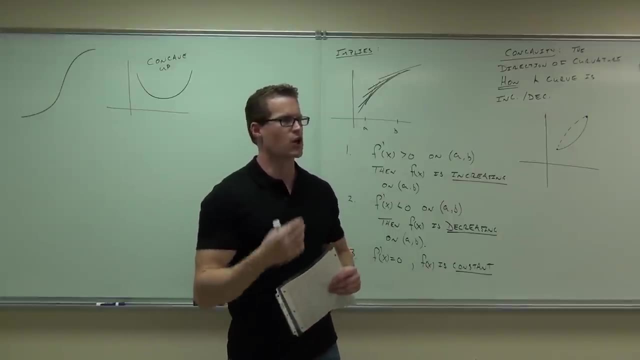 More positive, More positive. The slope is actually increasing The entire way through. Do you see the difference? It's difficult to think about because I haven't graphed the slope. I've graphed the function, But we're talking about the slope and how the slope is changing. for concavity. 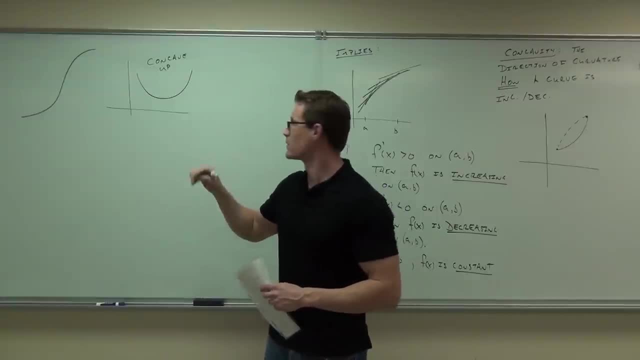 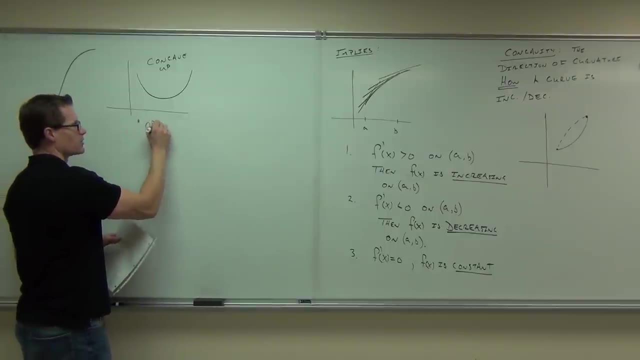 There's the distinction. So this is definitely concave up. That's concave up. What it says is: it opens upward. That's how people describe it. It opens upward Or it would hold water. That's probably the worst one. 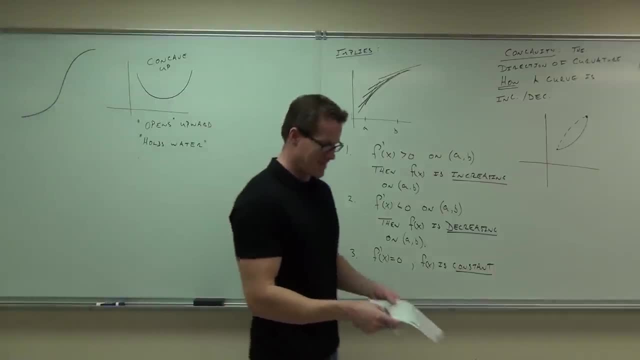 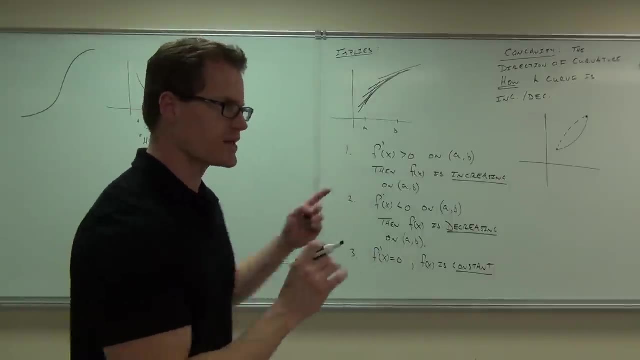 Here's what it actually means in mathematics: If you're concave up, it means your slope is increasing. The function is not necessarily increasing. We see that This is actually decreasing, But the slope is increasing. Do you see the distinction there between increasing and concavity? 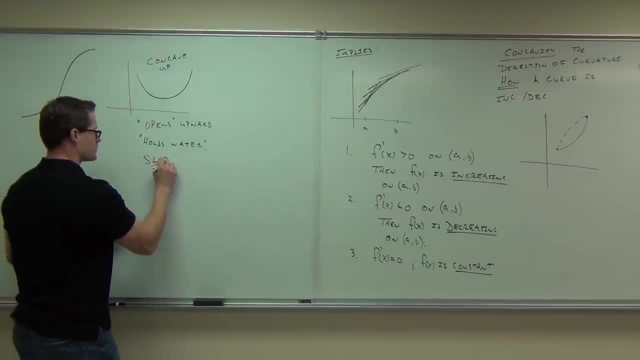 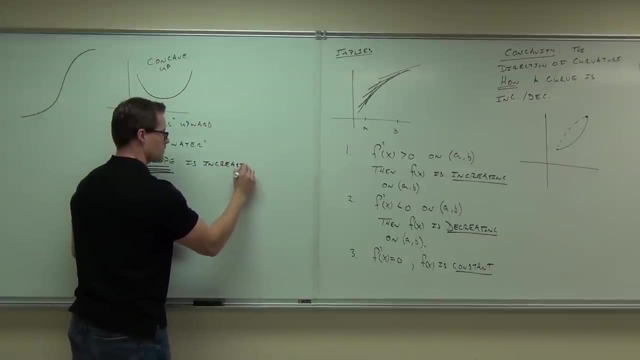 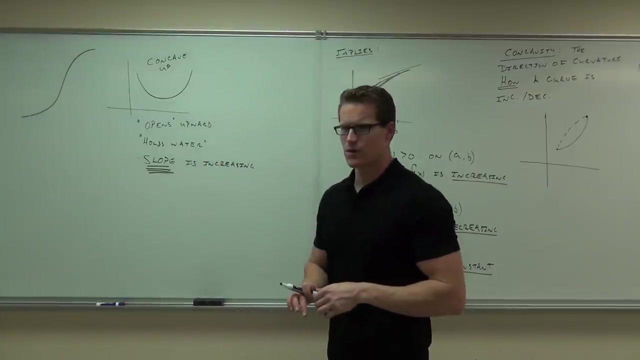 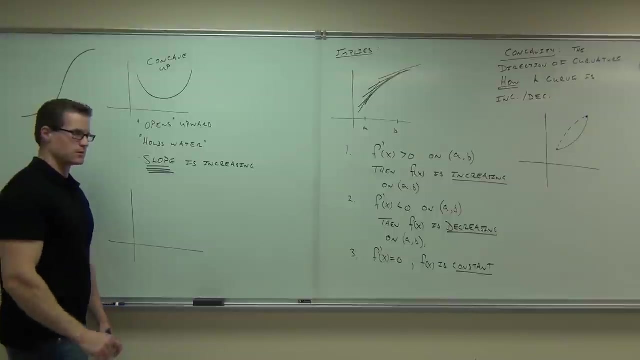 Less negative. The slope Is increasing on that interval. That's what concave up means You. okay with this. so far, Okay. What's concave down? look like Concave down Down, Concave down. Friday face, Friday face. 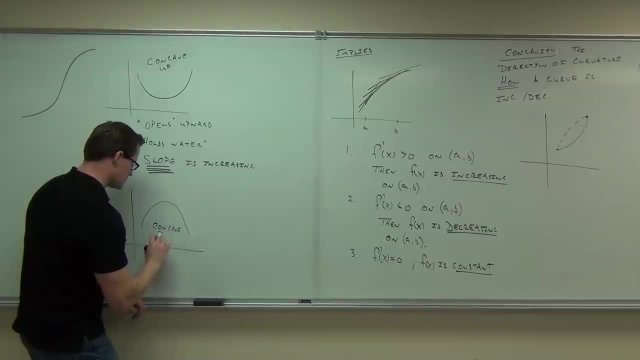 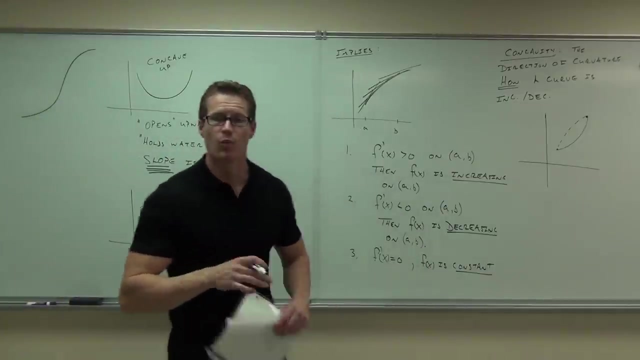 That's your umbrella. The water slides right off. it Opens downward and would not hold water. But really what it means is that your slope is decreasing. Your slope is the. whether your function is increasing or not doesn't matter for concavity. 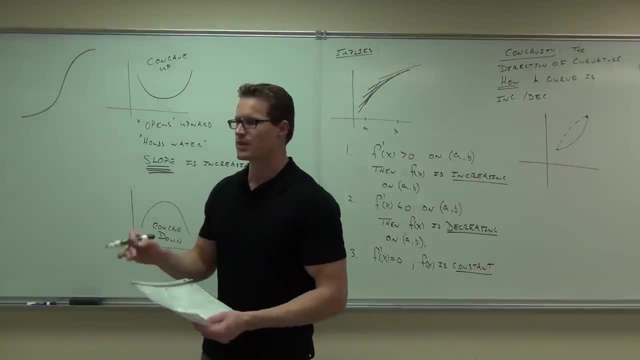 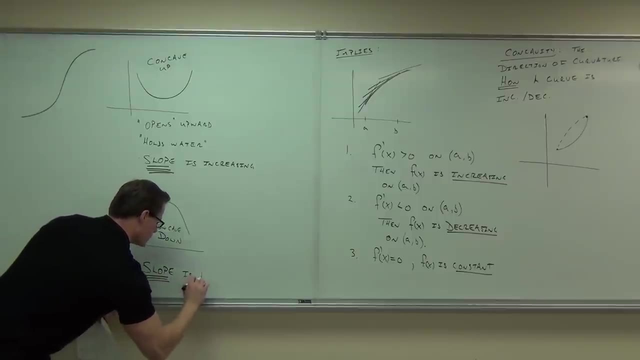 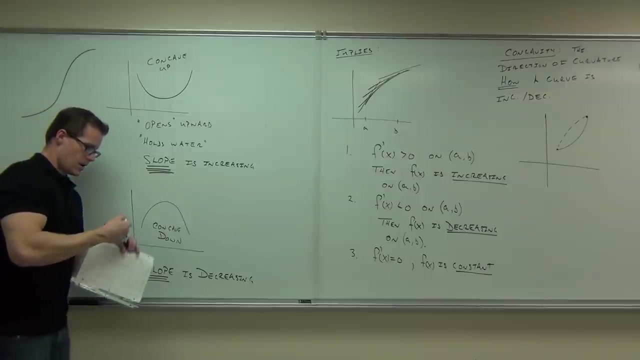 Concavity says: how is the slope changing? Slope changing for concave down means it's decreasing. Slope is decreasing. Okay, All right. Oh, and here, Notice, look at how's this curve go? Yes, the curve itself does this. 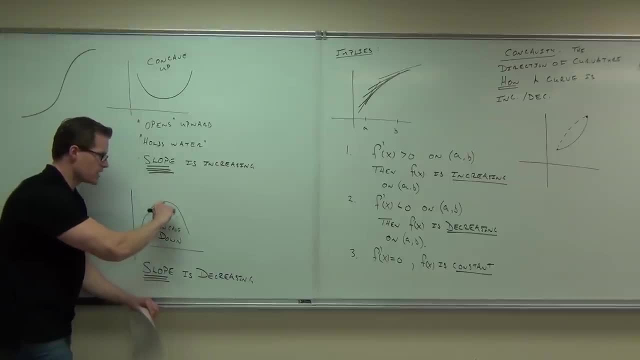 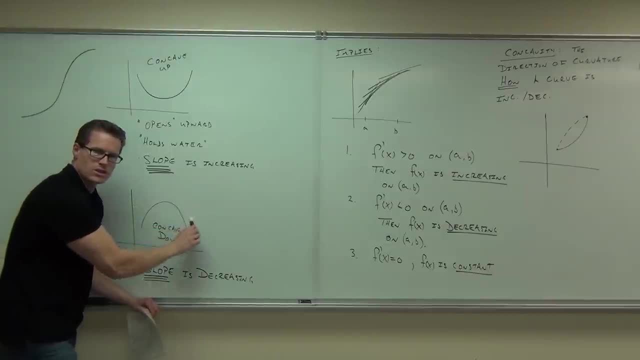 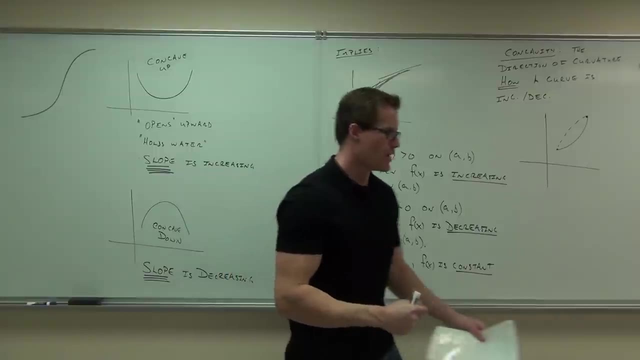 zero negative, more, more, more negative, more negative. It's always decreasing through the whole entire curve. You see what I'm talking about. There's a difference between increasing and decreasing as far as the slope is concerned. There's a difference between increasing and decreasing of a function. 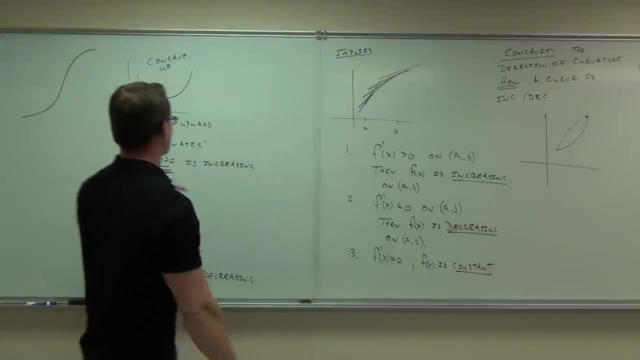 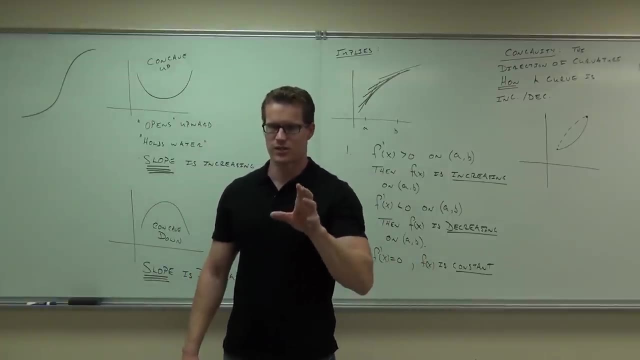 and the slope, how that changes on a function. Now here, can you tell me where my intervals are for increasing and where my intervals are for decreasing? Stop me when I for my slope. stop me when I change from concave up to concave down. 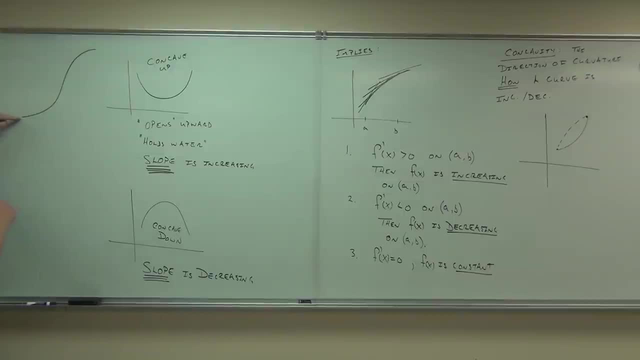 What do I start with from? let's start this way. What do I start with here? concave up or down? Concave up And Oh, you missed it. Let's try that again Ready? No, I'm just kidding. 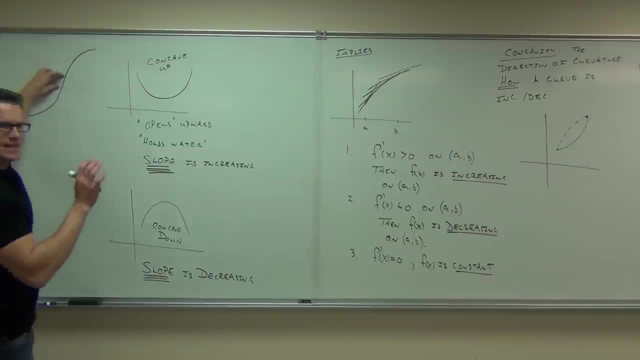 And Oh no, Yes, somewhere, somewhere in here Now, exactly where I don't know, because I don't know the function itself, But it's going to be somewhere right about, I would say there, Right about there we change. 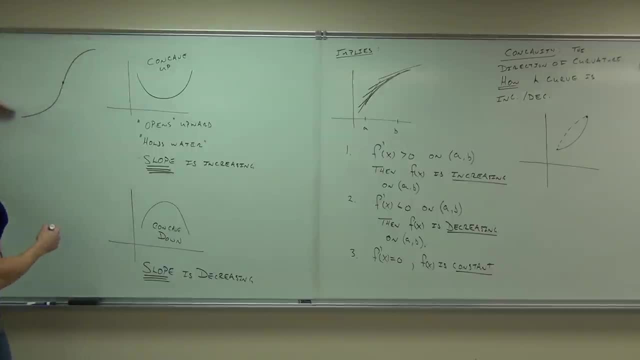 We change from holding water to being an umbrella, from being concave up to concave down From the slope, increasing, increasing, increasing, and the slope dies off, Decreases, decreases, decreases. Do you see what I'm talking about? 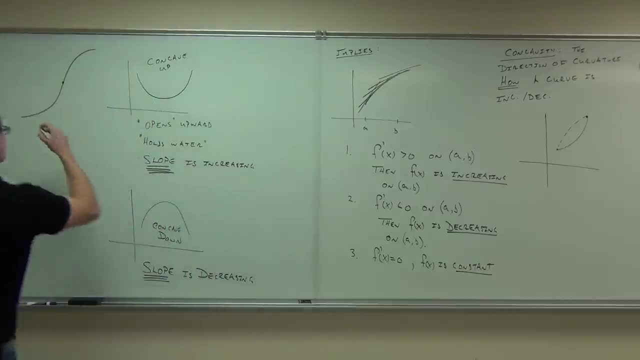 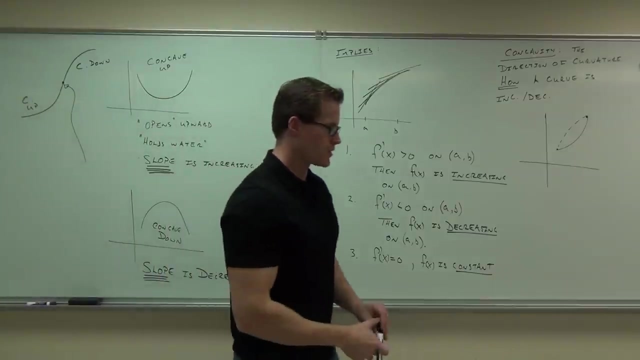 Yes, That's what I'm talking about there. That changes from concave up to concave down. This would be up, concave up, concave down. This point where you change concavity is called an inflection point. inflection point. 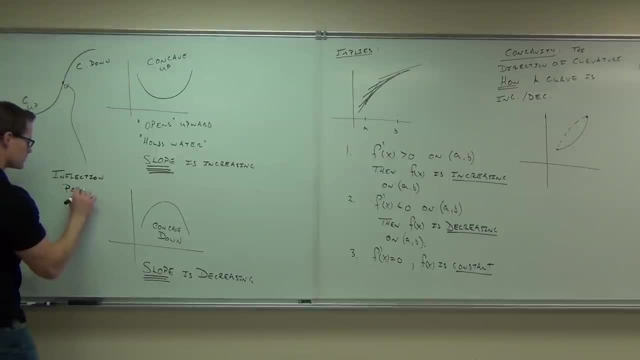 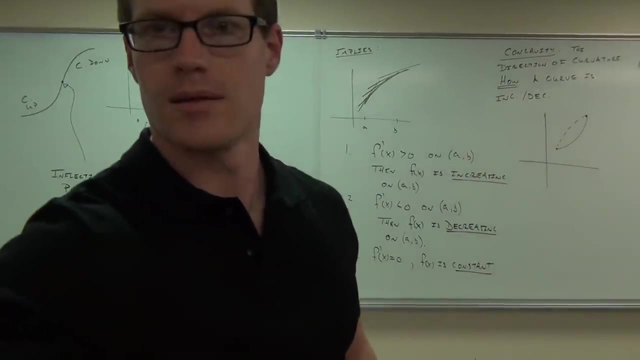 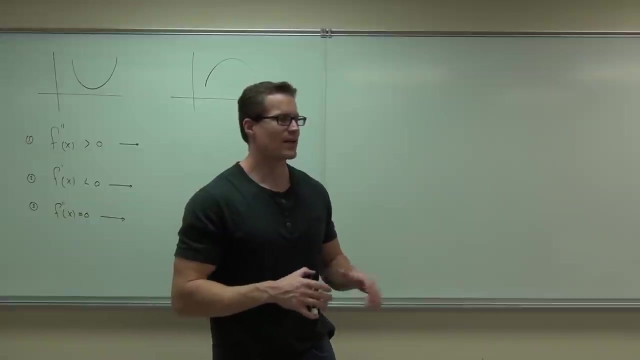 Or point of inflection. Okay, That's your inflection point. Well, we're going to continue talking about increasing, decreasing concavity and how that relates to our first and second derivatives. What we found out last time is that the first derivative is going to give you increasing 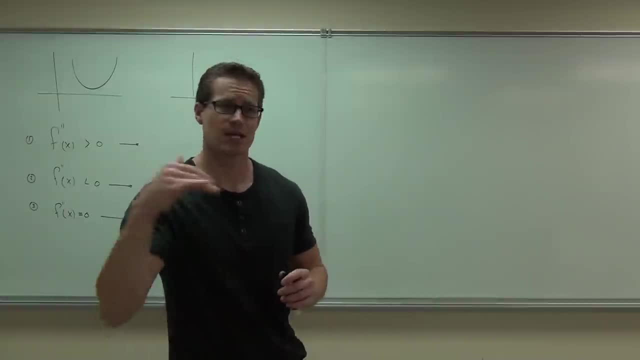 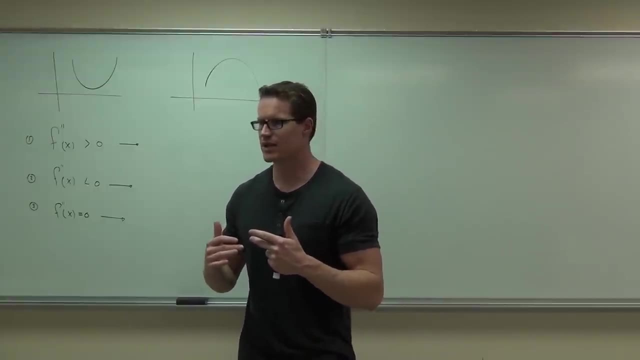 or decreasing, because if the slope is positive, you're increasing. If the slope is negative, you're decreasing. We also found about found out about the way the curve is shaped. so basically, how we're increasing or how we're decreasing is also important. 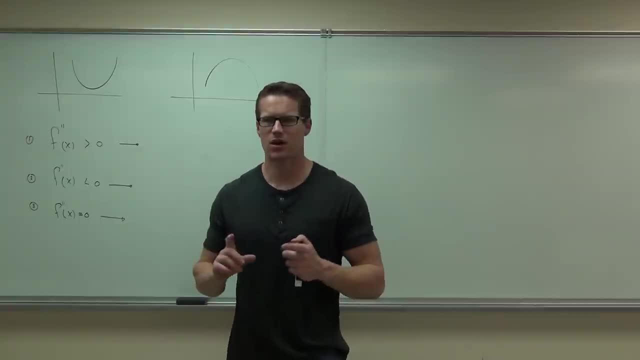 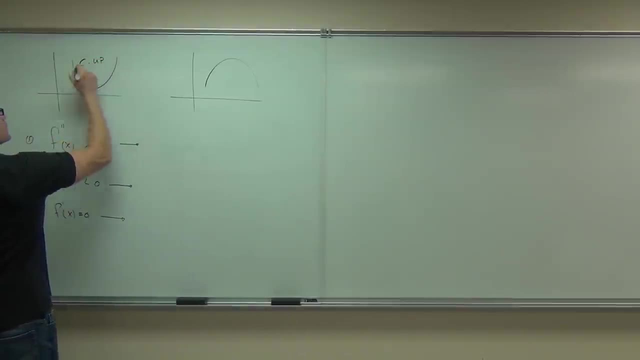 And what that was called was concavity. Can you tell me which one of these is concave up, the left or the right? The left? So this was the concave up and this was the concave down, and here's what we've determined. 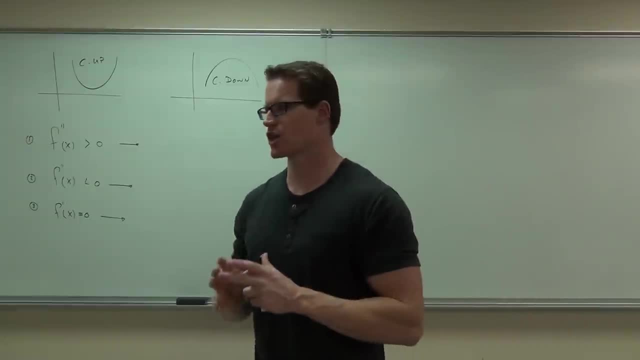 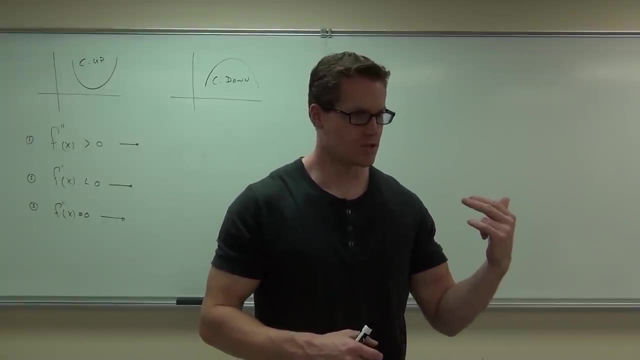 The second derivative, which is the way the slope is changing- if the slope is increasing or the slope is decreasing- will tell you whether we're increasing at an increased derivative or decreasing. Okay, Okay, Okay, And then we'll have a. you'll have an increase or decrease rate, or increase or decrease rate. 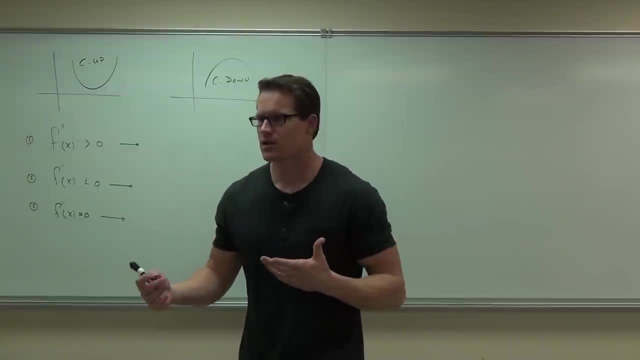 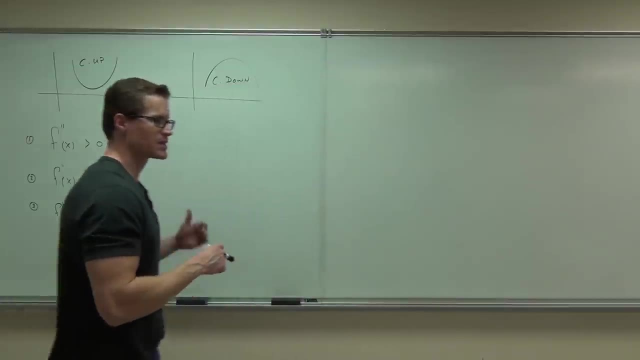 or increase or decrease rate. So basically how we're shaped. so here's what we said. There's a second derivative: is positive. What that means is the slope is increasing. If the slope is increasing, that means we're going to be concave up. 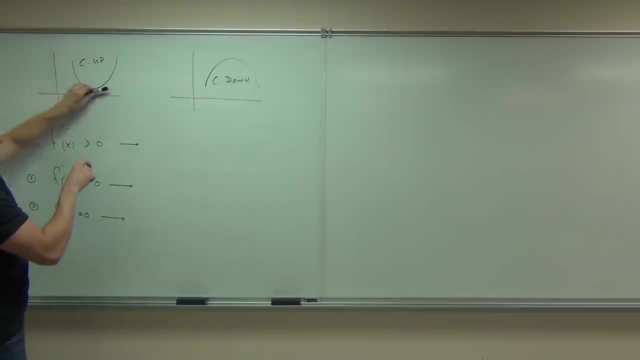 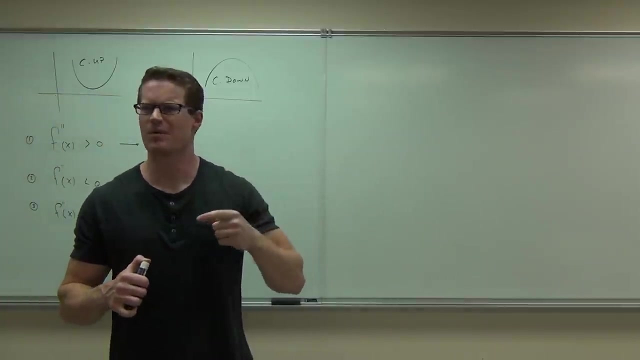 Notice what the slope is doing. The slope is increasing. Does that make sense? So if our second derivative is positive, the second derivative says the slope is increasing. Remember, the second derivative is the slope, is the rate of change of our slope. 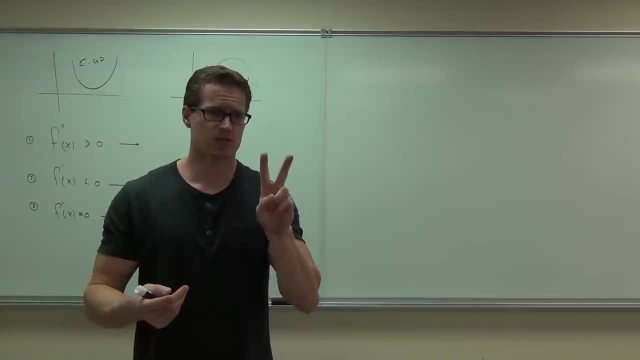 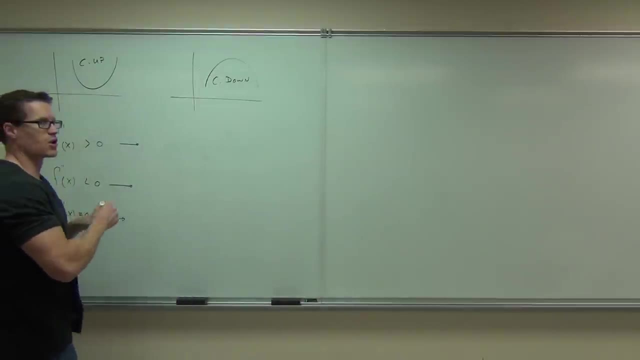 You with me on this. The first derivative was the slope. The second derivative is the rate of the change of the slope. Basically, if your slope is increasing or decreasing, So it says the slope's increasing, that's gonna give us a concave up. 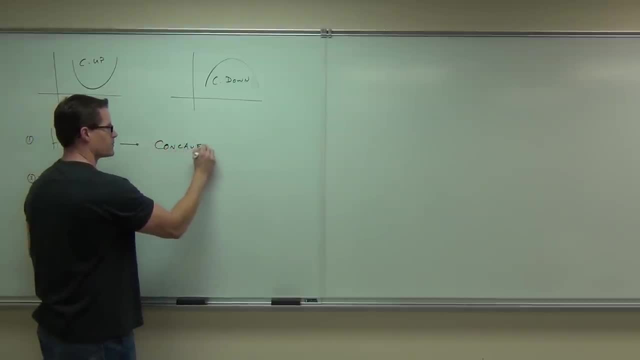 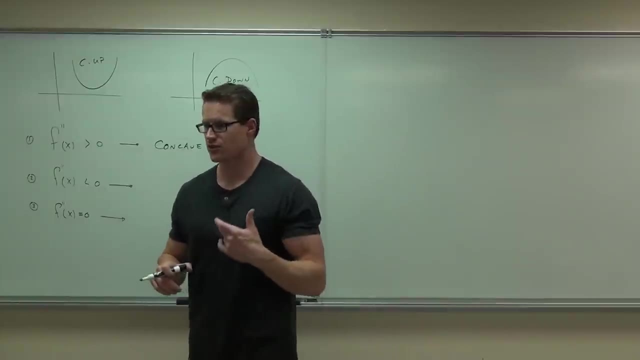 So this means concave up. If our second derivative is negative, that means the rate of change of our slope, how our slope's changing. that means it's negative. That means that the slope is actually decreasing. The slope is decreasing. slope is positive. 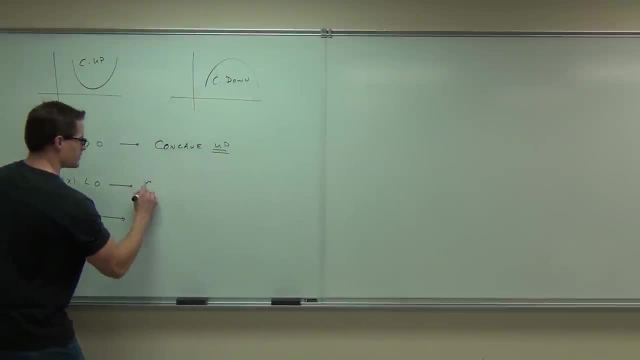 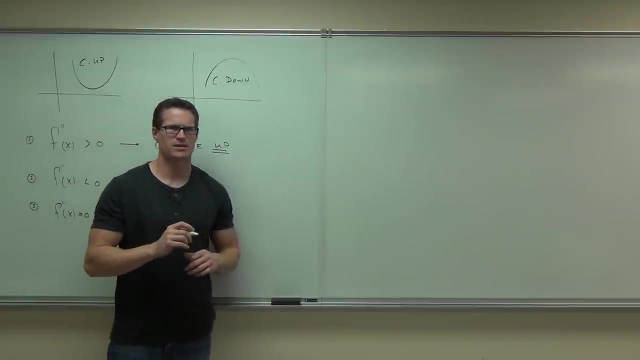 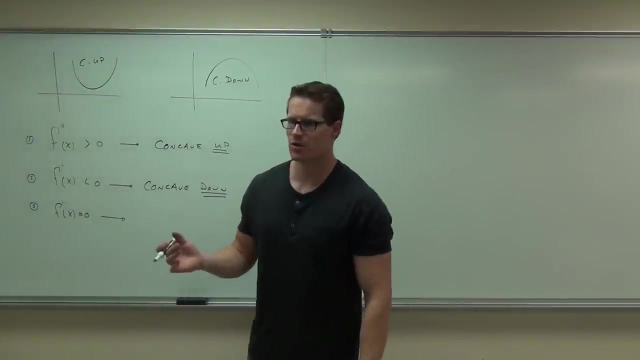 slope becomes zero. slope is negative. That gives us a concave down shape. I did explain all that last time, right, Okay, good, What would happen if the second derivative equals zero? Well, right now we have a question mark about that. 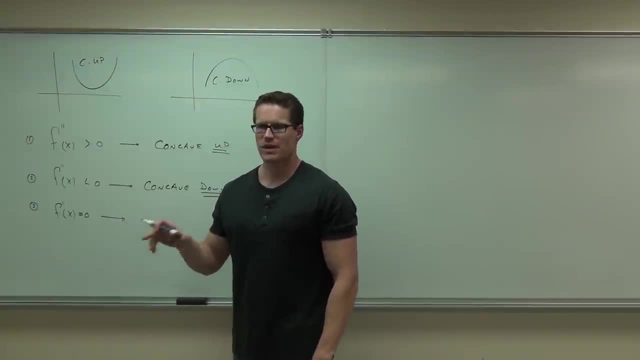 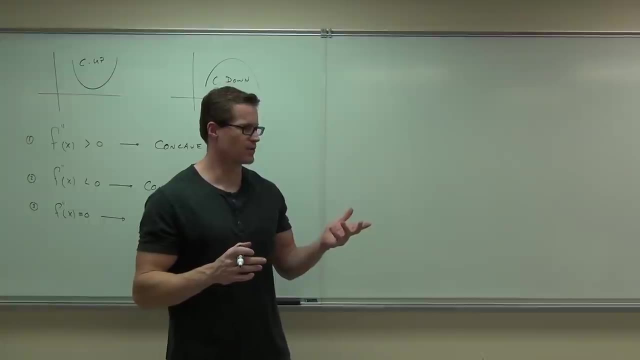 But here's what we're gonna fill this out as If the second derivative equals zero. that means the rate of change of the slope is positive. That means we don't know what's going on right there, but it could possibly be where it changes. 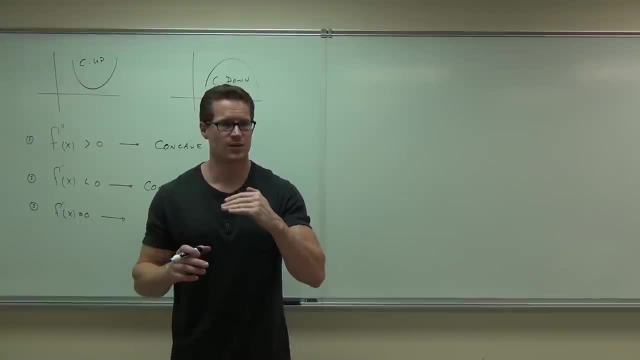 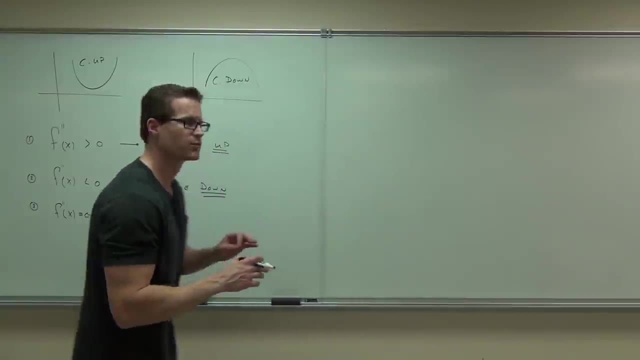 from concave up to concave down or concave down to concave up. Do you remember what that point was called Inflection point? This is a possible inflection point. There's cases where it's not, but it's possibly an inflection point. 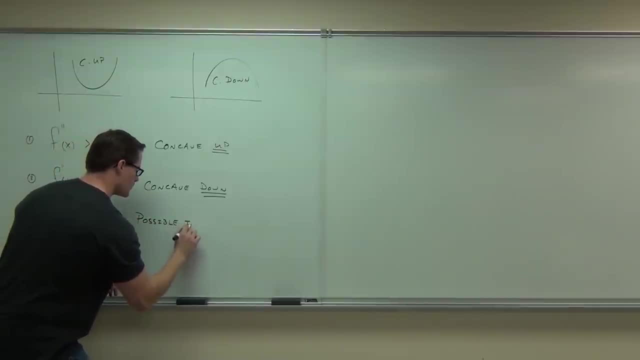 Or hip Hip. Let me review just a couple things with you. Let's give a couple graphs here. Do you have any inflection points on this graph? Yes, Could you tell me where it's concave up and where it's concave down? 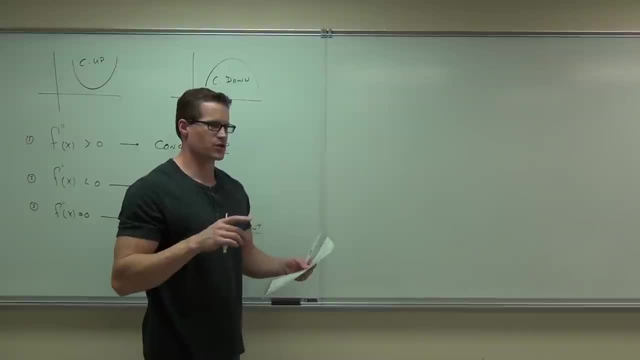 Yes, So if it's concave up and if it's concave down, then we're gonna have: if it's concave up, it's gonna be up, and if it's concave down, it's gonna be up. 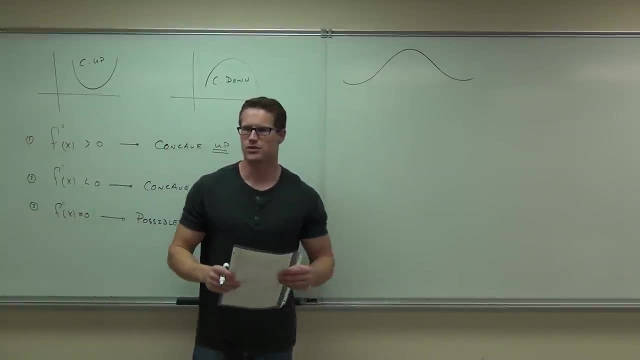 Then that's gonna be up. You don't have to be able to tell me if it's concave up or down. When it's concave up, it's gonna be up. Then you can't tell me where it's concave up. 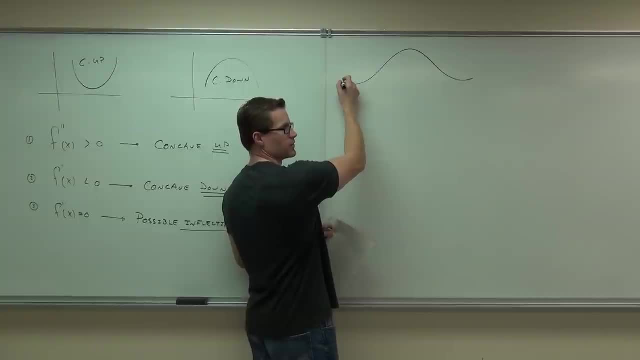 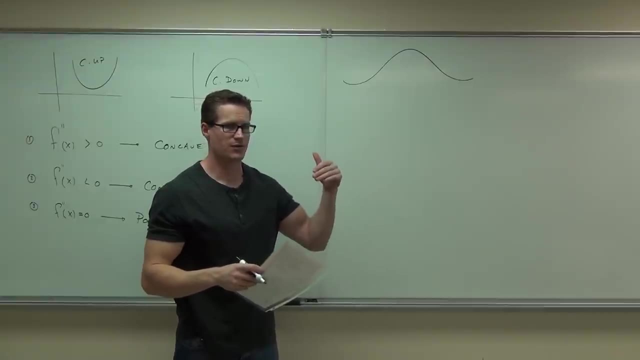 What am I starting out with? Concave up or concave down? Notice how concavity really doesn't have much to do. well, it does have to do with increasing and decreasing. but you can be concave up even though you're decreasing and increasing. 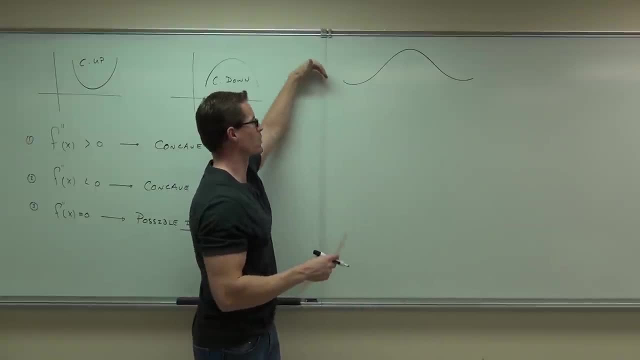 Do you see what I'm talking about Here? we start decreasing and then we increase. however, we're concave up the whole time. The concavity has to do with the slope, the way the slope is changing. If the slope is increasing, that means we're concave up. 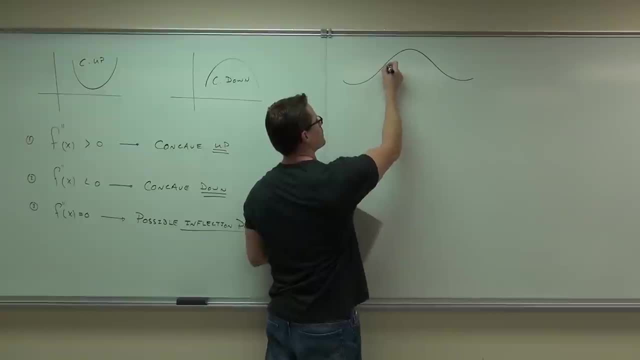 So we're concave up. tell me where to stop being concave up? Right in here. Somewhere in there? yeah for sure, Somewhere in there. we stop being concave up and we start being concave down. We start being able to hold water and 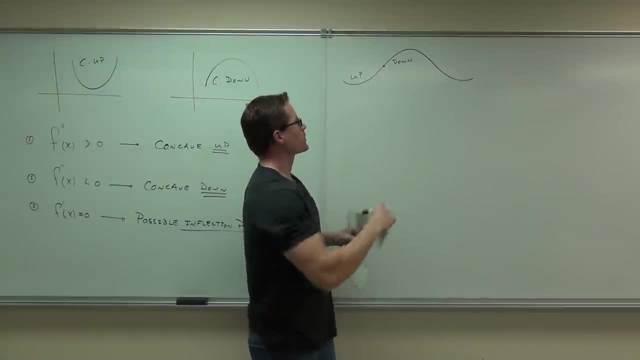 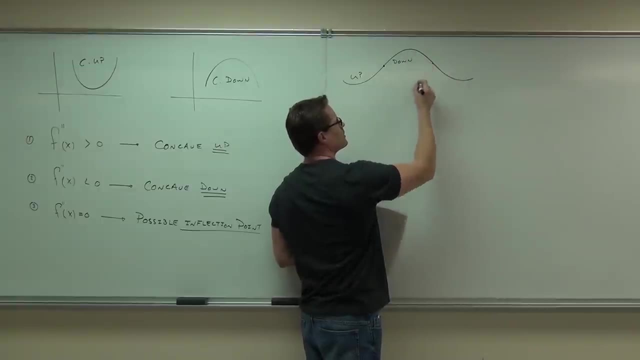 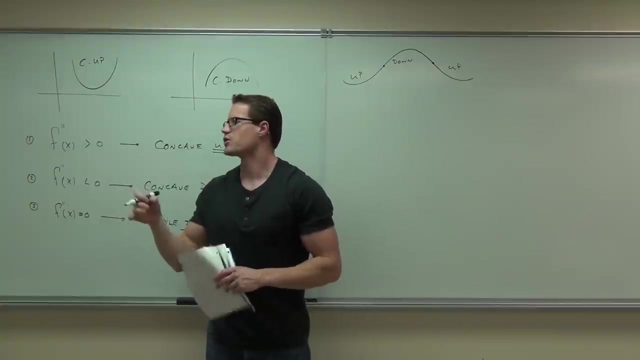 have something that doesn't hold water. Where do we stop being concave down? Somewhere in here? it looks like about right there to me, And then we're concave up for the rest of our curve. Those two points, those are called our. 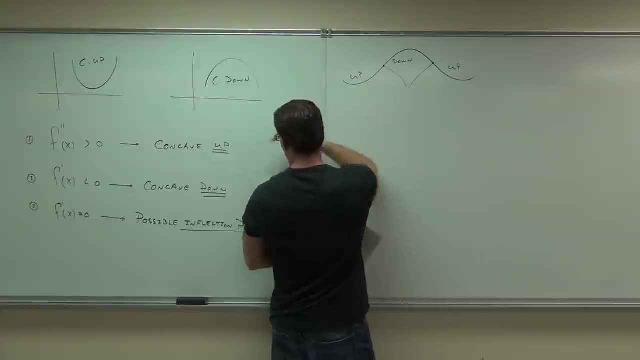 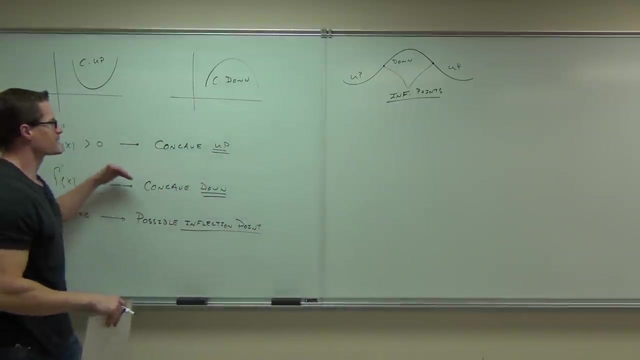 inflection points. So right here, this is how this would relate to this information. These are our inflection points. Let's look at the concave up. It says the second derivative should be positive. The second derivative says the slope should be increasing. Is the slope? 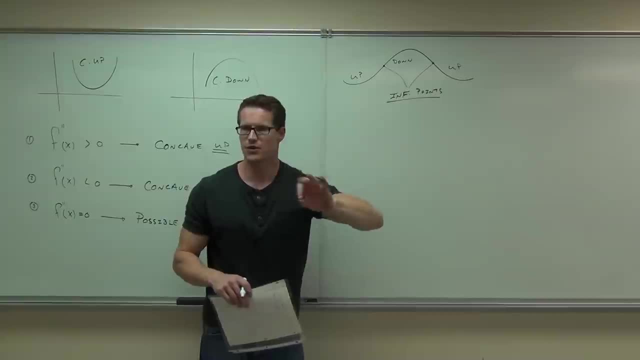 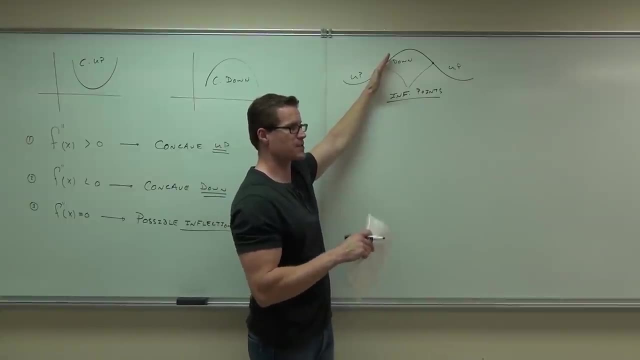 increasing here? Not the function, not the function, the slope. Is the slope increasing here? Sure, until it gets to that point? Guess what happens? at that point It stops increasing and it starts decreasing. In other words, our slope hits a peak and starts falling back down. 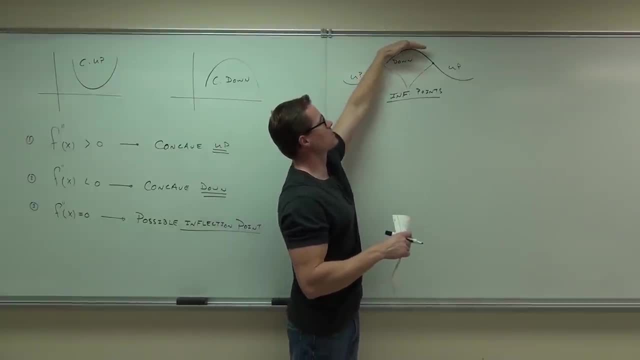 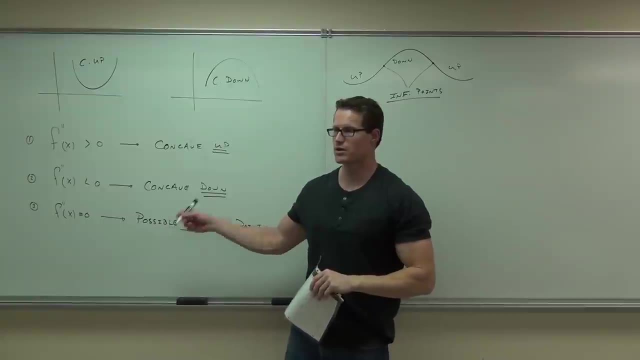 That's what that says. Now our slope is decreasing, decreasing, decreasing, decreasing, decreasing, until it hits that point and then starts increasing again At those inflection points. that's what's going to happen- is where your second derivative equals zero. 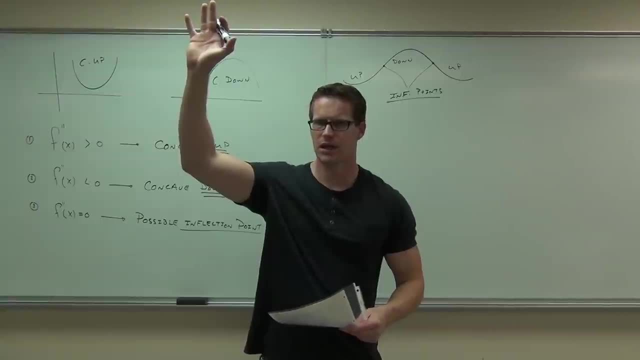 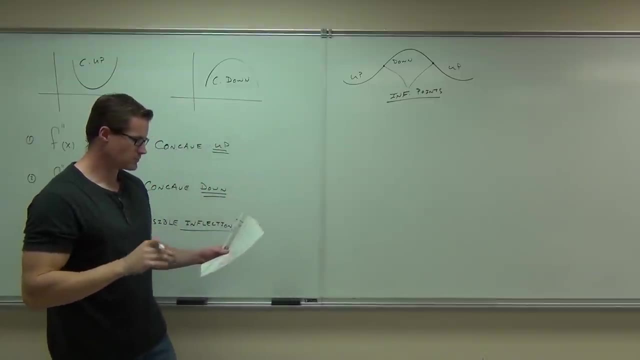 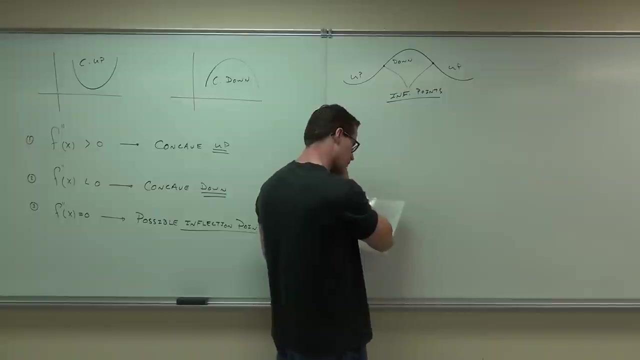 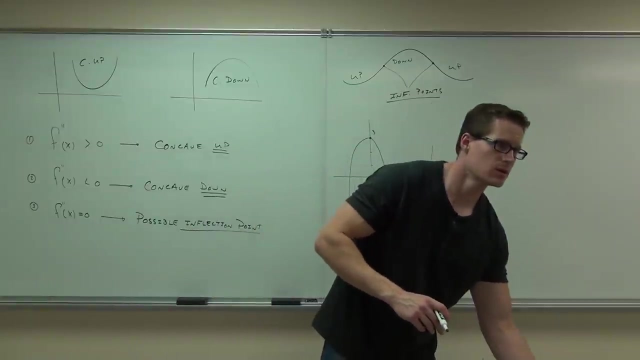 How many people have an okay understanding of our concavity and inflection points. I'm going to be very specific on how you actually find those later. okay, Okay, Would you be able to give me intervals of increasing, decreasing concavity? 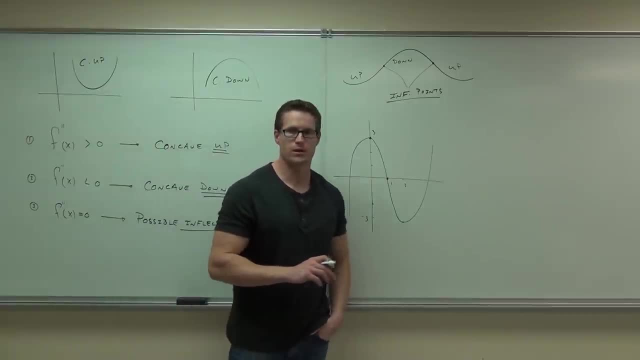 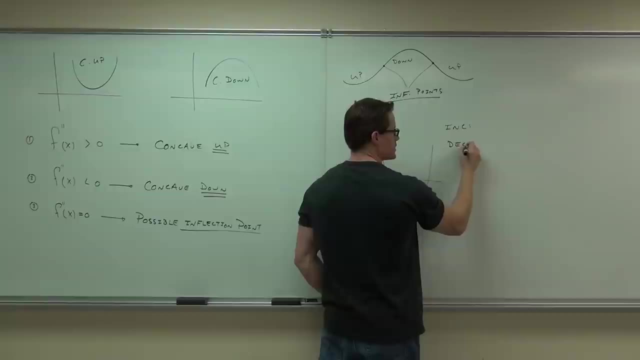 and any inflection points that occur. Would you be able to do that for me? Yeah, Can you tell me where we're increasing? Let's write that out: Increasing, decreasing, concave up, concave down and any inflection points. 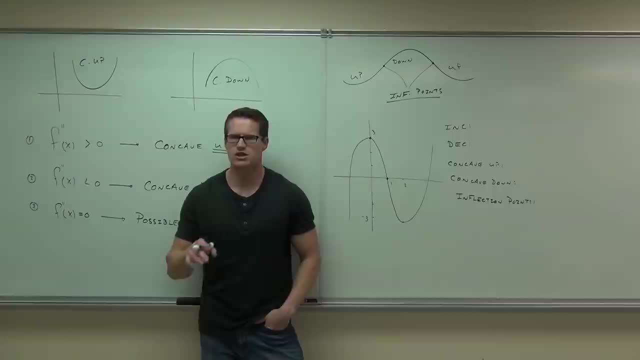 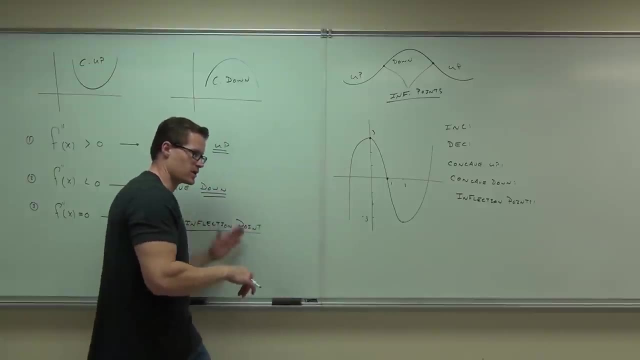 Where are we increasing? Give me an interval where we're increasing. Where are we increasing? The function needs to be going up from left to right. Where are we increasing? So, all the way from the start of our graph, which I mean, this goes way down. 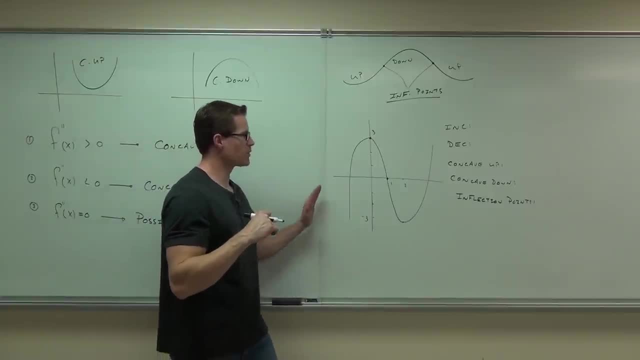 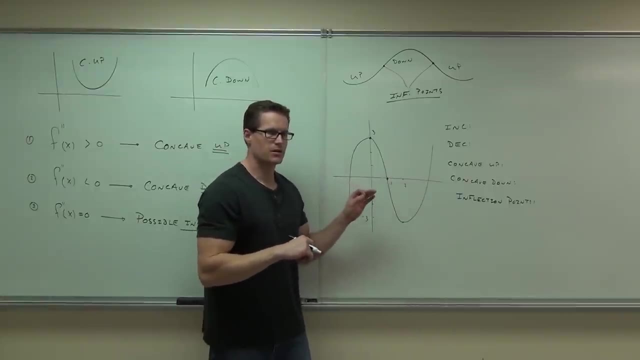 it can start ultimately from negative infinity. it increases all the way up. It's going up until we reach x equals what Zero? x doesn't equal 3.. I'm not talking about that. I'm talking about where does the function stop increasing? 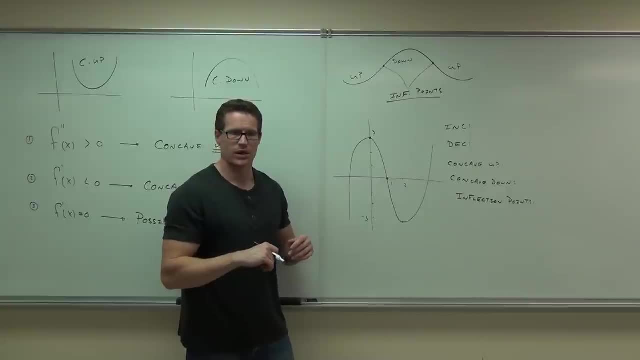 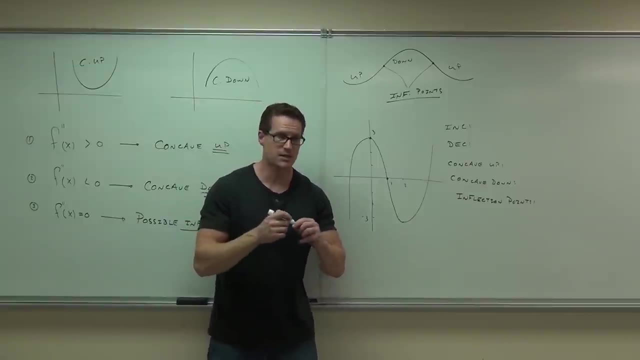 Where does it stop going up On the x-axis? where does it stop? When I say from negative infinity, here's what I don't mean. Some of you are a little bit shoddy on your graphing. Negative infinity doesn't mean I start down here. 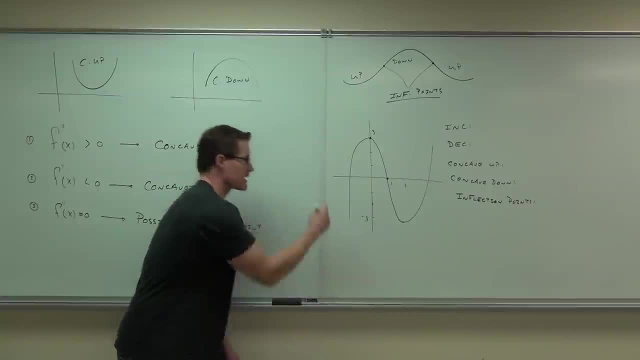 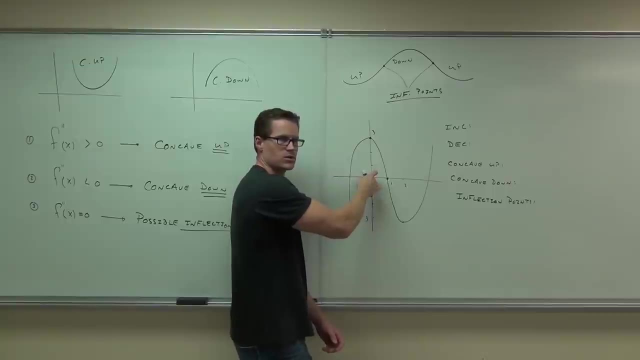 That's not what negative infinity on the x-axis means. The x-axis is this way right. It says: from negative infinity, I'm increasing all the way until I get to this point, which is zero. Do you see what I'm talking about? 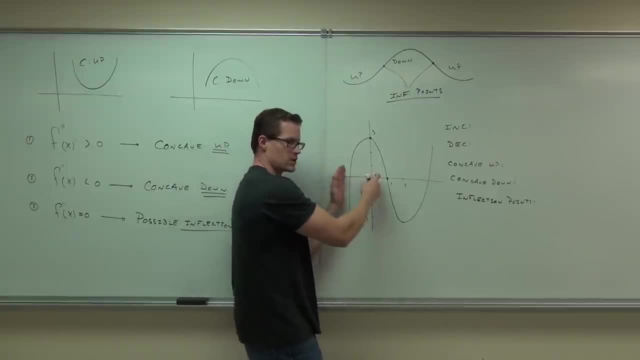 The function is going up. I don't care where the function stops, but on the x-axis, right there, it's increasing from negative infinity to zero. Are you okay with that? So not the height of the function, where it's increasing on the x-axis. 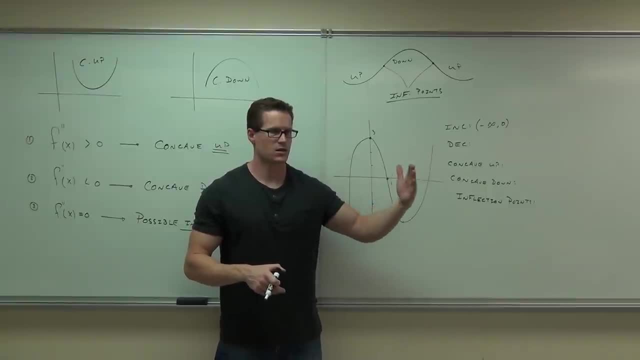 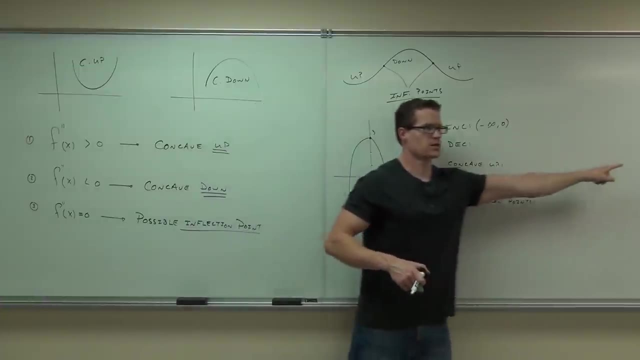 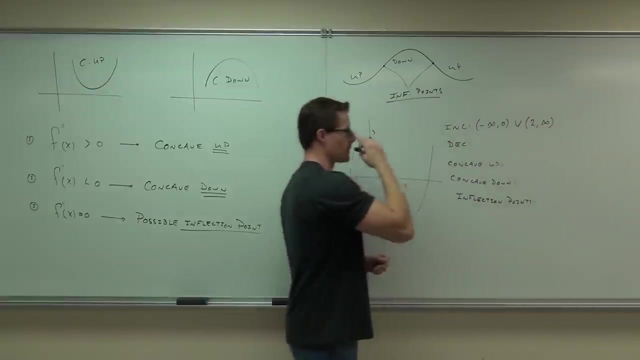 Does it pick up again and start increasing Mm-hmm? Where at x equals what Two? So from two to where? Infinity, From two to infinity on the x-axis would be another interval of increasing. Are you okay with the negative infinity to zero? 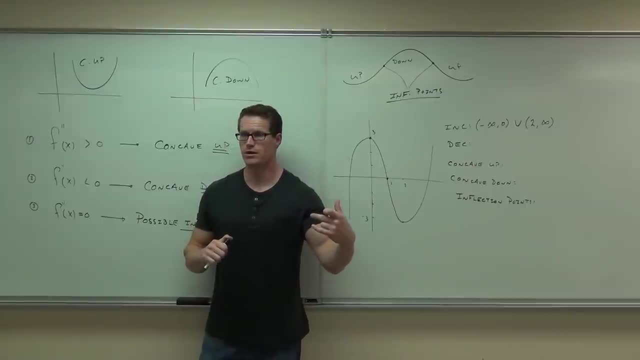 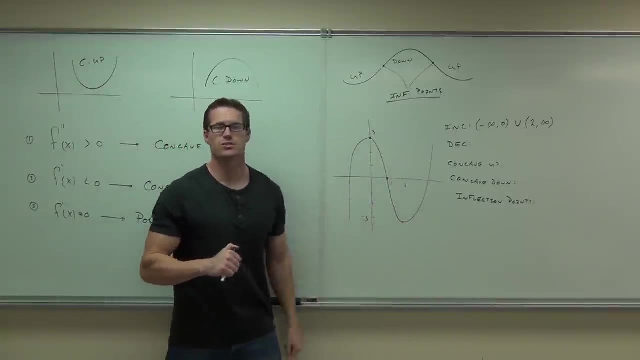 and then the two to infinity. I'm not sure if you are feeling okay with that. Okay, so we're not talking about this way. We're talking about what the function is doing as we're going along the x-axis. Give me decreasing. 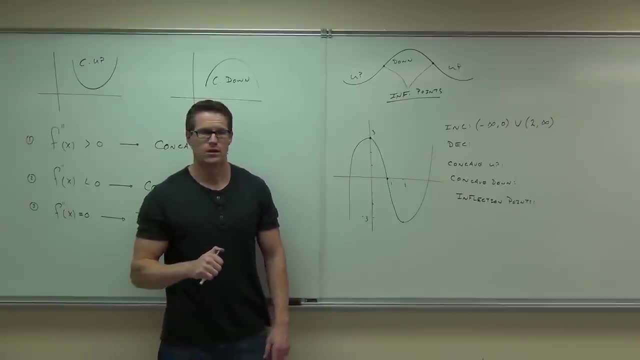 How many intervals do we have that are decreasing? One, From where to where? Zero to two. Yeah, if we're not understanding this, what some people will say is: from three to negative three. Is that our period of decreasing? No, no. 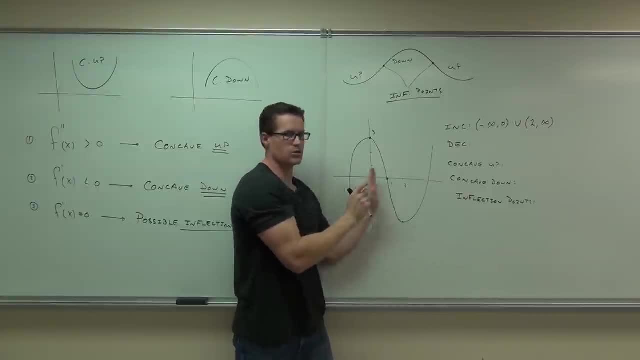 That would be the range that we're decreasing from here to here, which is what we're talking about there, Yeah or no? Are there questions about that? You guys are dead today. I see a lot of. It seems counterintuitive, not to say 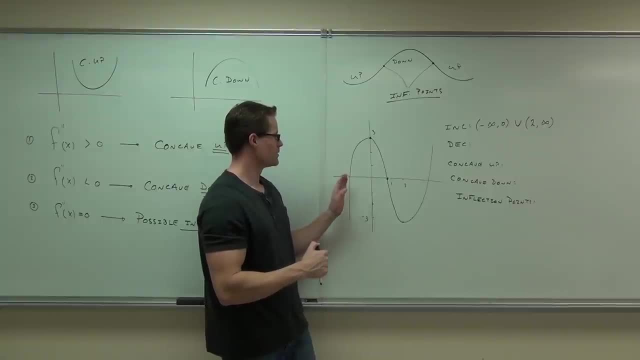 negative, one to zero. How do you get it increasing At that point where it crosses the x-axis the first time on the left, Right here, Yeah, But we're still increasing from here as well. So it's slowly eventually go. 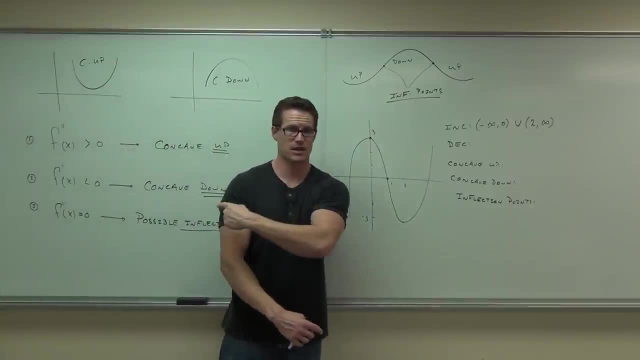 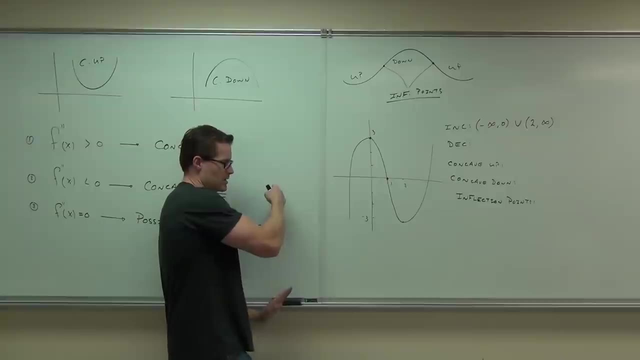 We always read from left to right: Negative infinity, because it never ends. When we start this function, it's automatically starting to go up And it keeps going up like a timeline right. It keeps going up, keeps going up. 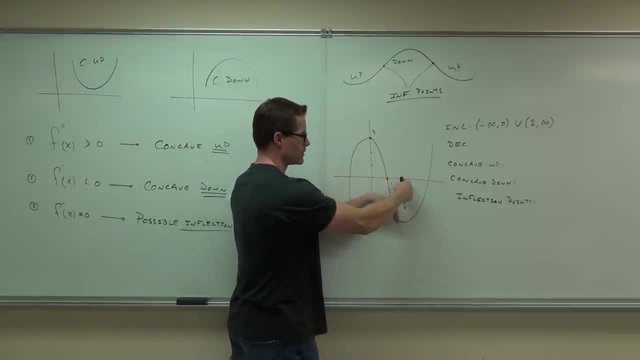 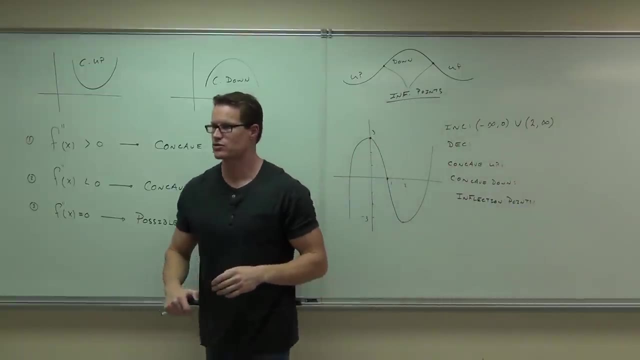 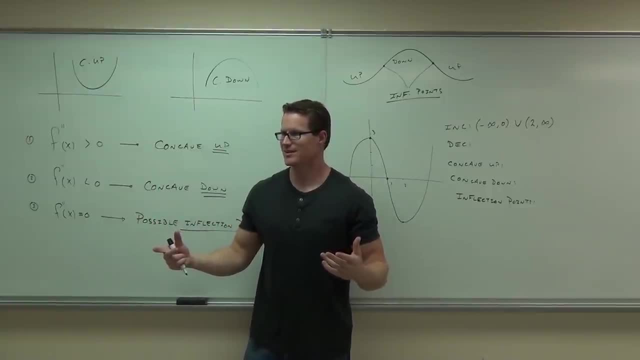 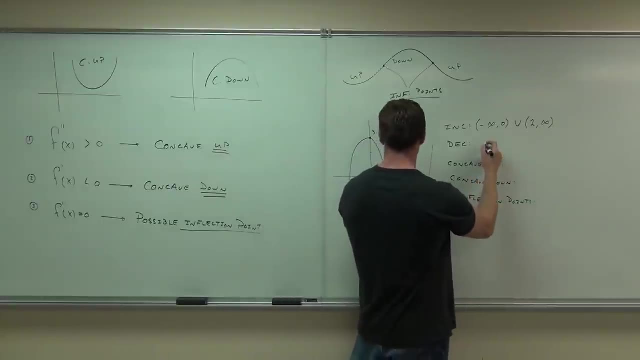 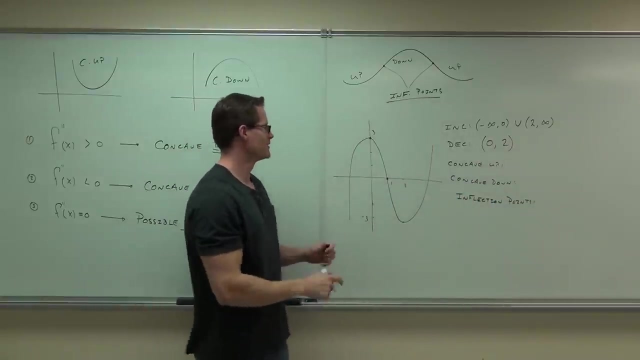 Have I drawled you into a state where you're almost sleeping now? Yes, Good, Two hours of sleep. Hey, me too. All you have to do is sit there. Think about me, Come on, Selfish people. Zero to two is decreasing. 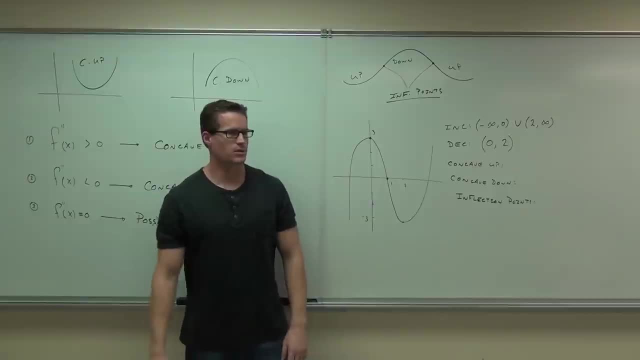 If you need more help on that, you come and see me. How about concave up? You need to be able to determine concave up to concave down. Am I concave up here? No, This is concave up, Concave up. 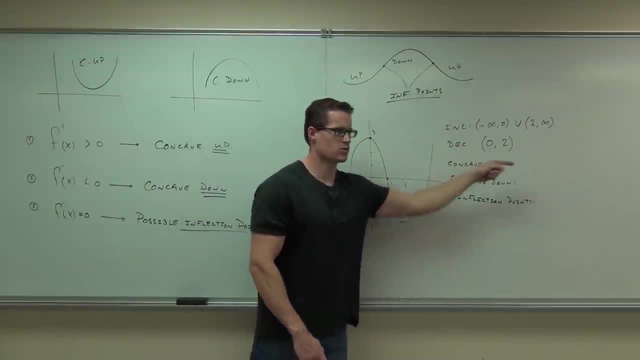 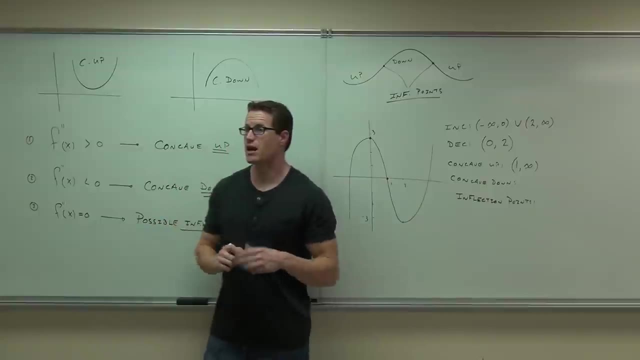 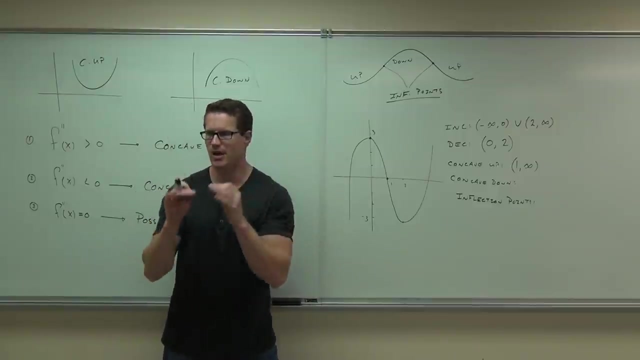 Forever. Concave up from one to infinity Concave down. let's start that. Remember it has to go in order of a number line. Where do we start being concave down? Remember you're talking about the x-axis, the x-axis. 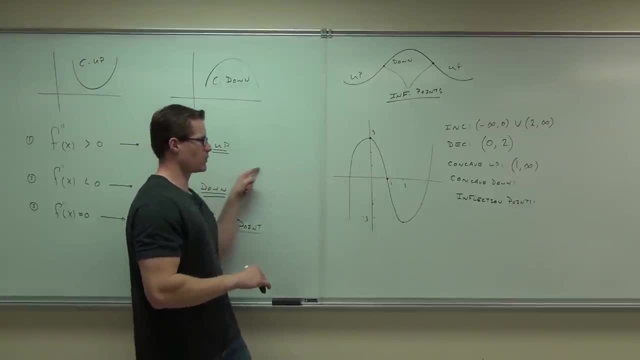 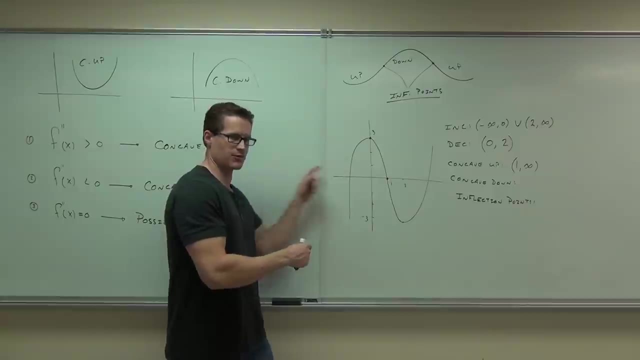 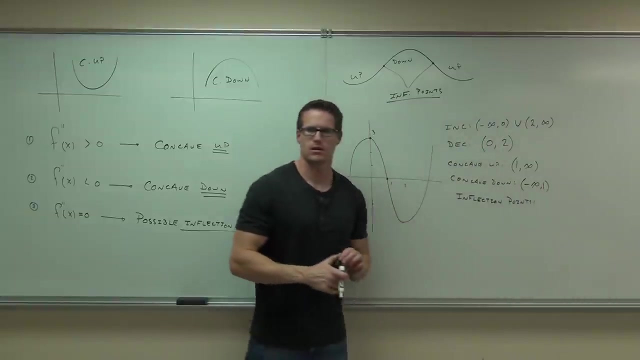 Where do you start being concave down? Up to what point? One? It's all concave down until you get to here. right, The x-axis says negative infinity to one. Is there an inflection point If you change the concavity? 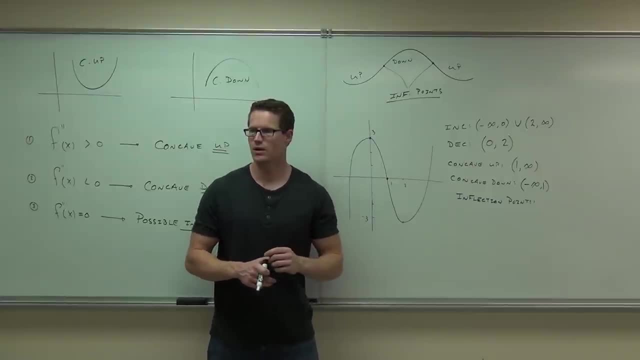 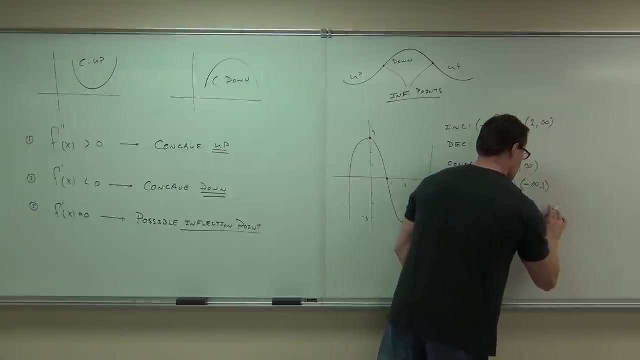 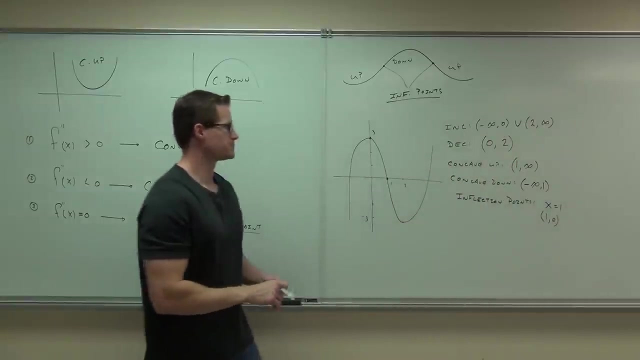 you have an inflection point. What is that Zero? Does it change the concavity here? Does it change the concavity here? No, x equals one, Or the point. I know the notation kind of sucks because we don't have different notation. 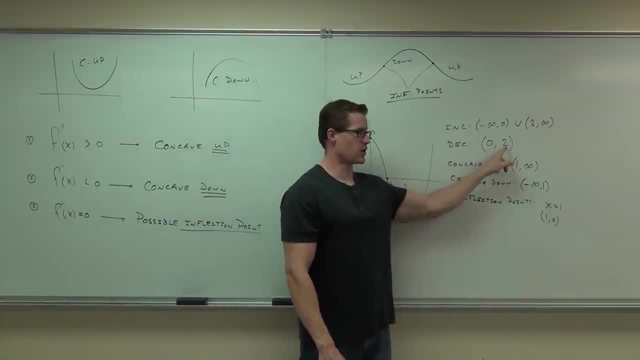 for intervals versus points. That's an interval That says from zero to two- non-inclusive, From one to infinity- non-inclusive, Negative infinity- to one non-inclusive. That's a point. one to zero, That's an actual, specific point. 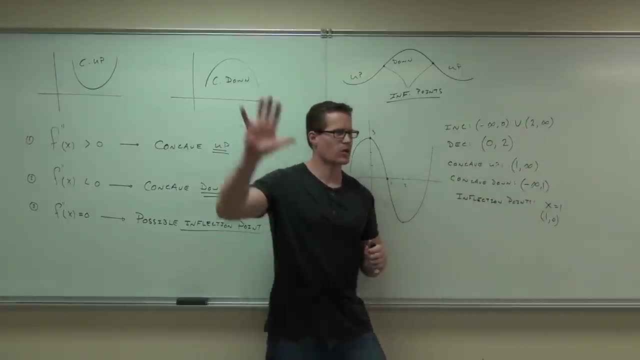 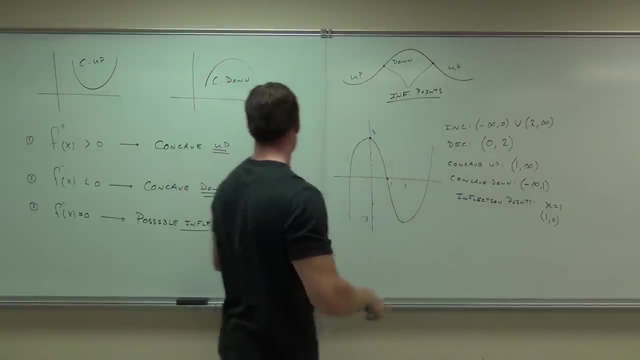 There are some numbers, but this is a point. Those are all intervals, But you have to be okay with our intervals of increasing and decreasing. Ify, stick with it. We'll talk about one more. You'll get practice on it on your homework as well. 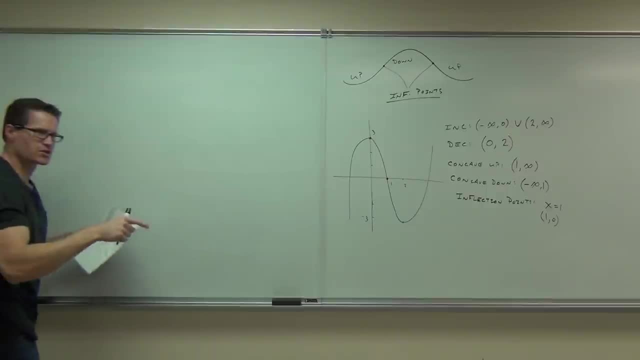 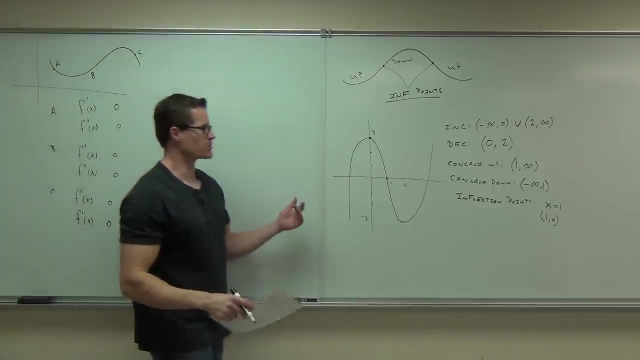 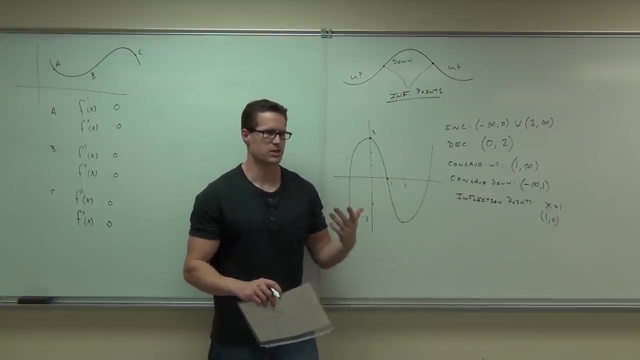 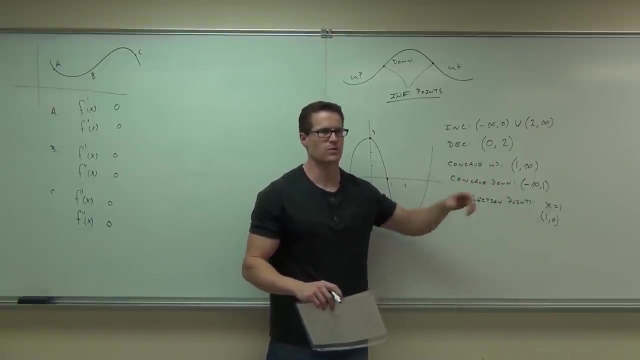 How about this? Let's see if you really understand what you're doing here again, from 2 to infinity, and that's what we're talking about, and that's what how. 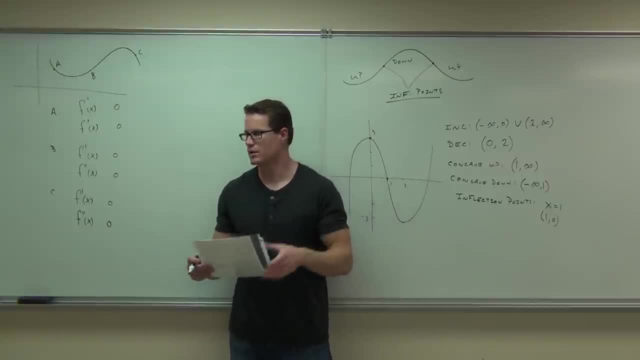 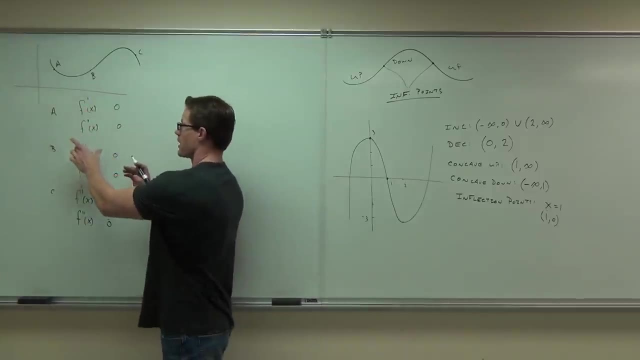 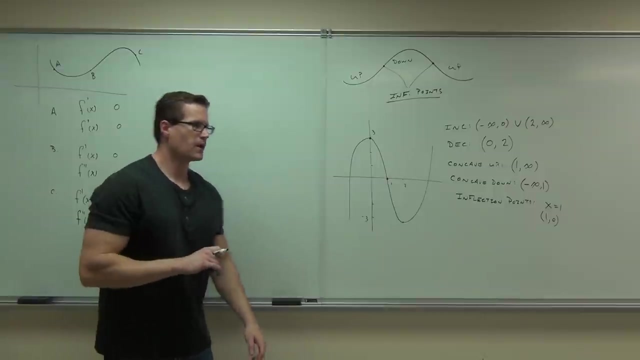 you determine those intervals. does that make a little bit more sense, hopefully now at each point. here's what I want to do. I want to determine whether our first derivative force and second derivative are positive or negative. that's what I want to do here. so let's take a look at it. let's look at point a. I'll help you. 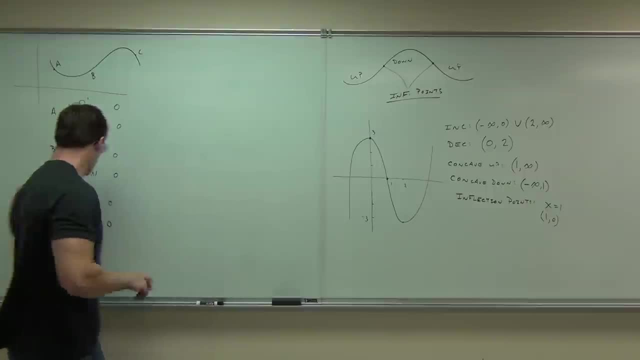 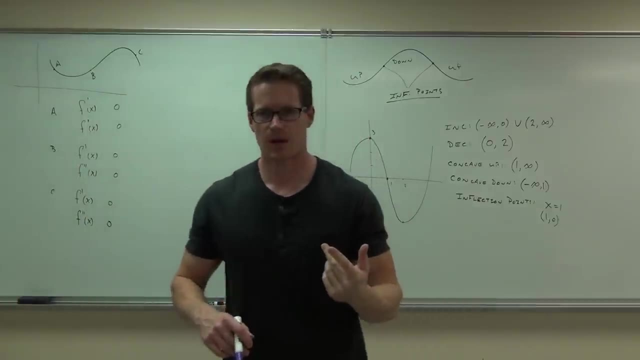 out with point a and then the rest of them I want you to do on your own, just practice it. on point a, I want you to look at our first derivative. the first derivative means slope. the first derivative says whether I'm increasing or decreasing. remember that first derivative says increase or decreasing. 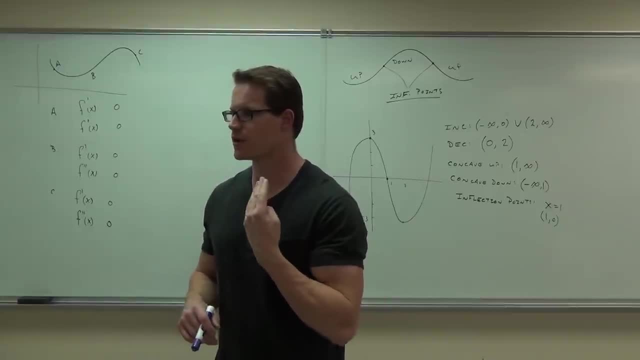 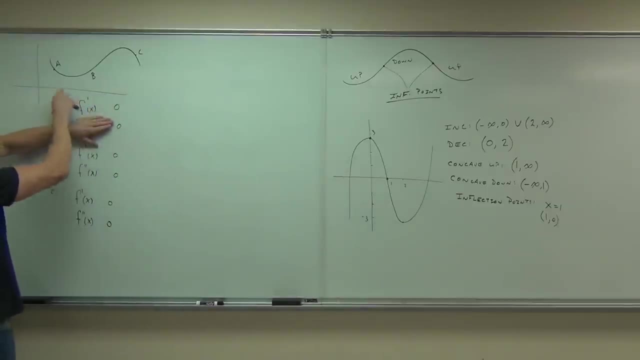 if the first derivative is positive, I'm increasing, going up. the first derivative is negative, I'm decreasing, going down. so let's look at very carefully, very slowly. let's think about the first derivative. at a, is my function climbing or falling? at the point a, is that increase or decrease? so should this be positive or negative? the first: 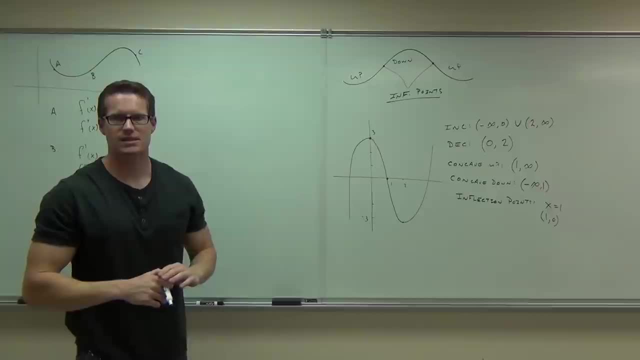 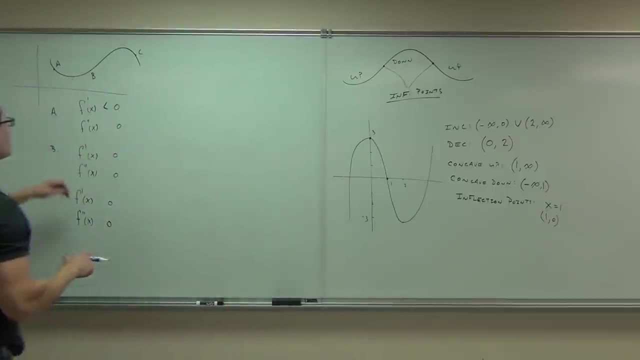 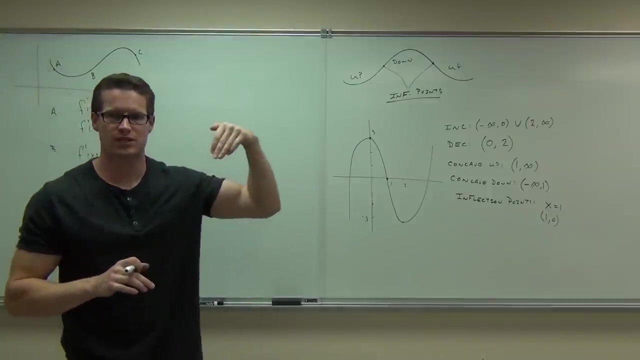 derivative will be negative. they're definitely negative. it says that my slope is negative. my slopes less than zero. that means I'm decreasing. do you follow me now? let's think about the second derivative at the point a. the second derivative says whether my slope is changing positively or negatively. 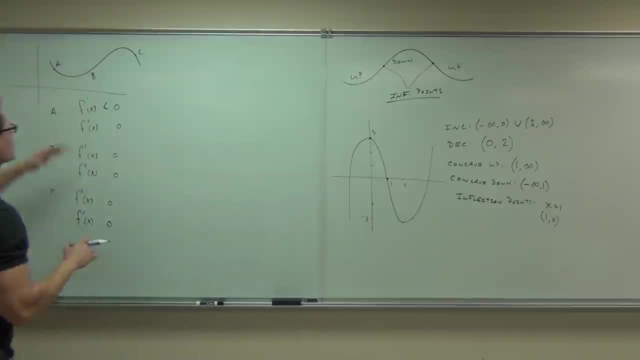 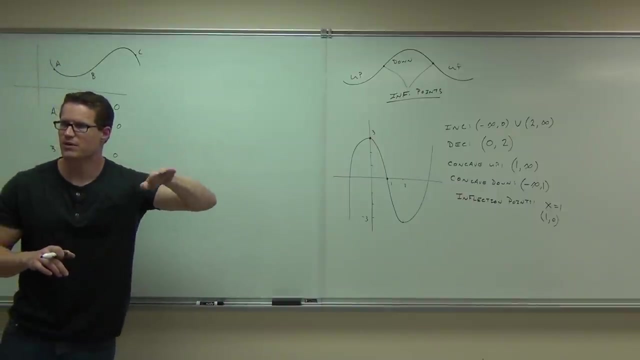 isn't. my slope is increasing or my slope is decreasing. so think about this: is my slope getting gradually bigger or getting gradually smaller, so that my slope is increasing? do you follow me? my slope is increasing also. that means I should be concave up, my concave up right there, for concave up is 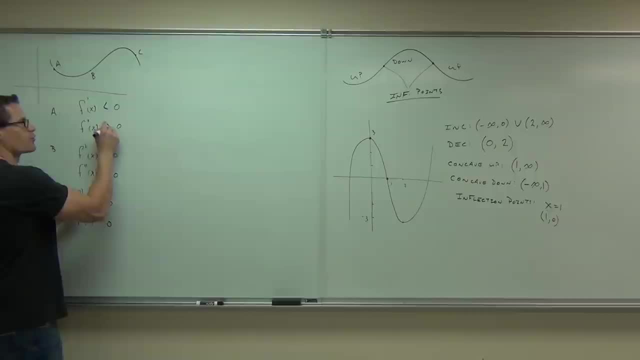 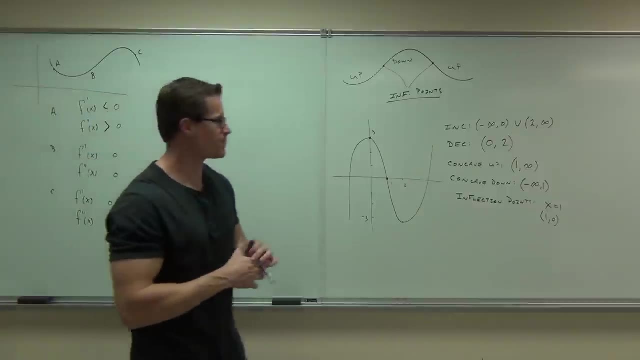 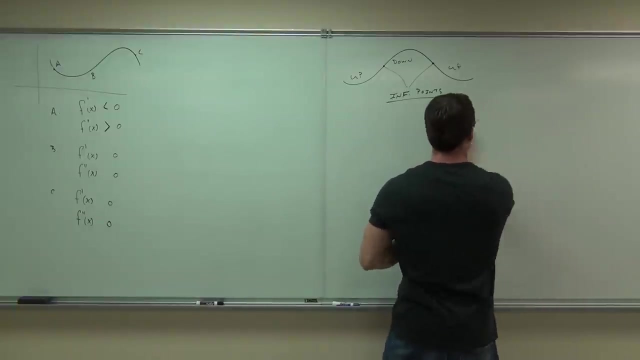 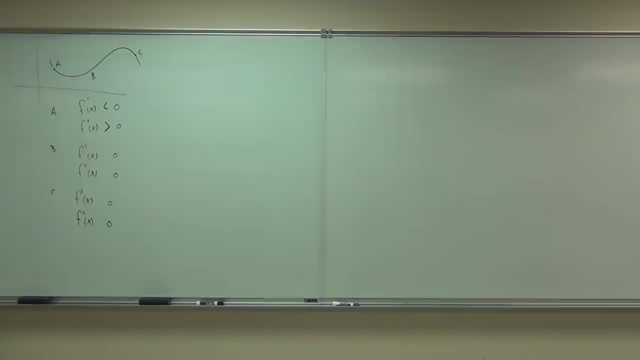 that positive or negative? the second derivative will be positive. it says my slope is increasing. my second derivative should be positive. do the rest do b and c? now? do I have a positive or negative derivative, or negative? i, i didn't see it. i i checked my slower, wasn't it? 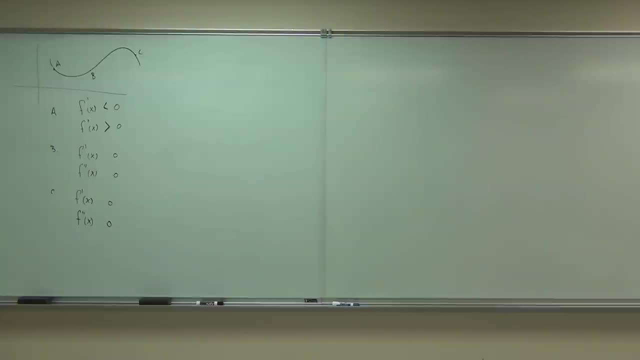 I make sure my slope moves up, because I know if my slope is losing i have to dismiss. All right, so let's go for it At point B. if I'm looking at point B, my function's increasing, My slope is positive, so this should be positive. 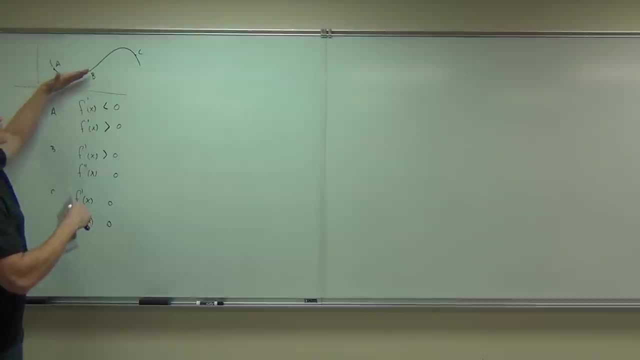 At point B. well, that's almost at the cutoff, but it's still. the slope is still a little bit increasing right there. So at point B we're still increasing. This should also be positive. Did you get both of those positive? 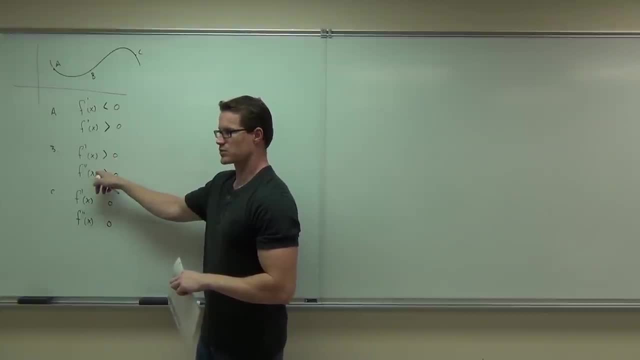 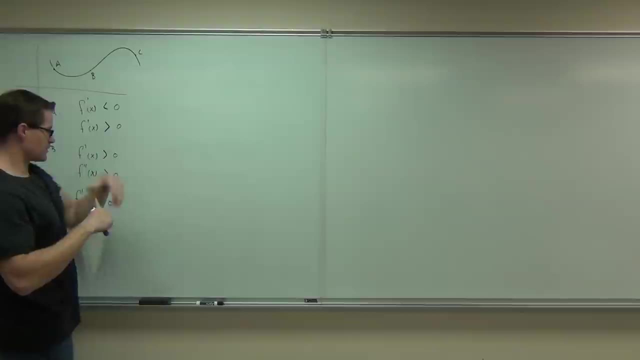 It's increasing and it's concave up. That's how you can view that as well. Point C: at point C, my function is decreasing. My slope is negative. That means my slope is negative. That's certainly true. And also my slope is getting gradually less and less and less. 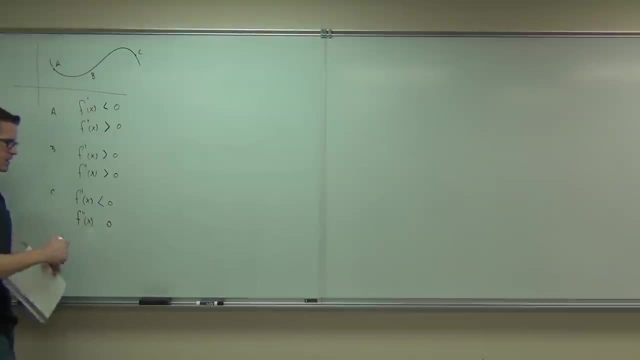 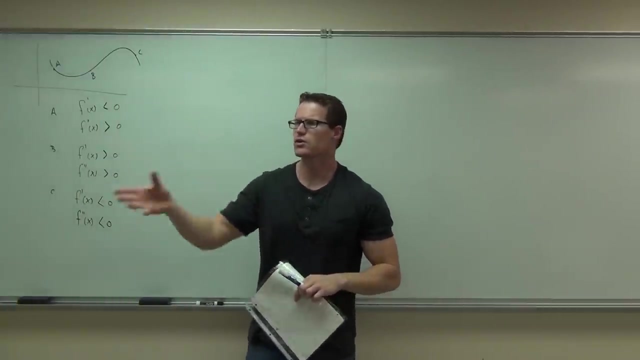 So my slope is decreasing as well. If my slope is decreasing, that's also negative concave down as well. How many of you got both of those right? Good for you. If not notice where your mistake was, Was it the first derivative or second derivative? 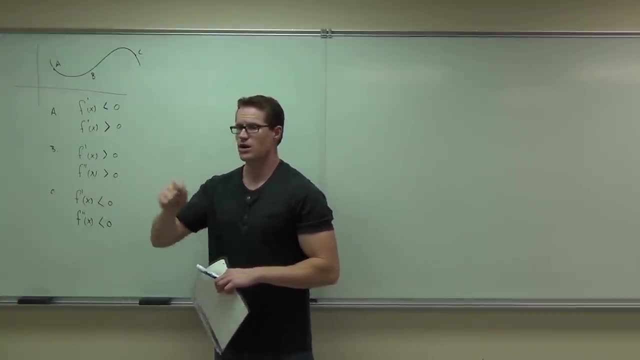 First derivative is increasing, decreasing. Second derivative is concavity: Decreasing concave up. Decreasing concave up. Increasing concave up. Increasing concave up. Decreasing concave down. Decreasing concave down. 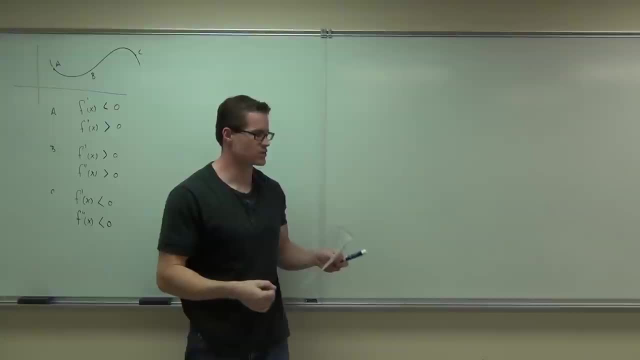 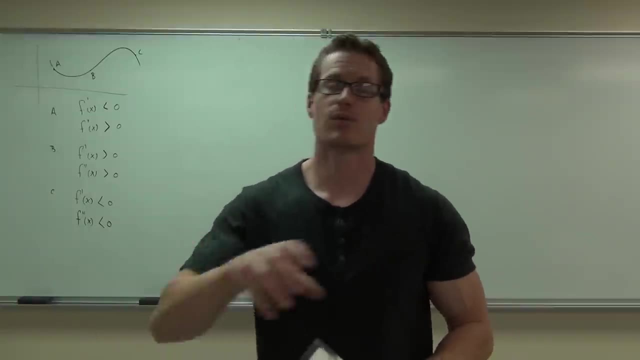 That's the same exact language or the same exact idea that we just talked about. Now the next thing we're going to start getting into is relative extrema and how that relates to graphing polynomials. So let's look a little bit about what relative extrema means. 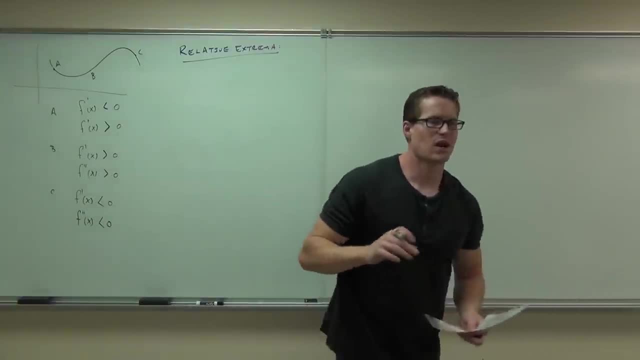 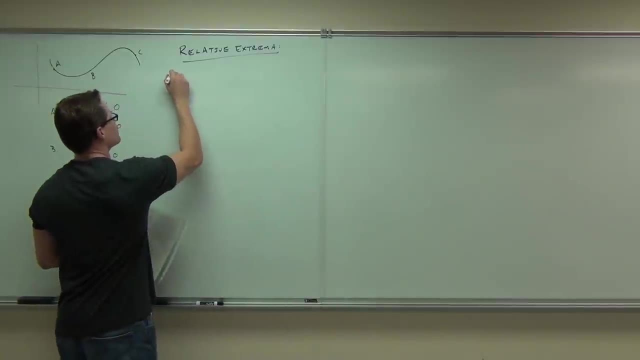 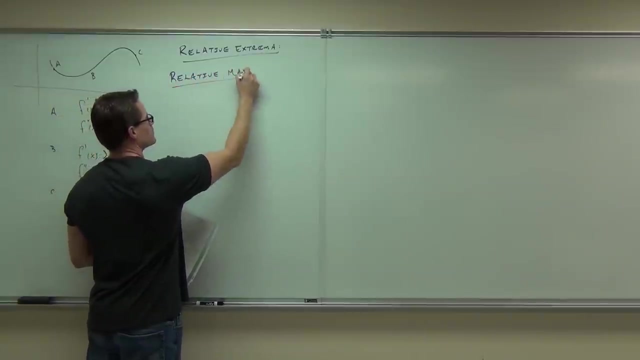 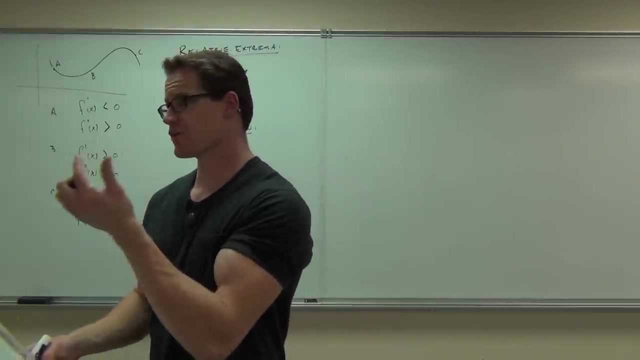 It's not. It's not. Here's what a relative extrema means. It means a relative max or relative min. You've heard that before. Yeah, Just to refresh your memory. a relative max is basically the idea of a high point on an interval. 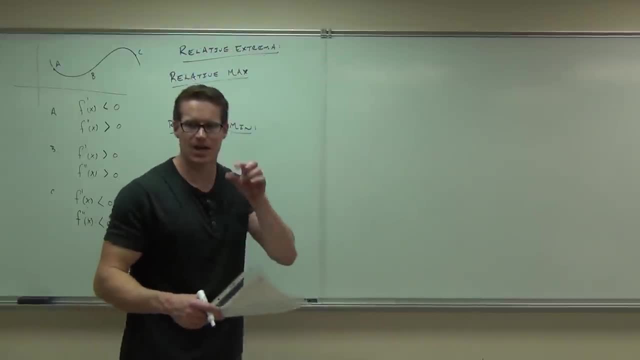 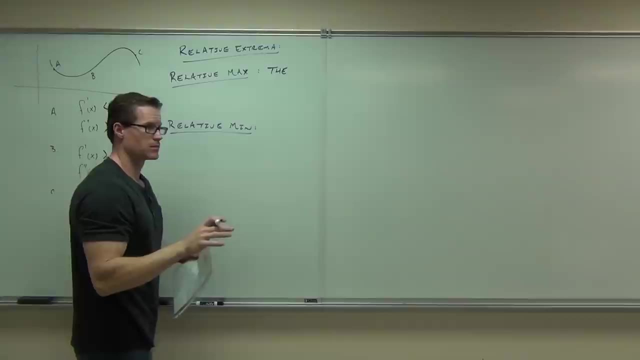 It doesn't have to be the highest point on the graph, It just has to be the high point on a little interval. It's about the peak right. It is a peak. It is a peak. It's a peak for an interval. 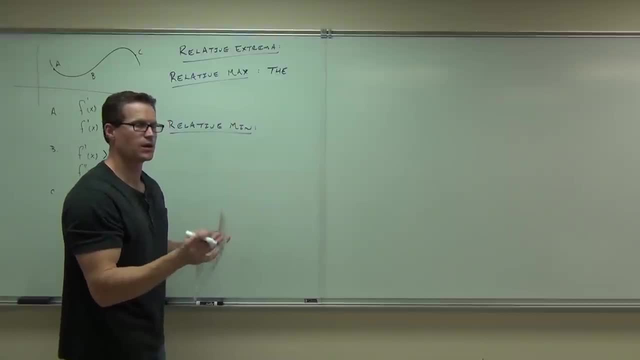 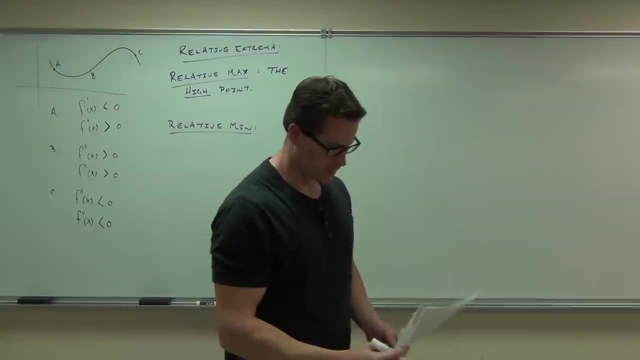 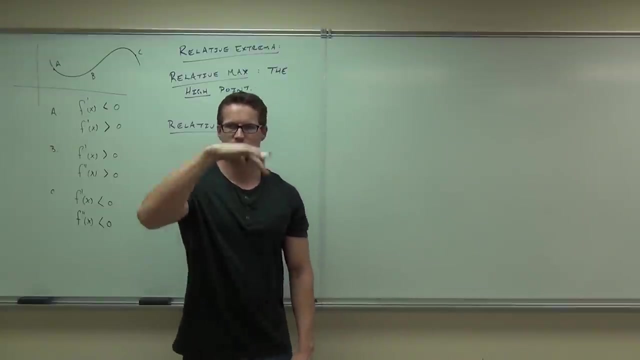 Not the absolute. not the absolute max necessarily, but it is for an interval. The high point Here's a better definition. A relative max happens when a function changes from increasing to decreasing. That should make sense to us, right From increasing to look at from increasing. 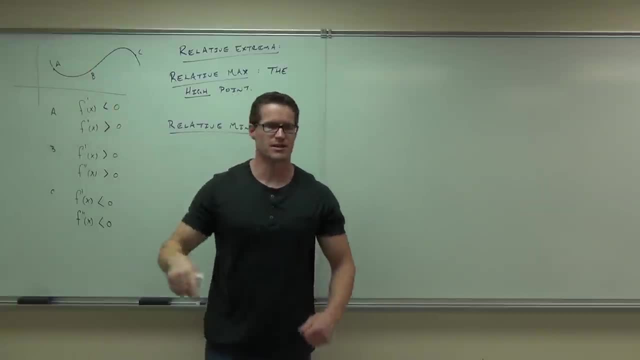 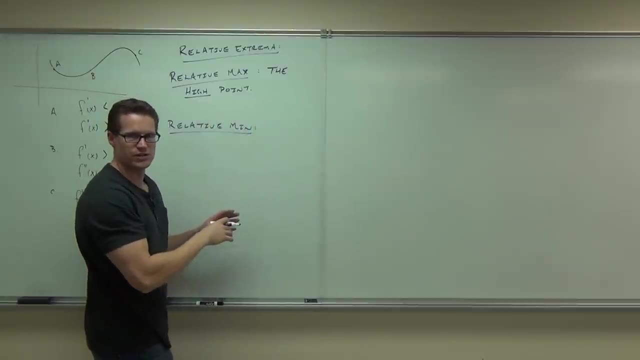 to decreasing, we should have a peak. That's a relative max. It doesn't have to be the highest point on the graph, but that's the definition for relative max. So the high point, that's kind of an old, old definition. 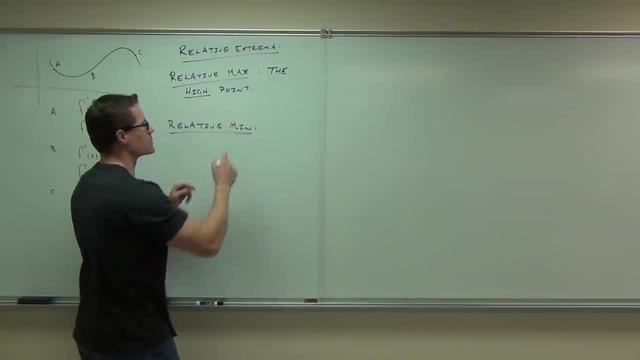 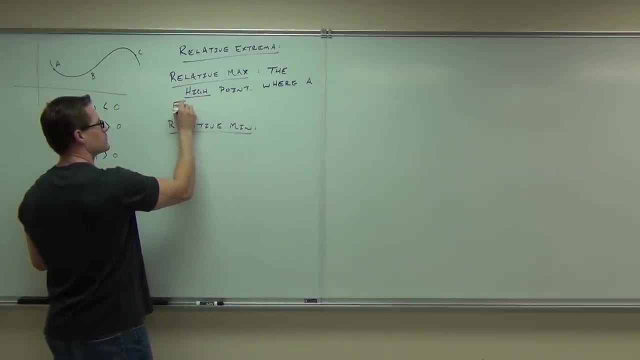 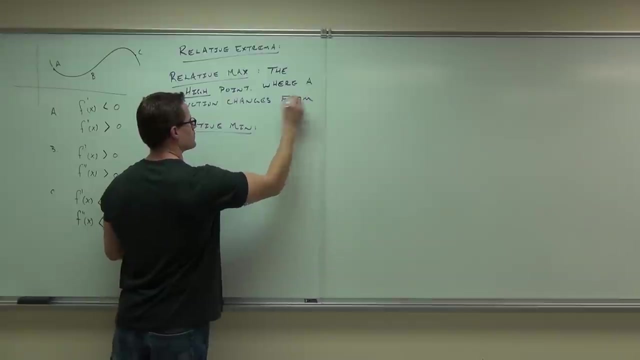 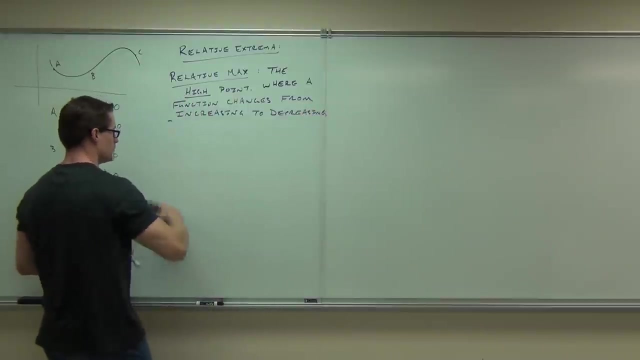 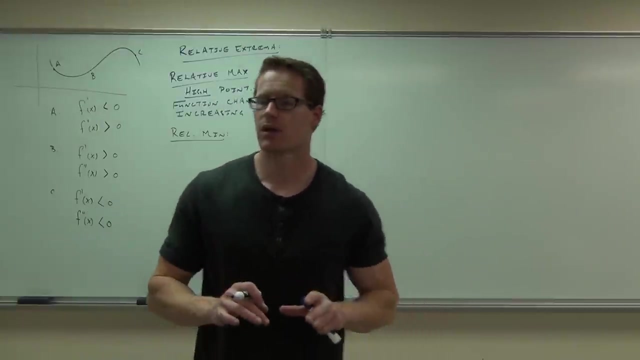 It's not very mathematical. This is where a function changes from increasing to decreasing. You know what relative min has? basically the opposite definition, right there. A relative min is going to be a low point in an interval. In other words, it's going to be where you change from decreasing to increasing. 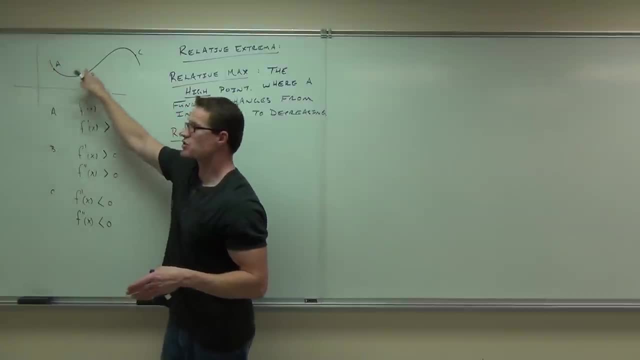 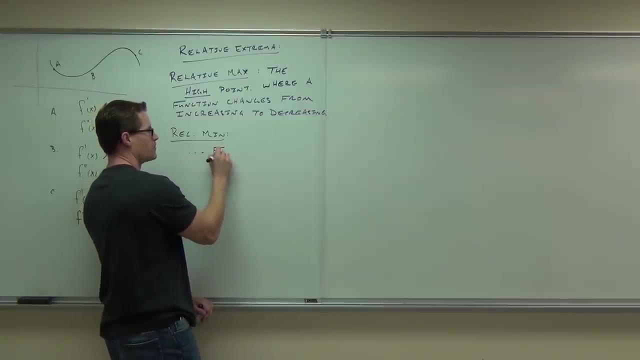 And that's what it does. That should make sense, right? If you go from decreasing to increasing, you're going to have a little valley, a low point. So dot, dot, dot, where the function changes from decreasing to increasing. 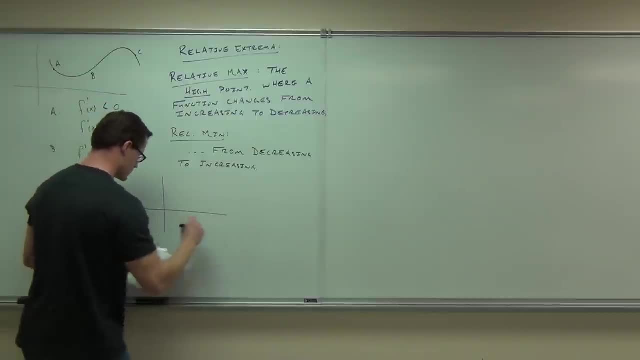 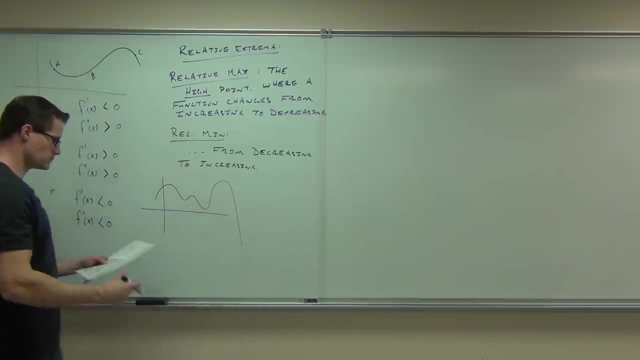 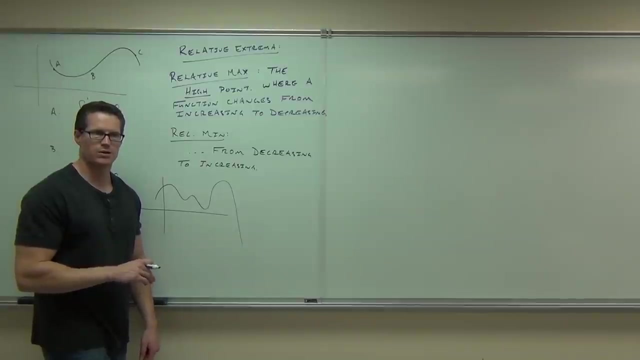 Very quick examples for you, just so you have a little look at this. Would you be able to find me my relative extrema here? Relative extrema happens where you are changing from increasing to decreasing or decreasing to increasing. So stop me when I get to relative extrema. OK, 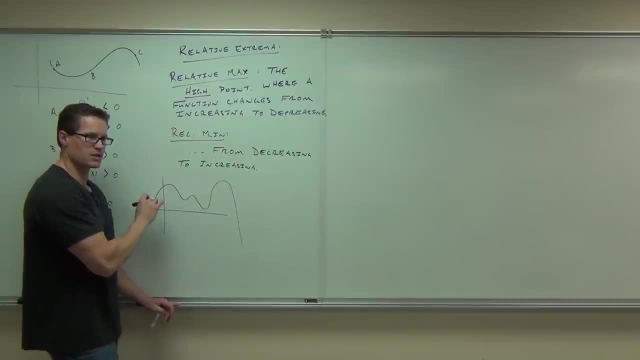 Here? no, No, because we're not changing from increasing to decreasing. OK, You have that as part of our definition, So we're going to start here. no, Where do I get one? What is this Relative max? very good. 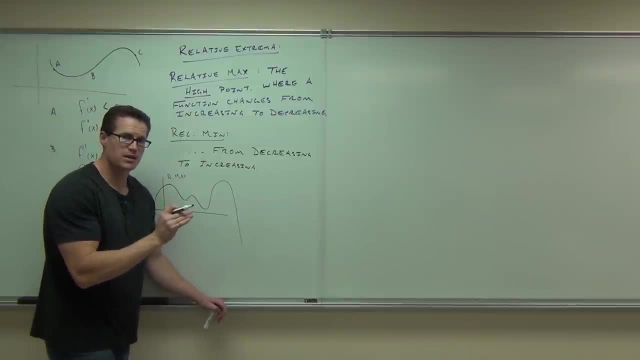 Relative max. Is it the absolute max? Is it the highest? my function goes. That would be right. That would be. How about? let's keep going. What else Here? that's a relative min. Relative min, Keep going. 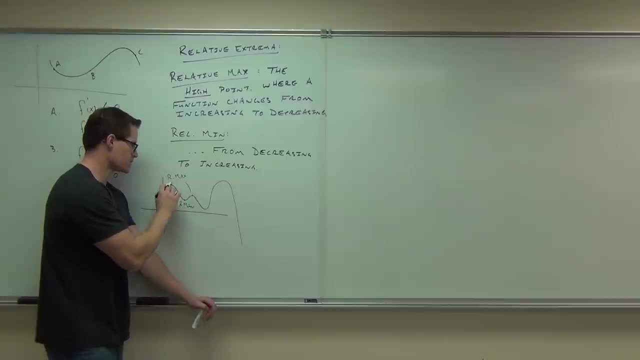 This one There, Yeah, That's another relative max. And then there, that's another relative min. And then how about this one? Even though it's an absolute max, which we'll talk about later, it could still be a relative max, no problem. 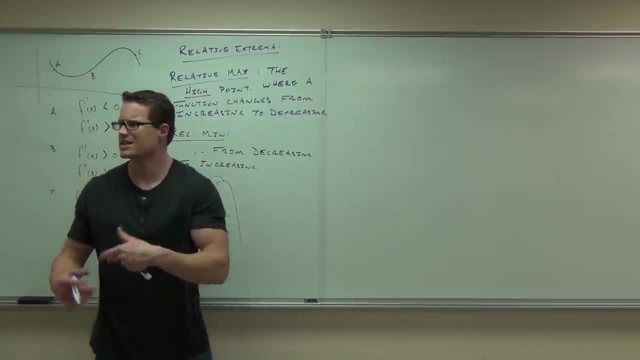 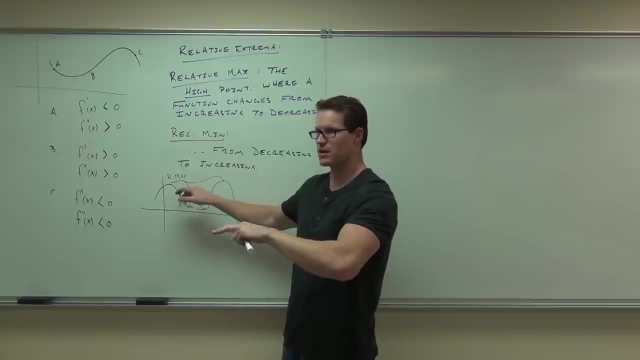 We have three relative maxes. We have two relative mins. on this problem, Do you understand the idea of a relative max, relative min Changing from increasing to decreasing four maxes? that gives us a peak Decreasing and increasing for relative min. 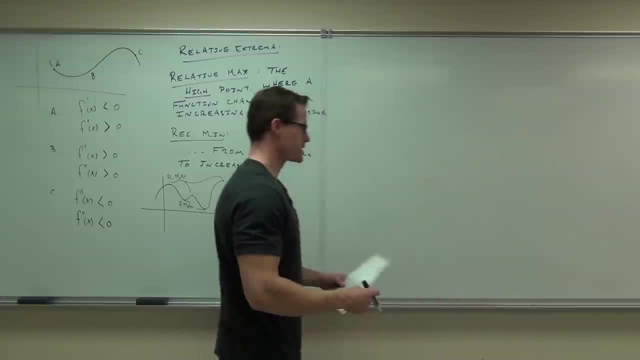 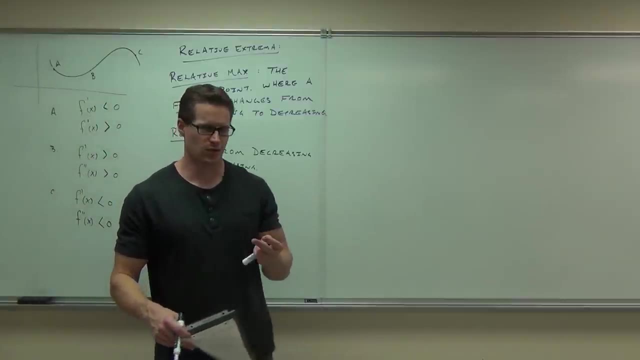 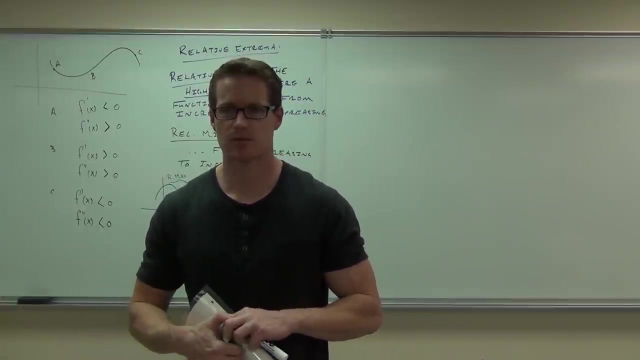 that gives us a value. My question is this: If this is a change from increasing to decreasing or decreasing to increasing, that has to do with the slope, doesn't it? If the slope is positive, we're increasing, right. The slope is negative, we're decreasing- true. 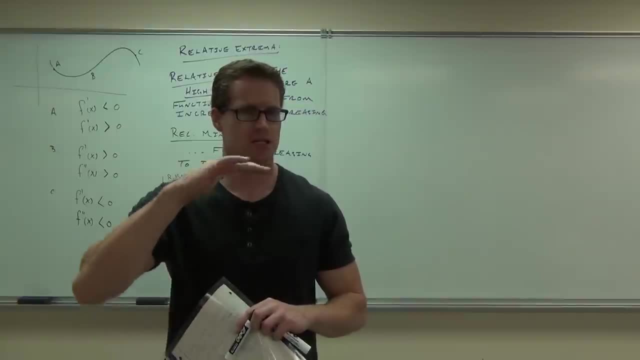 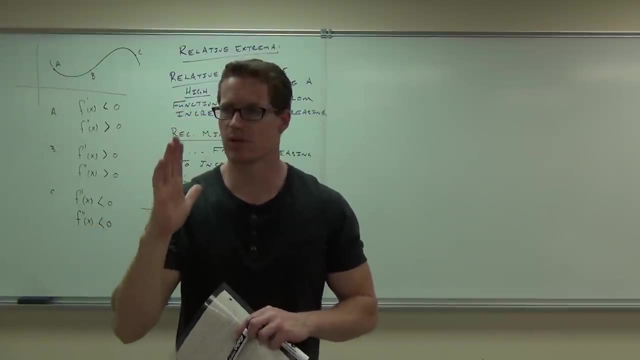 Well, what happens at a change from increasing to decreasing? What does the slope automatically have to do with that? It has to do if we're going from increasing to decreasing. At some point between a plus slope and a minus slope you have to hit what number. 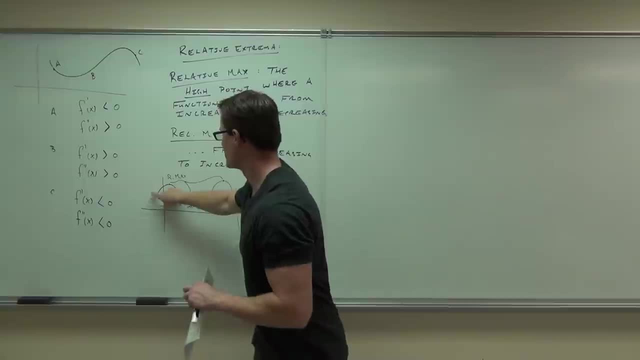 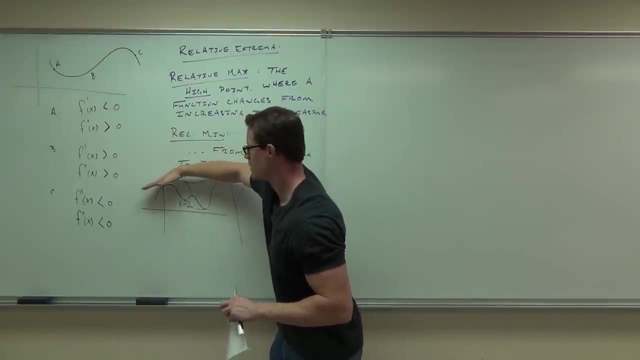 Zero. You have to hit a zero. So what's happening to the slope as I'm getting to a relative max, as I'm getting to a relative min max, min max. what's happening to the slope at those points? Positive, increasing zero. 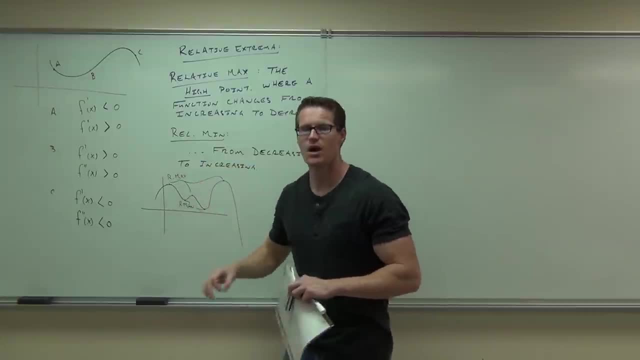 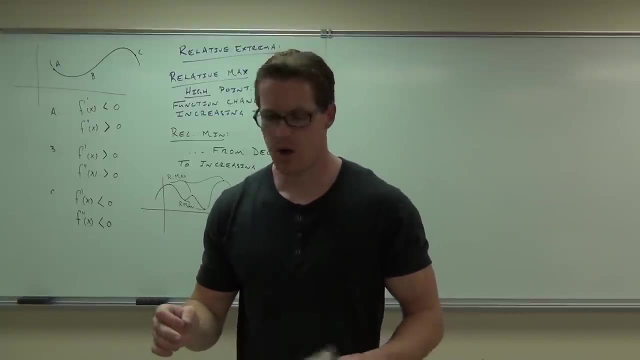 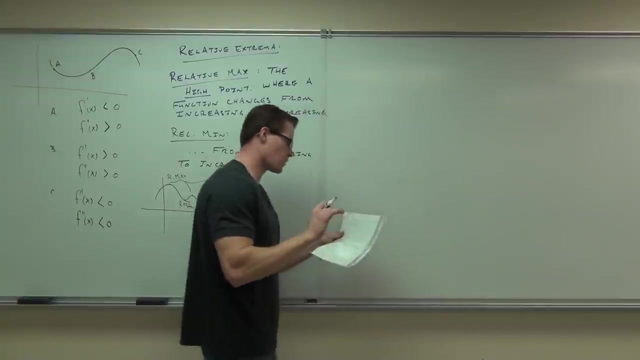 Negative, decreasing zero, Increasing zero, decreasing zero. So everywhere where we get a slope of zero, we're gonna have a possible relative max, relative min. But what we call those are critical numbers. So what's happening to the slope at a relative max or min? 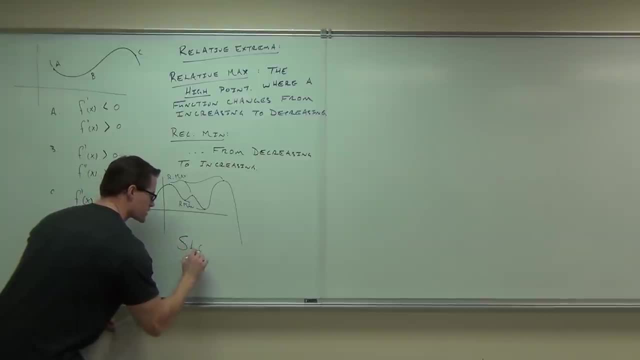 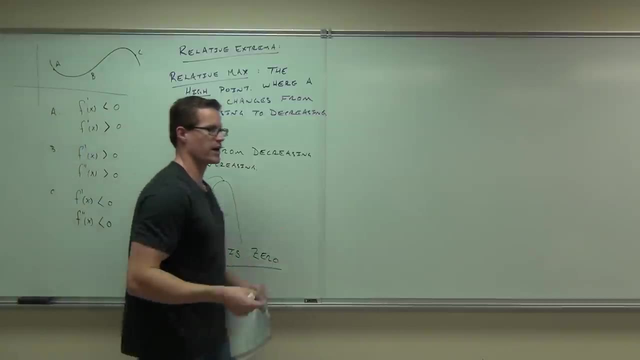 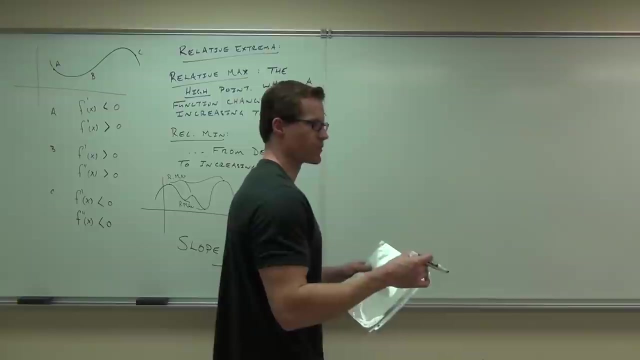 The slope is zero. So at all these points, note the slope is zero for the relative max, relative min. The point at which a curve has a horizontal tangent, or in other words the slope is zero, is called a critical number or a critical point. 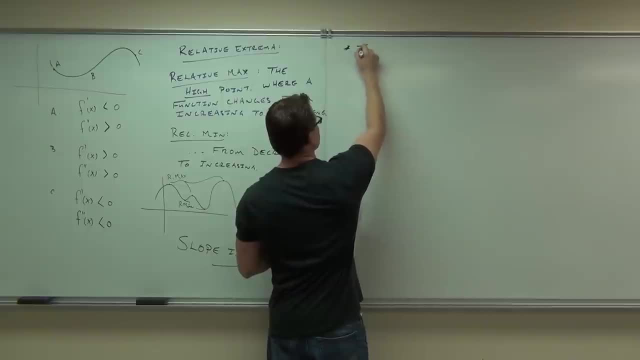 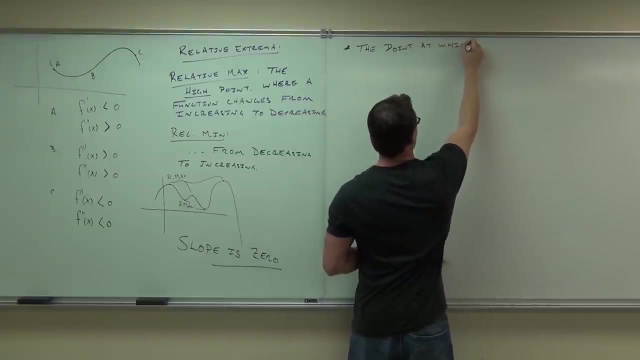 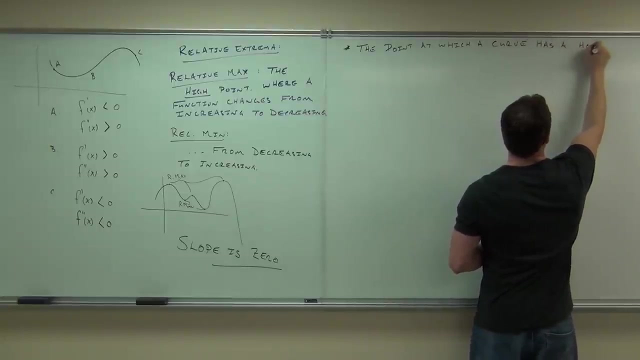 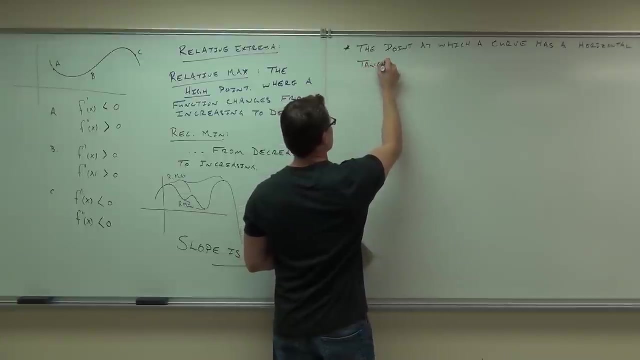 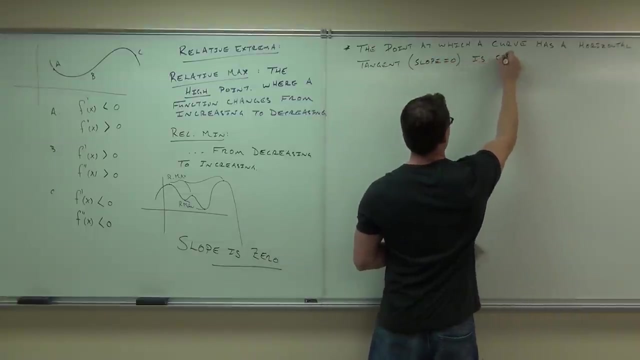 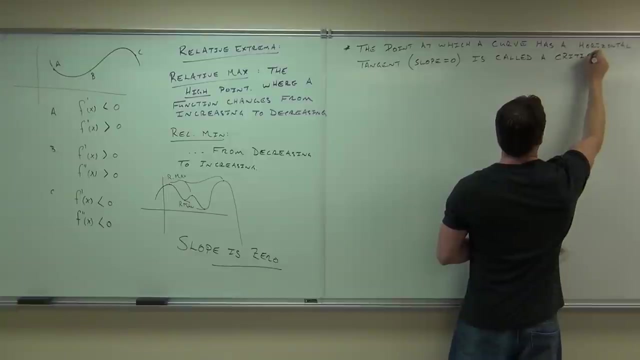 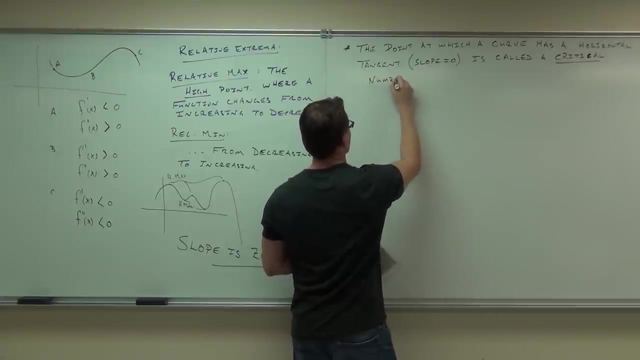 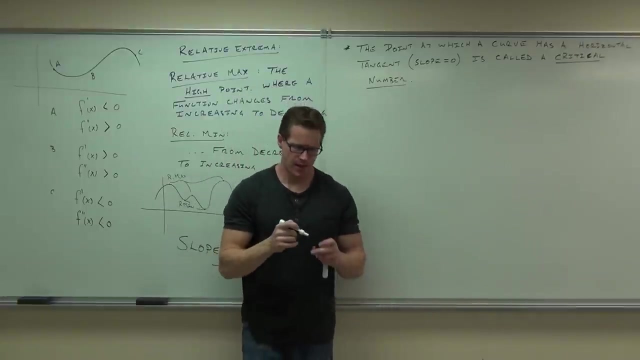 That's a little definition, Okay, All right. Okay, It's called a critical number, Okay, okay. well, let's think about this for a second. All right, If your critical number is a place where your slope equals zero. 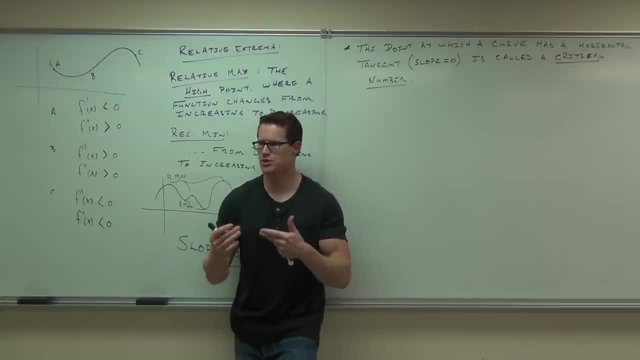 do you understand the definition, firstly, of a critical number? Critical number is a place where your slope equals zero. Are they always relative maximum ends? No, they're not. You can have other things that happen, So, for instance, this curve: 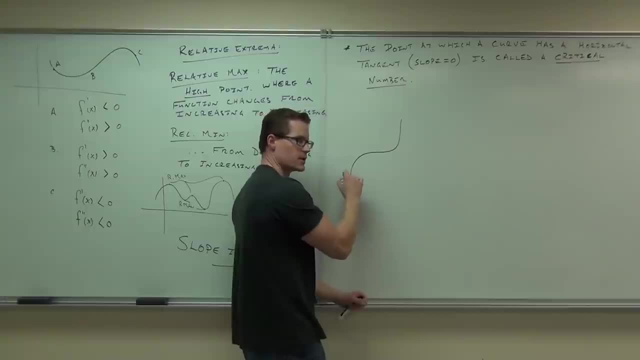 Do you have a point where the slope is zero? Yeah, but this is not changing. from increasing to decreasing, It goes from increasing to nothing to increasing again. Just a different concavity, Do you see it? So that could give you a relative maximum end. 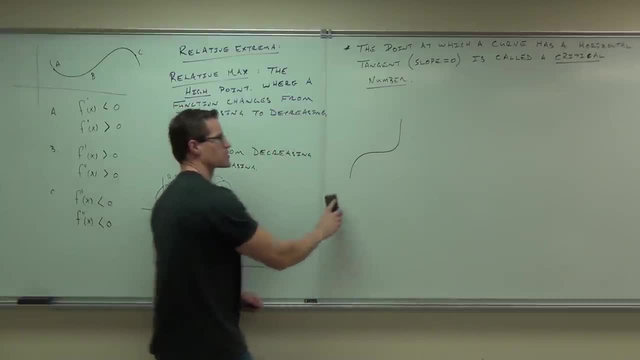 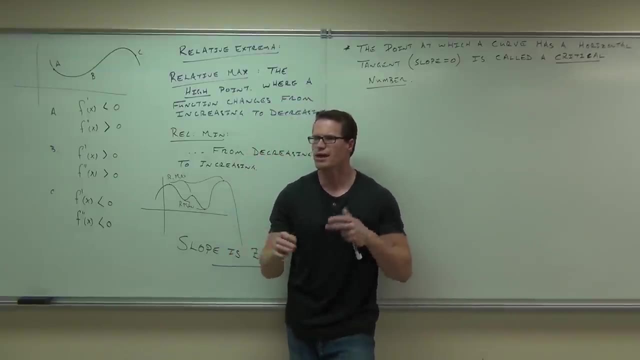 but it doesn't have to. That's the idea of a critical number. It's just a place where your slope is zero. So if we're trying to find out where all of our slopes are zero for a function, can you explain to me maybe the process of doing that? 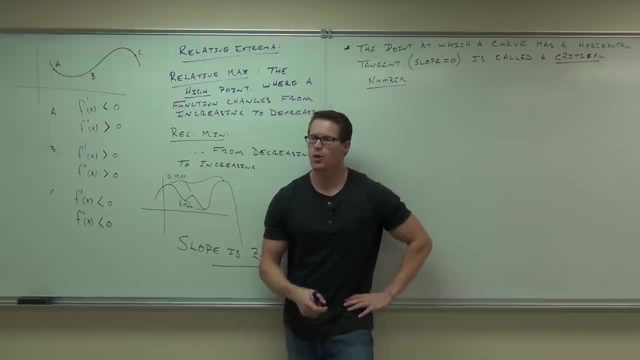 Let's pretend I give you a function and I say I want you to find the critical numbers. What might you have to do to find the critical numbers? Take the derivative and set it equal to zero. So the derivative gives you slope, true? 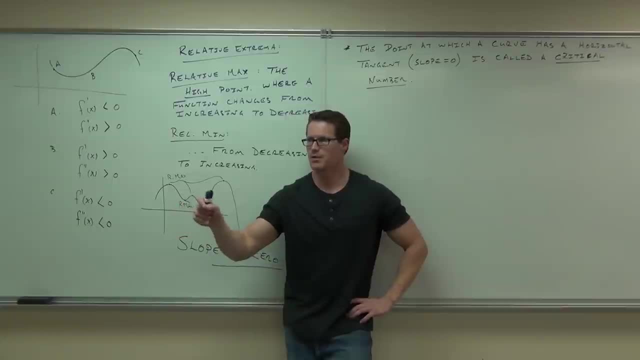 If I take the derivative and I set it equal to zero, I'm gonna find out all the places where my all the critical numbers, where my slope equals zero. Do you follow me on that? That's gonna give me all my potential relative maximum ends. that's the idea. 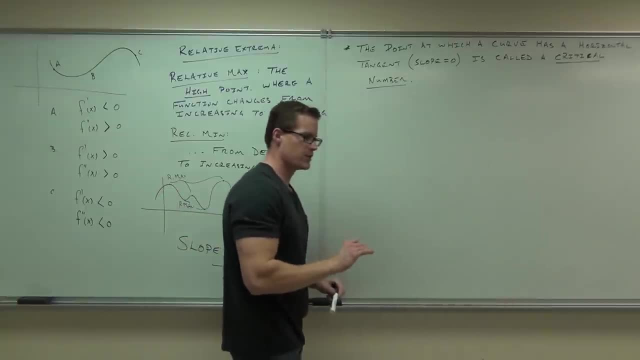 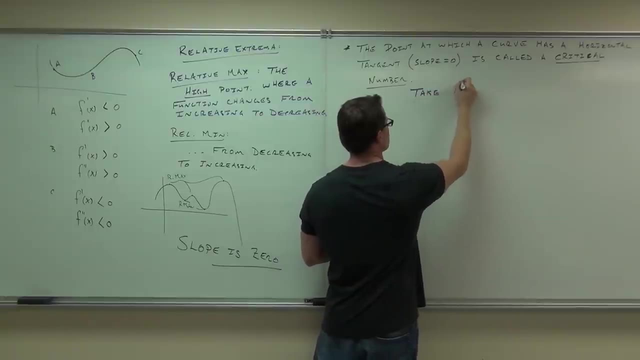 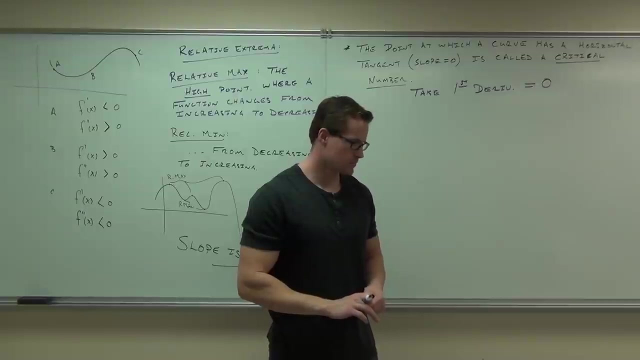 So to find a critical number, critical numbers, we're going to take the first derivative and set it equal to zero. Take the first derivative and set it equal to zero. You okay with that as well. One more side note: if you get a fraction, 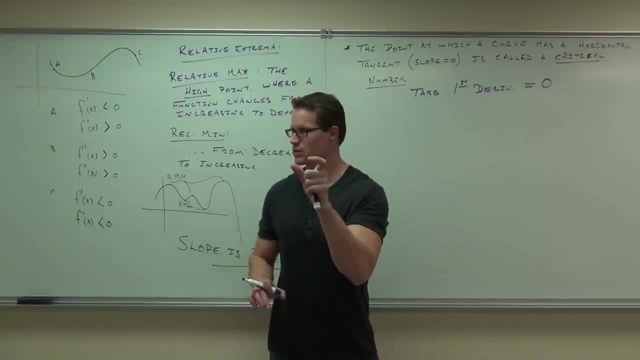 typically, all you have to do is solve for zero is to set the numerator equal to zero. right For this process. what we're gonna learn is that for both the first and second derivative- I'm gonna give you a first and second derivative test- 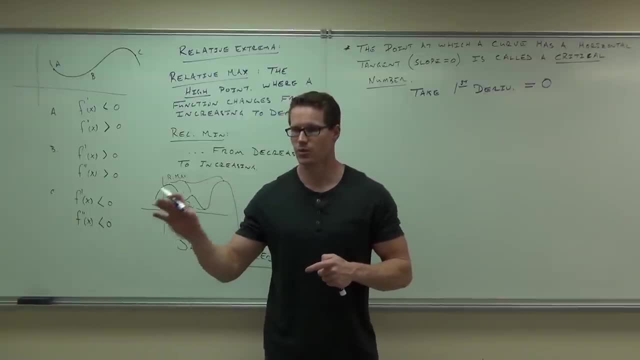 in a little while, like probably a week. But when you get there you also have to check the points where the denominator equals zero as well. So if you get a denominator, you must set that equal to zero as well, If that gives you undefined points for your slope. 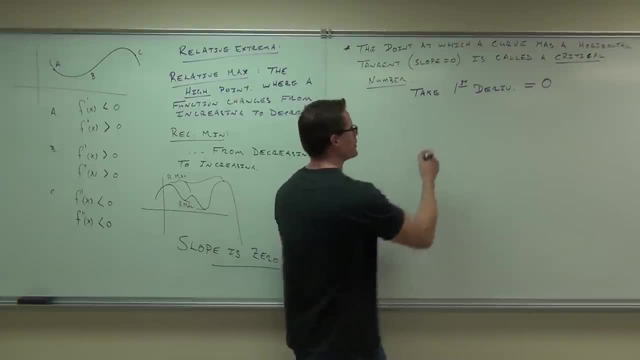 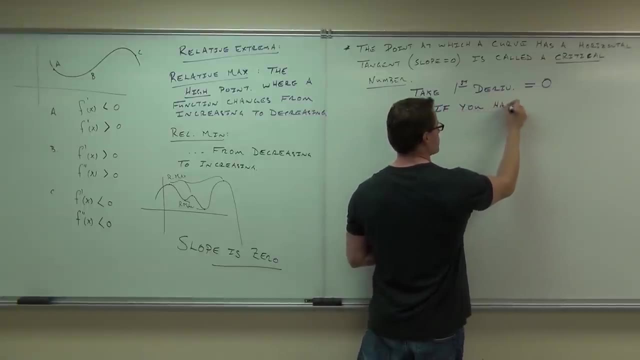 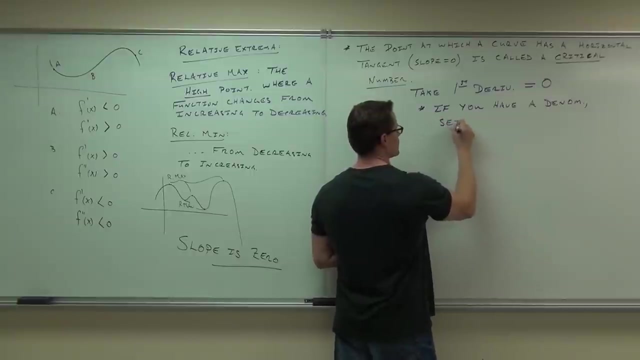 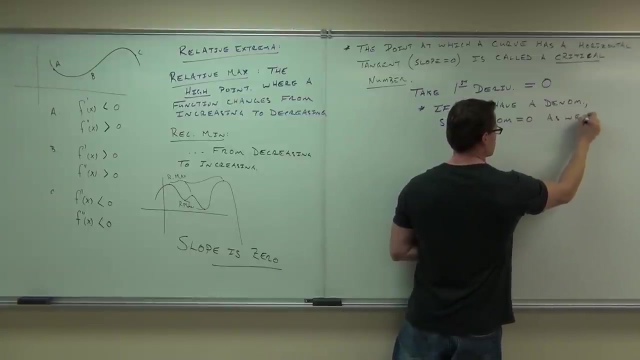 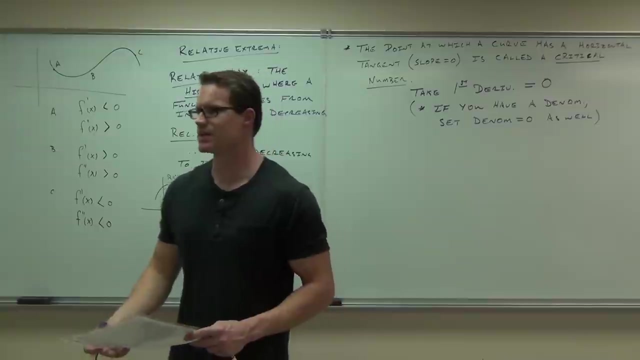 you need those. right. You need any undefined points for your slope. that's important, So little note. if you have a denominator, set the denominator equal to zero as well, That could give you any undefined points for your slope, which would be a big deal. 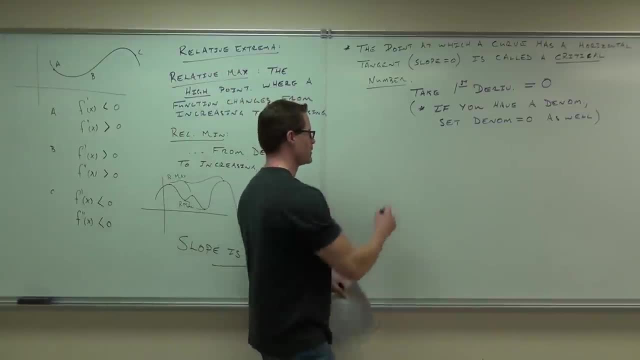 You can change from increase and decrease to undefined points. let me prove that to you. Increase and true Decrease, and, yes, Slope is undefined. You're gonna change from increase and decrease at that point, Even though it's not differentiable. 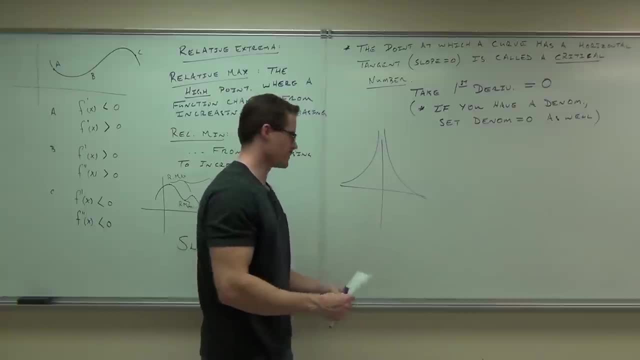 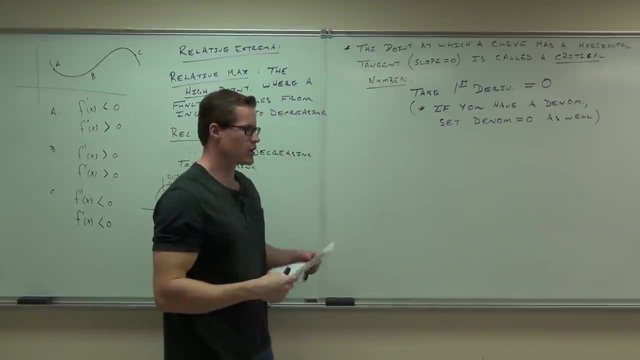 that gives you a point of change, of increase and decrease. Do you see what I'm talking about? So, denominator in the first derivative. In the first derivative, You set it equal to zero. Yes, Okay, The denominator of the original function will just tell you where you're undefined. 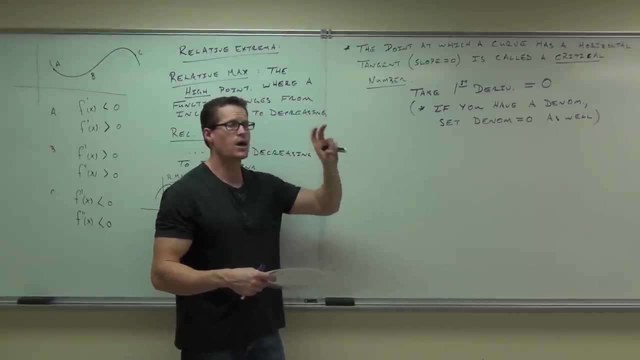 A lot of times that will match up okay. Where you're undefined in the function is where you will be undefined for your slope. Most of the time that happens, but occasionally you get some weird stuff that happens, So you need to do both. 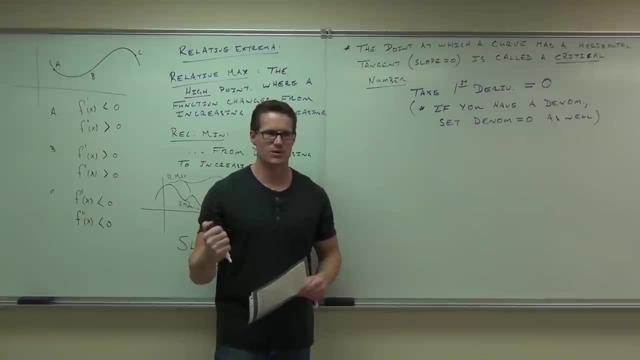 Can we do an example, to finally get away from all this theory stuff and really get into an example? Can we do that, please? Are you guys ready for it? Yeah, All right, let's go ahead. let's find the critical numbers. 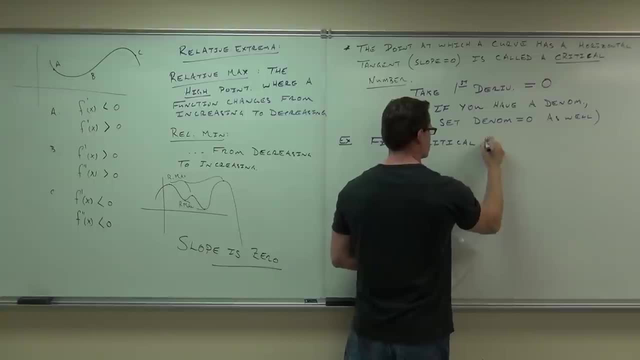 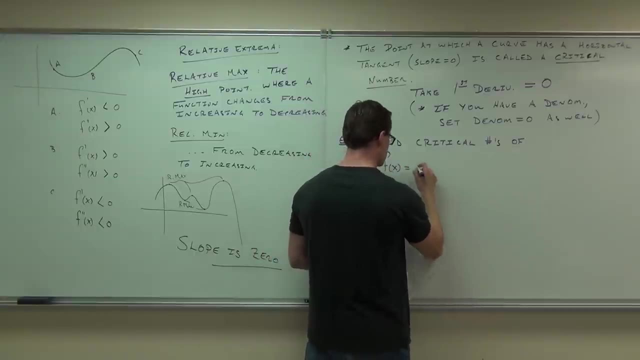 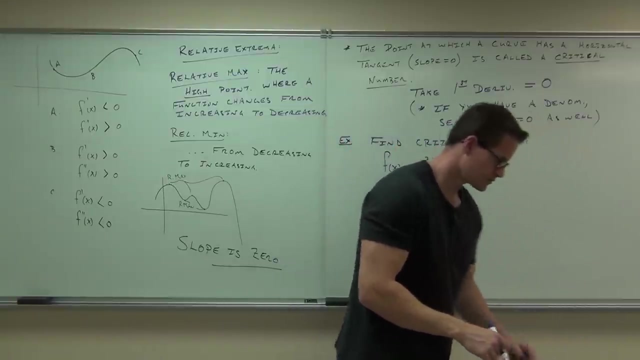 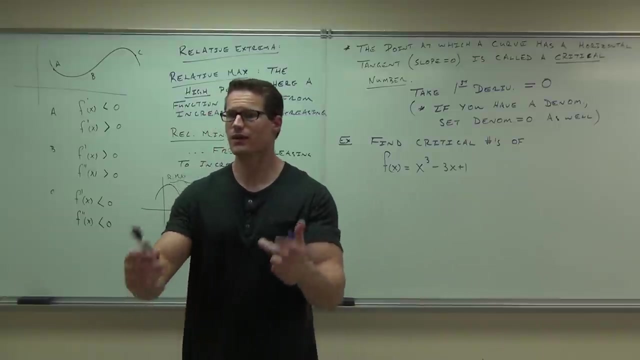 This: Find the critical numbers of that thing. What are we gonna have to do to find the critical numbers? Well, critical numbers involve slope, right. It asks where's the slope equal zero. So find the slope function. right now. That means take a derivative. 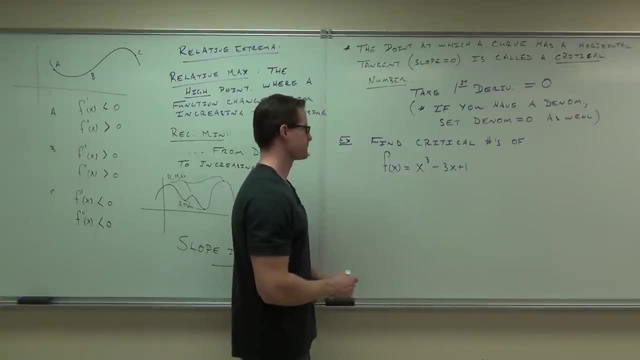 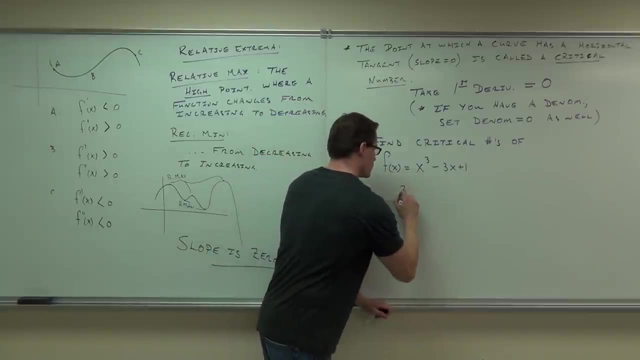 Go ahead, take a derivative. Derivatives should be pretty easy. What's the derivative of this thing? Man, I'm a nice guy, Don't you see? I'm a nice guy, I'm a nice guy, That's nice. 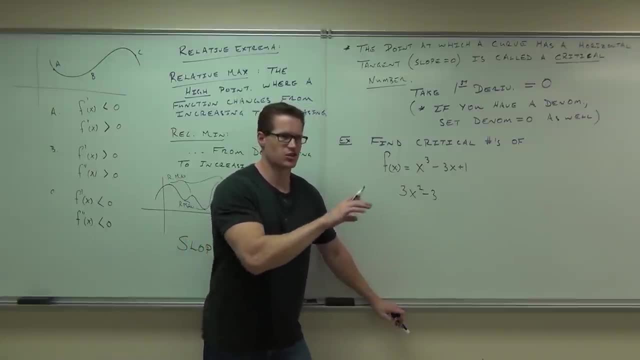 That's nice. Why? Why is that nice? What are you gonna have to do? That just gives you the slope right Because you just found the derivative. Derivative means slope. Our critical numbers occur where our slope equals. what? Zero. 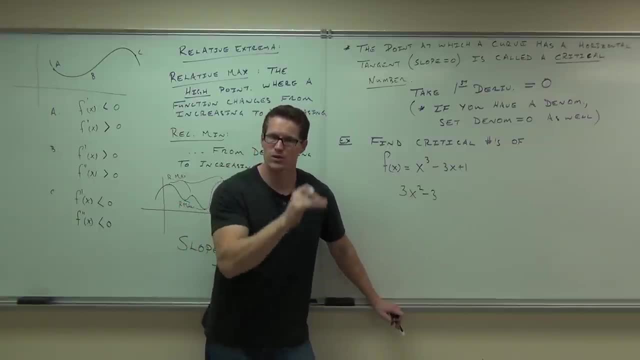 Set equal to zero, Solve it. That's gonna give you the x values where your slope equals zero. Can you solve that? Yeah, that's like a piece of cake to solve. What are you gonna do? That's why I'm a nice guy. 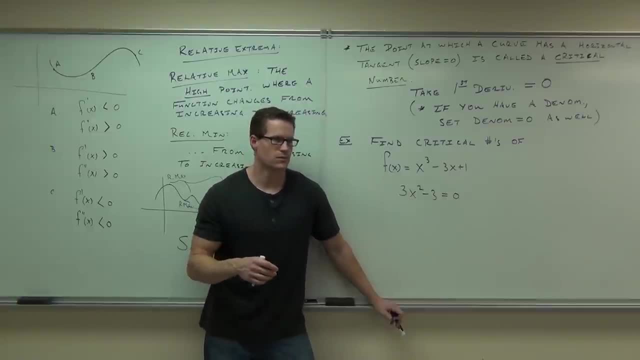 You have options. really: Add three, divide by three Square root with a plus and minus. That's gonna give you plus and minus one. Factor out the three different squares: plus and minus one. either way. You can do that two ways okay. 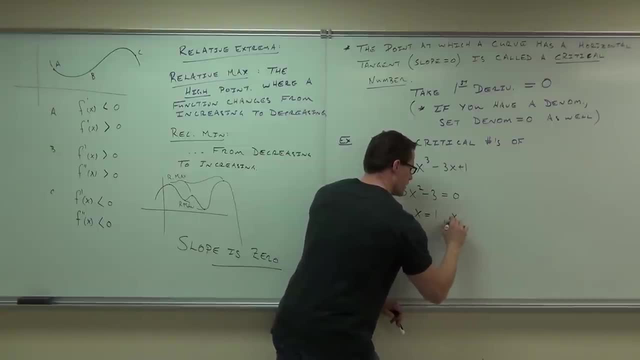 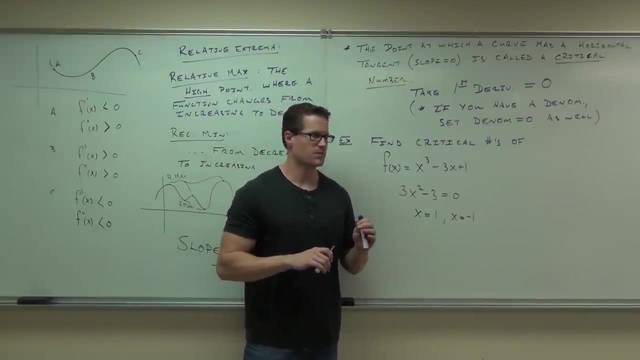 So in either case, here x equals one, x equals negative one. Are those my points for my relative max and relative min? Those are my x values of my potential points for relative max and relative min. Are these in this case yes? 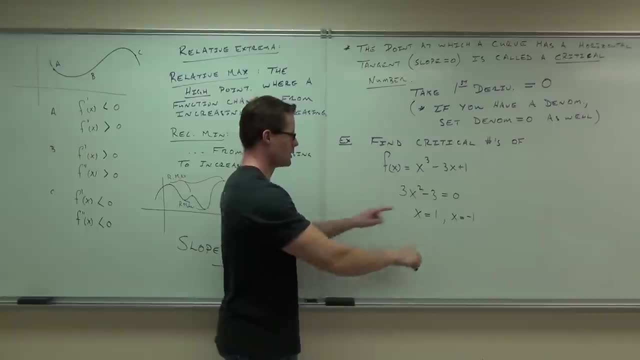 This is gonna be a relative max and a relative min. This one should go max- min. Okay, that's what that should be. Now, we're gonna talk all about that later. Right now, I'm just asking you to find critical numbers. 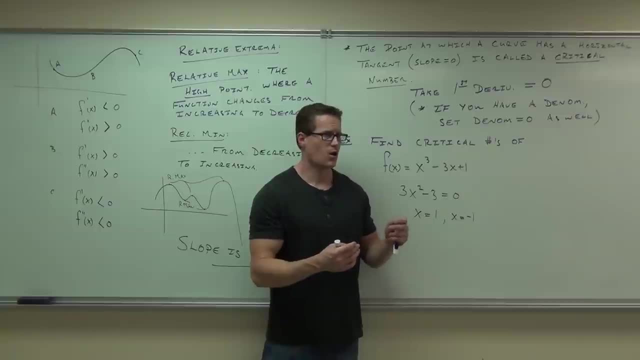 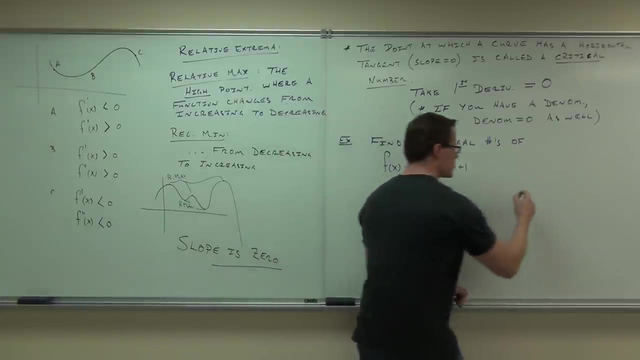 I'll show you how to determine that at a later time. Are you all right with that? Are these always giving you the same number? Are these always giving you relative max and relative min? The answer is no, no, they're not. I've given you one example of that already. 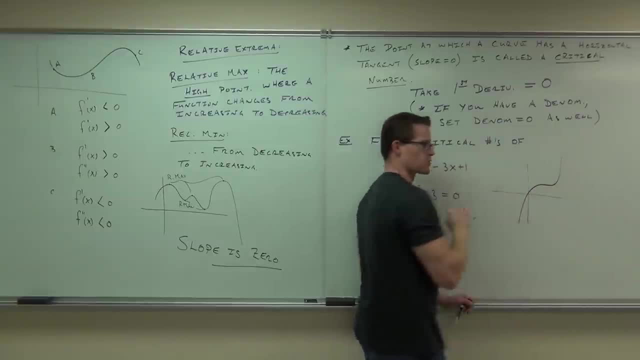 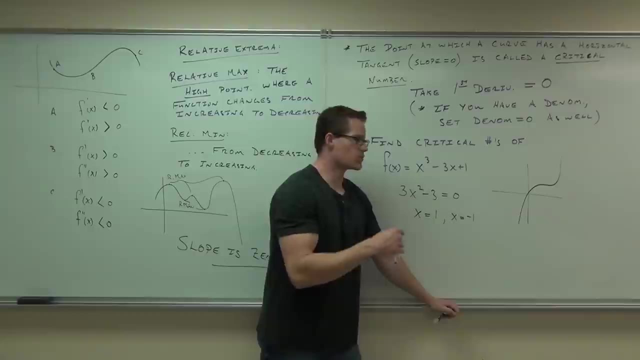 This right here is gonna show up as a critical number. Is it automatically a relative max or relative min? No, no, there's some cases where it's not okay, So you really do have to check on those. I'll show you how to check on them later. 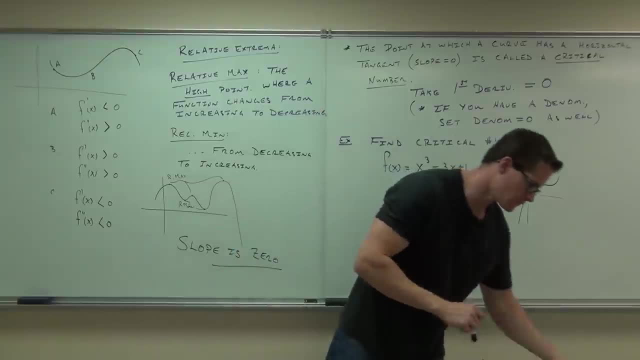 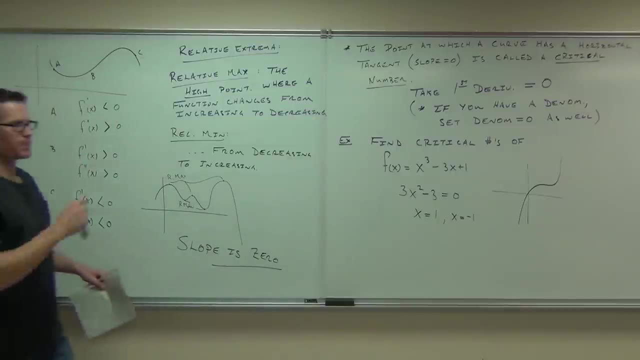 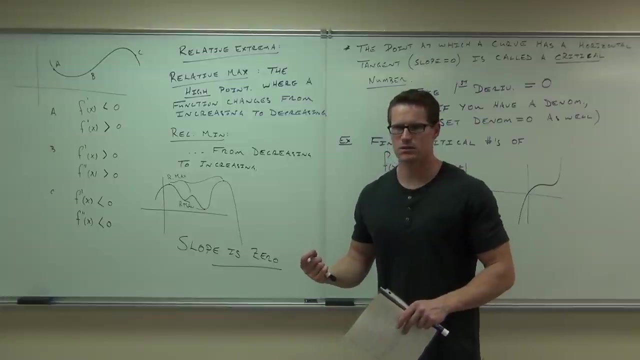 but they're not automatically relative max or relative min. We're gonna switch gears just a little bit. We're gonna move from relative max and min to absolute max and min. Now, what's absolute mean? A high absolute value, Yeah, absolute value would be like positive, always positive. 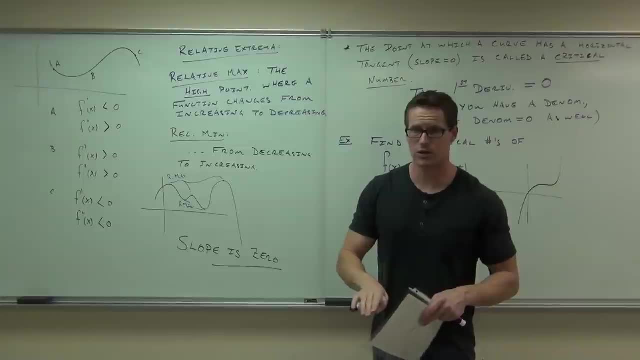 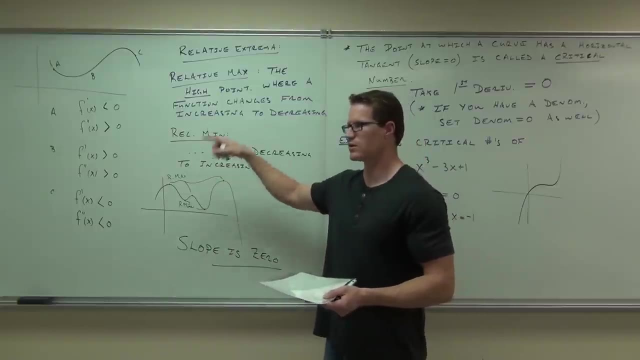 But absolute means it's the most high or the most low Relative. you're noticing this? we can have lots of relative maxes right. Think about a sine curve. Oh my gosh, there's relative maxes all over that thing. 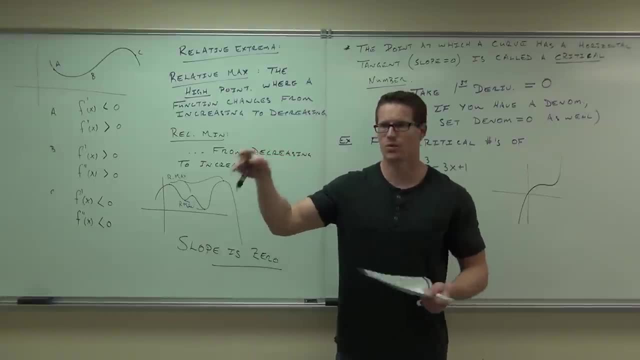 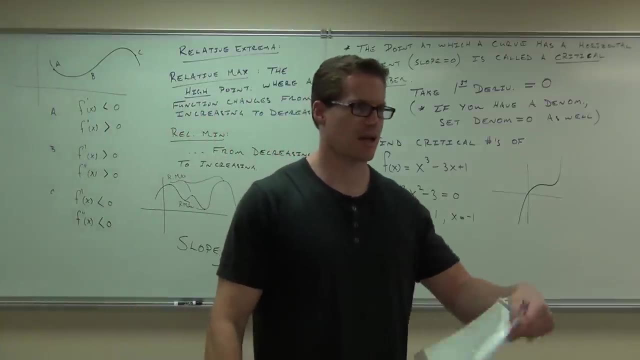 Those all happen to be the absolute max for a sine curve, but they're all relative maxes as well. For the absolute max it says what's the highest number you attain, if any Relative absolute max and absolute min means what's the highest or? 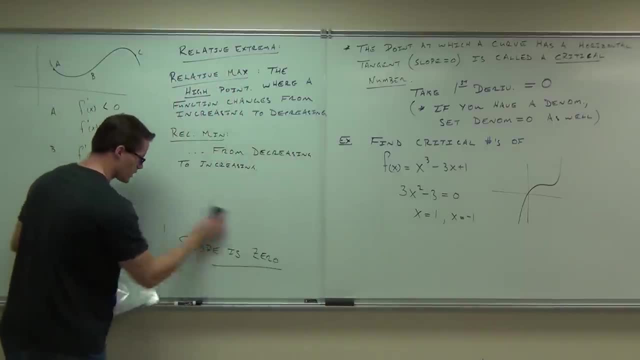 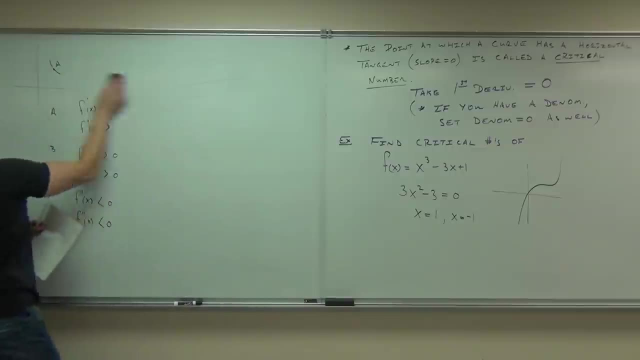 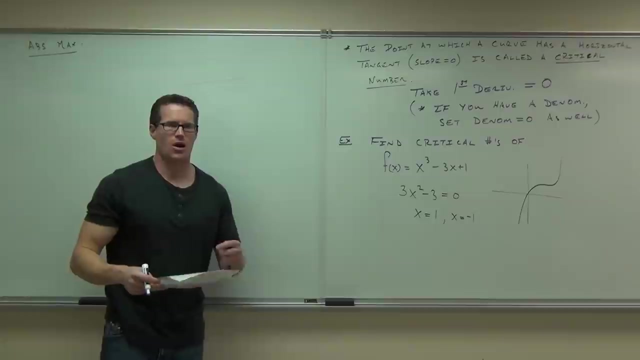 lowest value attained throughout the whole. So we'll talk about that. We'll talk about how to determine it. It's not bad, so don't let it scare you. So when we talk about the absolute max, what we mean is the highest point on an interval overall. 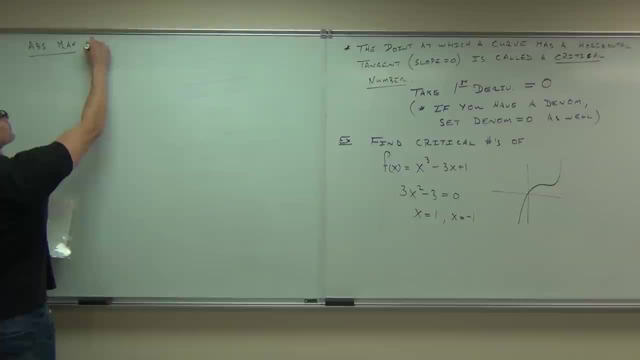 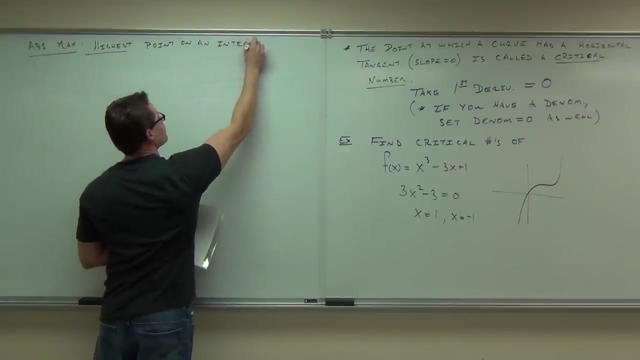 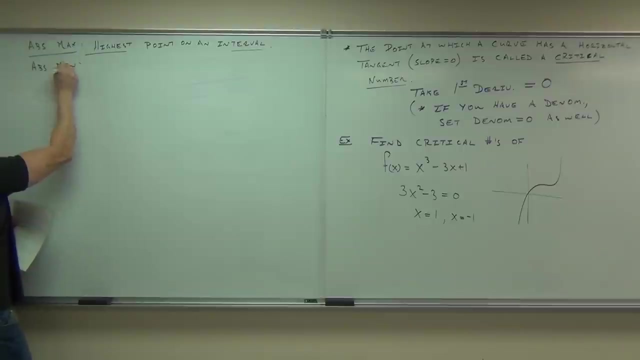 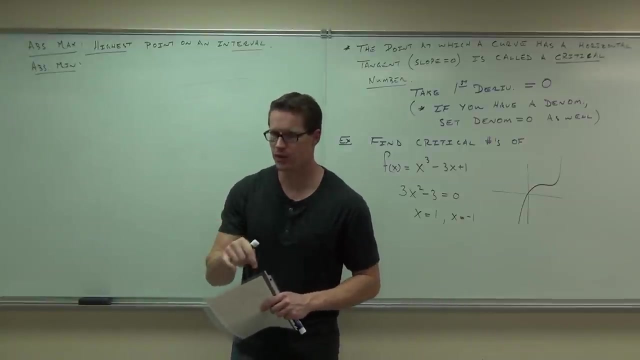 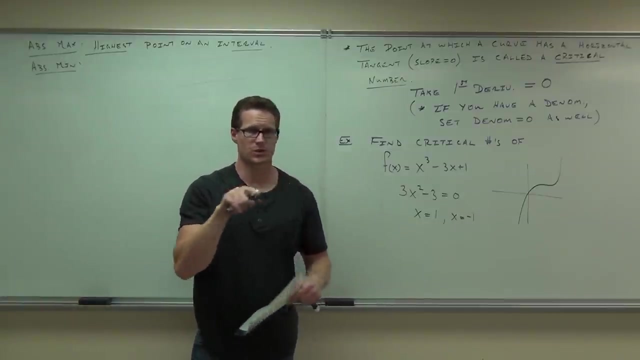 the highest point that happens on that interval. Well then, that would mean the absolute min means the lowest point on an interval as well, Not one of the low points, the lowest. That's how that differentiates from the relative Relative could be. well, there's a few low points. 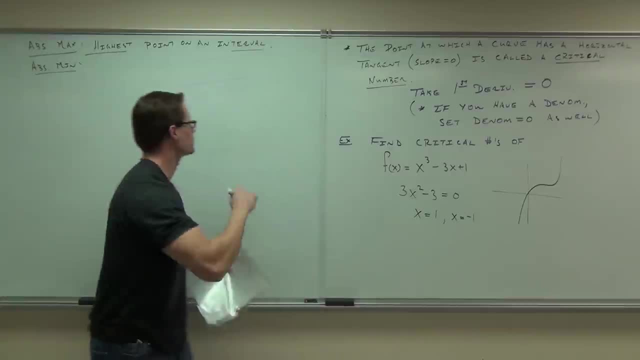 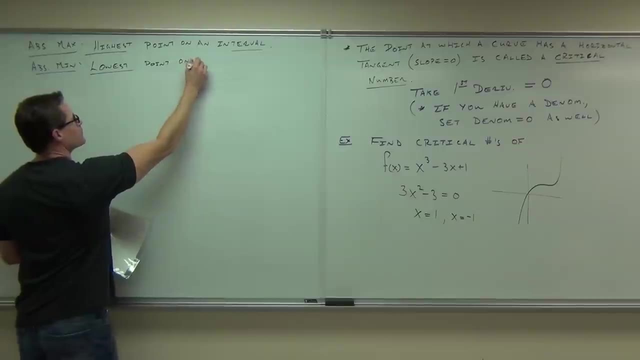 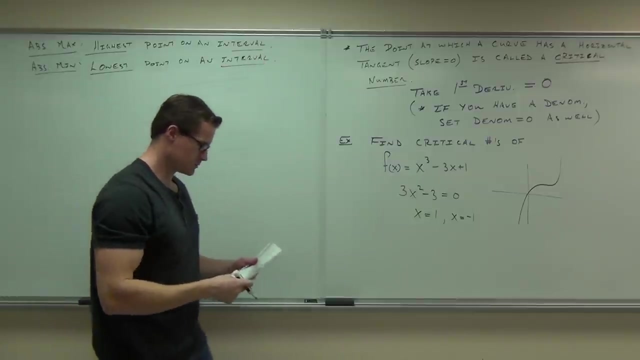 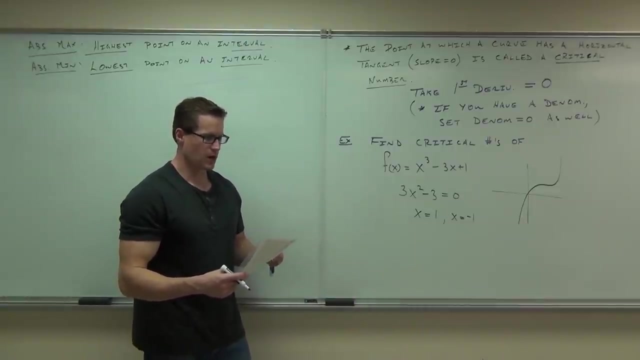 Absolute minimum means the lowest, Absolute max means the highest. Is that on an interval or on the function On an interval? Now, the interval could be from negative infinity to infinity, But a lot of graphs don't have an absolute max for min on negative infinity to infinity. 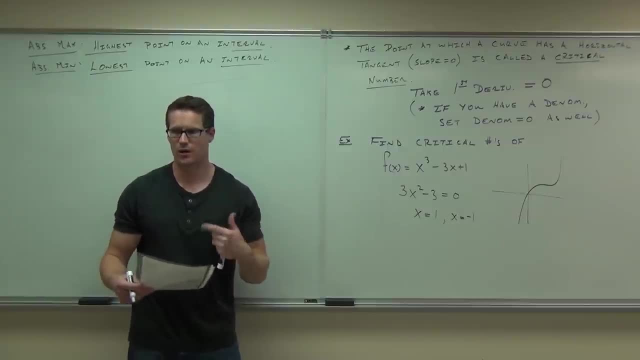 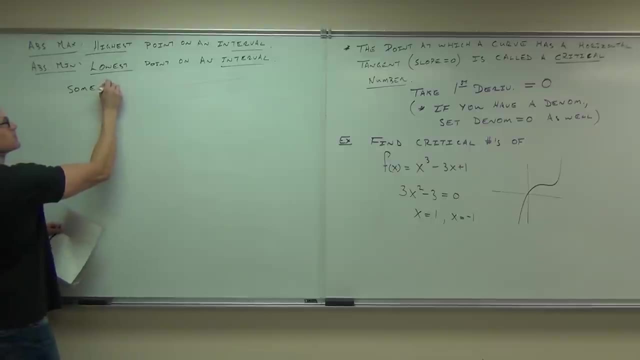 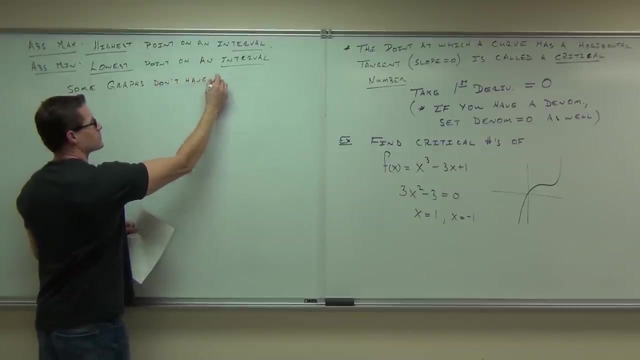 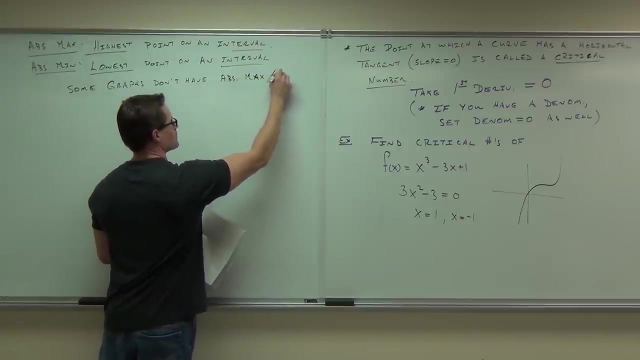 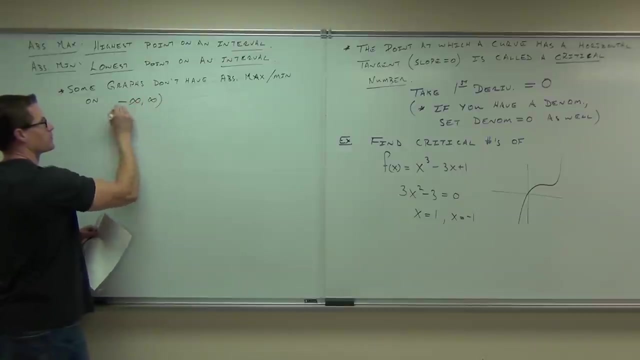 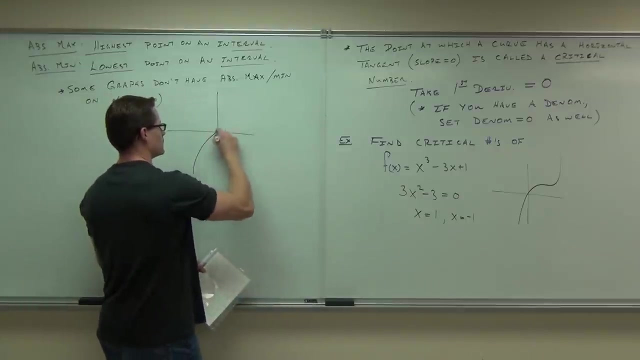 In fact lots of polynomials don't. So we talk about on intervals as well. So some graphs don't have absolute max or min On this interval. for instance, just think of an x cubed. OK, What's the highest point that obtains? 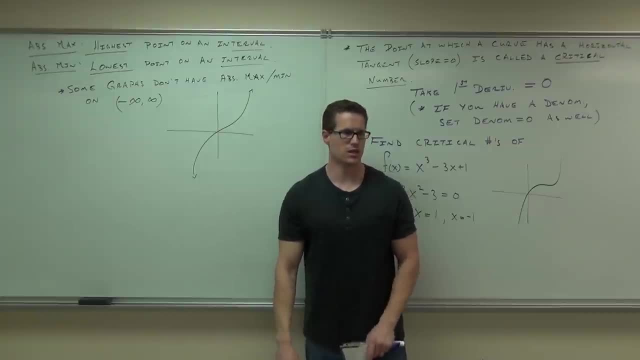 So it. Can you say the number? Does it reach a peak Ever? Do you know how much infinity is? Because I do. No, I don't. No, it's infinity. It never reaches an ending point, does it? 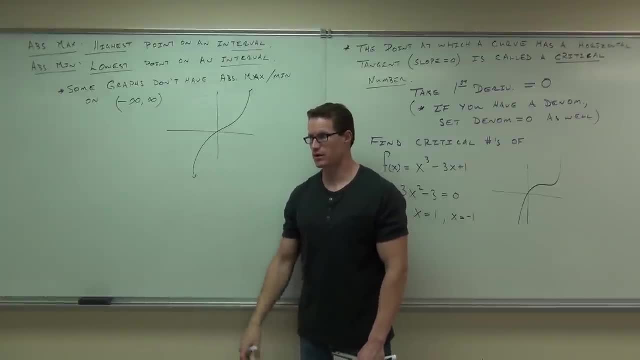 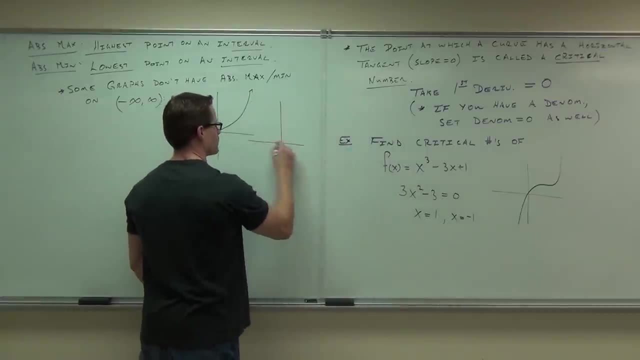 It doesn't reach a highest point. It keeps going and going and going and going. Does it ever have a low point? The lowest point? No, this doesn't have an absolute max or an absolute min. How about this one? Does that have an absolute max? 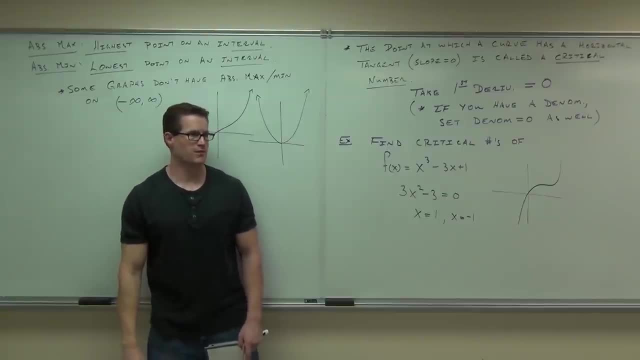 Max? No. Does it ever reach the highest point? No, No, it's infinity. Does it have an absolute min? Yes, It's right there, That's 0, 0.. That does have one, But you'll see that some curves don't have the absolute max or min on negative infinity. 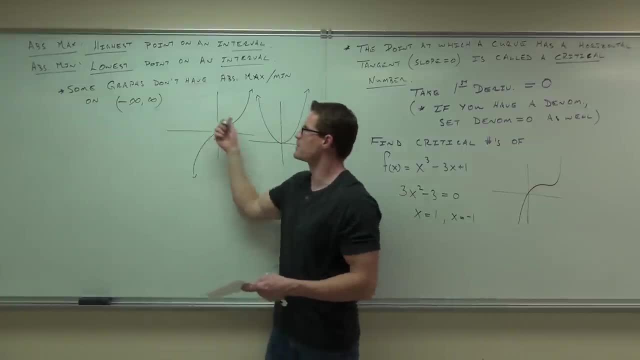 to infinity. Some do, Most don't. Every polynomial doesn't have it has one or the other, because polynomials go to infinity somewhere or another right They're never horizontally asymptotic. So you know, it's not always the case. 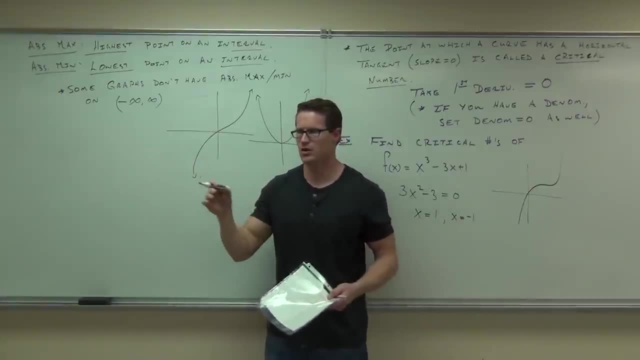 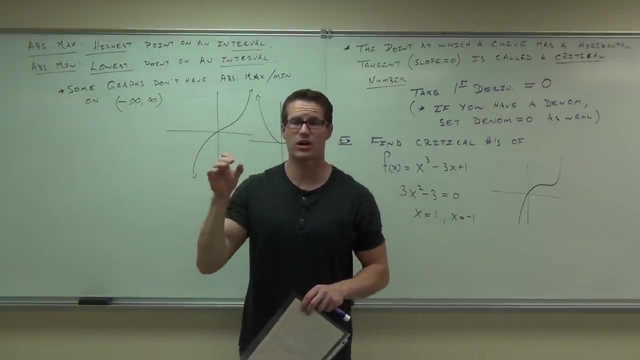 Yeah, they're never horizontally asymptotic, so you're always going to get one. So we like to distinguish between everywhere and then certain intervals. So an absolute max is going to be the highest point on an interval that you say it is. 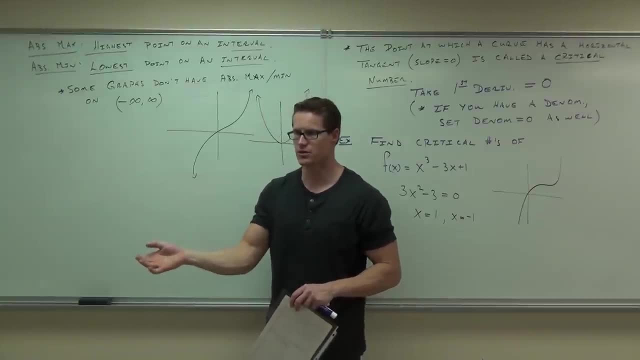 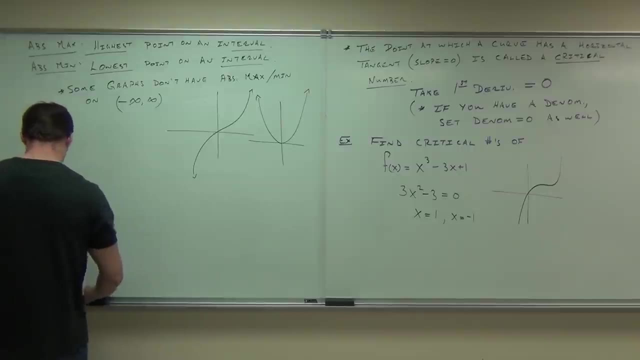 And the absolute min is going to be the lowest point on an interval that is defined for you or that you say it is. Do you follow that, that logic there? Okay, Okay, don't have an absolute max or an absolute min on this. 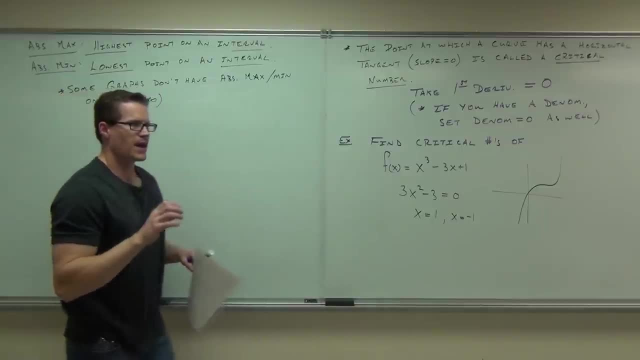 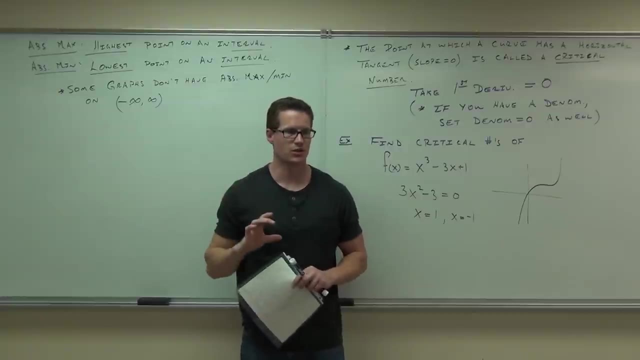 Let me make a little suggestion to you. I'm going to suggest that every curve in the world has an absolute max and an absolute min on a closed interval. Would you agree with that? On a closed interval, so if I say from 3 to 2,, 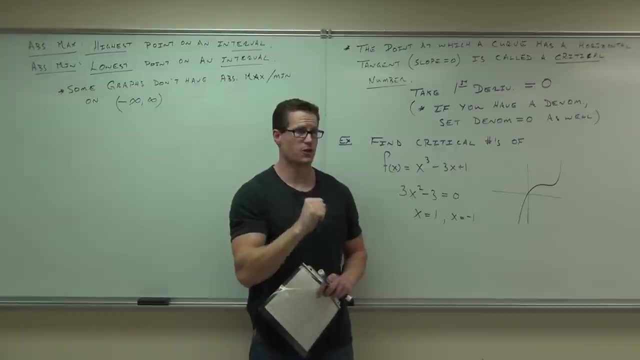 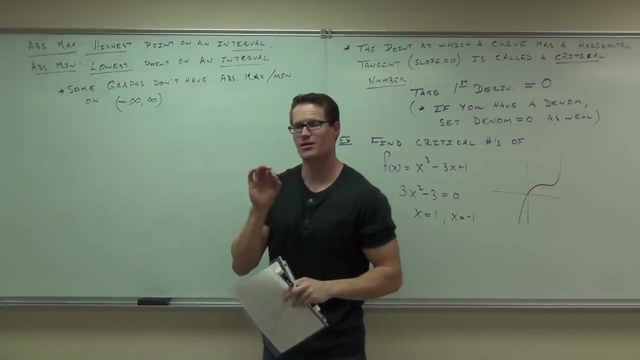 there's going to be a highest point, there's going to be a lowest point, as long as the function is continuous. Yes, We don't want this idea. That would not. But as long as it's continuous, that's going to happen. 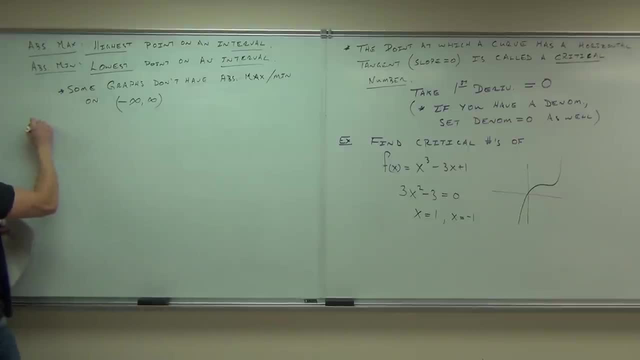 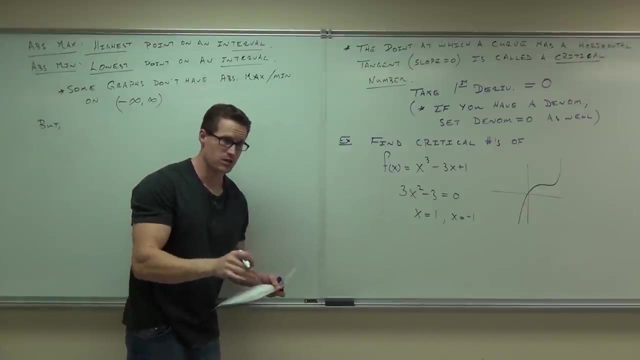 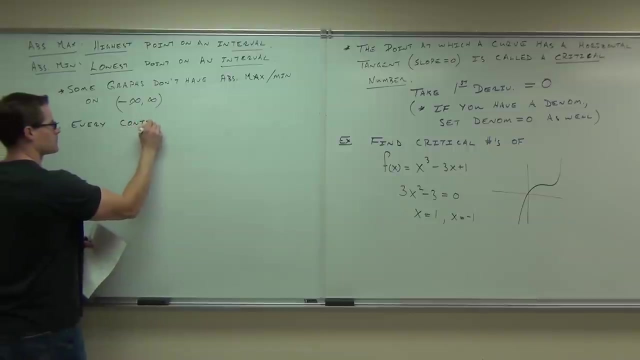 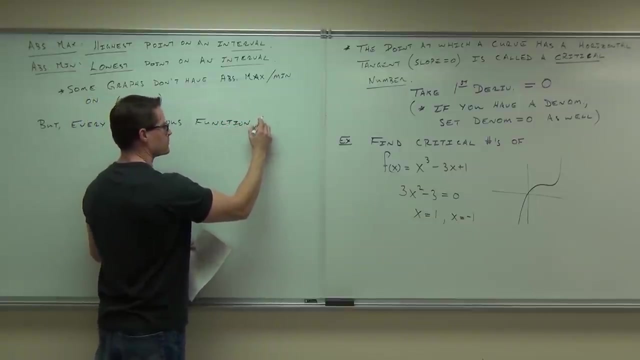 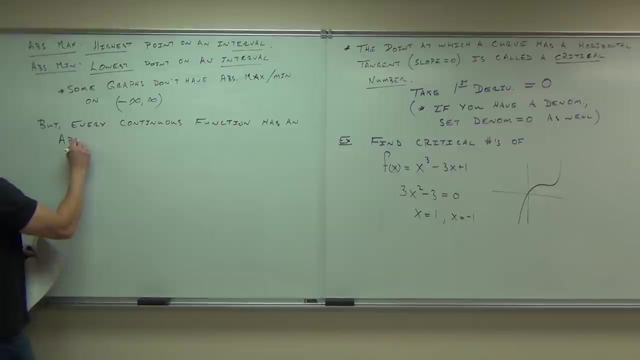 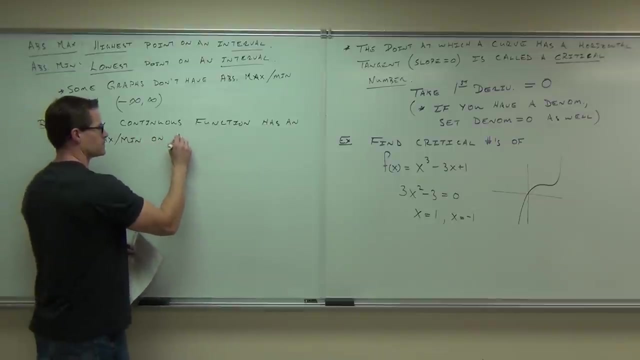 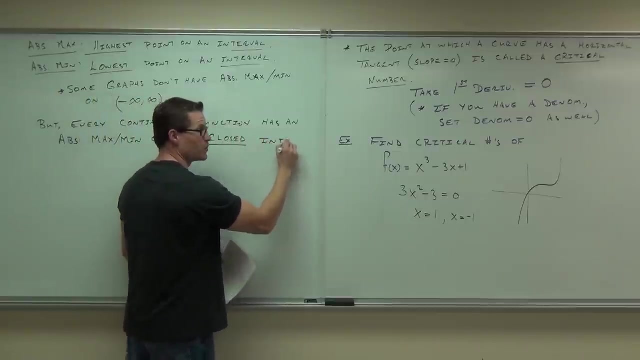 So this not so much. But every function has an absolute max and min. if the function is continuous on any closed curve- I swear you practice this so hard In front of your mirror- On any closed interval, Open interval, Not necessarily. 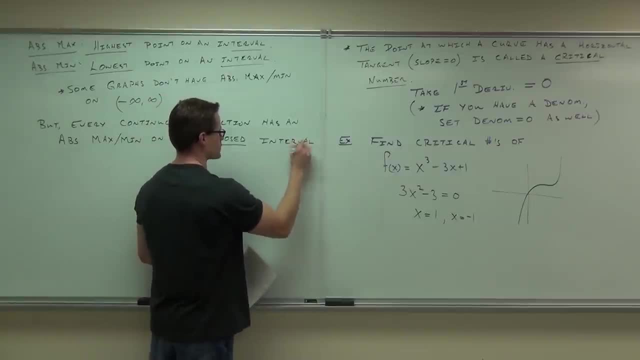 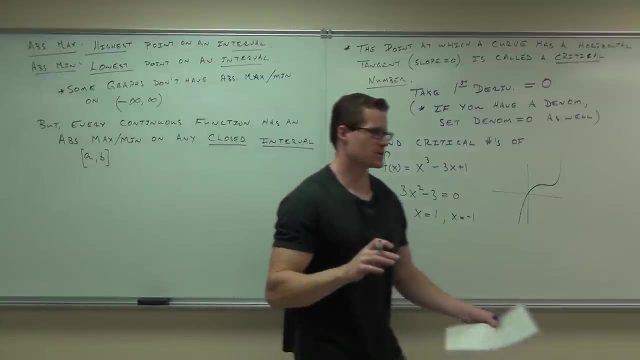 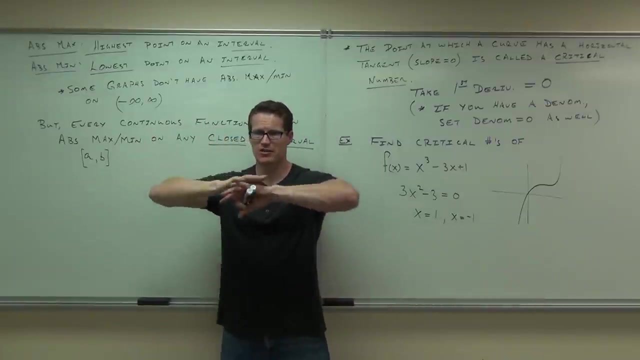 We'll talk about that in a bit. But closed interval: absolutely, yes. Okay, here's. let me talk about one little piece of information. you kind of need to know Every continuous function. what that means is the function doesn't have to be continuous for the entire space. 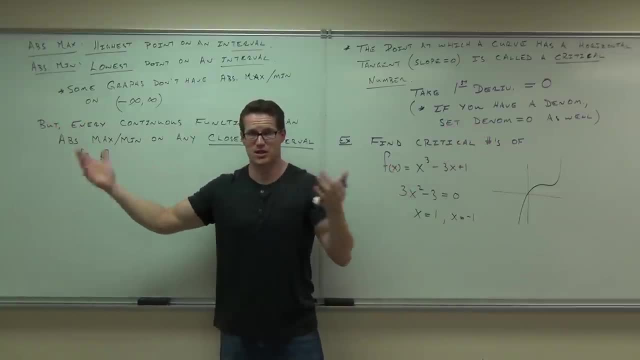 of human existence, what it has to, or x existence, I guess, whatever. but it has to be continuous on that closed interval. Does that make sense to you? It's got to be continuous here. If it's continuous there, it will certainly have an absolute max. 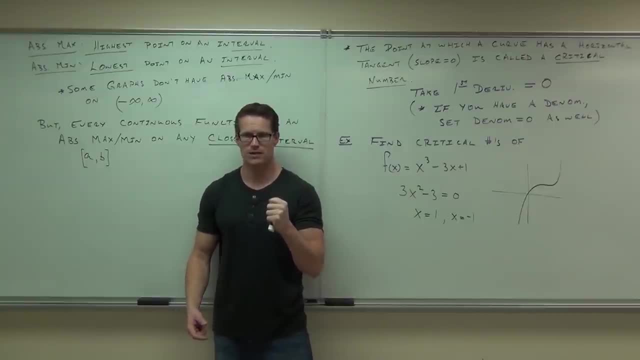 a highest point and an absolute min at the lowest point. Do you follow me on that? If it's continuous for this part, it'll be there. Now, where might it exist? Where might that happen? Well, there's only a set number of points. 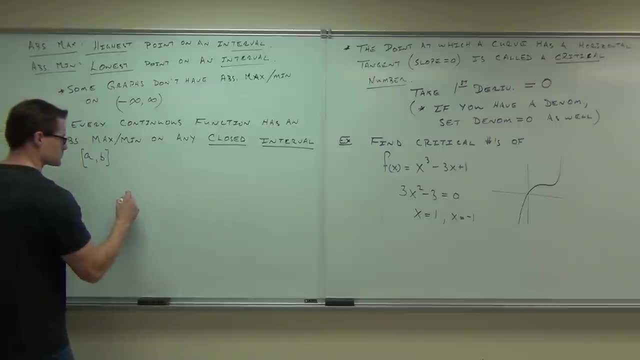 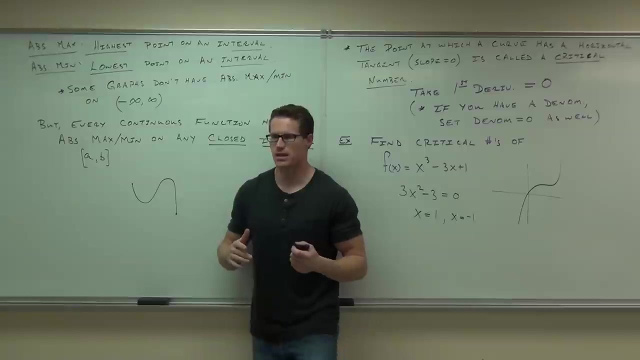 If you think about it, if you think about it, that's a closed curve, true, Closed curve. with my closed interval, Where could the absolute maxes and mins possibly occur? Well, they're either going to occur at a relative point. 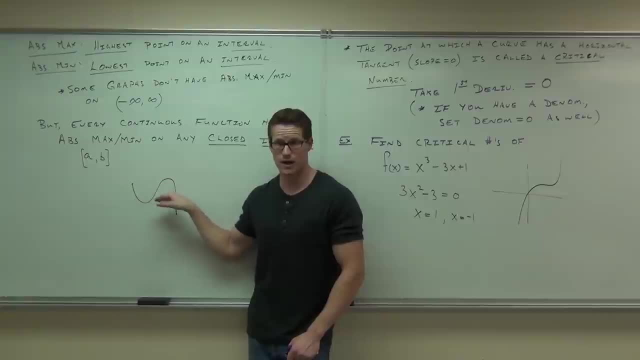 where I'm switching to the absolute max. I'm switching from decreasing to increasing or increasing to decreasing. It's going to happen either there or it's going to happen at the end point. There's only two cases: It's either switching from going up to going down. 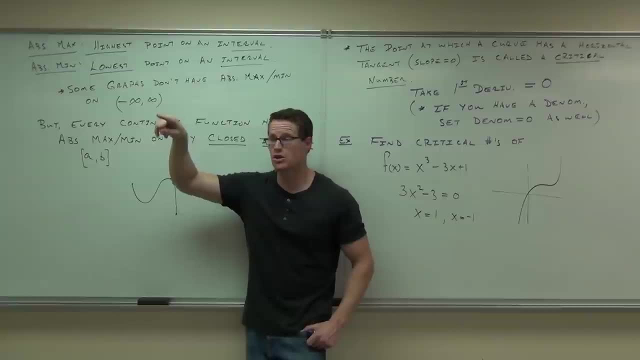 that gives us a low point or a high point, or it's at the end where I would continue to go up, but I just chop it off and I go. no, you stop there. ha ha, ha, ha ha. 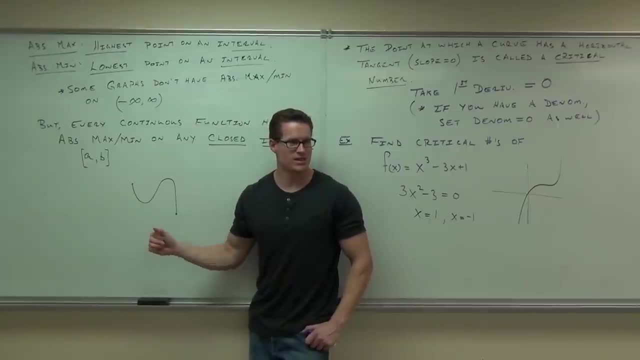 And then it has to occur there. Does that make sense to you? So it's either got to be at an end point or at a relative max or min. That means a critical number. So what's going to happen for your absolute max or min? 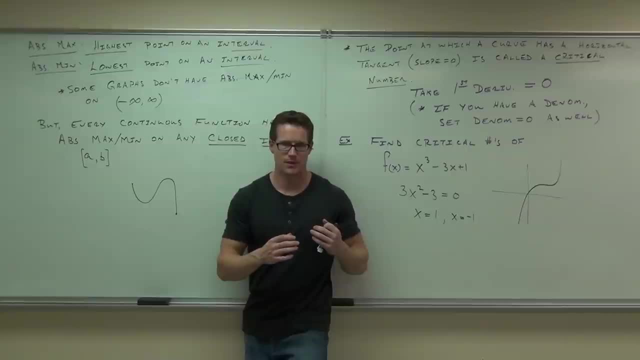 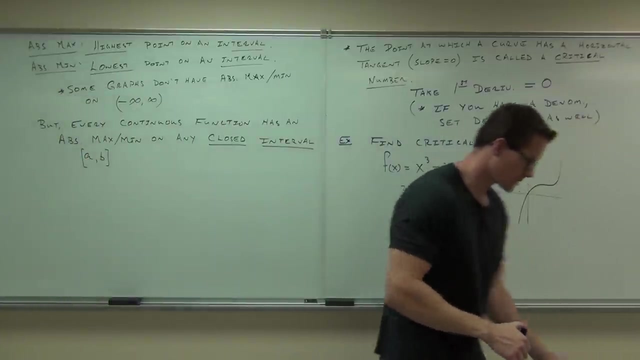 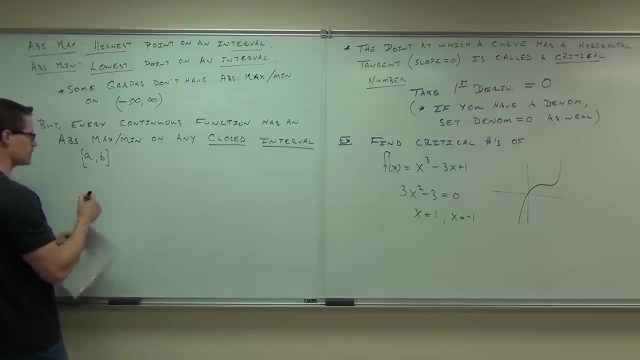 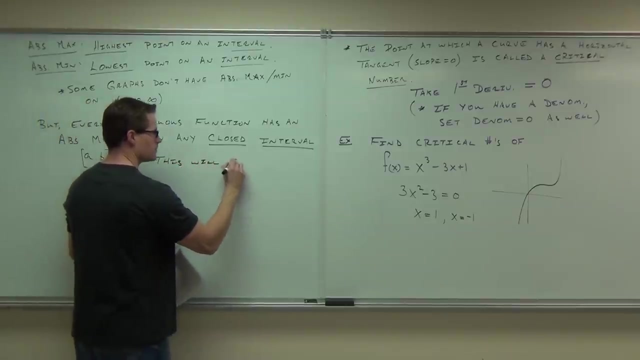 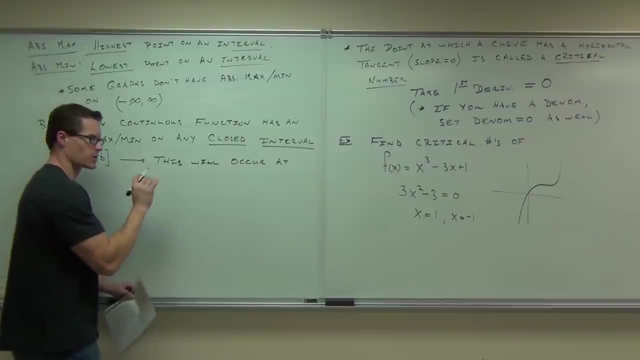 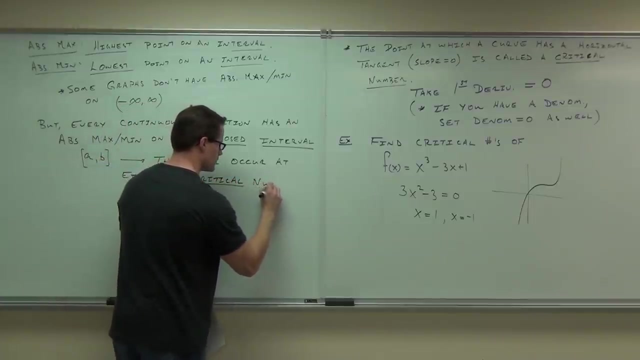 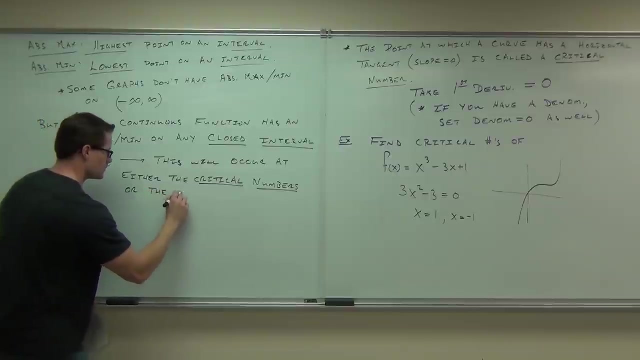 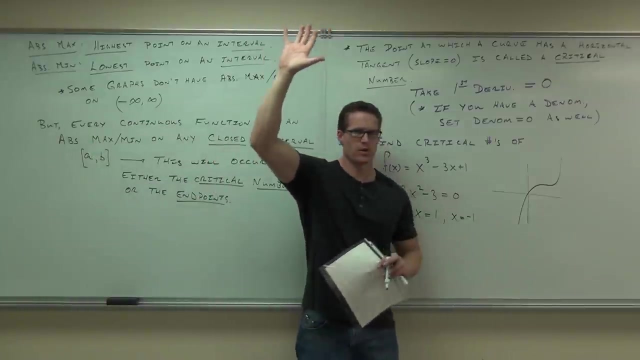 For any closed interval, it must take place at either a critical number or an end point. This will occur At either a critical number or the end point. Can you raise your hand? if you understand that logic, That it's going to be one of those two places? 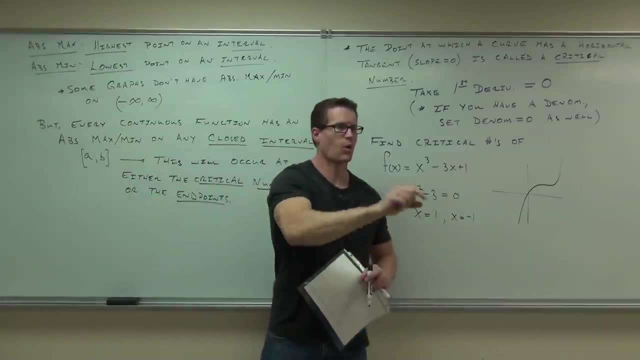 Either it's going to be where our function changes from going up to going down, going down to going up, or at one of the stopping points of our interval. Do you follow me on that? It's got to be one of those places. 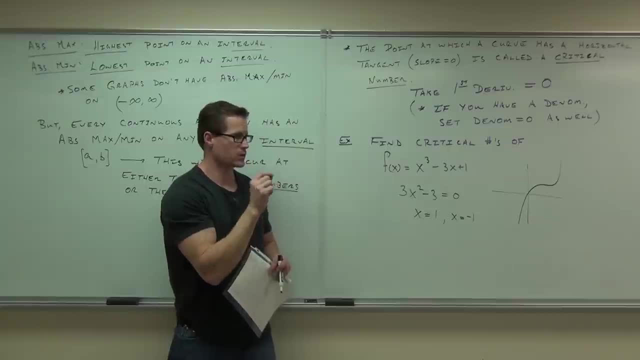 Which means there's only a few points you need to check. when you find an absolute max min, You're going to be checking your critical numbers by plugging them into your function, but you're also going to check your end points. We'll do some examples of that in just a second. 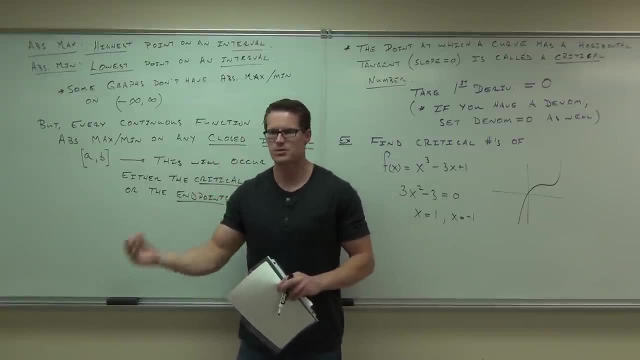 And whatever's the highest one, that's your absolute max. Whatever you're looking for, The lowest one, that's your absolute min. That's it. That's all we're going to have to do. This implies one more thing, though kind of like a corollary. 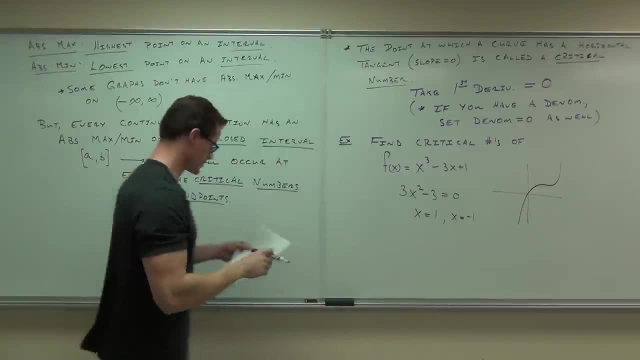 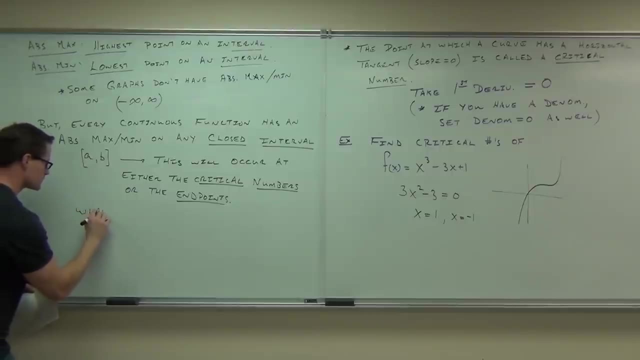 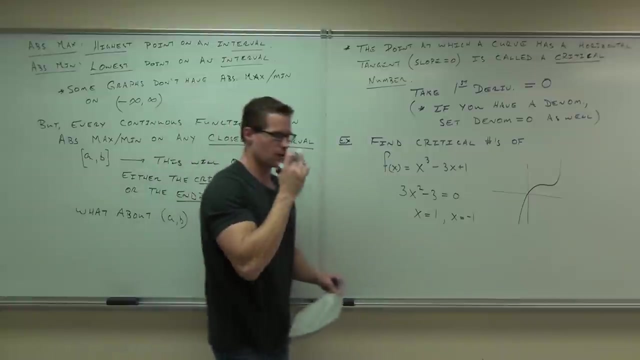 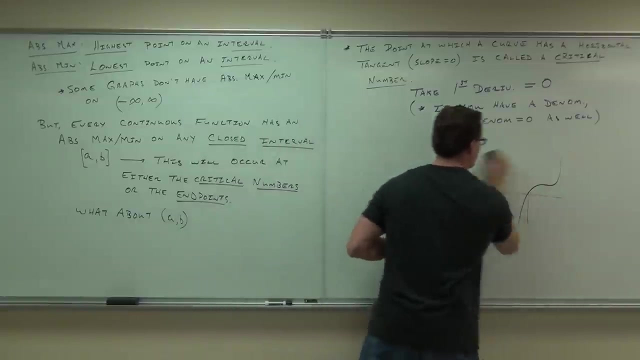 What if I don't have it closed? What if I have this? What if it opened? Think about this for a second. This is an interesting case. okay, Check it out Now. check out my erasing. Check out what I'm going to write after I erase. 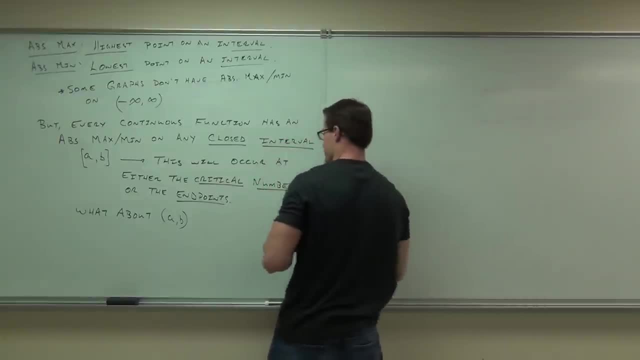 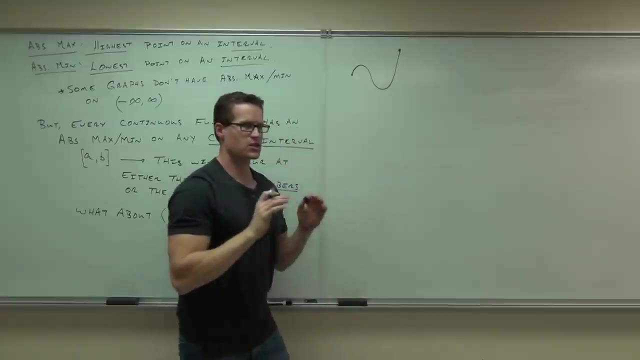 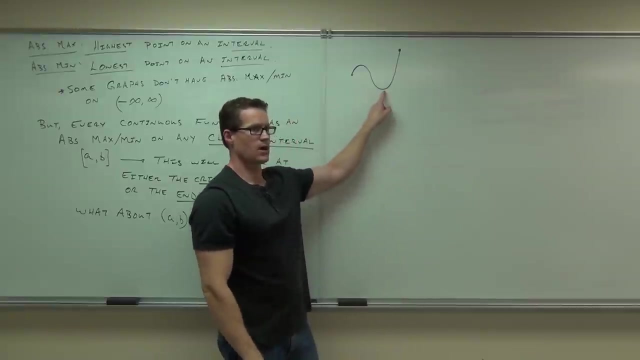 Check it out. I can erase really good. If this is closed and the points are included, can you all see that the absolute minimum for this interval is right there. That happens at actually a relative min where we change from decreasing to increasing. 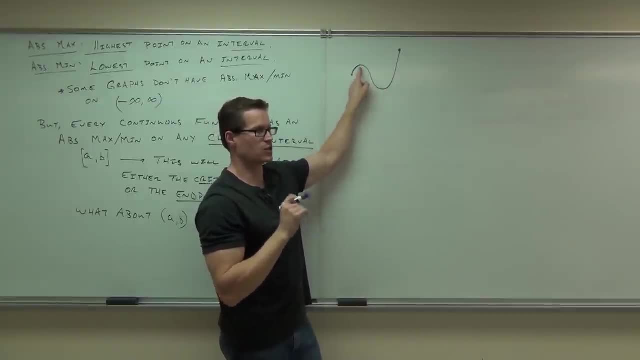 The absolute minimum. The maximum is not this point, because there's a point higher. It actually occurs at the end point. You follow me, But now watch what happens if I say ah-ha-ha-ha. That would be this case, by the way, where you're closed. 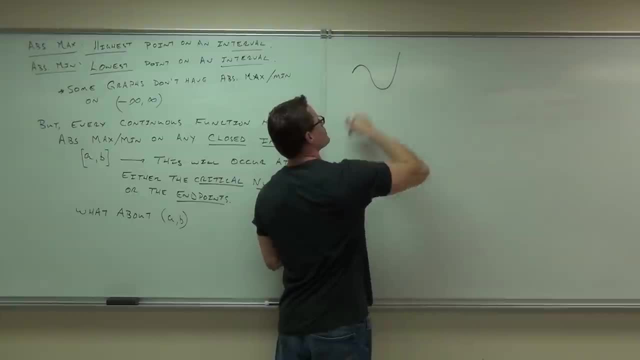 What happens if I say no, No longer. do you have those points Now this and that where they're not included. That's this case. That's this case. Do you still have an absolute minimum? Yes, That point is the same. 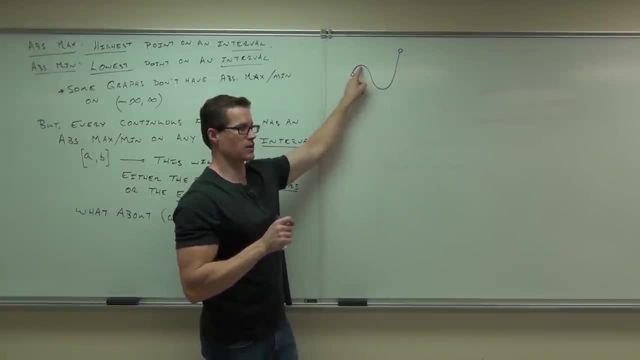 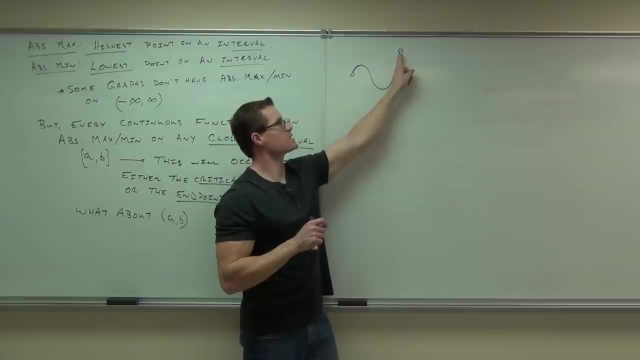 Do you have an absolute maximum? Mm-hmm, It's not here anymore, is it? Do you have an absolute maximum? Think about the question: Does this ever stop getting closer? Let's say this level is 3.. Let's just pretend that's a 3.. 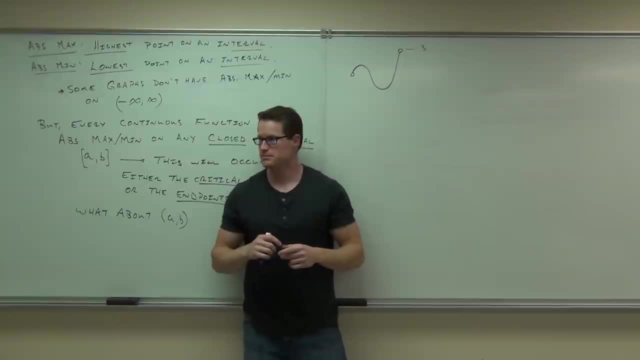 Does it ever get to 3?? No, Does it get to 2.9?? Does it get 2.99?? 2.9999.. 2.99999999999999999999999999.. Can you keep doing that forever and ever and ever? 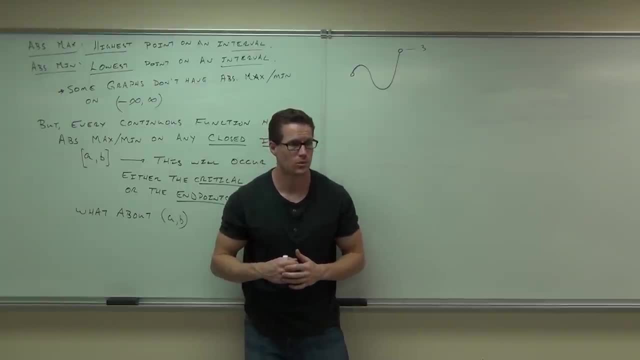 So do you ever reach an absolute max? No, No, No, you don't, because you can keep getting closer and closer to 3.. Between any two points you can find an infinite number of points right Between 2.999, however much you want to go- and 3,. 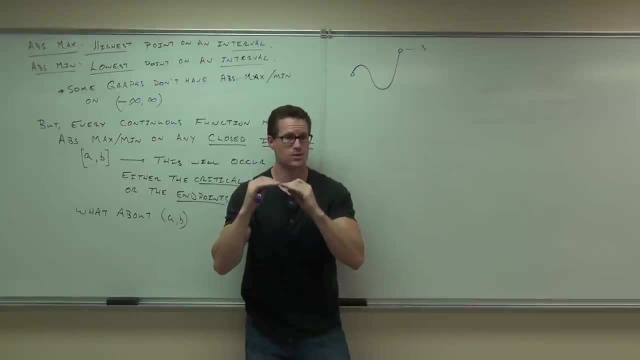 there's an infinite number of points that you can attain, So there is no absolute maximum here. What this says is that, if you listen carefully, if you've got a closed interval, you are going to have an absolute max and an absolute min if it's closed. 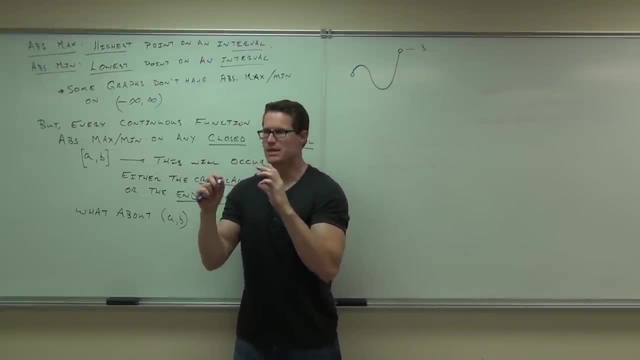 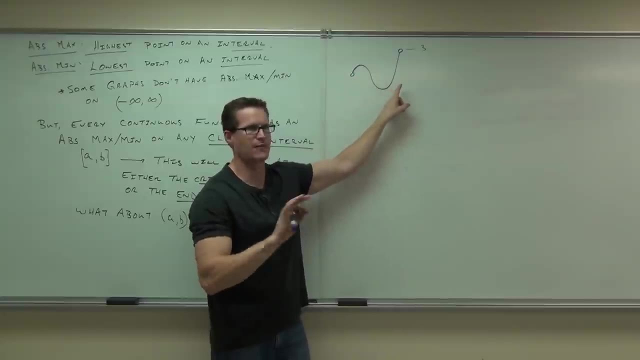 Understand. If it's open, that means the absolute max and min must happen If they occur at a relative point, at a critical number. that's where they have to occur. If they don't occur there, then they don't exist at all. 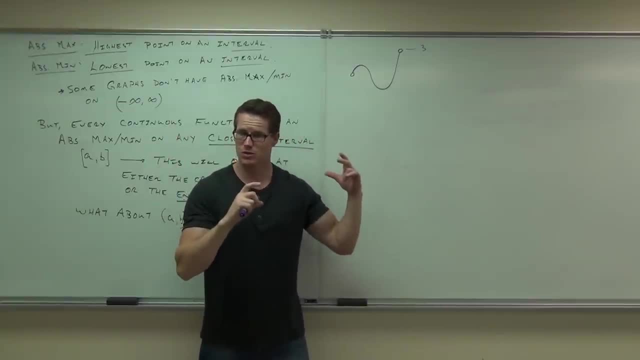 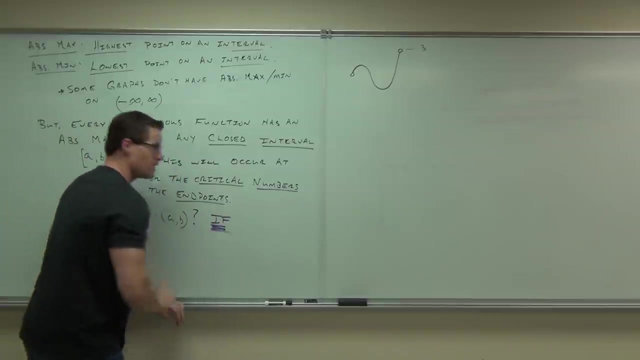 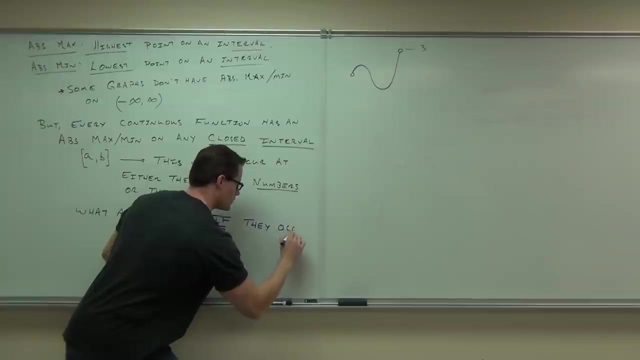 Closed intervals. you've got both Open intervals. if they were to occur, they would happen at your critical numbers. If they don't, then they don't exist If they occur. if they occur, They do so at critical numbers. 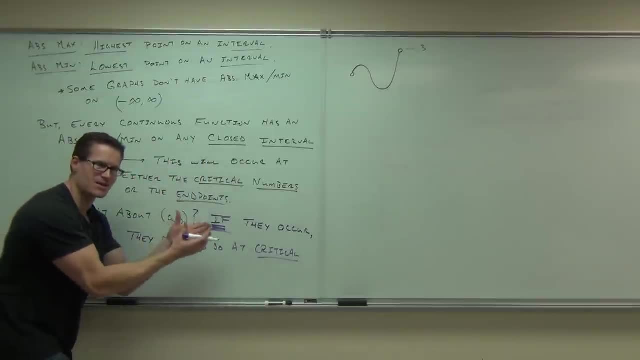 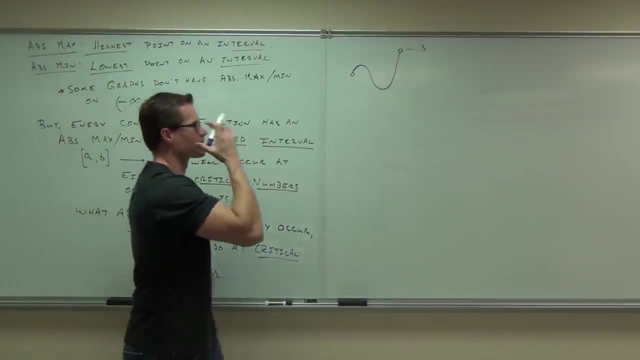 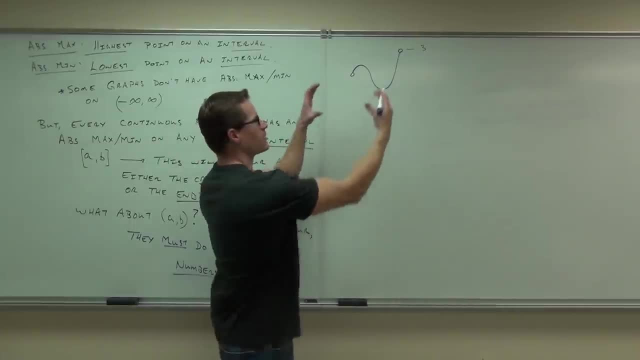 I'll tell you one thing for you. okay, Let's fill out. let's say that this is no longer just open. let's say this one's closed. Does it change the fact that we have an absolute min, but we don't have an absolute max? 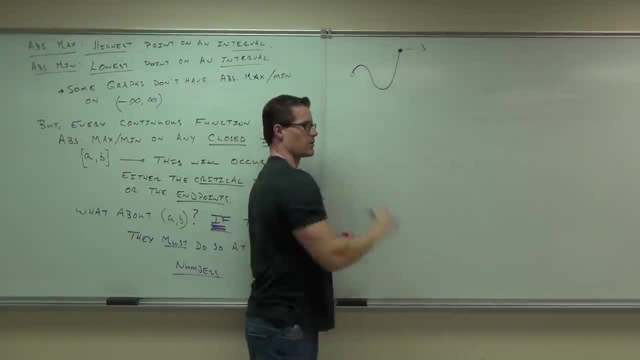 Let's say that I open this one back up and I close that one. does that change the problem? That now has an absolute max and that's the idea You're gonna be dealing with those type of intervals on your homework, where you're gonna be finding 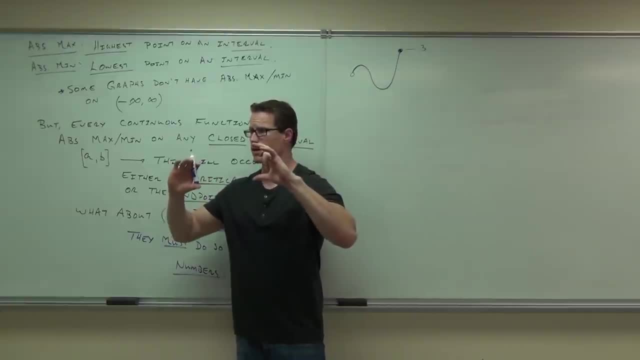 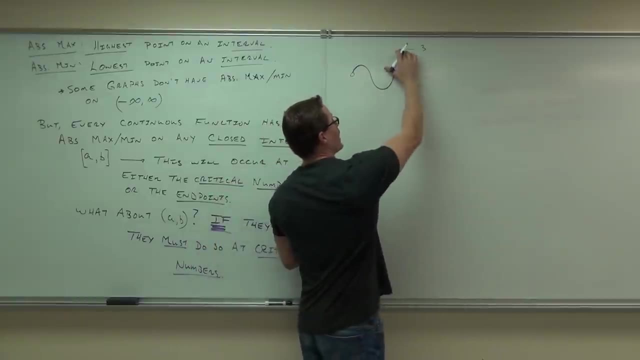 your critical numbers, no problem. If they're closed intervals, you check your end points. If they're not closed intervals, you check your end points. and they don't, you check your end points. You would still check this. you'd say: 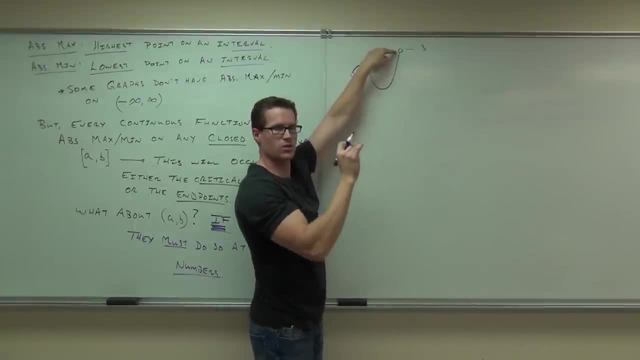 how high does that reach? How high does that reach If it reaches close to three? if I were to plug it in if it reaches close to three, well then that is bigger than this point, right? That means there is no absolute max. 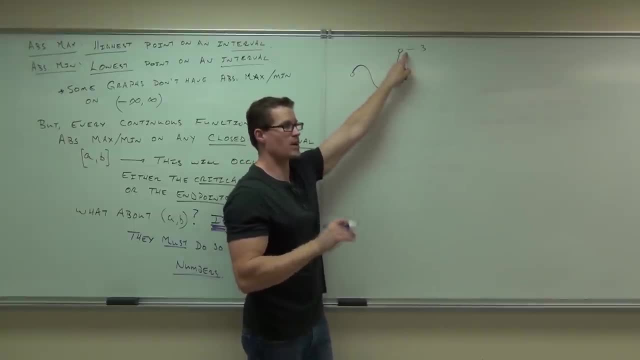 That means that, yeah, I get really close to that number. it's bigger than this one, but I never get there. therefore, there is no absolute maximum. So, for instance, if I asked you this question, find the absolute max between the interval of: 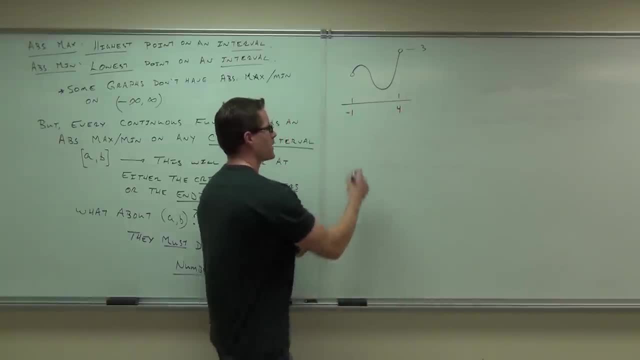 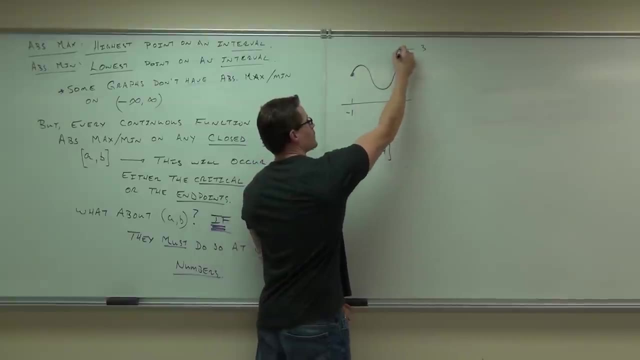 negative one to four. And I ask it to you this way: If it's this way, they're both closed in You follow me. Absolute min is here, absolute max is there. If I ask it to you this way: absolute min is here, absolute max is there. 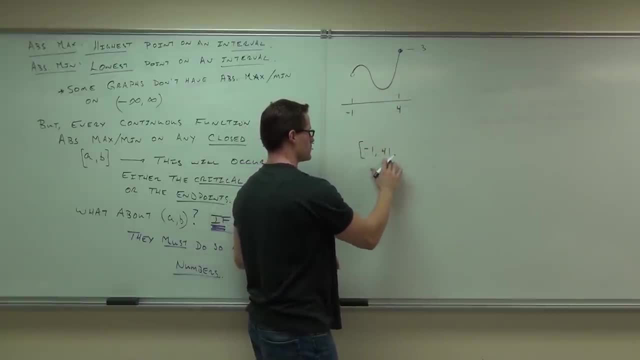 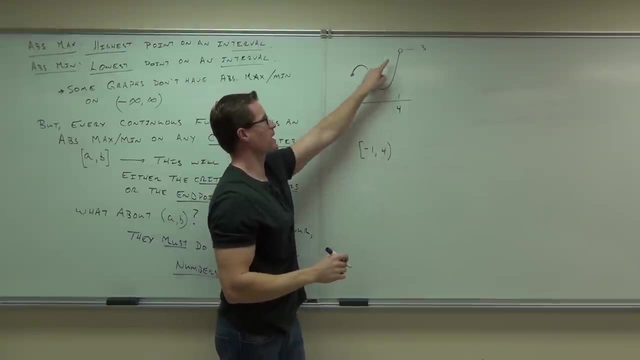 If I ask it to you this way: absolute min is here, absolute max is up. Looks like that. Absolute min is here, absolute max is up, Doesn't exist. Why not? Because you'd say, well, if it were to exist. 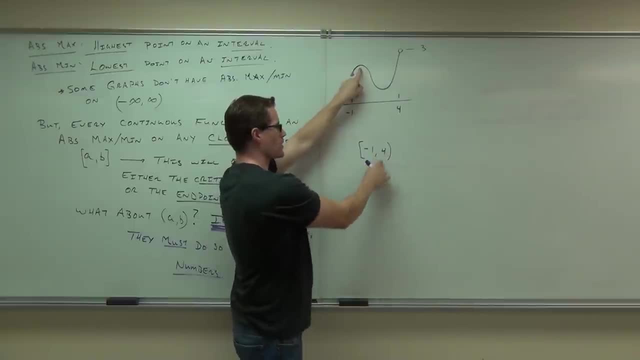 it would occur either here at a critical number or here at an endpoint. However, I don't have an endpoint, So all you have to do is this. This is what you would do: You would take this number even though it's not. 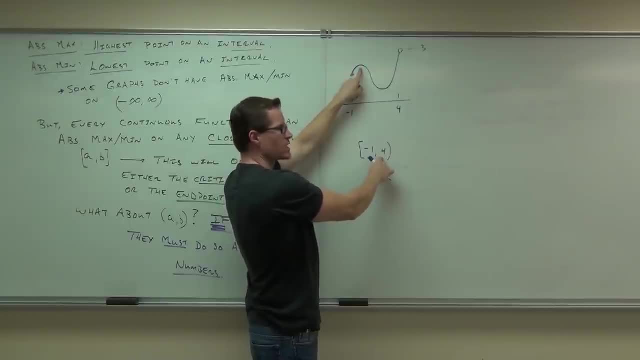 an endpoint. you'd plug it in, You'd plug it into your function and you'd say: is this value? is this value bigger than this value? function-wise? Because you're not going to have a graph, You're going to do this all with your functions. 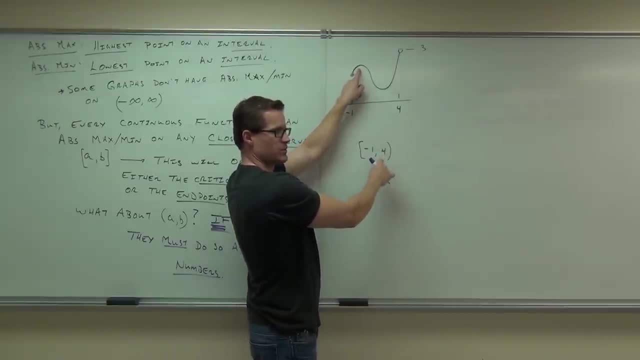 You'd plug it in. If this number, when you plug it in, is bigger than this critical number- the height of that, then you can't possibly have an absolute match, because this one's going higher than that. That's what you're talking about. 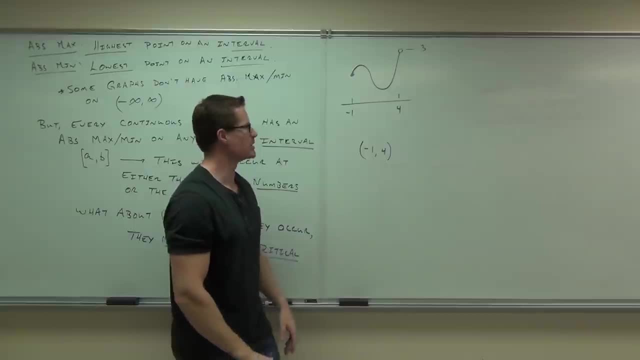 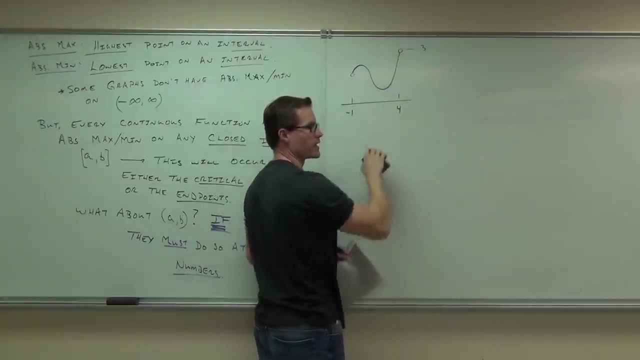 If you do this, nothing changes, Same thing. So if you were to go on with the function to the right and come back down and then put the input, what interval would you say? Like right here? Yeah, You'd have an absolute max. 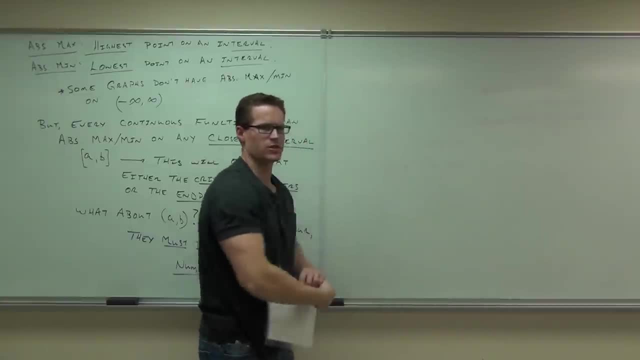 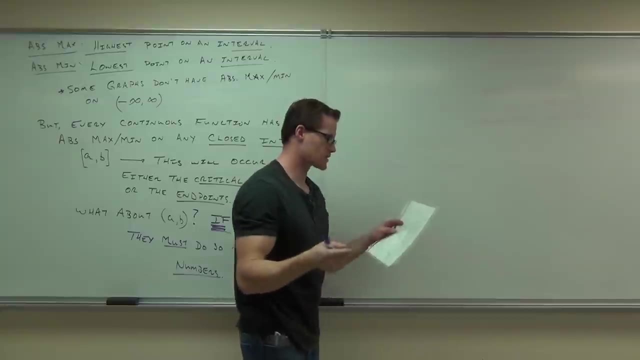 OK. Well, why don't we say: we do a couple examples here, We'll start one. Remember that clocks a little fast, so we save some time. So, to find your absolute max and min, you find your critical points and you evaluate them. 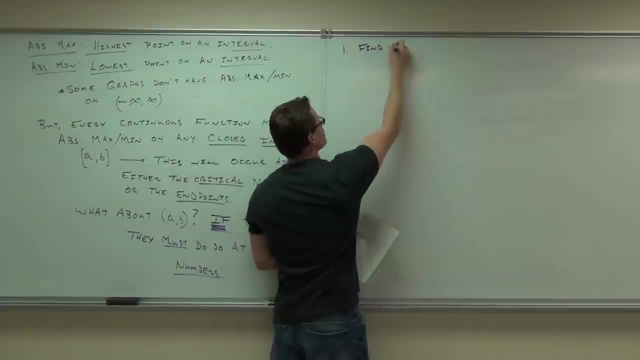 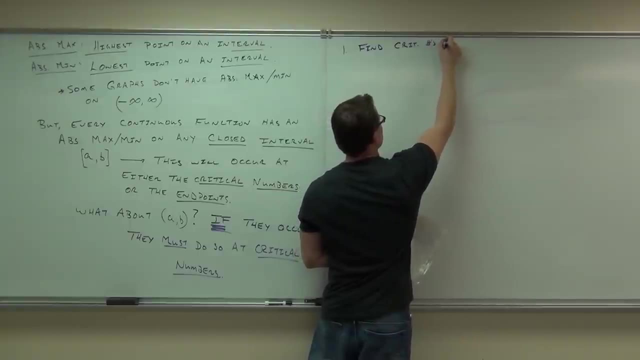 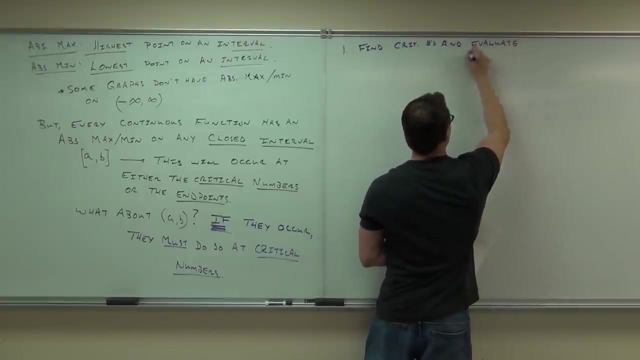 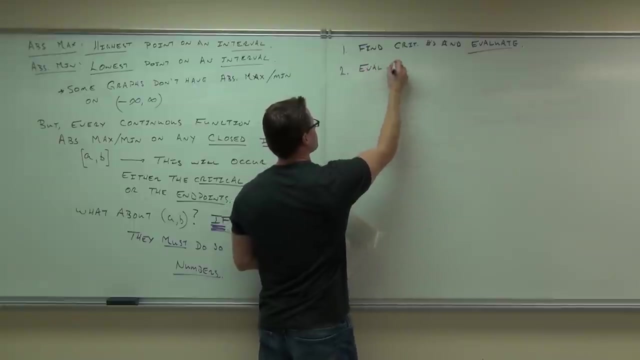 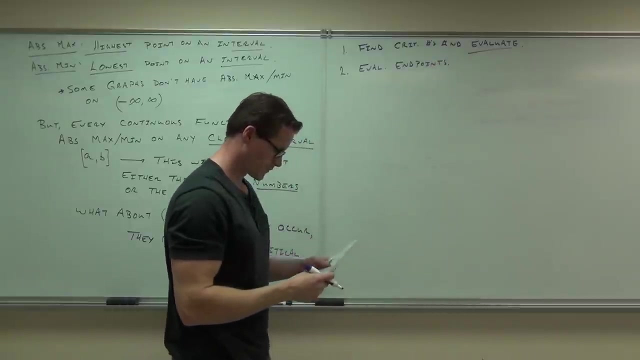 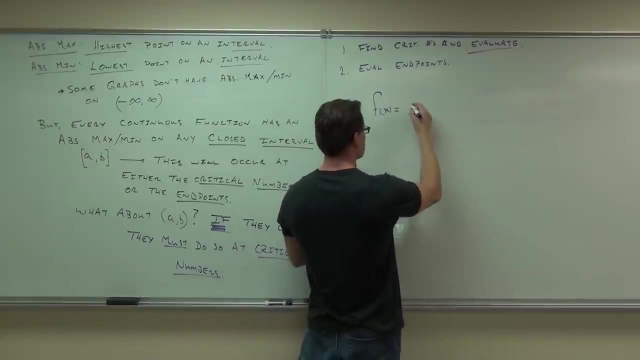 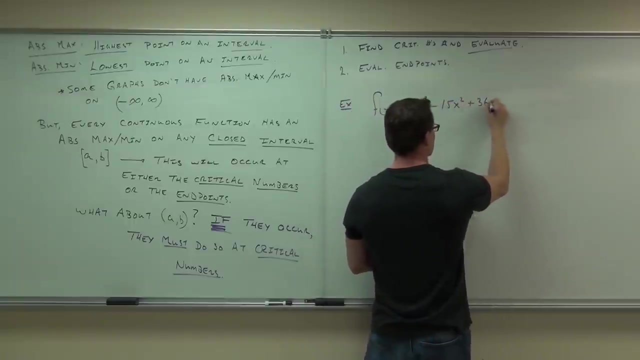 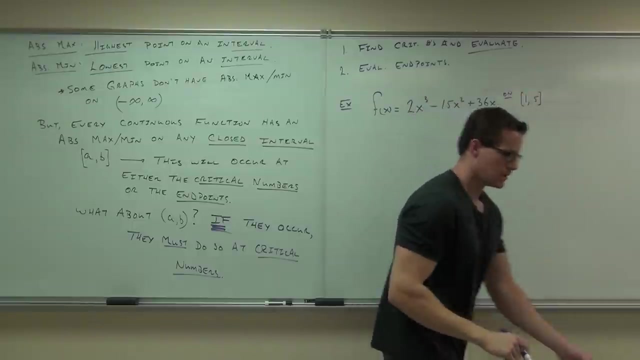 Critical numbers And you evaluate your endpoints. Let me give you an example so that I can really flesh this thing out For you, and then we'll end our day. Make everything nice and clear. Tell me the first thing you do. We're going to do it very quickly. 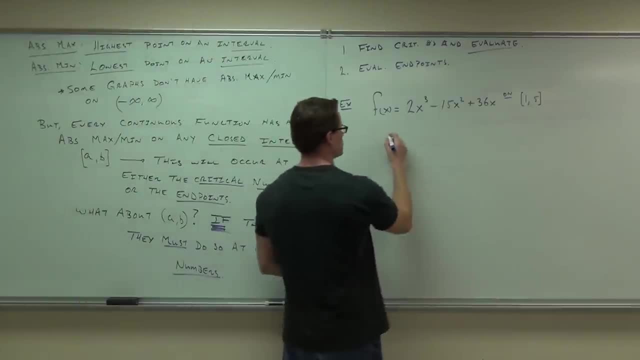 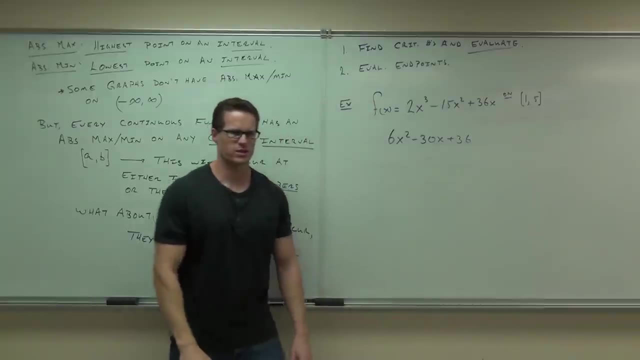 What do you do? Curate the curve, Do it? That's your derivative. Did you get the same derivative? Oh good, My derivative hat's on Taking it right today. What do you do with that derivative, folks? You set it equal to 0, because you. 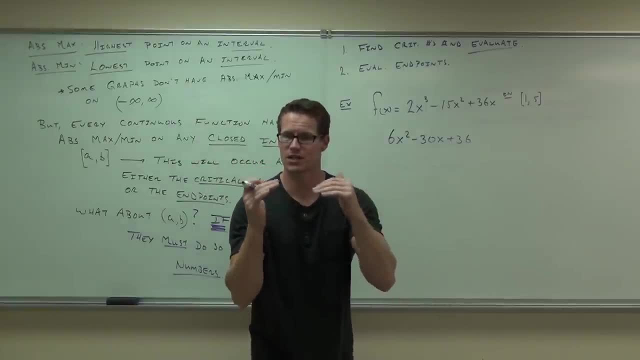 want to find the place where the slope is equal to 0,. right, That's your critical numbers. That's the only places where you could possibly go from up to down, down to up. So set it equal to 0, and factor and solve. 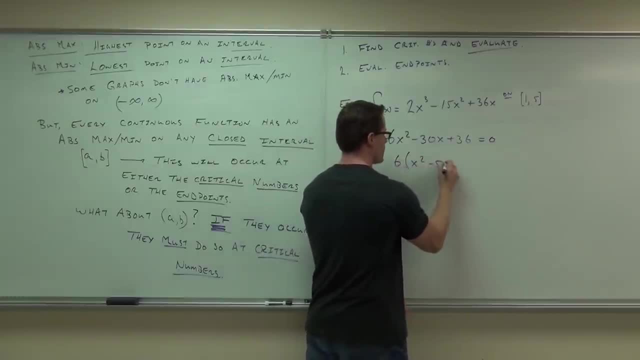 What are you going to factor out of that? You're going to get x squared minus 5x plus 6 equals 0.. You're going to continue to factor, You're going to get x minus 3.. You're going to get x minus 2 equals 0.. 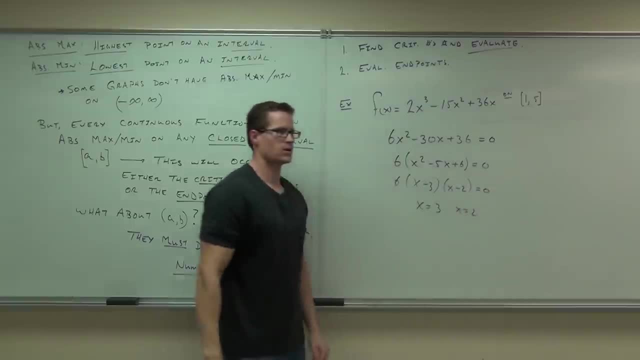 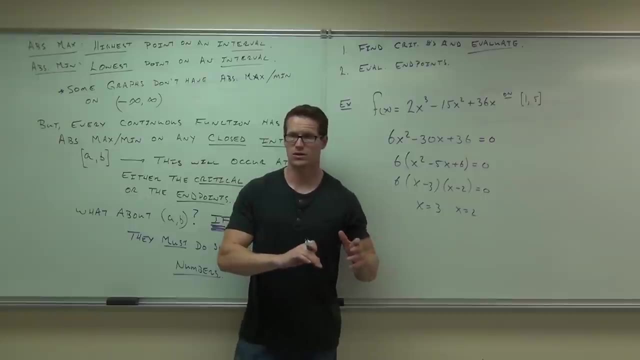 You're going to get x equals 3 and x equals 2.. I factored that very fast, but that should be kind of rare stuff. Are you guys OK getting the 3 and the 2? Are you sure? So here's what you check. 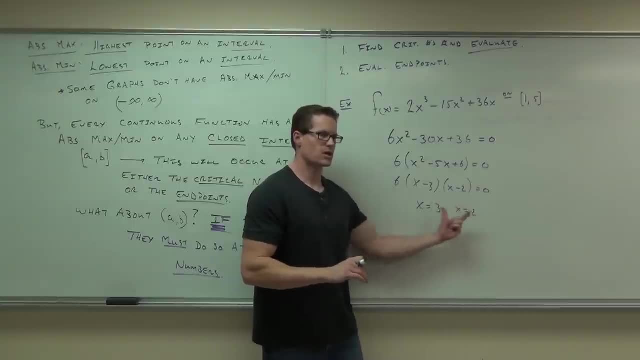 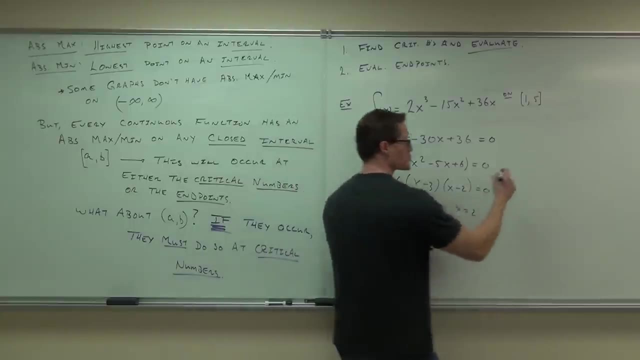 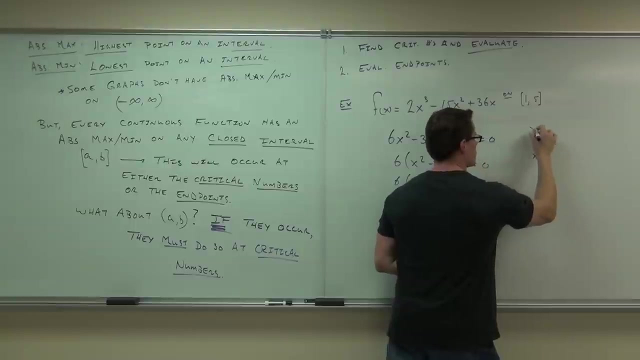 These things right here are called your critical numbers. They are the only potential for going from increasing, decreasing, decreasing, increasing your relative max and min. So what you check, you check for sure your critical numbers: x equals, 3, x equals 2, x equals and x equals. 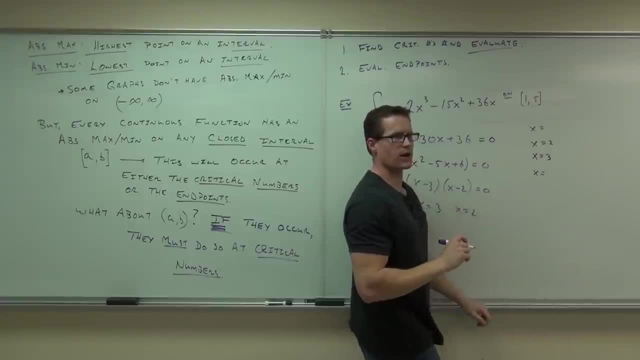 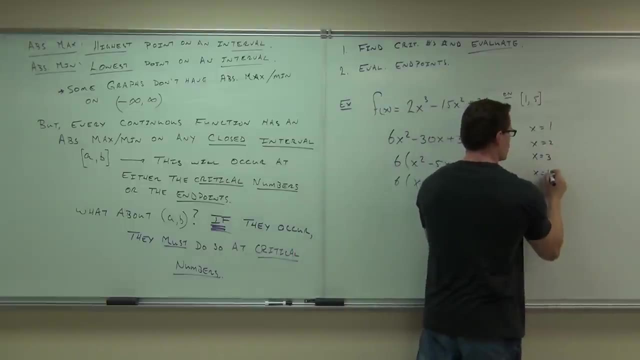 What numbers are you going to go here and here? 1 and 5.. Very good, 1 and 5.. Where am I getting the 1 and the 5?? Sure, so 1, 5.. Where do I evaluate those? 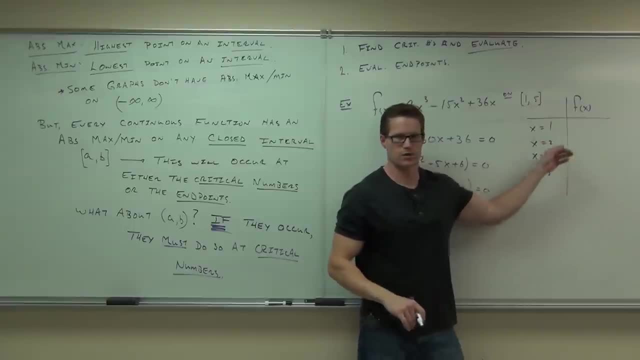 The derivative is just going to give you 0s here. That's going to give you 0s. That's something worthless for those two. We plug into original function because the original function gives you heights. Do you understand? The original function gives you heights. 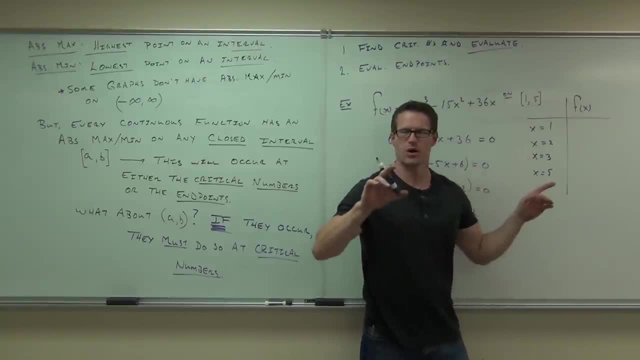 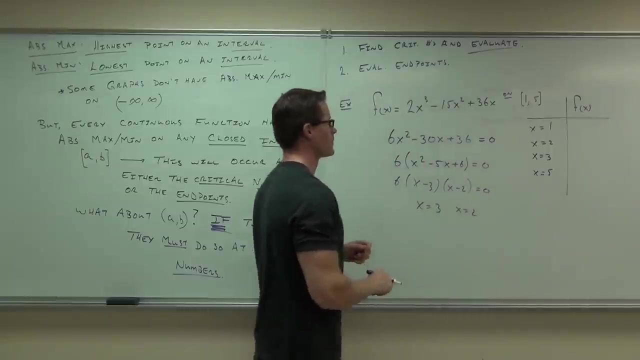 We want to find out what's the highest and what's the lowest. Would you take those numbers? people on the right side, my right side- you people Plug in the first two. you people Plug in the last two. Make it quick because we're running out of time. 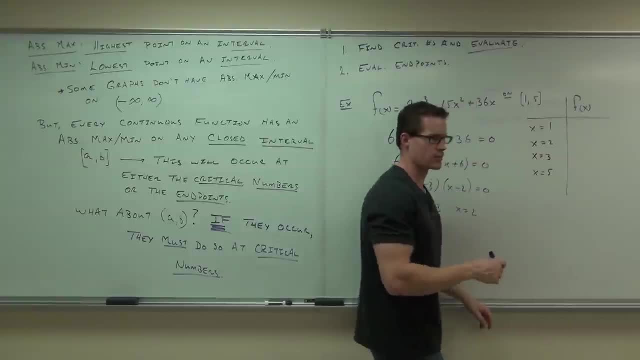 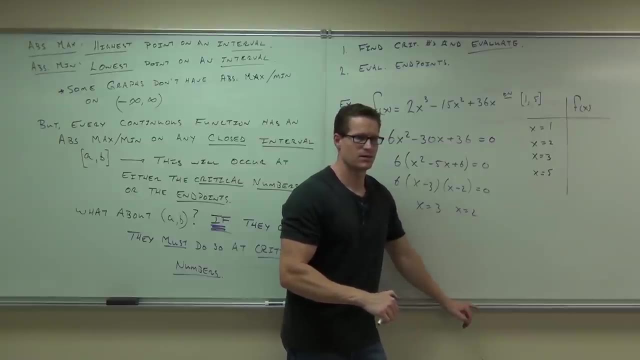 As soon as you get them, just yell them out to me for the 1 and the 2 and for the 3 and the 5.. You guys have it easy. I can't do it. in my head I'd probably do the 1 if I really thought about it. 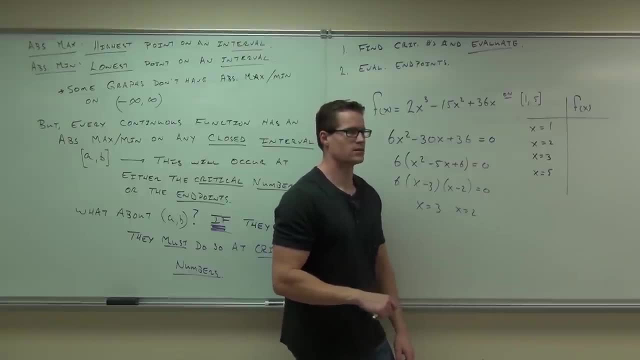 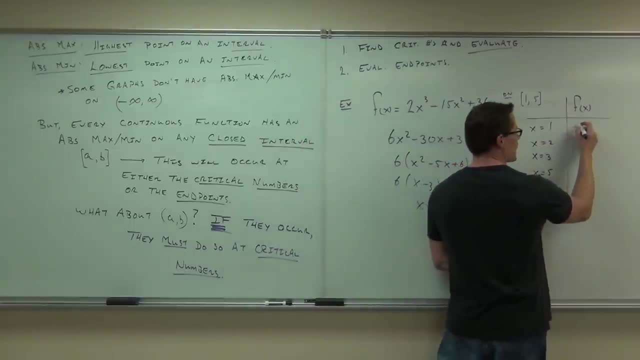 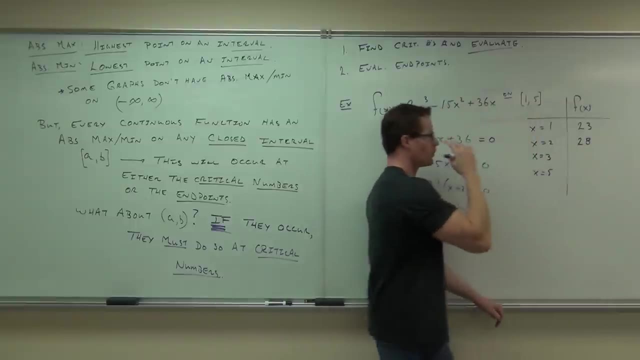 23. This gives you a height of 23.. True, This gives you what now? 28.. 28,, OK, OK, What else? What's a 3?? 3 and the 5.. Come on, 3 and the 5.. 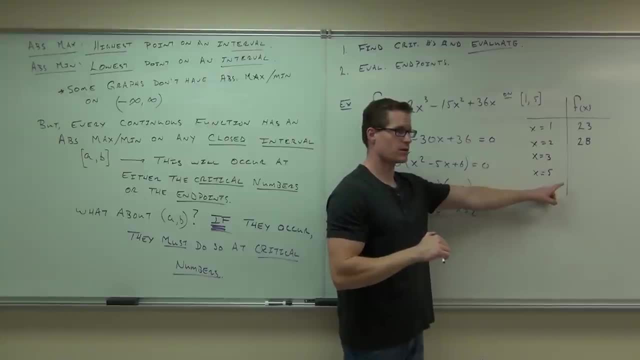 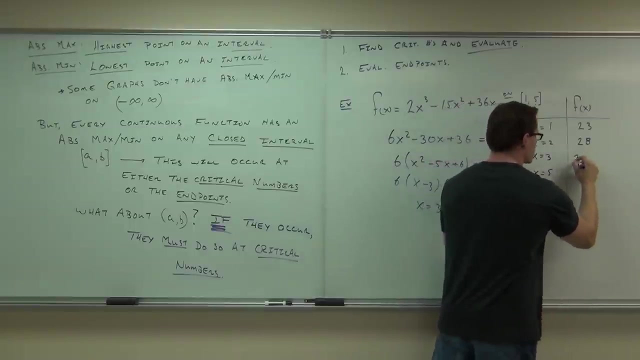 The 5,, I think, is 55.. The 5 is 55?. Maybe not 55,, OK, 55.. What's the 1. 27 for this one? 27?, 27?, Perfect, This is perfect numbers for us. 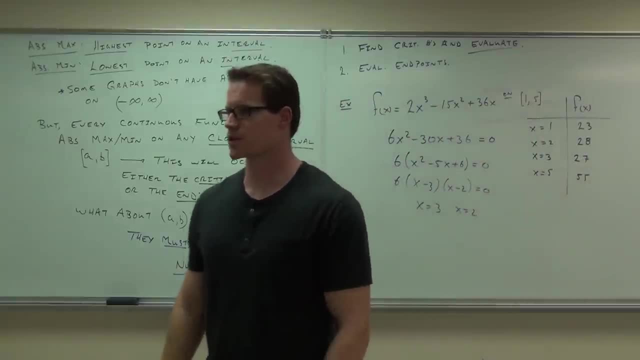 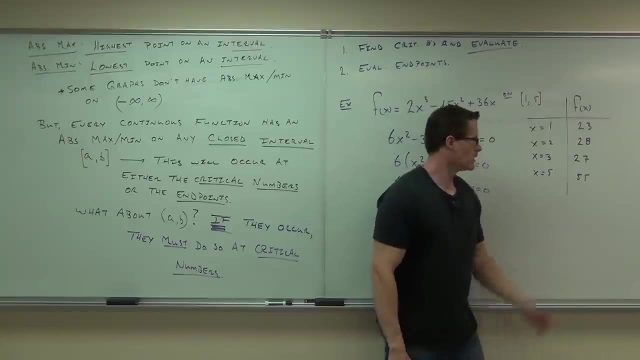 Here is the explanation of absolute max and absolute min. You need to watch carefully. This is going to put everything together in your heads right now. okay, What's the largest number that is attained? 55.. That is now your absolute max. Your absolute max is not. 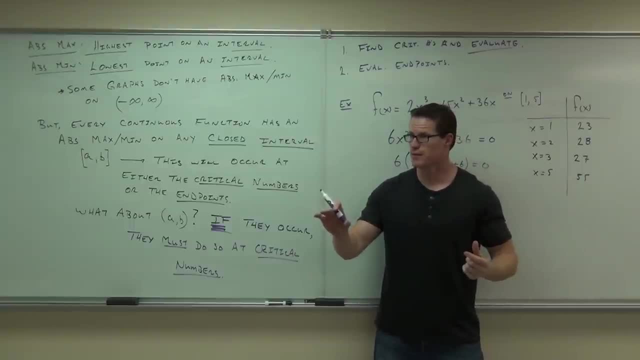 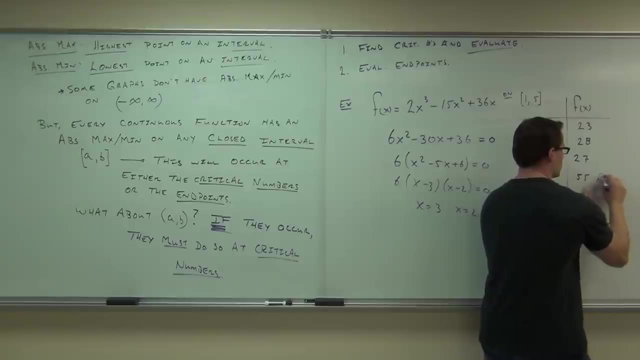 5.. Your absolute max is 55. It occurs at x equals 5.. Does that make sense to you? The absolute max is 55. It occurs at x equals 5.. That's the end point. Do you see how the 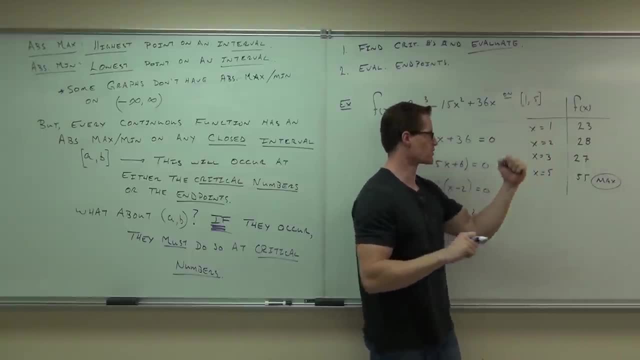 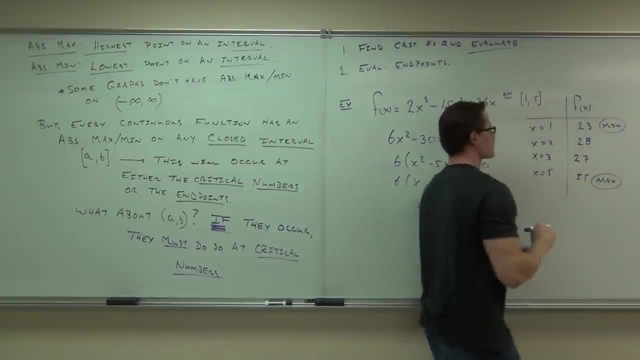 end point comes into play for us. So this goes up and then stops. That was the picture I had drawn earlier. What's the minimum value that's attained? Did they occur at critical points or end points For this one end points. 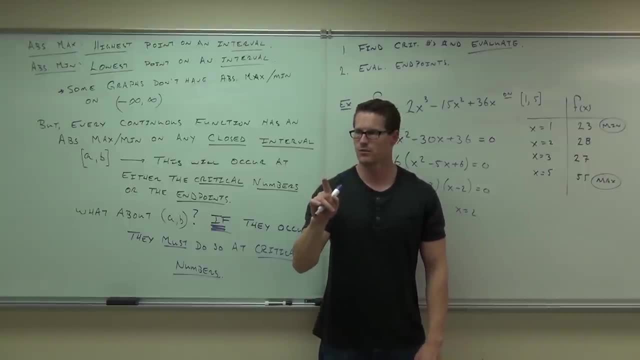 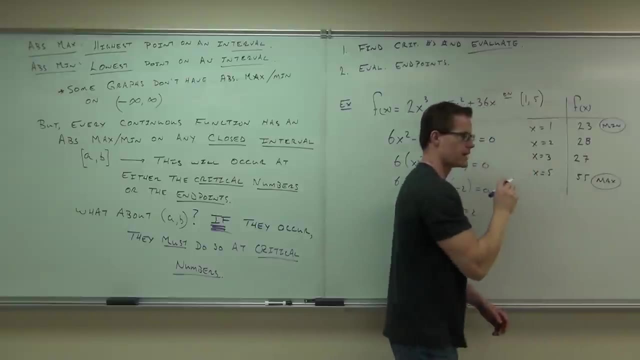 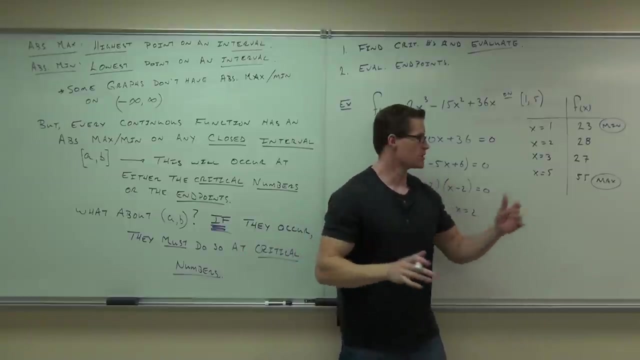 Sometimes they'll be critical points. Let me make one more thing very clear to you, and then we'll stop for today. What if I had given you this and that? Listen, You do exactly the same thing, Exactly, Only when you plug this number in and you get the 55. 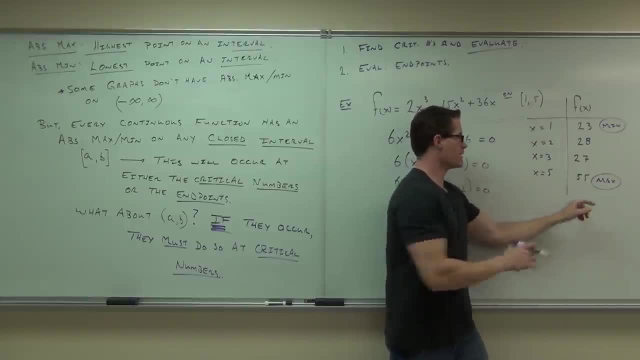 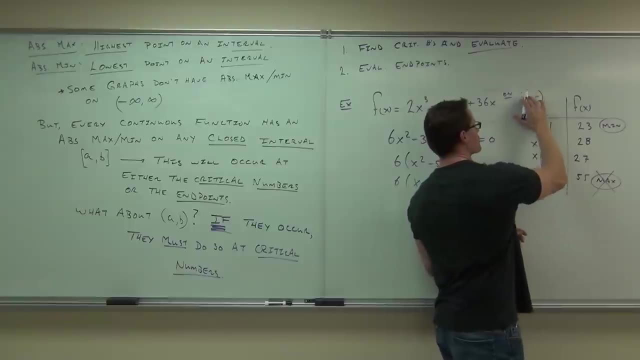 can you actually get to the 55. Then you are gone with the max. That's how that would disappear. This would only have an absolute min in this case. If I did this, you'd have nothing. No absolute max, no absolute min. 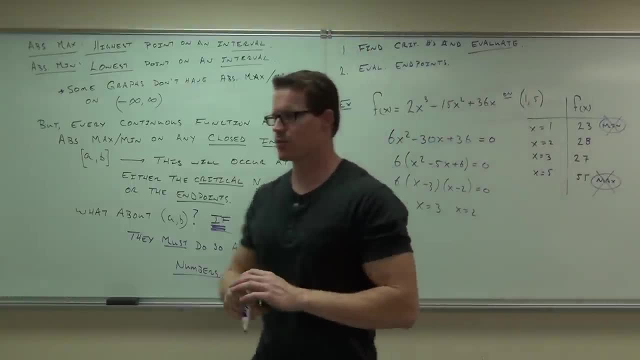 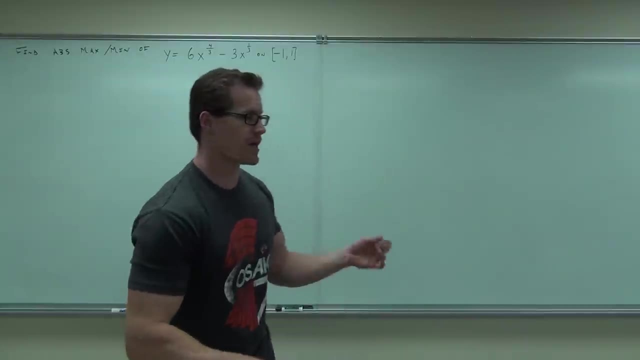 How many people understood today. We'll do one more example of this next time, and then we'll continue. Right now, we're in the business of finding absolute max and absolute min. What we discovered from last time is that- let's see what you know about this. 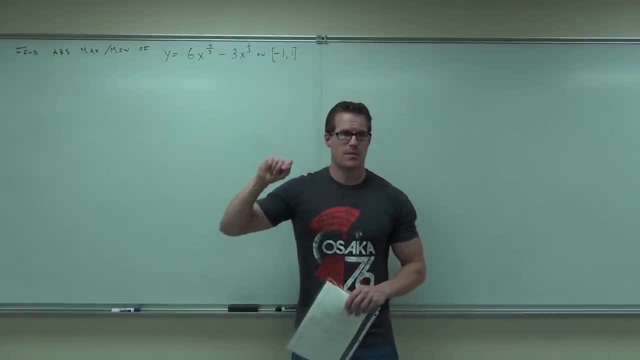 Is this going to have an absolute max and min for sure? Why would you say that If it's continuous, that's closed? The absolute max for min, if this is continuous on the interval, will either be between that open interval or at an end point. 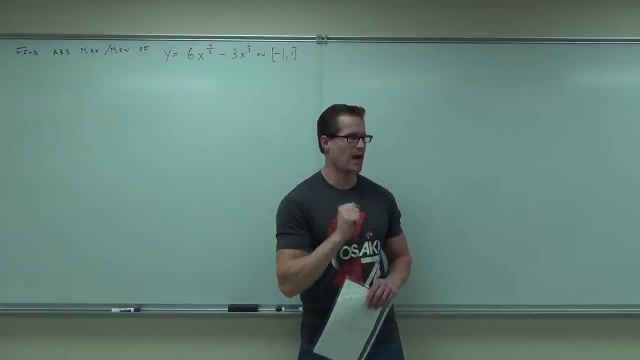 So those closed end points dictate, if that's a continuous function, that we will have an absolute max or min. If I have them open, do we necessarily have to have an absolute max and min? No, not necessarily. It could go way higher than a. 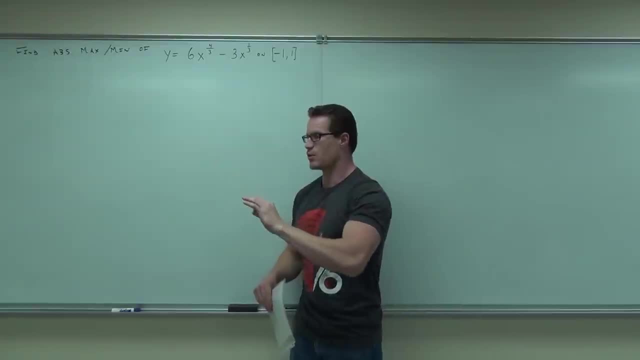 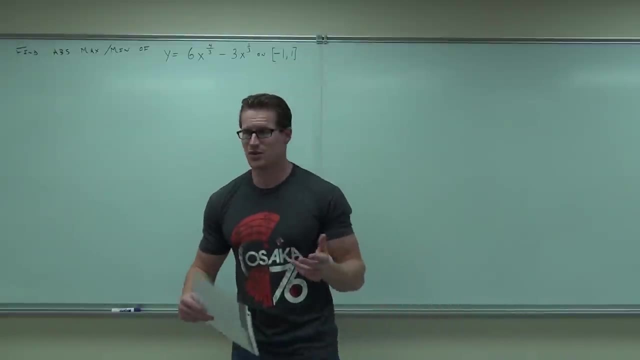 relative max, relative min, And never actually get to that point. What's our idea of how to find an absolute max or min? What do we do? first, Derivative and derivative. That's like, if you don't know, just say derivative and 90% of the time you're right, It doesn't count. 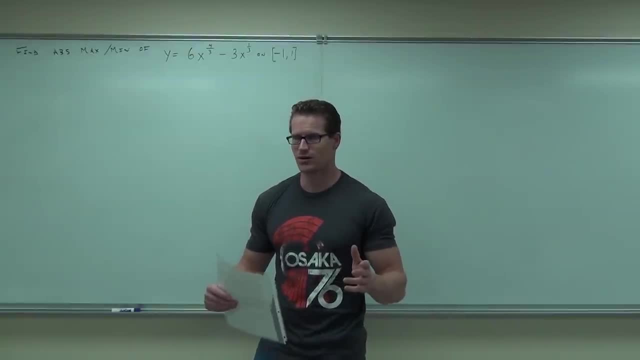 In calculus the answer is derivative. In calculus 2, the answer is integral. So if you're falling asleep and you're like Mr Leonard says what's this, You go derivative 90% of the time. you'd be right. 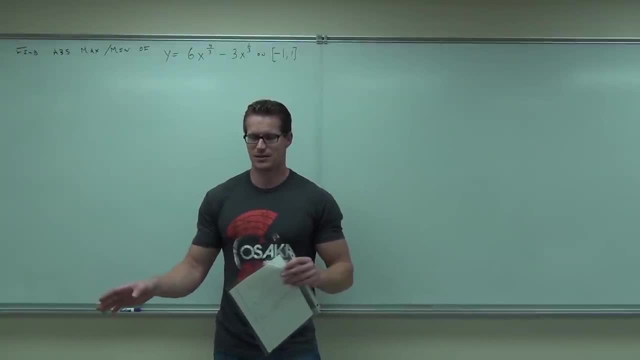 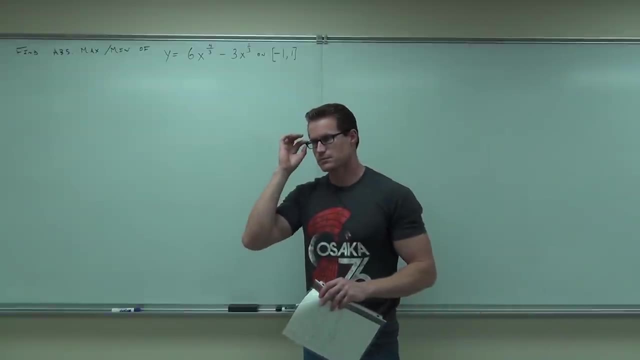 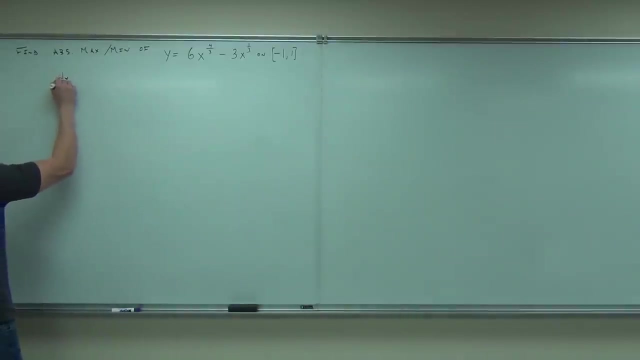 Okay, In Math 4B it's integral. Yeah, you're right, That's not most of the class. So, yeah, it's a derivative. But why? Oh good, Ah, very good, Okay. so what we're doing here is realizing. 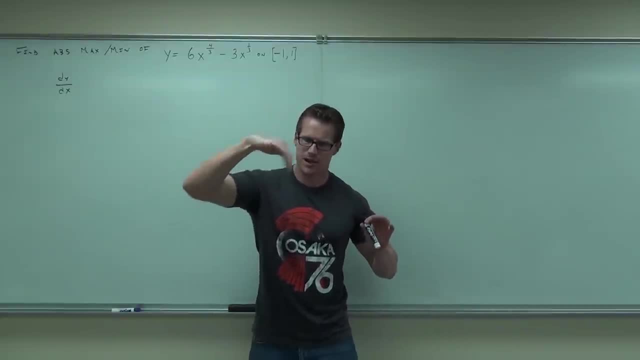 that absolute maximums have to occur at either a relative max or relative min or at an endpoint. To find relative max or relative min, that's kind of hard to do right there To find that you find where the slope is zero. Change from increase. 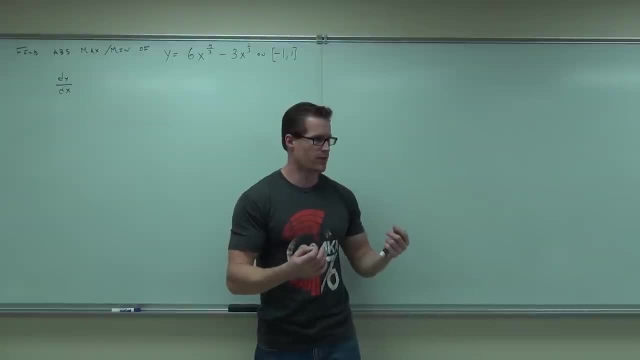 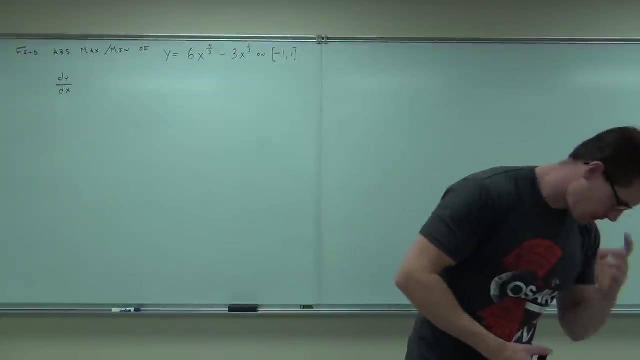 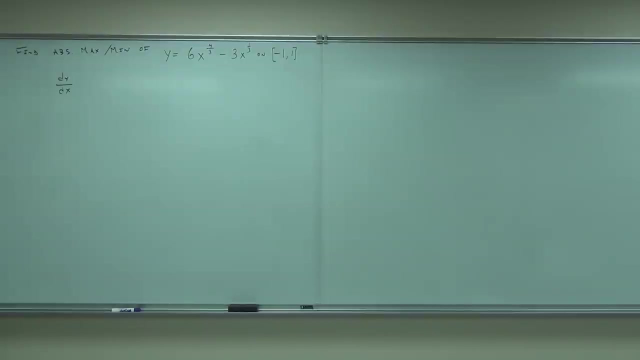 to decrease and that would give you those peaks and valleys. We evaluate all of the critical numbers and the endpoints and that will tell us the highest and lowest. Find me the first derivative, please. Okay, first derivative, If you do this, 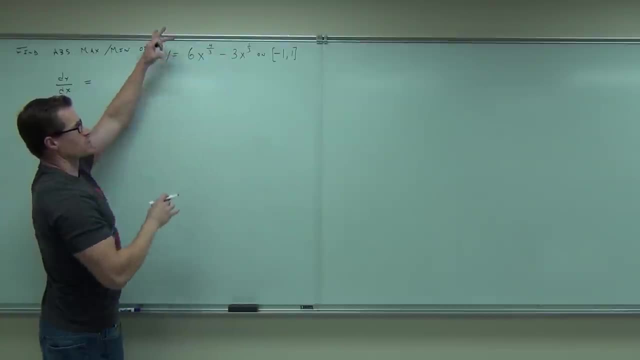 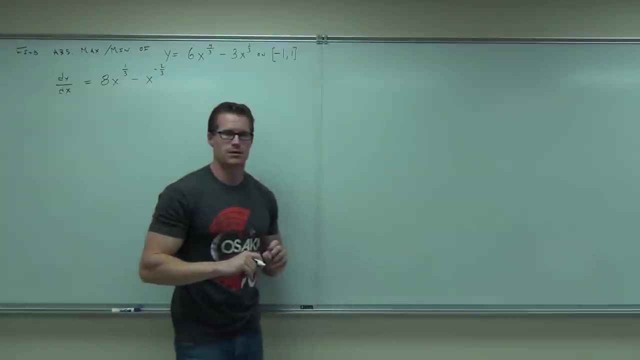 first derivative says: you take down the 4 thirds, you're going to get 24 over 3, or you simplify as you go. Either way you get 8.. X to the Good Minus Perfect. Very good. How many people were able to find that? 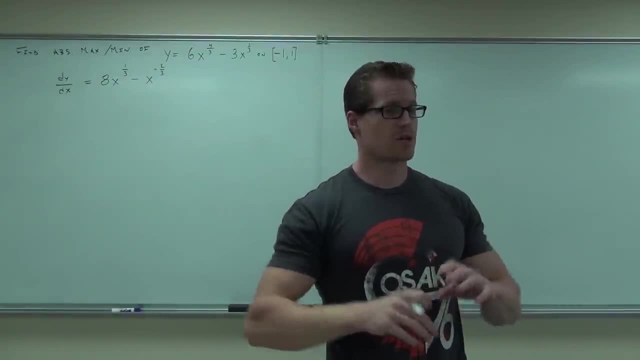 Good for you, Alright. Now what do we do with that? Good, because that is my slope. I want to find out where I have a horizontal tangent, That's, the potential places where I could be switching from increase to decrease, or 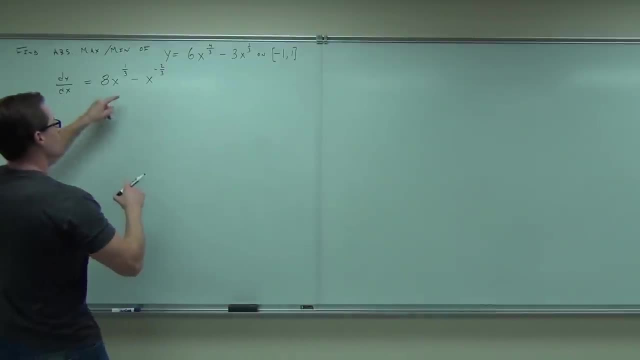 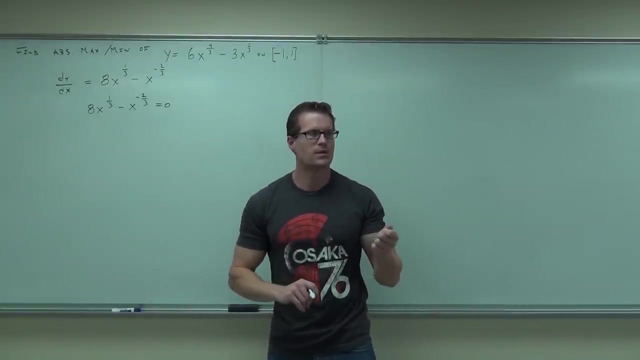 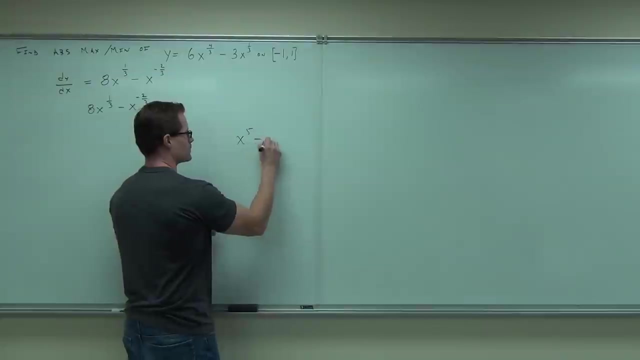 decrease to increase in potential places. We'll check that. So here we're going to go ahead. set this equal to zero And solve for X. How a fifth out of that would you? 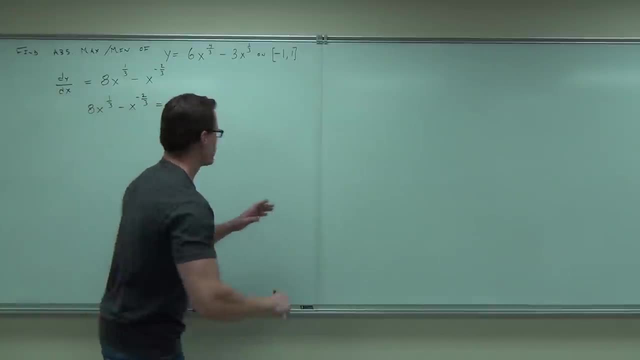 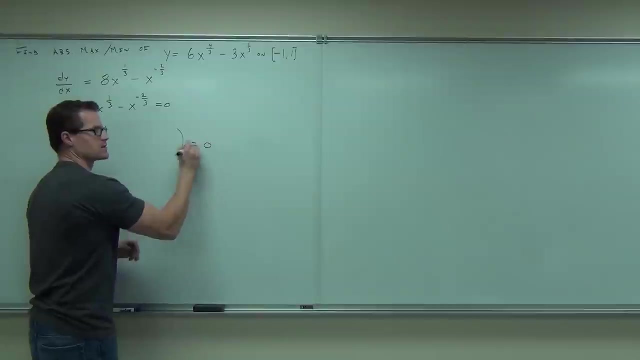 Try to factor out x to the smaller one and a lot of times it's gonna help you. So if I factor out x to the negative 2 thirds, remember that factoring means divide. right. Factoring means divide. Distribution means multiply, so factoring means divide. 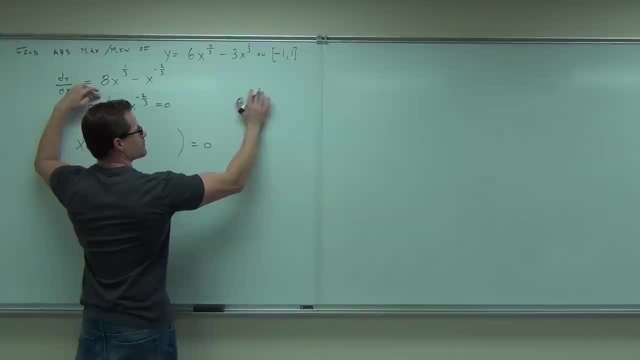 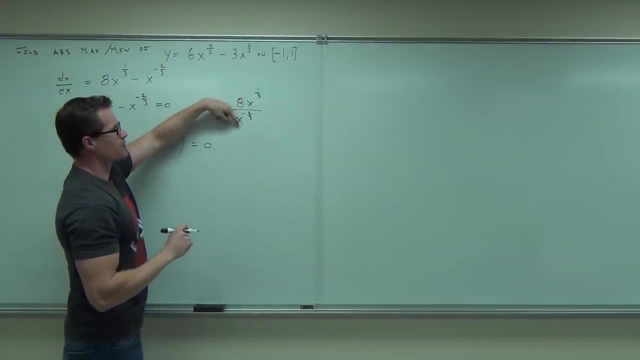 We're taking our first term, sorry- divided by the term. we are factoring out What happens when you have common bases being divided. You are subtracting exponents. so do this math in your head: 1 third minus negative, 2 thirds. 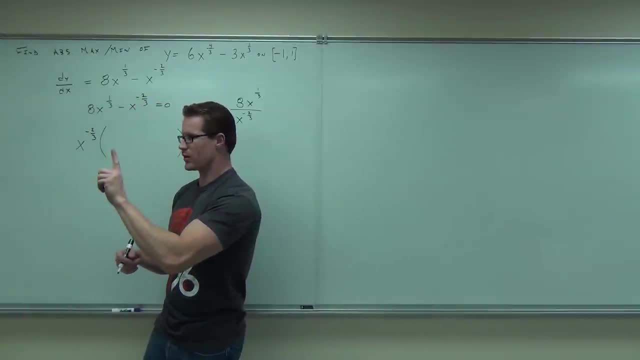 You're actually adding 2 thirds there. You're gonna get x to the first power. Do you see what I'm talking about? You're gonna get x to the first. So this right here gives you 8x. Reason is because you have 1 third minus negative 2 thirds. 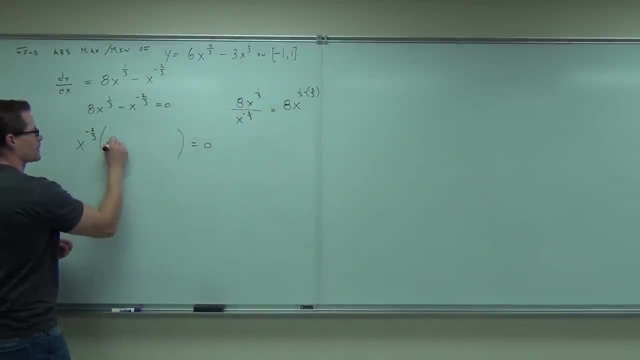 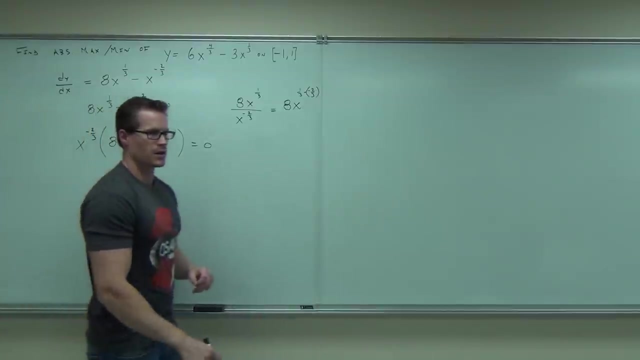 That's three, oh three, that's gonna be 8x Minus. well, this one's easy X to the negative 2 thirds. you pull the whole thing out, we get one. Is that a lot easier to solve? 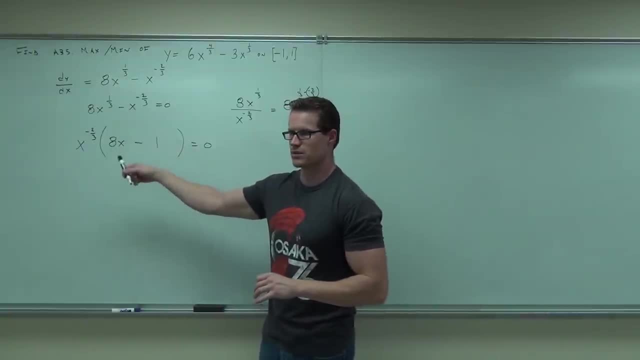 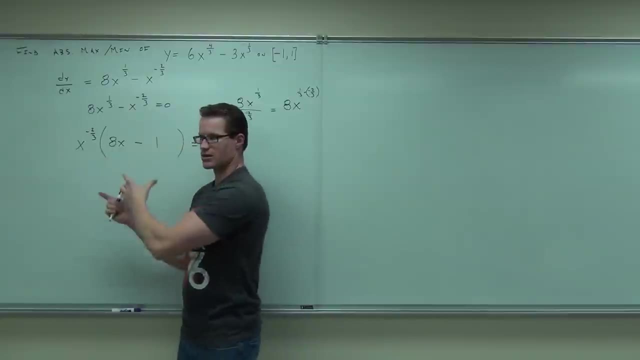 Oh heck, yeah. Yeah, this is. you'd be stuck on that if you couldn't factor Stuck. But here we now know that we have two factors being multiplied together. that gives us zero. The zero property says that either this one is zero. 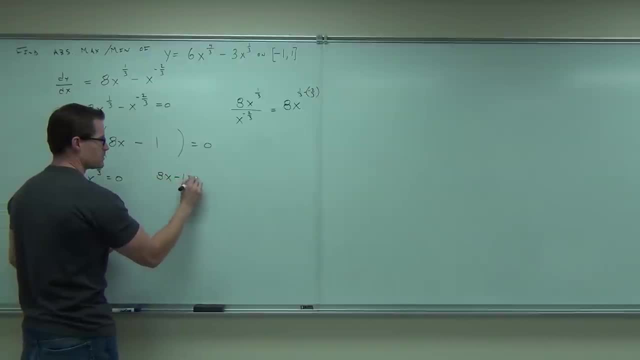 or this one- don't forget about that one, by the way- or this one is zero. That means x equals zero or x equals 1 eighth, What are those numbers called that we just found? What are those Critical points? 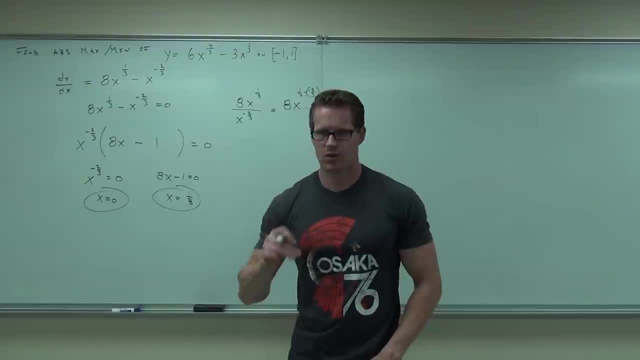 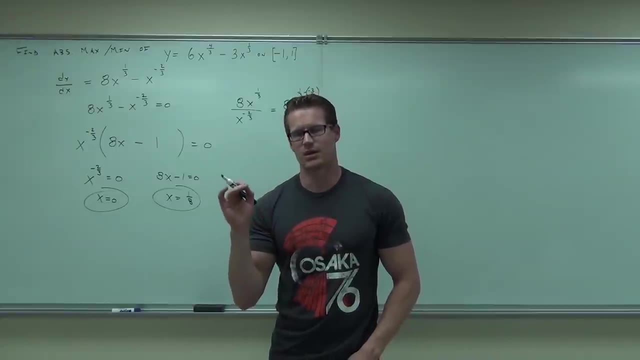 Critical points are critical numbers. I think your book might use critical numbers. Critical points are critical numbers. That's what those state. Those are where you have the potential of having a horizontal slope, or, I'm sorry, you do have a horizontal slope. 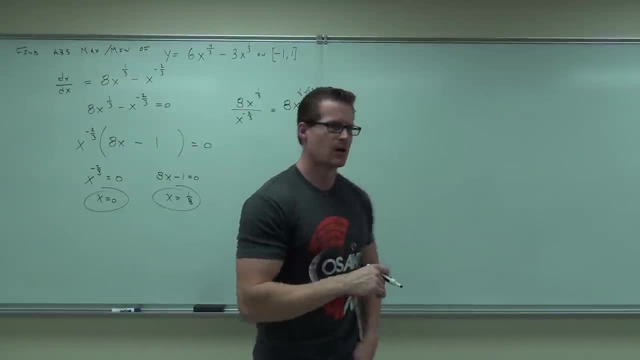 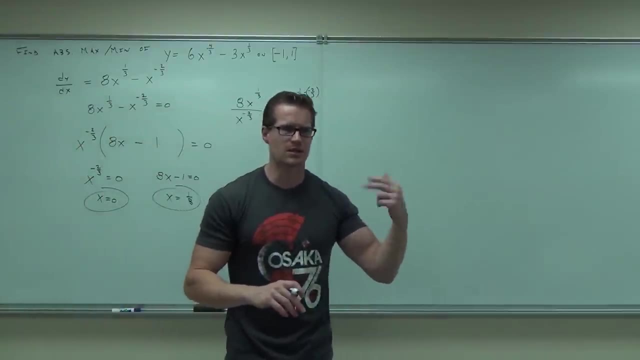 Potential of having relative match or relative min. Are you okay on finding that? The basic algebra Does that help on that? You can come and see me. I'll show you how to factor out negative exponents. that should be in from your Math C classes. 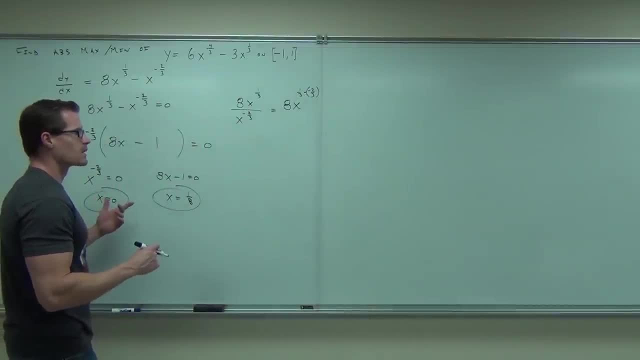 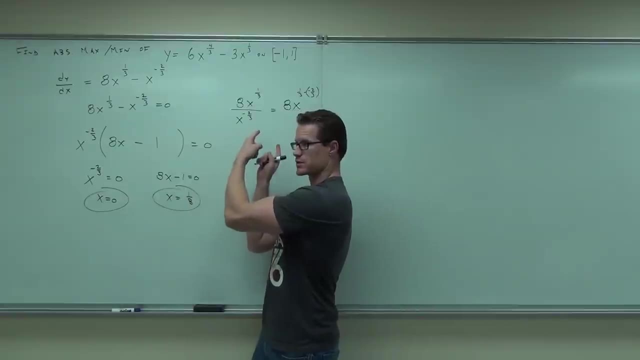 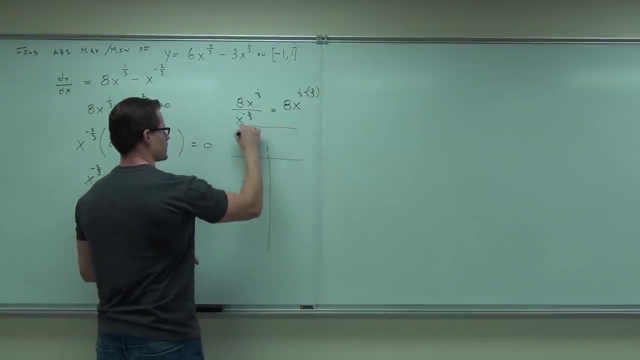 or your intermediate algebra classes. Now, what do we do after that? Plug it into the marginal points, These two and what else? Organic points, Endpoints, so do that. So here's our x values. we're plugging in. 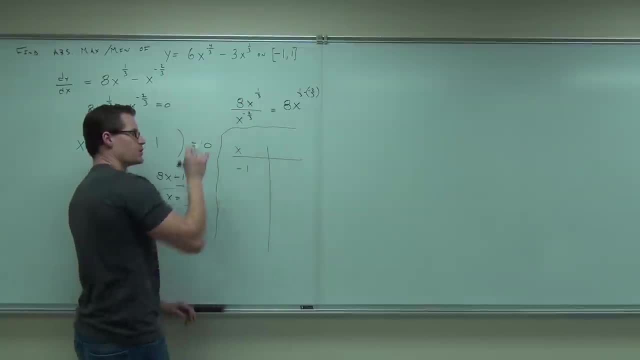 We're doing negative one because that's in the middle. Negative one, That's an endpoint. We're going to do zero because that was a critical number. We're going to do one eighth, because, hey, that was a critical number. 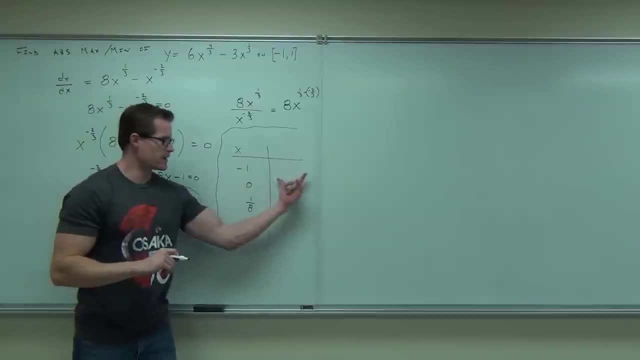 And we're going to do one, because that's another endpoint. Whichever one of these values is biggest, that's your absolute max. Whatever one of these values is smallest, that's your absolute min. And these are the places where they occur. 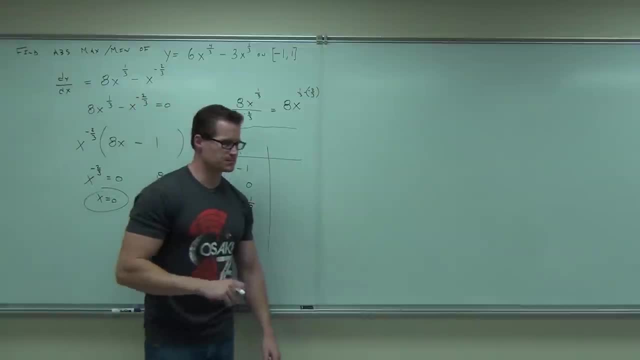 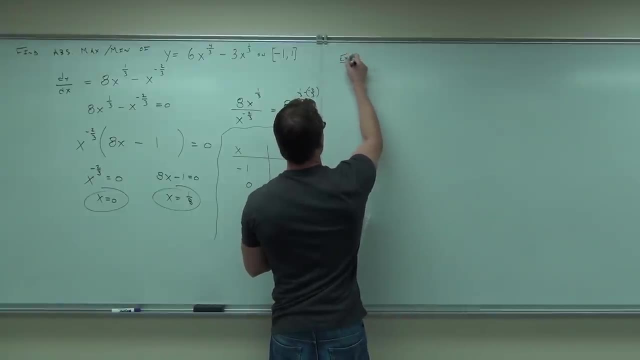 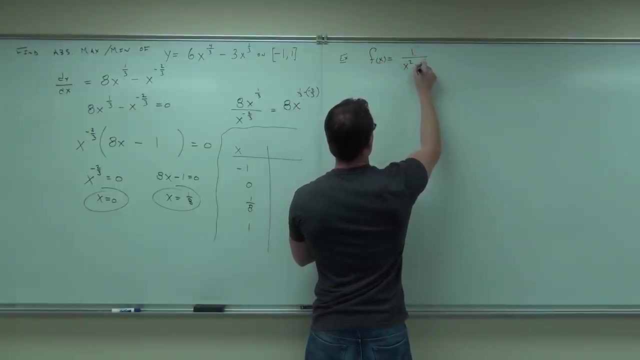 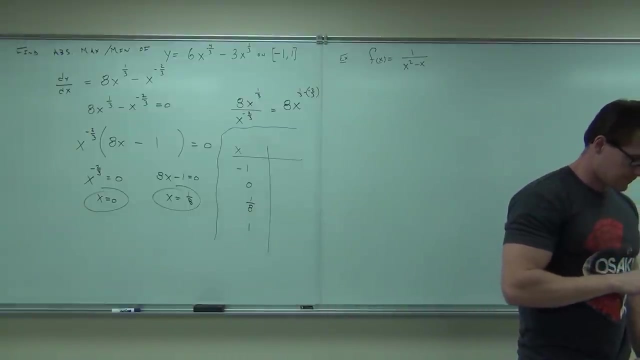 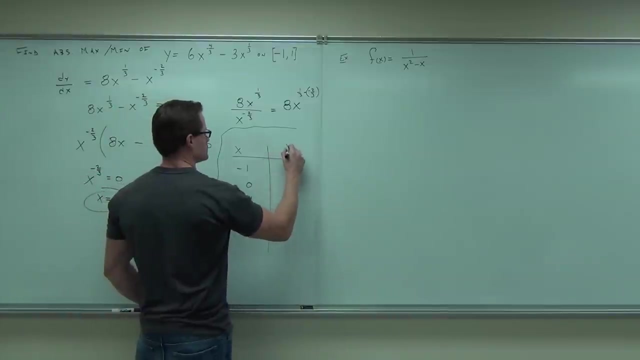 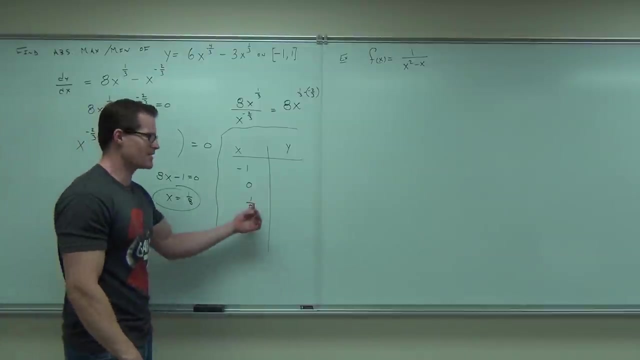 I think I made that point last time. Go ahead and plug those in for me and find out what you get. Thank you, Oh, how nice was I that I gave you one eighth huh, Of course, that was so nice. Cube roots. 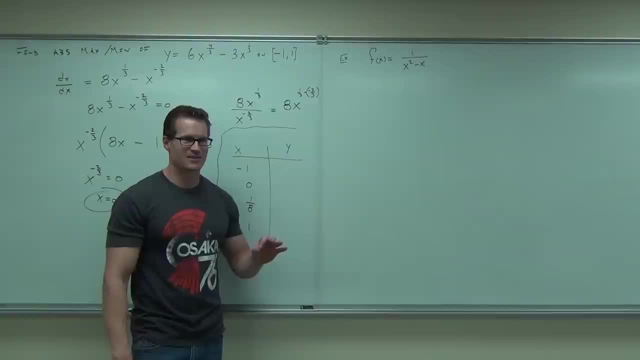 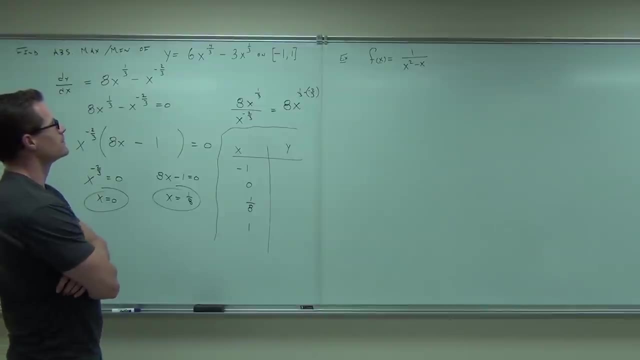 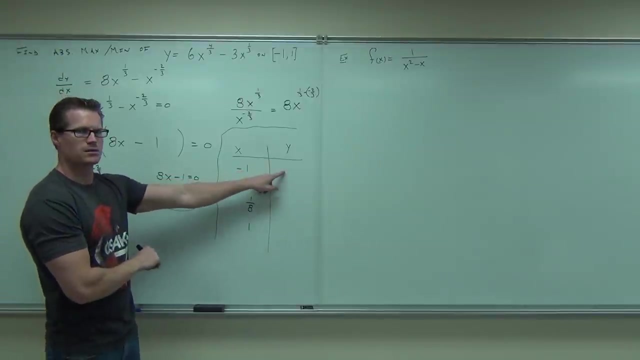 Oh, you love me now, don't you? No, I made it that far. Okay, you will love me. Get down to here a little bit. Let's see Negative one. What'd you get? nine, Tell you what. 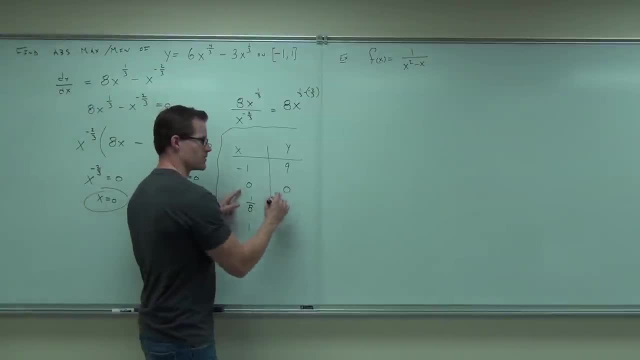 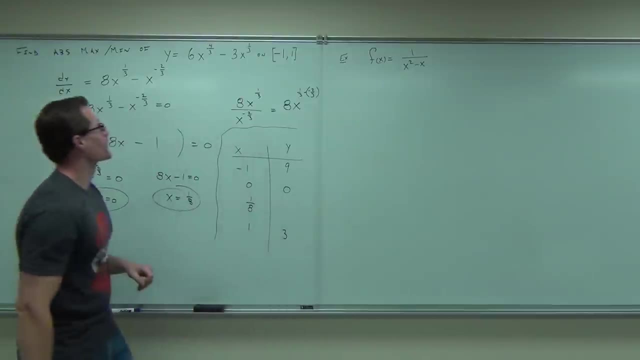 I'll do this one for you guys, just because I'm a nice guy. Give me that one. Three, Sixteen, What's sixteen times six? Ninety-six, Sixteen times six, So ninety. Better do that wrong. 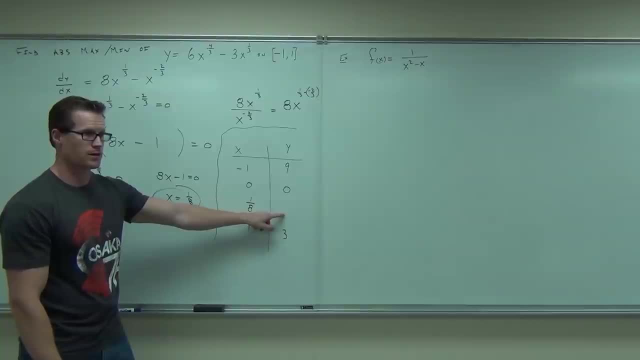 Ninety-six, Ninety-six, Wait for the whole thing. Oh no, No, you have to subtract six. I believe Someone tell me what that is. You should be looking at me blankly right now. You should have a calculator and you should be working on it. 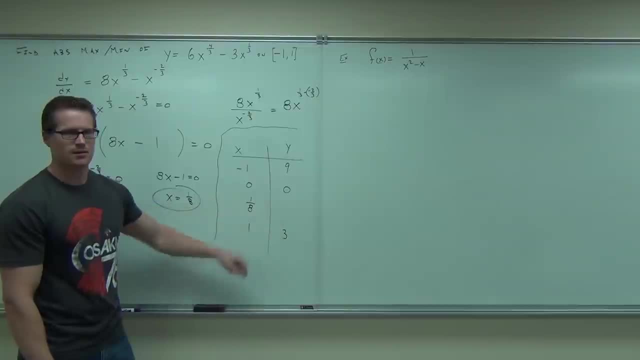 Don't look at me blankly. Come on, if I can do that in your head and you have all the calculators, you should be able to work that out. Oh, you know I did it wrong. It's it's. I was wrong on that. 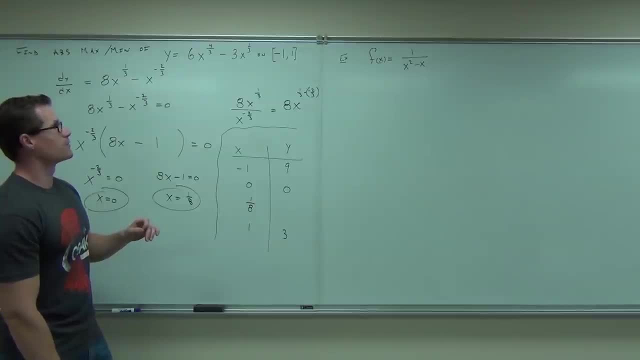 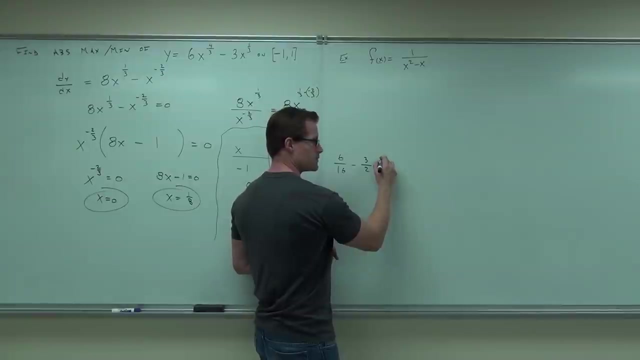 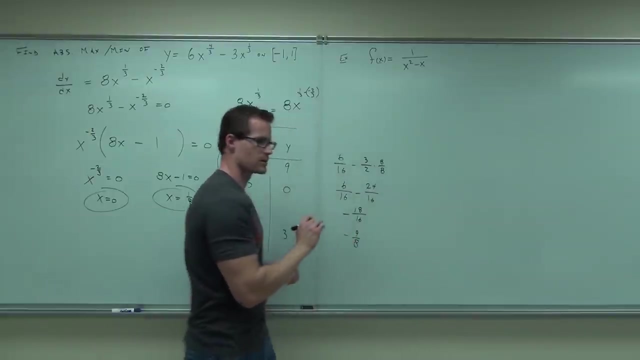 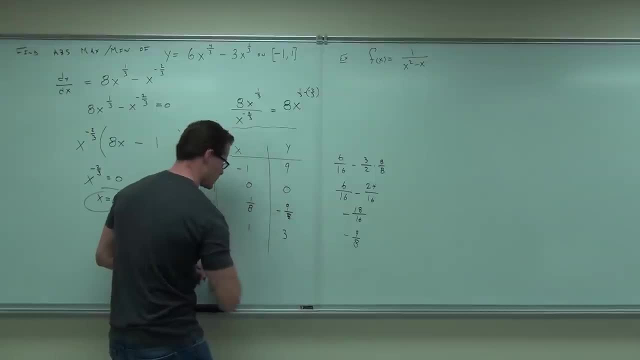 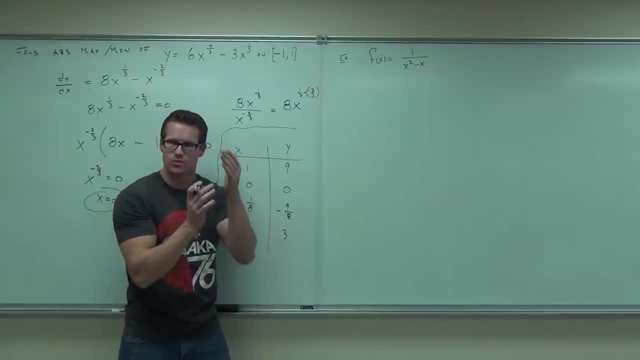 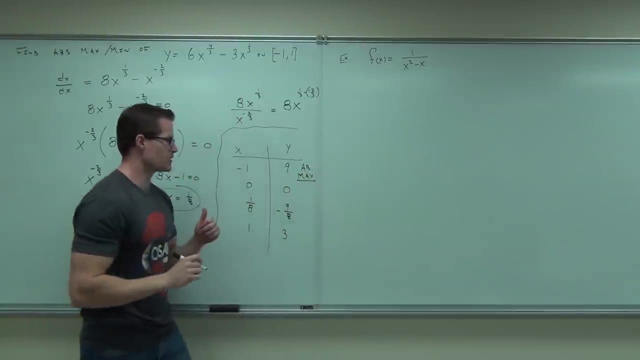 The absolute max is not negative one, Okay. That's just a place where, on the x axis, where you get it. So this is your absolute max. It occurs at x equals negative one. What's your minimum Negative-ninth? That's the one, yeah. 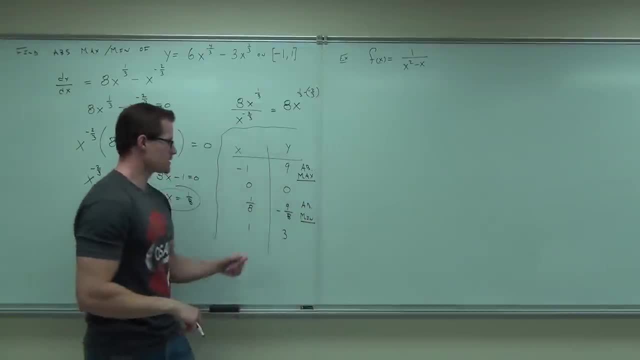 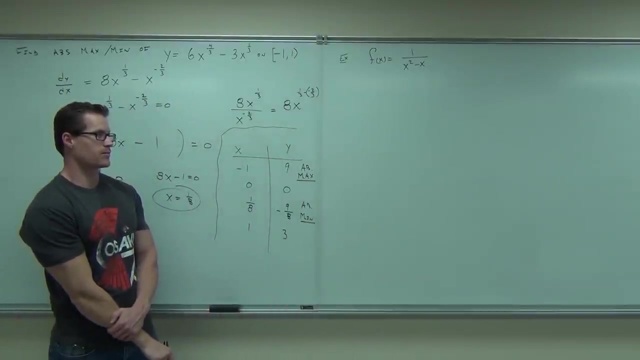 Absolute min's n occurs at x equals 1, 8.. So let's do a couple more questions here. okay, Let's say that I did this. Do I still have an absolute max? Yes, Absolutely. Yeah, that's that end point, right. 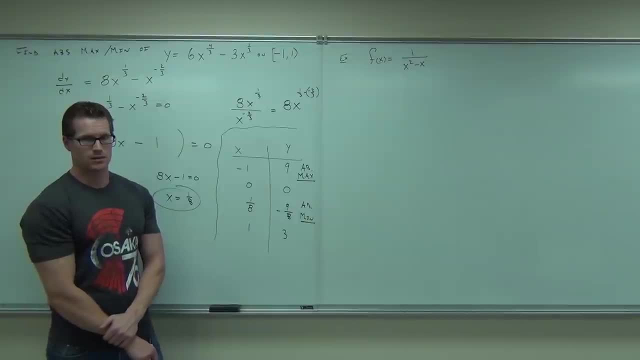 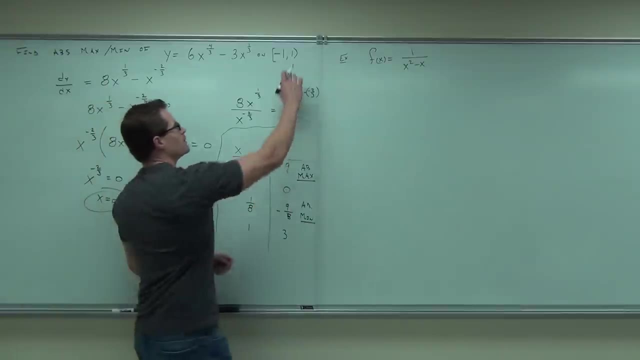 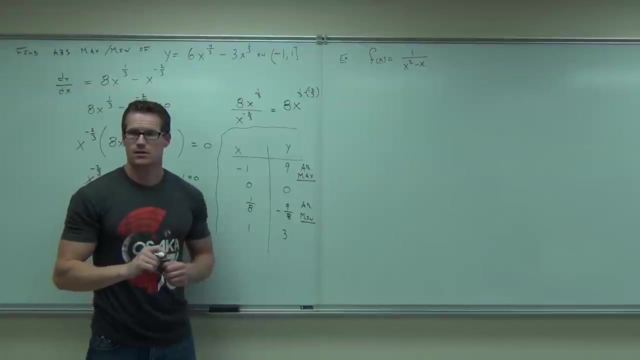 I didn't get rid of that end point. Do I have an absolute min? Yes, Min, Is that an end point? Then I still have it, That's fine. Absolute max: No, that's off the table right now. So the negative one's gone. 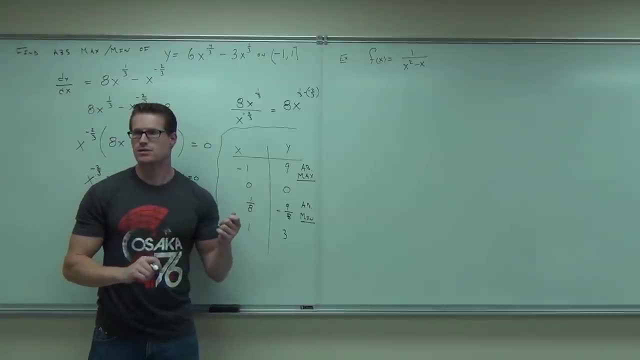 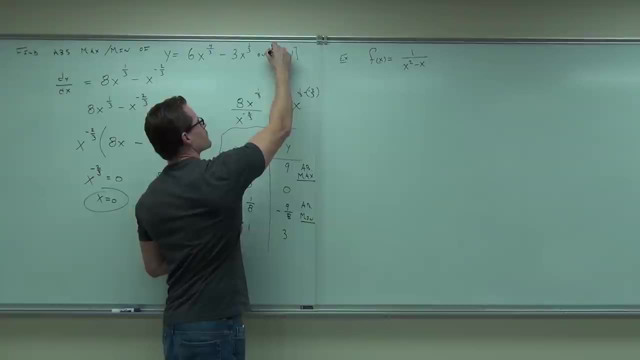 Okay, no. absolute max, Absolute min. Yes, Yes, that's still there. Okay, So are you starting to see how the end points play a factor in what you're doing here? Now let's try one more. I want to find the absolute max and min on that function. 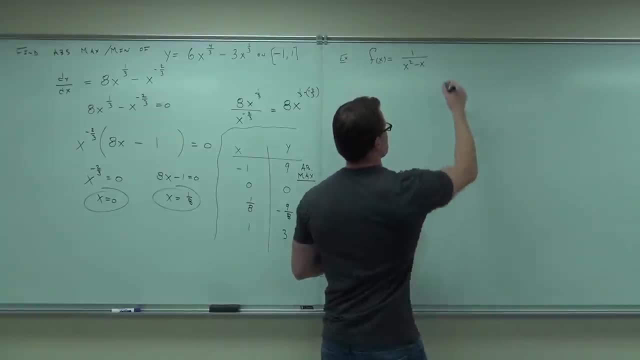 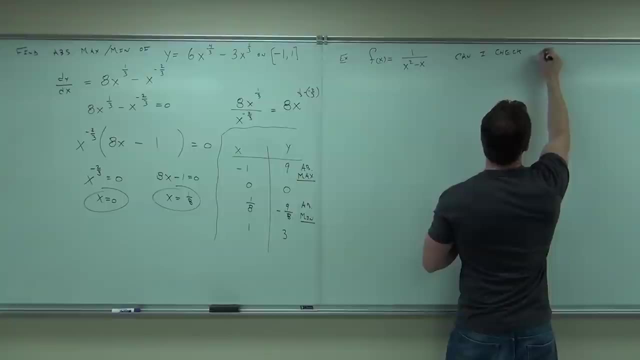 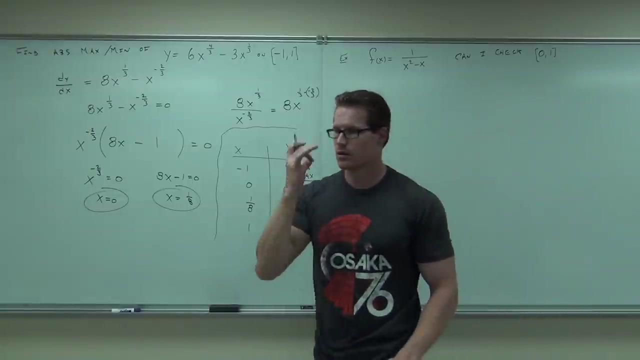 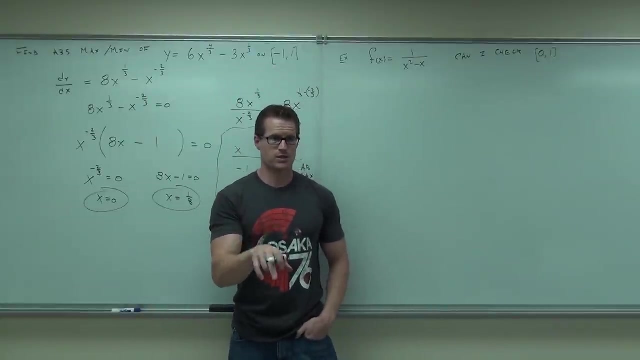 My question is: can I check this? Can I check it on that closed interval 0 to 1?? Why or why not? So if I plug in 0, I would get a 0, right on the denominator. That's not a good thing. 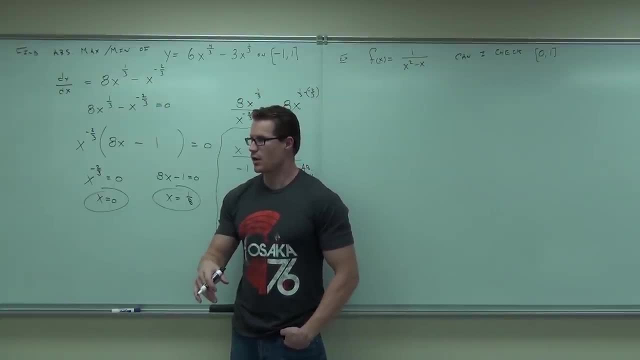 If I plug in 1, I'll also get a 0 on the denominator. Do you see what I'm saying? So on this interval, I'm not going to have any end points because those are at that spot. So I'm not going to have any. 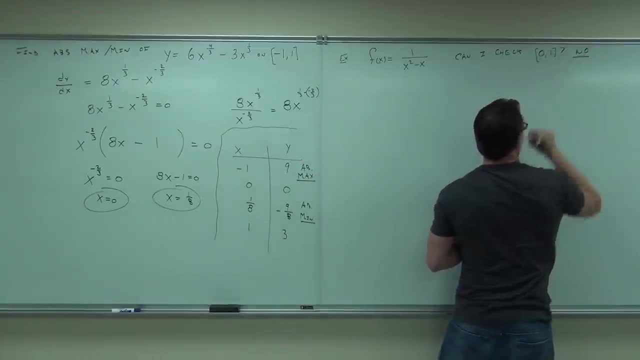 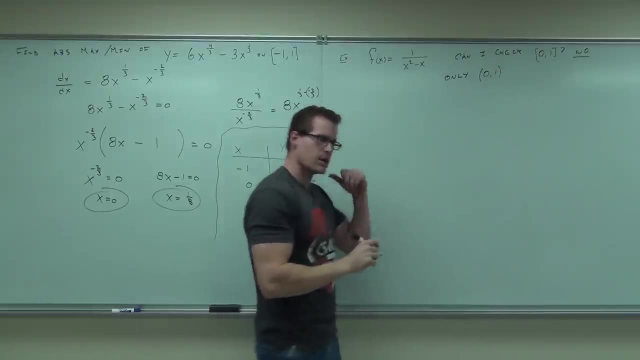 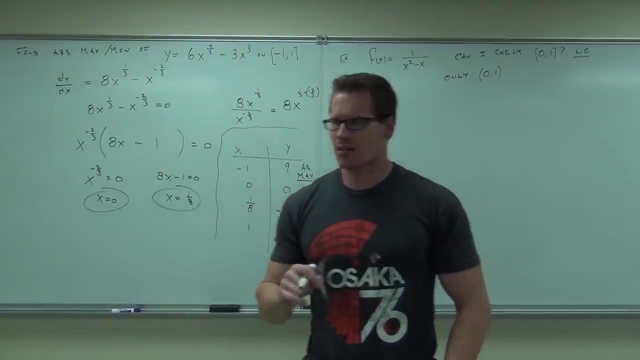 So I can't check this. Can I check this? No, No, I can only check the open interval, So, okay, well, how do we do that? Well, when we're doing something like this, it's not like you can plug in 1 and 0, right. 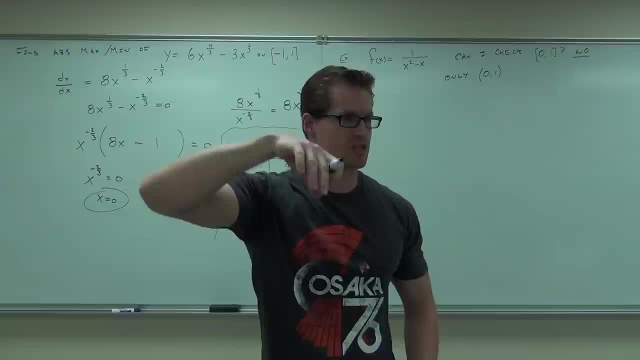 like the polynomials. You could just plug those in and see if they're getting bigger or getting smaller. You can't do that here, So what we're going to have to do is find first the critical numbers. That's what we do all the time. 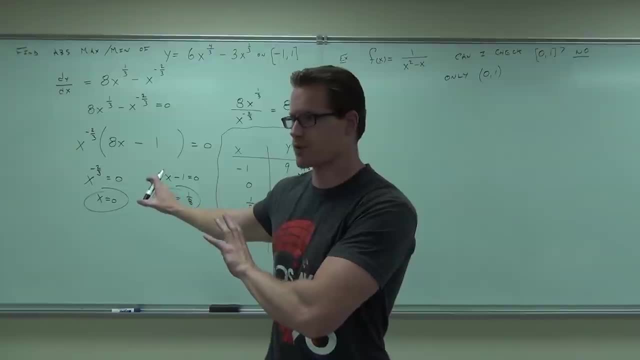 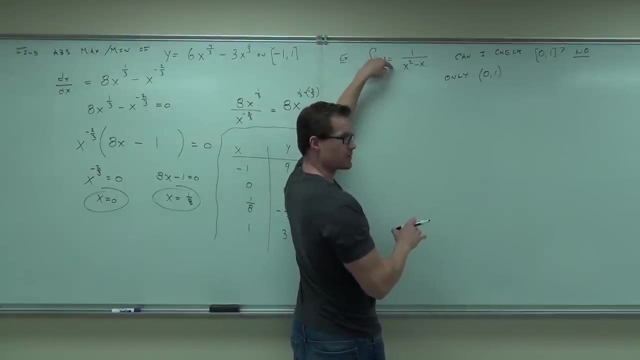 Are you with me? Find critical numbers. you said equals 0, you said they're derivative equals 0.. That's fine, But then we're going to have to take some one-sided limits. We're going to have to find the limit of this thing as we're going towards 0 from the right. 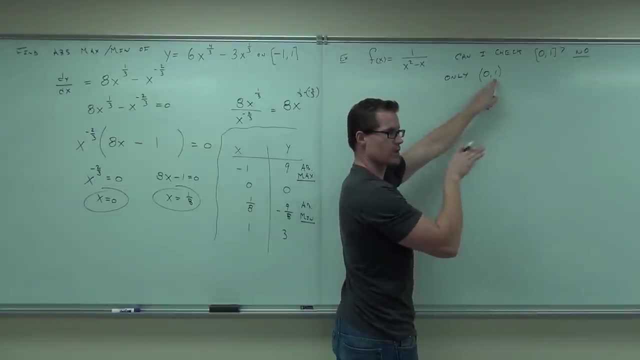 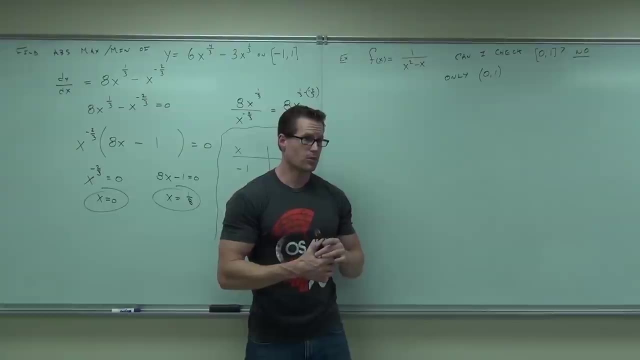 and the limit of this thing, as we're going towards 1 from the left, That's going to give us where our function's tending. Now let's stop for a second. Just think critically about this. You know that there's going to be a 2.. 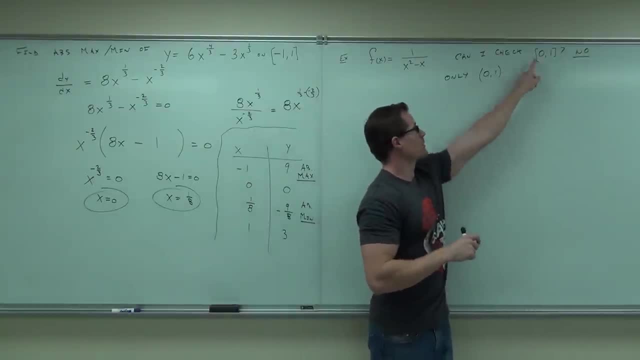 You know that there's going to be a 2. be an asymptote here and here, right. so this function is either going to be going way up high or way down low, and then way up high or way down low, so somewhere we're not going to have an absolute max or min or both. we all know. 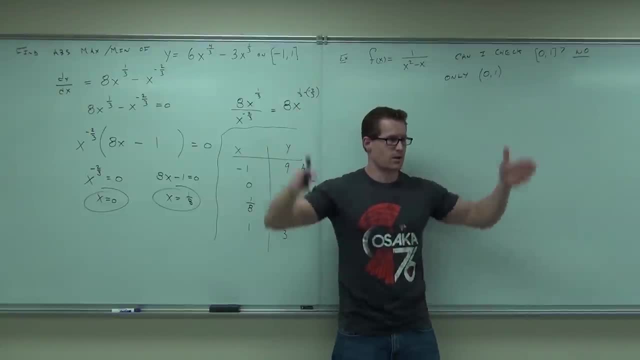 we just need the limit to tell us where it's going. it could be going like this, right? in that case, we'll have an absolute min, but not an absolute max. could be going like this: in that case, we'll have an absolute max, but not min. could go like this or like this, in which case we're gonna have nothing. you. 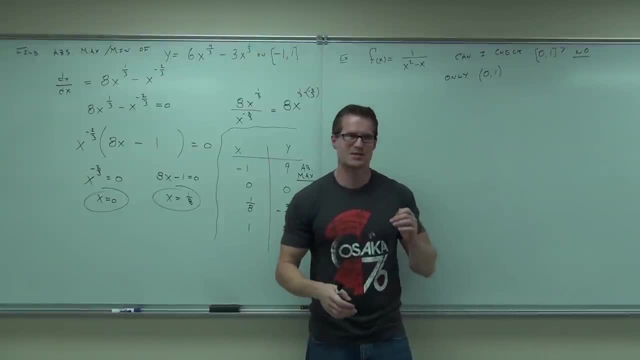 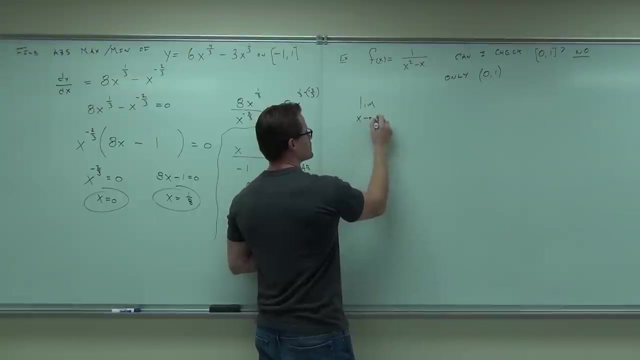 follow. so we're gonna do that now. let's go ahead and let's do that before we do the derivative, because if it's like this we're done, that'd be kind of nice, right. can we do the limits first? so limit as X approaches zero. X approaches one. 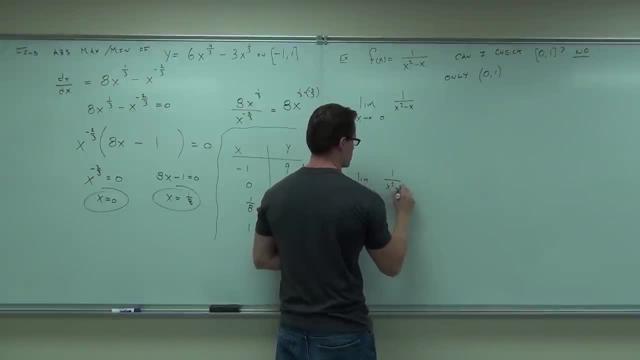 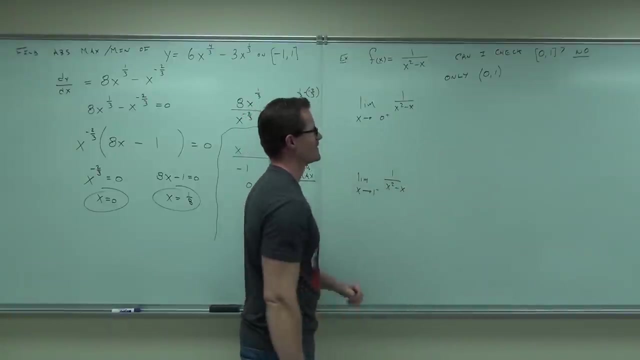 zero. are we going to be going from the left or from the right to get to zero? from the from the right? zero one you're off to get to one. you're coming from the. yeah, now let's do the limit. is there anything to factor? well, yes, yes, there is. you can factor on X. is there anything to simplify the X? so, 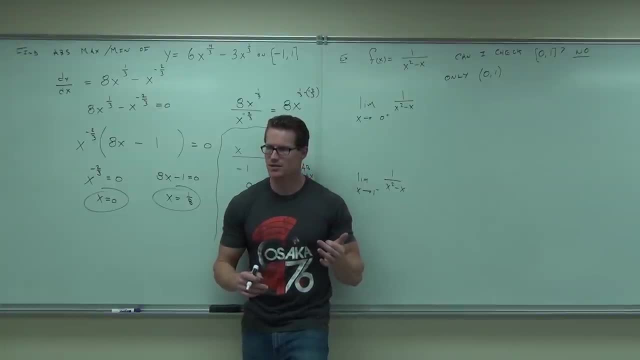 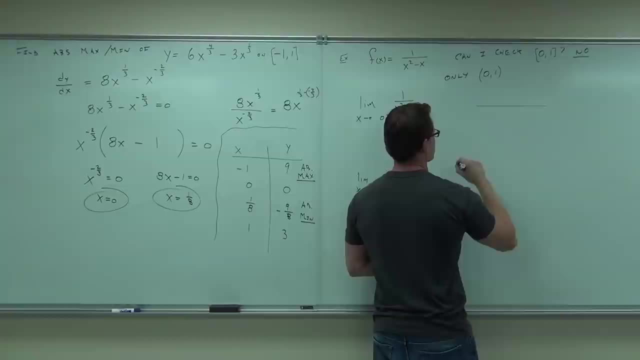 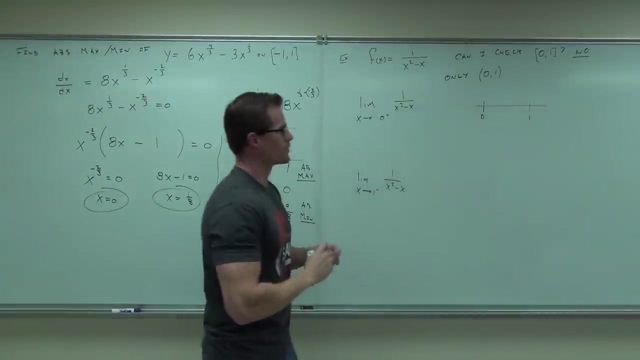 what you need here is a sine analysis. remember the sine analysis that we talked about. so if you're talking about sine analysis- zero to one- oh, you know what we might need: a derivative. actually, this is going to be as a separating point. there you can plug in a number really close to zero and see what it's doing it really 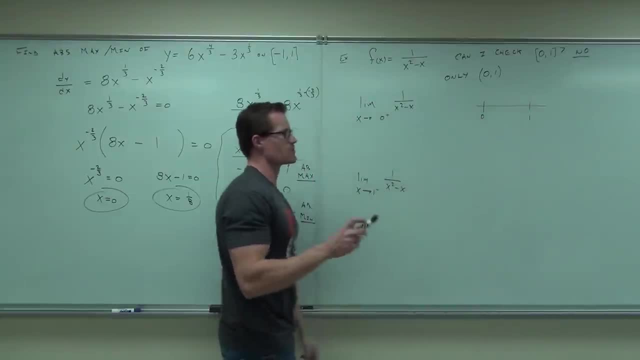 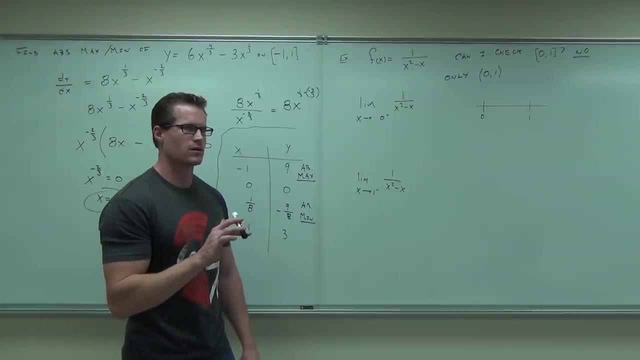 number really close to one. but I do want you to check this out. let's find the derivative and find our critical numbers and see how it plays a part here as well. it might, oh it might not play a part. no, you know what? I doubt it. plug in a. 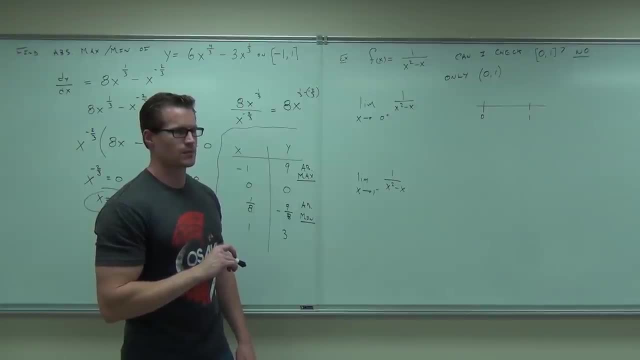 number between zero and one, would you agree that those are the only places where we actually have a problem? so it's zero to one. so anywhere between between 0 and 1, our signs are all going to be the same, true? So we're going to be either all positive or all negative. 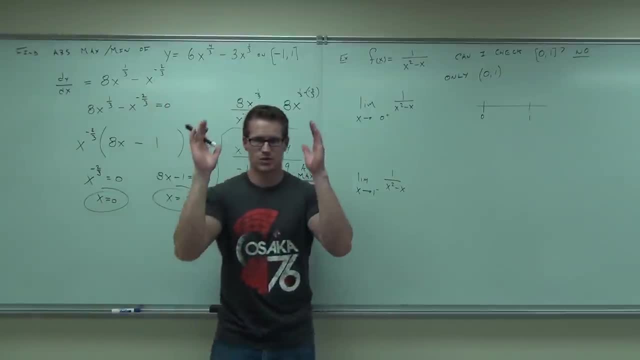 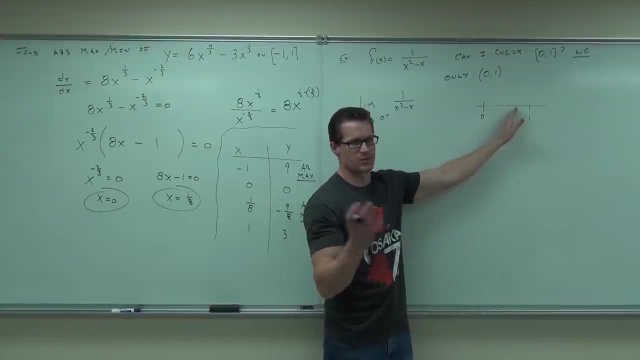 That's going to be interesting. So we're probably going to be in one of these situations: all up or all down. We don't have a separating point here. The critical number won't give us one. actually, It's just a misspoke earlier, like five seconds ago. 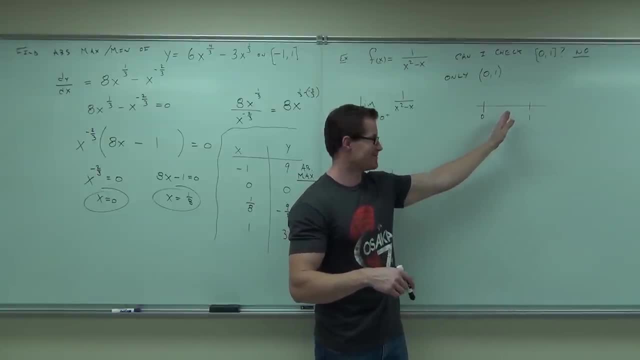 Keep track of that The only time that happens, Kidding. Anyway, since we don't have a break between there and that is our interval, these are all going to be either negative numbers or all going to be positive numbers. I'm guessing, since when you square fractions, they get smaller. 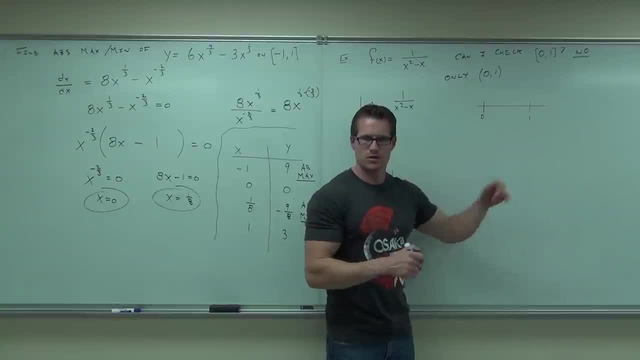 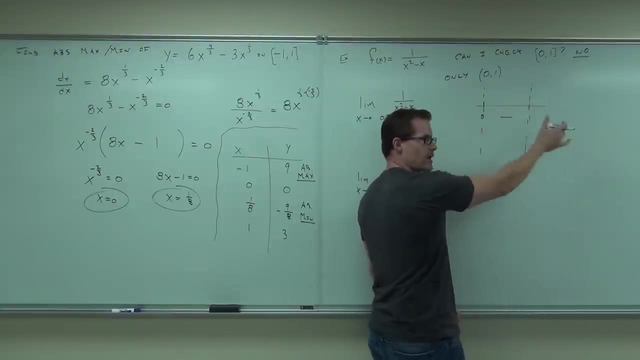 that this is probably all going to be negative. Is that true? So I've plugged in a number between here, Since these are asymptotes and we got negative the whole way across, whether you plug in 0.1 or 0.999,. 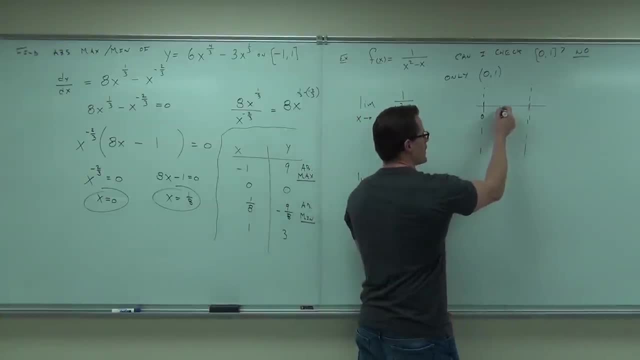 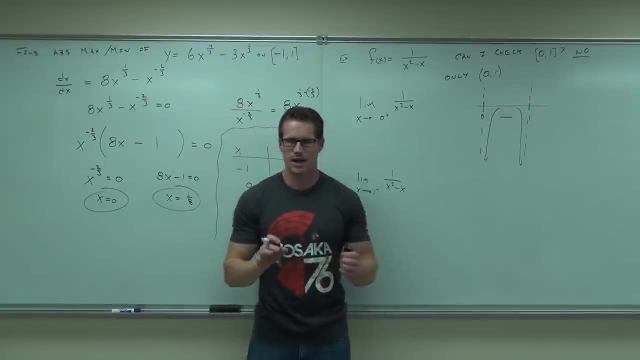 you're going to get all negative numbers. That means our asymptotes look like this: I can guarantee you right now that we're not going to have what Minimum. We're not going to have an absolute minimum. Why not? Because it goes to negative infinity for sure. 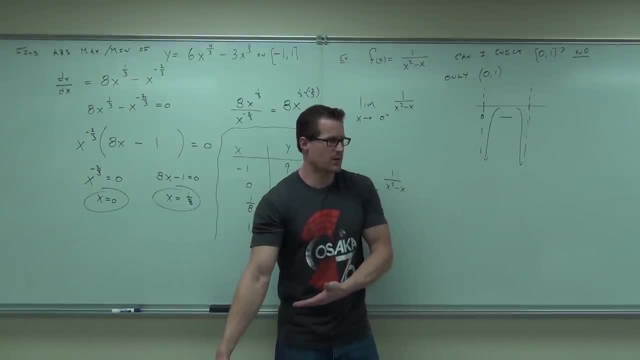 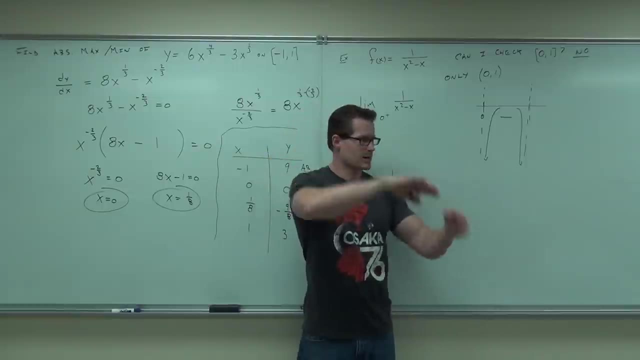 Even if one side went to negative infinity, it still wouldn't have an absolute minimum. You okay? Which one will we have? Why It's going to come up and it's going to go back down, That says, on a continuous function. 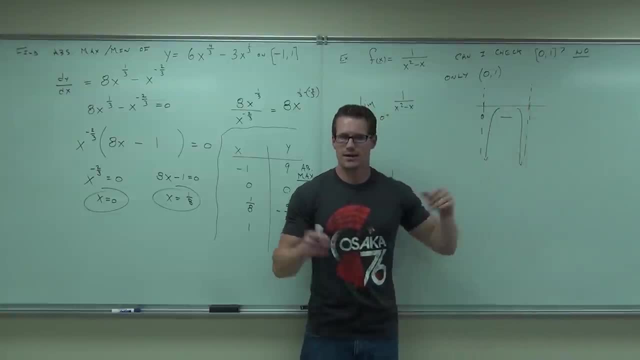 which this one is in that interval that's continuous, in that interval That says I will have an absolute max there. How do we find it? That's where the first derivative comes in. Do you understand this? This said: coming to 0 from the right gave you negative infinity. 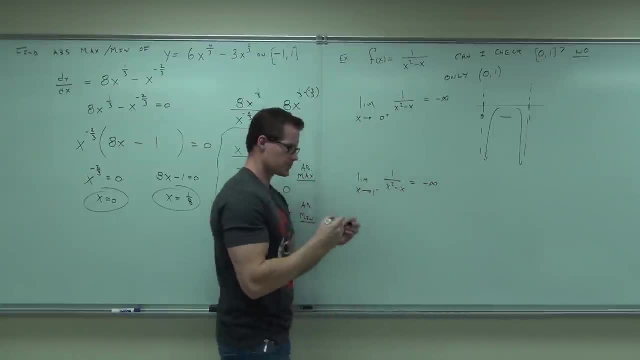 Coming to 1 from the left gave you negative infinity. Negative infinity is way smaller than any number you could find, so that means there's no absolute minimum. That's going to the same place. No absolute minimum. They don't have to go to the same place, okay. 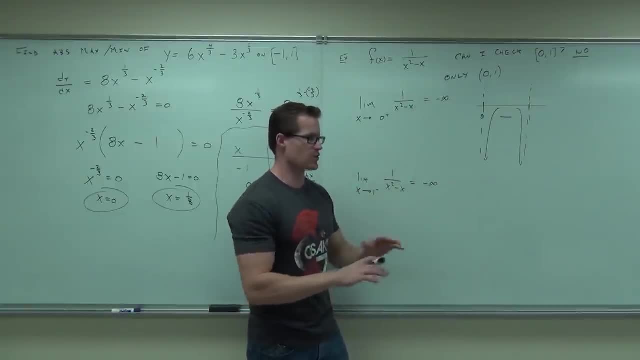 They go to positive infinity, But this just says that in both cases you're not going to have an absolute minimum. Do you follow? If this one had magically gone to positive infinity, we'd have neither, If they'd both gone to positive infinity. 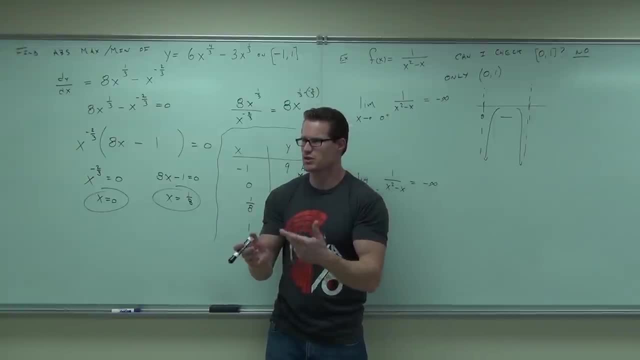 we wouldn't have an absolute max, but we wouldn't have a min. Are you with me on the logic there? So find these first. That might be a great way to do it: Eliminate some of your problems or eliminate some of your choices. 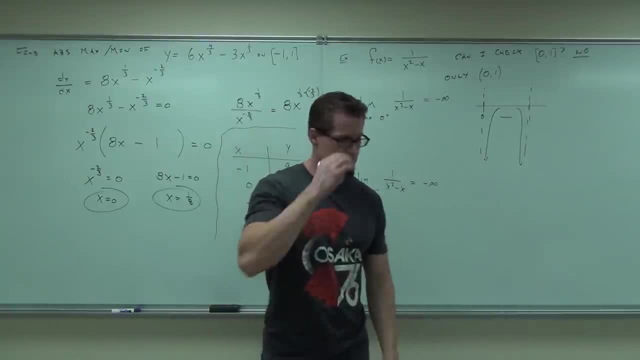 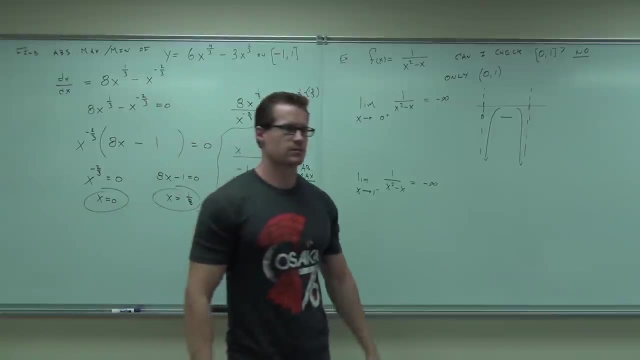 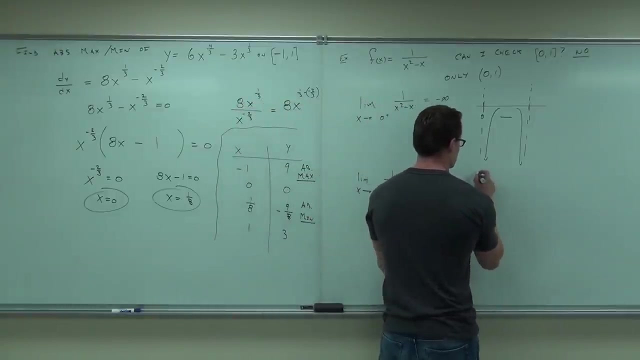 We're not going to have an absolute min, We're just going to find the first derivative. There's a couple options. You can move that thing up top and make it negative. 1. You can do a quotient rule. So if you're going to have a positive min, 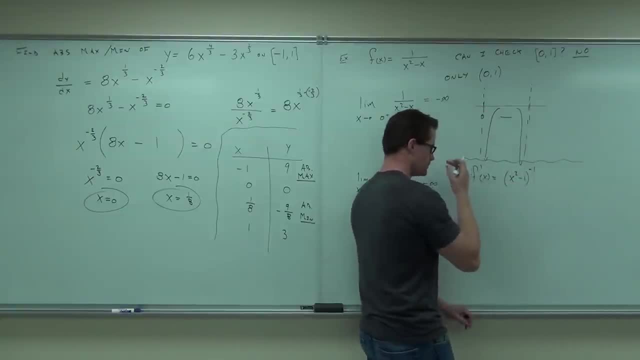 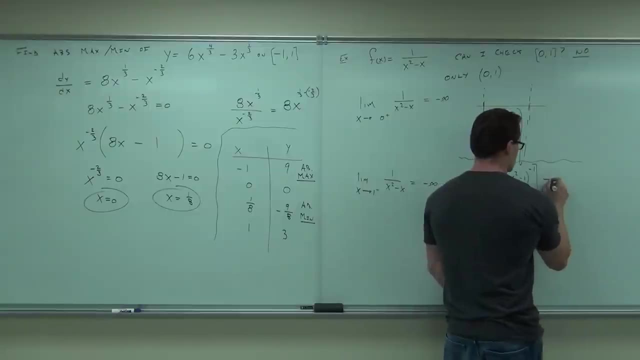 We're going to create something called a quotient rule. So you're going to create a quotient rule And the quotient rule is going to say, if you move a negative min, It's going to be negative 1 for twice. So you have to make it negative 1 for 100%. 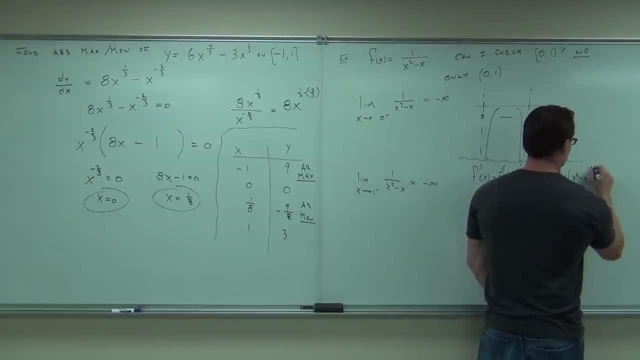 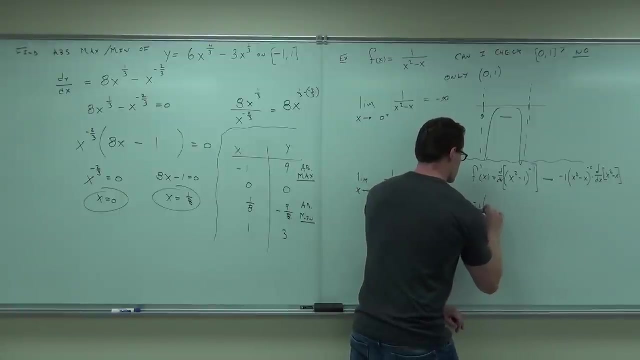 You don't want a negative min, So you're going to create a quotient rule. What you're going to do is that you're going to do a quotient rule. Hopefully, you're able to find about the same thing. By the way, some of your negatives are nasty. 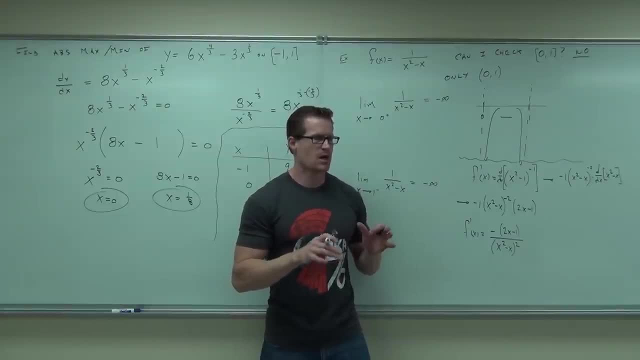 Some of you are ruining some of your problems based on your negatives, especially distributing your negatives on your implicit differentiation. So when you get that homework back it's already graded. I've looked at it, but it's just too much to pass around in one day. 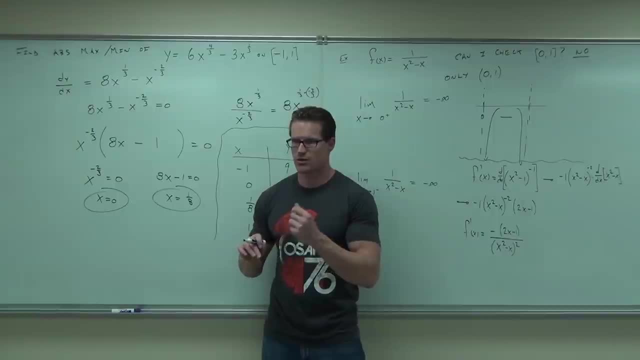 There's a lot of it. So when you look at that, check out your – I've circled your negatives. You're just not distributing negatives. Be careful on that stuff, Like here. if you don't have that parentheses, you put a negative up front. 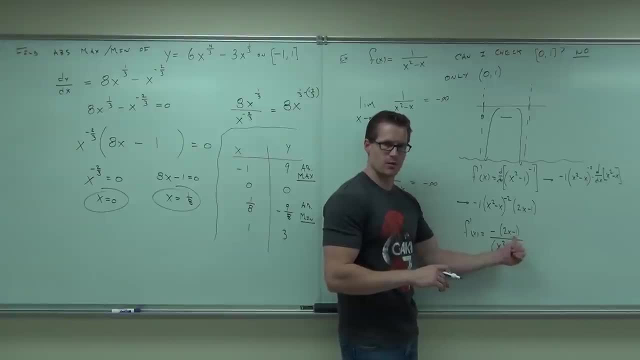 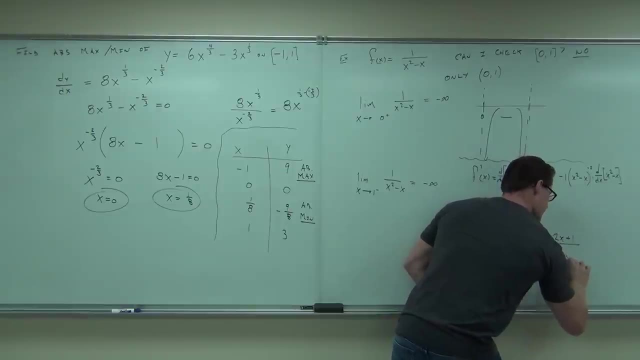 Without distributing. you're going to be wrong on that plus 1.. Do you see what I'm saying? Do you see what I'm talking about? You'll be wrong there. So here this is definitely negative: 2x plus 1 over x squared, minus x squared. 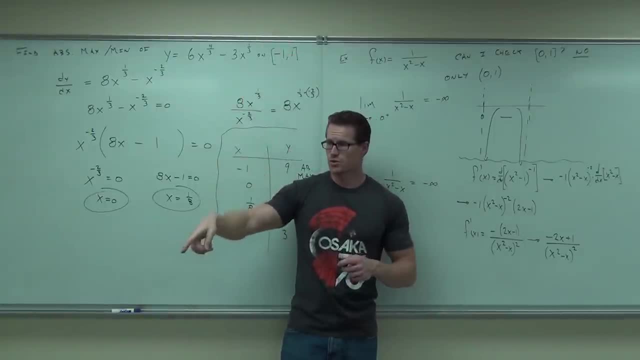 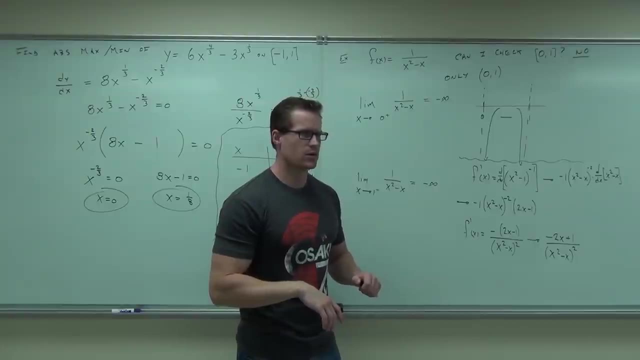 Show of hands. how many people were able to find that derivative? If you did the quotient rule, you'll get the same thing. You just have to distribute okay, And you'll get negative 2x plus 1.. Did anyone do it that way? quotient rule. 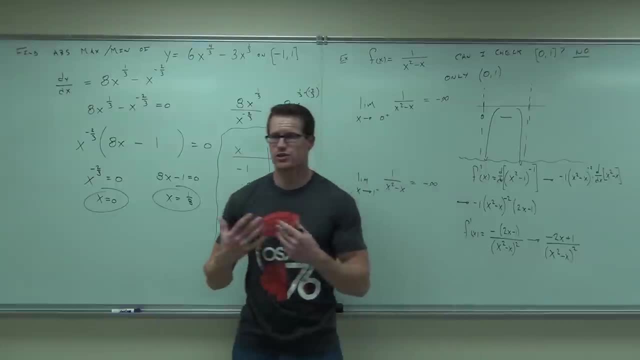 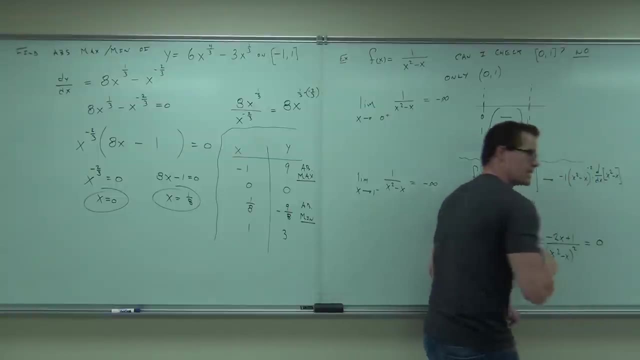 You got the same thing, Perfect. What do we do with our first derivative in order so that we find our critical numbers? What do you set equal to? So do that. What do you set equal to 0?? Now, even though that looks really really nasty, think about something. 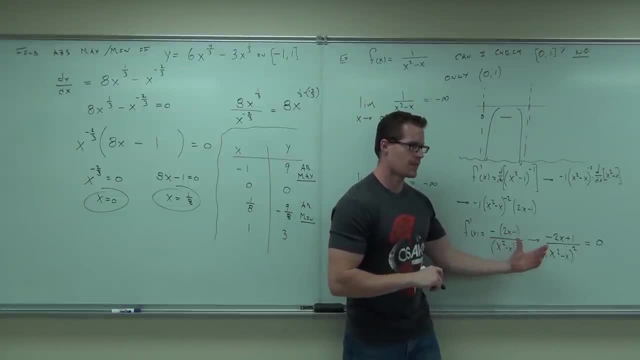 Just think: Where could this possibly be equal to 0?? It's not where the denominator equals 0, because that's going to give you undefined points. In fact, that's just going to be 0 and 1 again, isn't it? 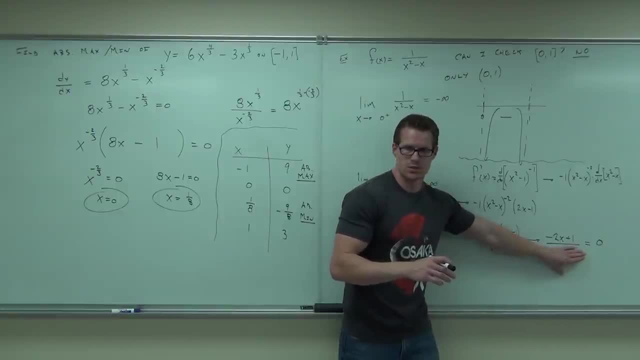 So the only place it could possibly be equal to 0 is where the numerator equals 0. So when you're solving rational equations like this- is which you've done before- you just have to set the numerator equal to 0. And that, in this case, is very easy. 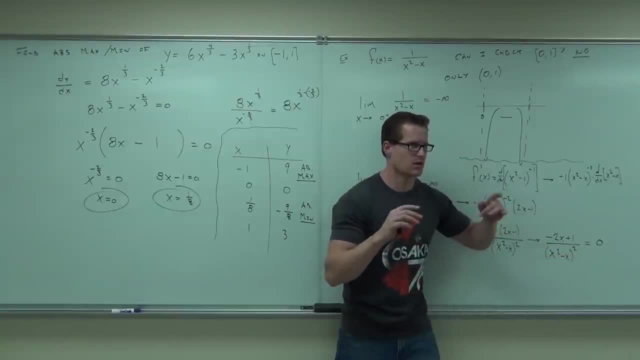 Which, by the way, you remember when I had you do all the distribution on quotient rule And you're like, oh my gosh, do we really have to do that? Can we just leave it in parentheses? No, because you have to solve it. 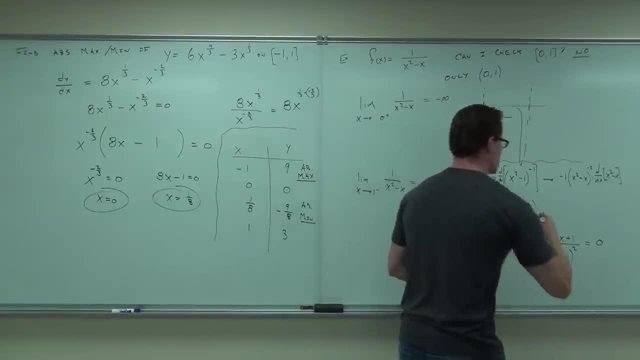 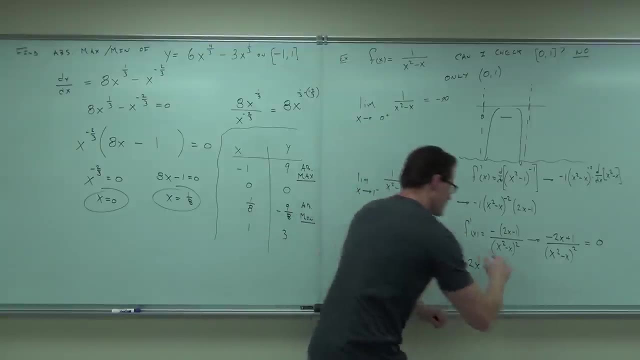 So you're going to have to distribute it anyway, So you may as well do that. You're going to get negative. 2x plus 1 equals 0. Subtract 1, divide by 92.. x is 1 half. Show of hands: how many people feel OK on getting the? x is 1 half. 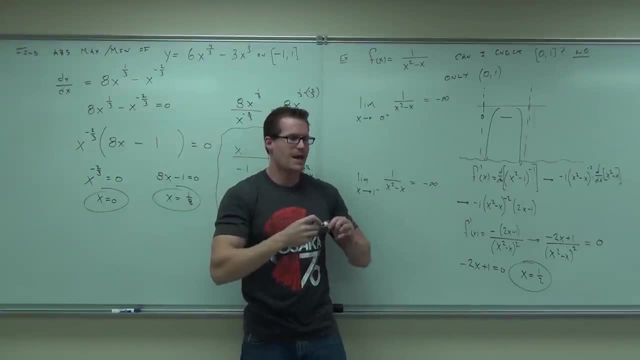 This row. are you guys OK on this? All right, Hey, x equals 1 half. Is that in our interval? You should check that, right? You should probably check that. So that's in our interval. That means, with that interval we are certainly, as I magically predicted, we're going to have some sort of a critical number there. 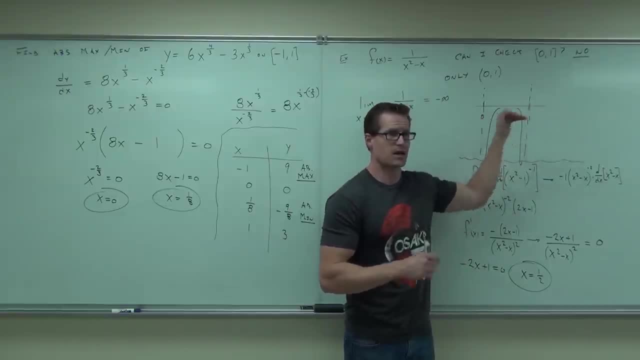 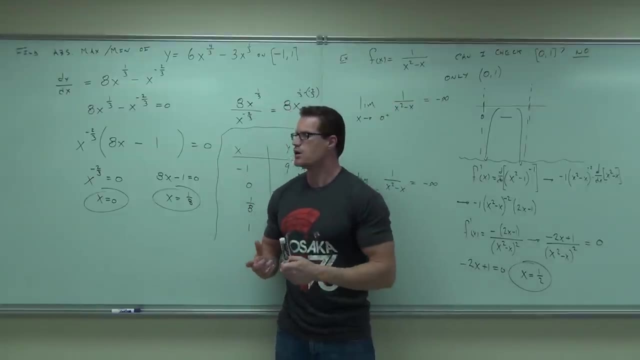 Because we were down here. we're down here. It's got to reach a peak at some point, at least one peak. How do you find that peak? Plug it in. Do I need to check my endpoints? No, Do I have any endpoints? 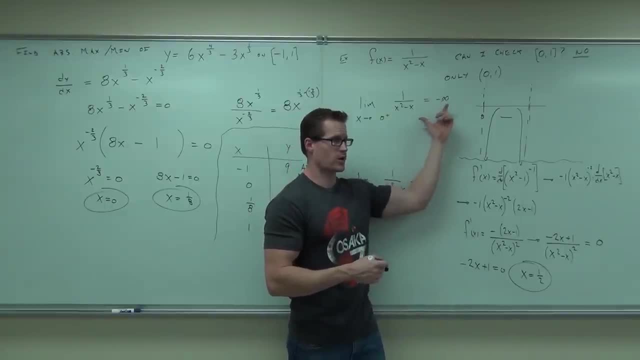 No, We've already done that work. first. We know that our endpoints are going to keep going down forever. So all you've got to do with this, since you know it's going down forever, you know for certain that is going to be an absolute max. 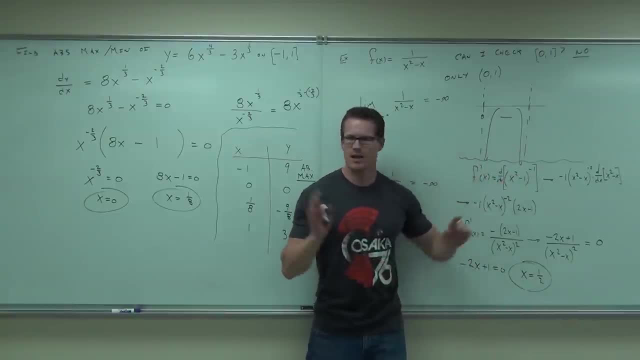 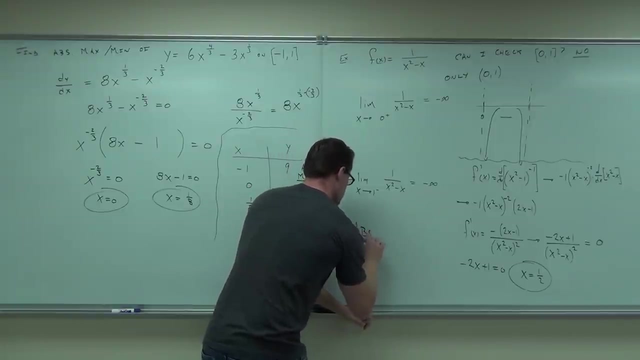 It's continuous. This is negative infinity. That's negative infinity. It has to go up, It has to come down, since it is continuous. So you just plug in 1 half, Whatever value that is, that's an absolute max, Negative 1. fourth: 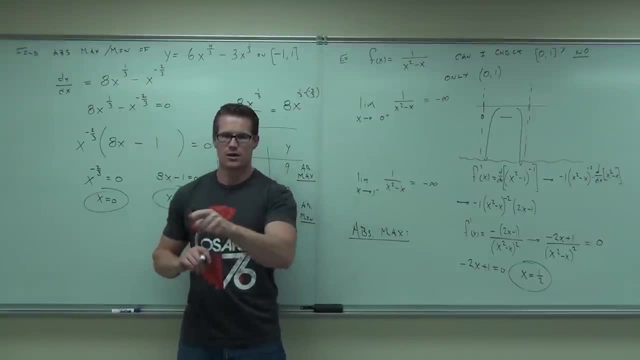 What did you get? Negative 1 fourth. Anybody else get negative 1 fourth. Yes, You plug it into. well, not your derivative right? That would just give you slow Plug it into here. So is the absolute max 1 half or is the absolute max negative 1 fourth? 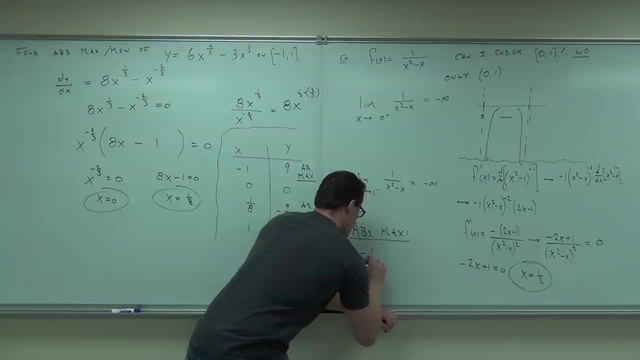 Negative: 1 fourth. Negative, 1 fourth. Wait a second, It's actually 4.. I don't know. It's 1 fourth on the bottom: Negative 4. Negative, 4. Negative 4.. I was just taking. 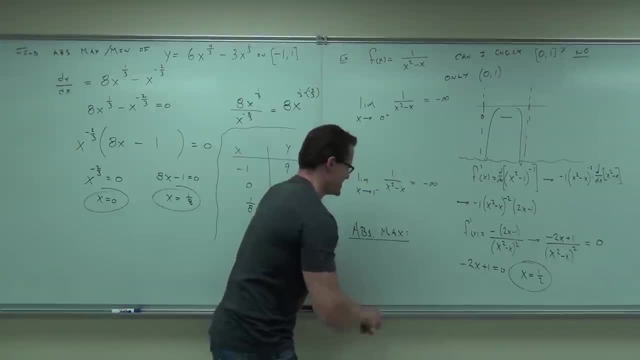 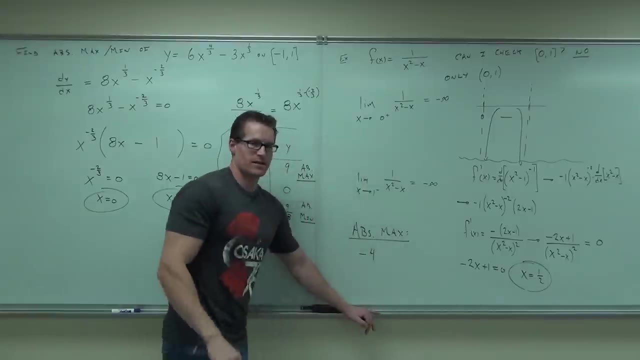 Whatever I was just plugging it into the end, It's all good, It's all right. You reciprocated. You're going to get negative 4.. I forgot about that Is the absolute max. negative 4 or 1 half. 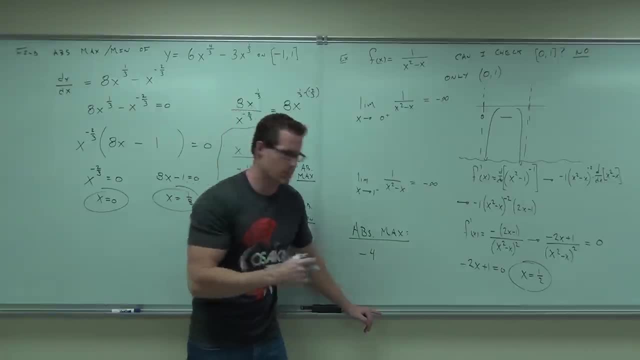 It's negative 4. It occurs at x equals negative 1 half, So at sorry, x equals 1 half And that's your absolute maximum for that function. Can you do it? Yes, How many people feel okay with what we just talked about? 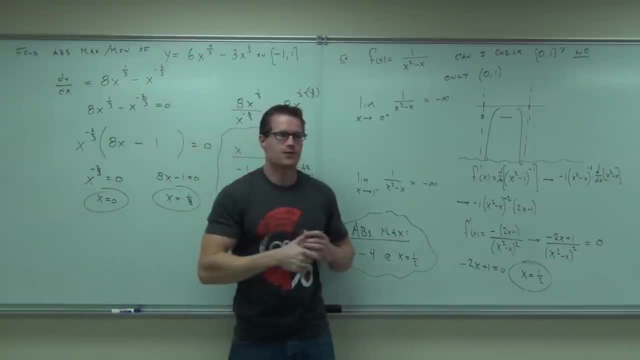 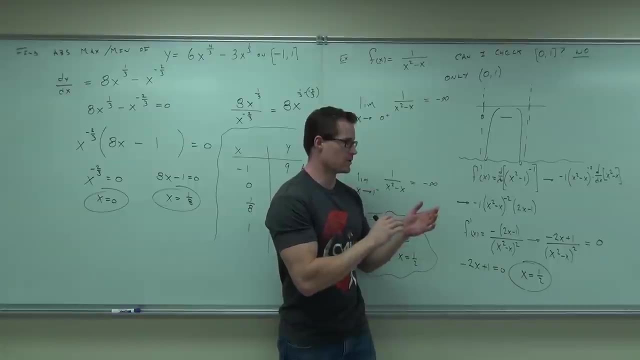 Yes. So our ideas are: if you don't, if you have one of these weird functions, man, and you can't plug in the endpoints you're going to, if you can't plug those in, if it's not a polynomial and you literally can't plug it in, do your sign analysis. 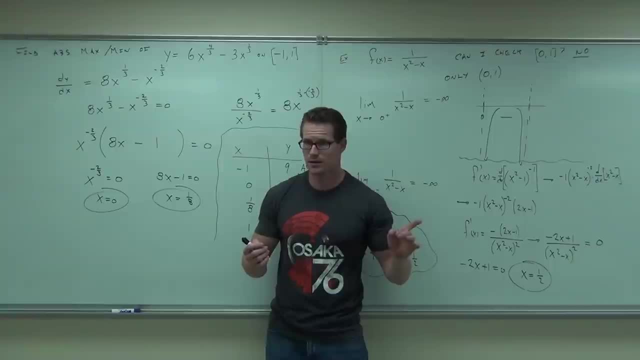 You know they're going to be asymptotes. right, We've talked about that. You know they're going to be asymptotes. They're either going to do this, this or this. They're going to do one of those things. 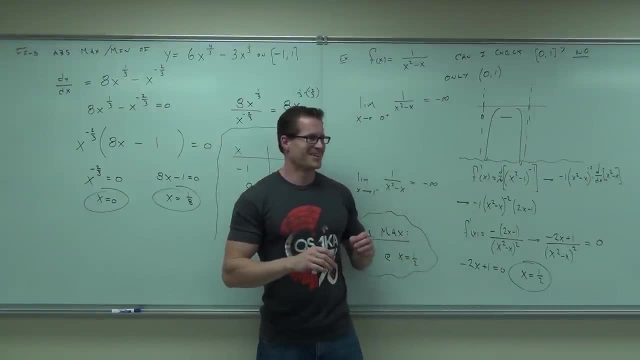 It's like dance moves. That's what it's going to be. It's going to do this. It's going to do that. It's going to do that. It's going to do that. It's going to do this. It's going to do that. 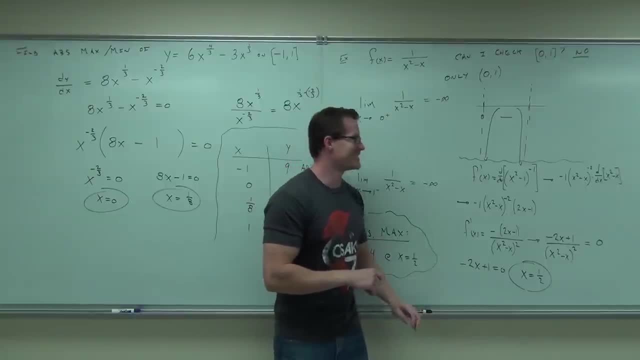 It's going to do that, It's going to be, It's going to do this or this or this. I'm so awesome at dance, by the way, I'll do my calculus dance, So you know you're going to eliminate some of your choices here. 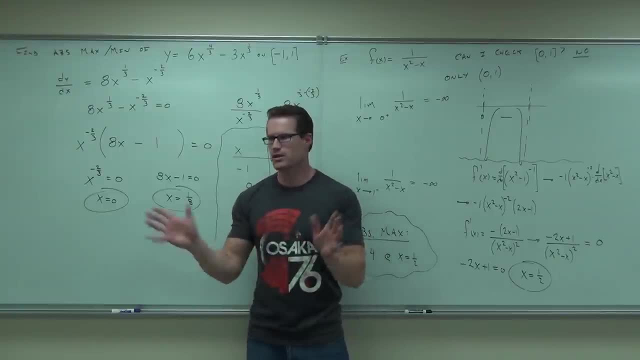 So there won't be minimums and maximums in some cases. Then you find your derivative. then you know what you have after that. If you get a minus and a plus, then you're done. You're done. Those are nice problems. 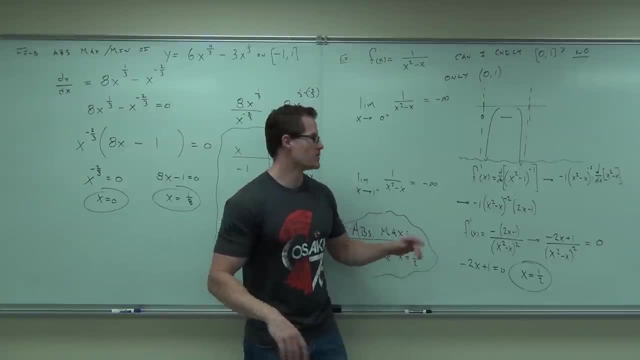 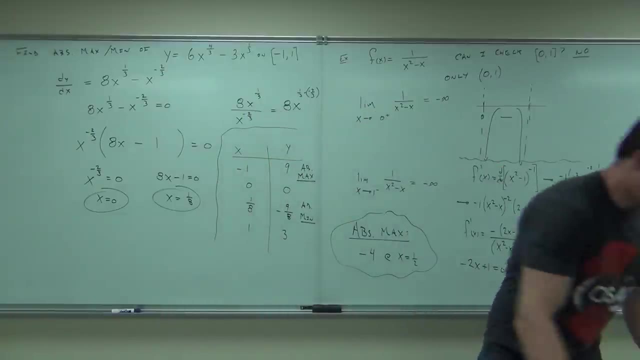 Those won't happen very often. They're often, but those are nice problems. Most of the time you're gonna get this or that. otherwise the problem is kind of stupid, right? Anyway, Do you have a good feeling about absolute maximum?